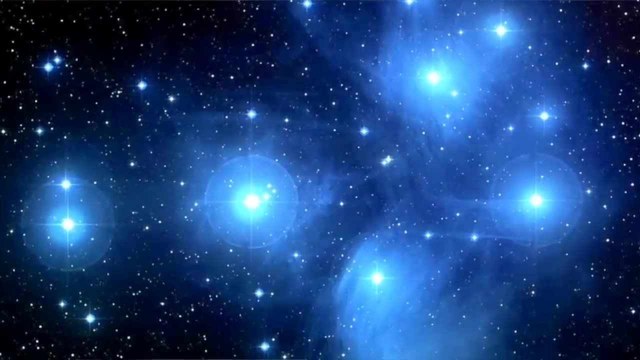 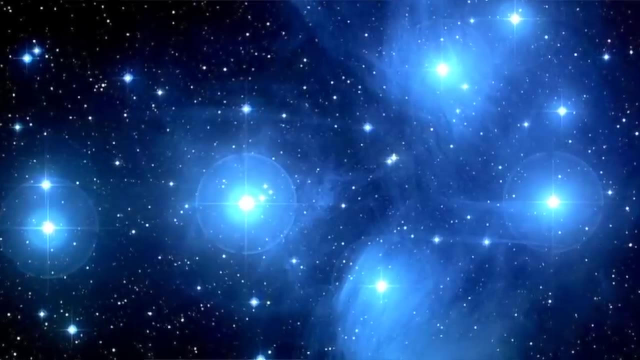 change. They're things that shine by their own light. They have nuclear fusion going on in the cores. They are much more massive than planets, much bigger In fact. stars tend to be hundreds of thousands of times, tens of thousands of times massive, more massive. 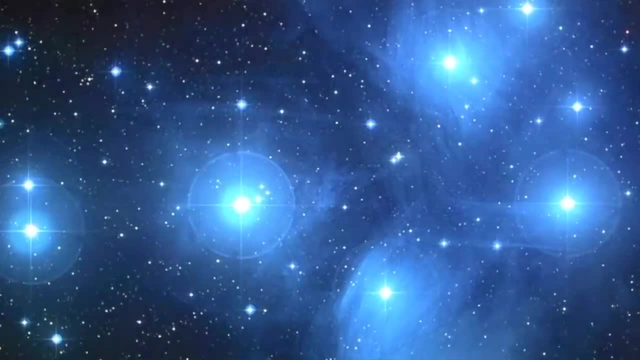 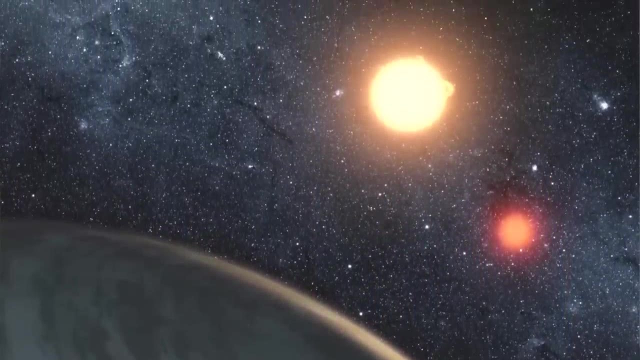 than planets And they actually live for much longer periods of time And they're the center of various solar systems. In all cases, all planets orbit a star. Now there can be rogue planets that for some bizarre reason are flung out, But in general, planets orbit stars. 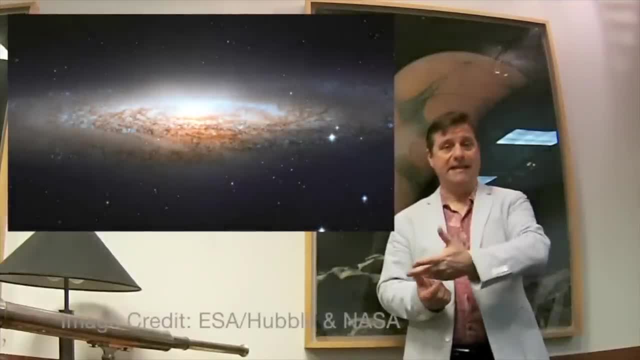 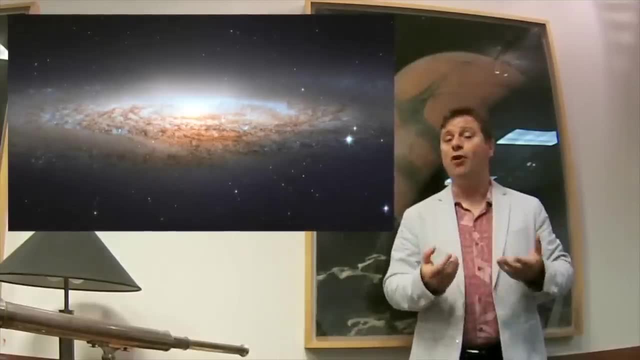 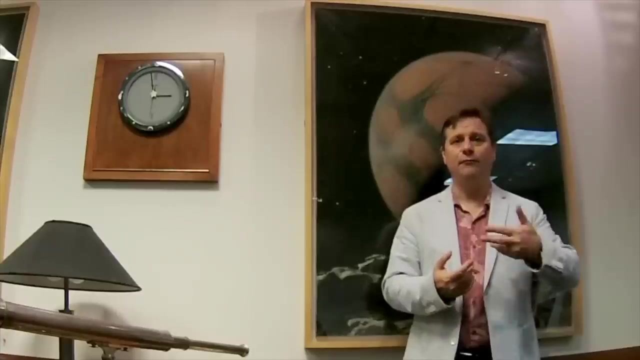 And that's one of the definitions. Okay, so stars then come in great, huge groups. Hundreds of billions of stars can all group together and be part of what we would call a galaxy. Our Milky Way is such a galaxy. The Andromeda Nebula is such a galaxy. M101 and M31 and M74 are such kinds of galaxies. 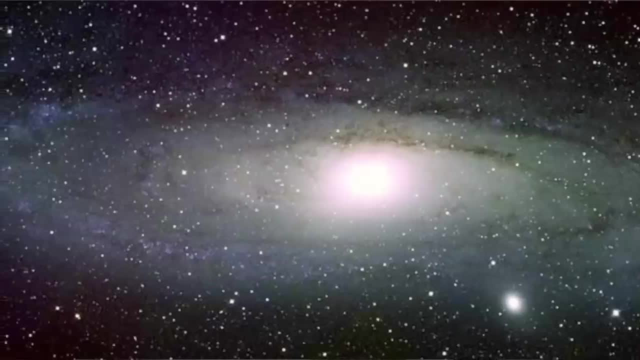 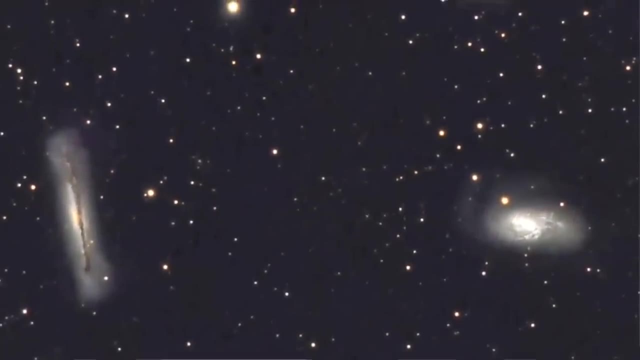 And these are wonderful objects to go out and see. They're very, very distant, And the spaces between them are enormous. The sizes of galaxies tend to be about hundreds of thousands of light years across, And they're separated by such distances as well, Now bigger than 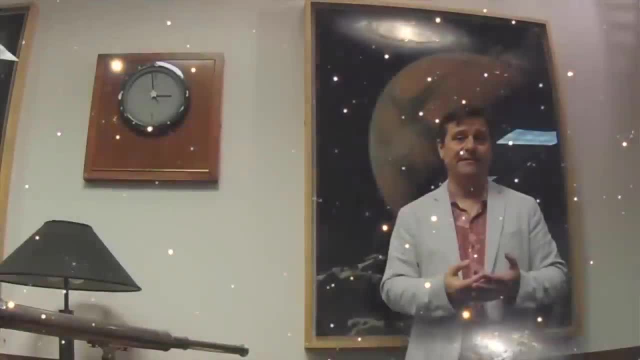 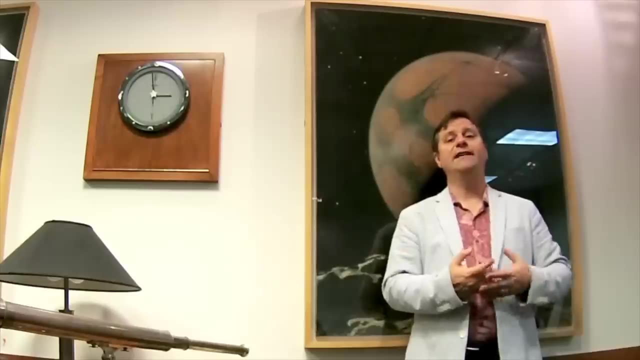 that is, the construction of hundreds of billions of galaxies, And the hundreds of billions of galaxies that are out there. we would call that our observable universe, And when we get to later chats we'll learn that the observable universe is a thing, that which we can see. 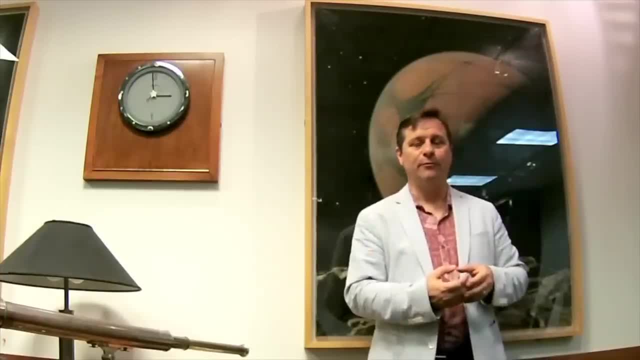 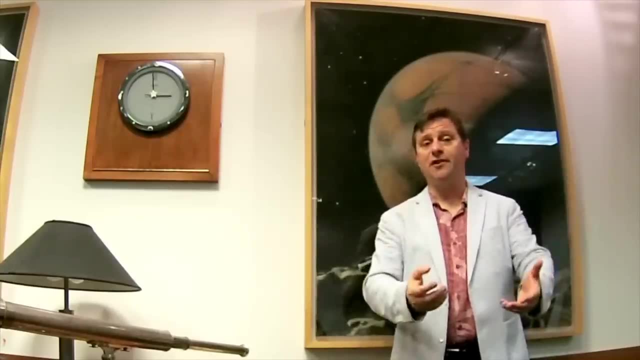 So there could be more stuff that we can't see. But, more importantly, the observable universe is that which we can see. So the observable universe is composed of galaxies. these are composed of stars, and stars have planets orbiting them and creatures like 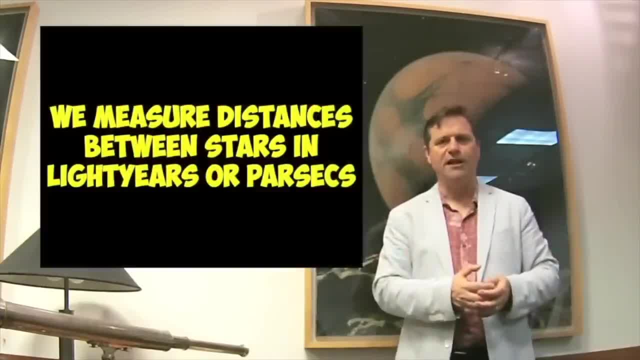 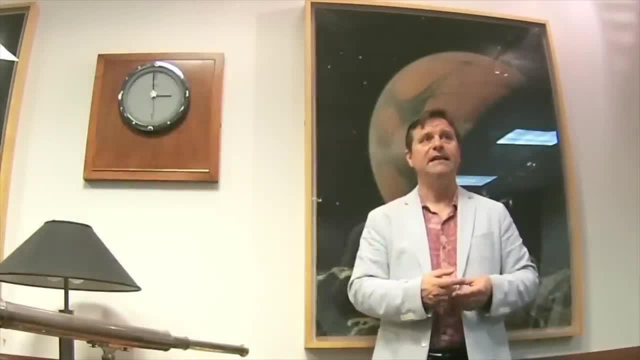 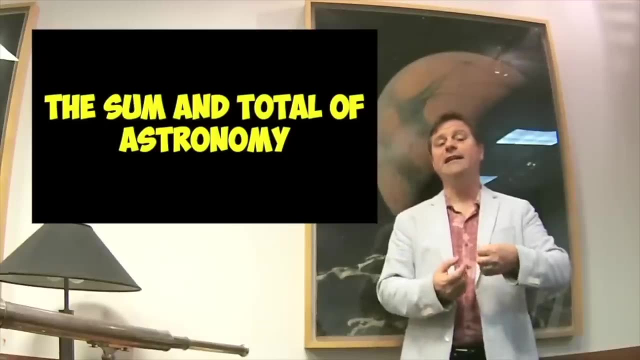 us live on. planets And stars are very, very far apart, separated by trillions and trillions of miles, which we tend to measure in light years or parsecs as a distance measurement. So astronomy is the subject matter that covers all these types of objects and tries to define 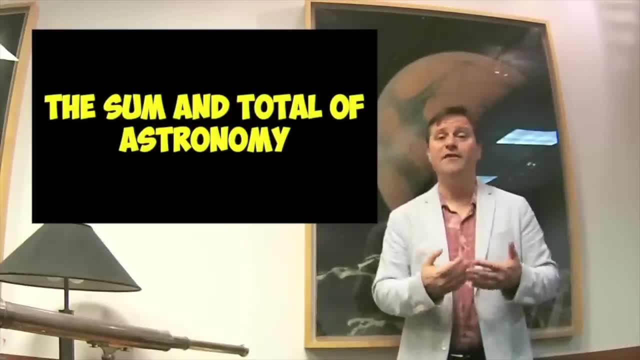 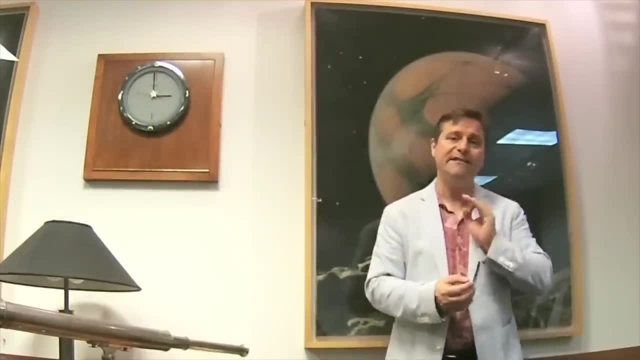 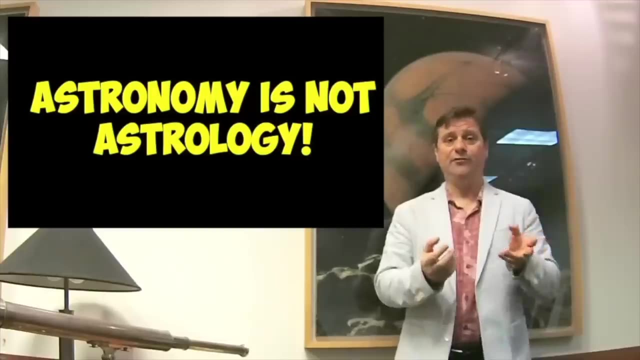 how they're born, how they live, how they die, what they do when they're living, how they actually come to be And what processes by which they act. Astronomy is not astrology. Astrology is looking at the stars and trying to decide whether or not your future shall be bright or dim. Basically, 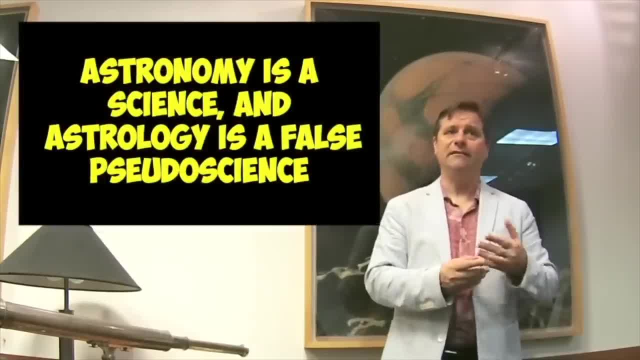 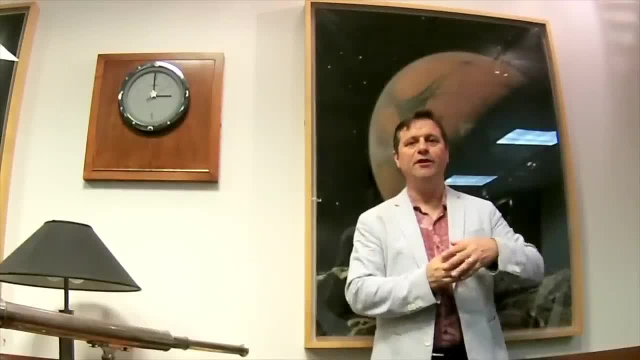 astronomy is a science and astrology is a pseudoscience, So we can kind of dismiss with that immediately. Well, one of the first things that we want to do when we study astronomy is we go outside and we look up, And when we look up on a very, very dark night, we see a star. And when we look up on a very 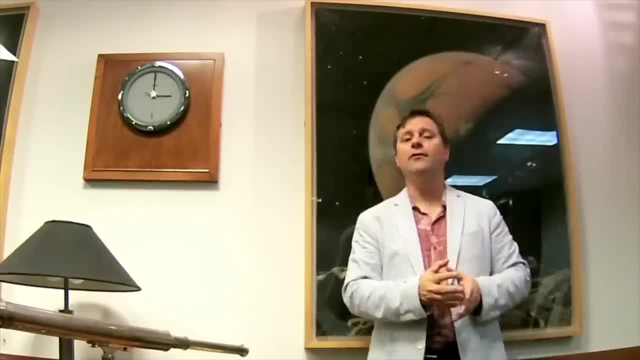 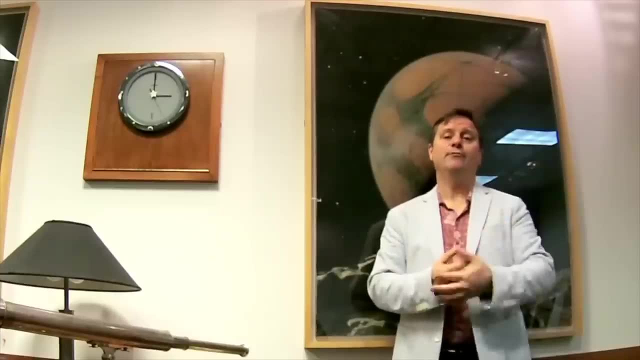 clear sky somewhere, way deep somewhere. Maybe you're on the tops of the islands of Mauna Kea, maybe you're out in the desert, maybe you're in a city, or maybe you have the opportunity to go to someplace dark like Cherry Springs State. 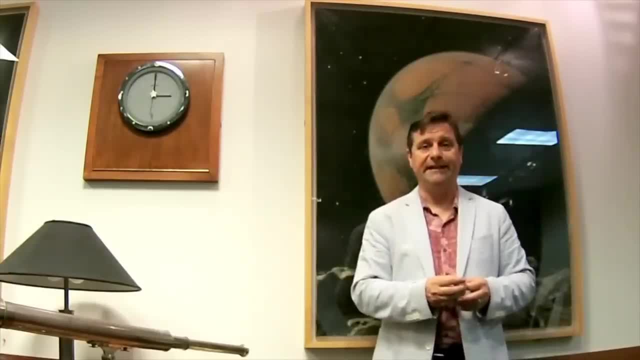 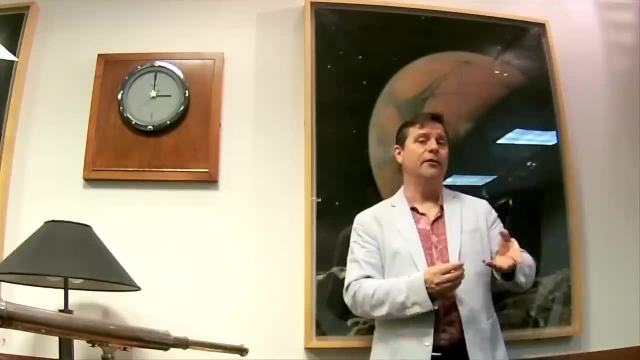 Park, which is in northwestern Pennsylvania, a gorgeous place to go stargazing. And when you look up, you see a dark sky and you see stars. You'll notice that stars come in these patterns that you'll see year after year after. 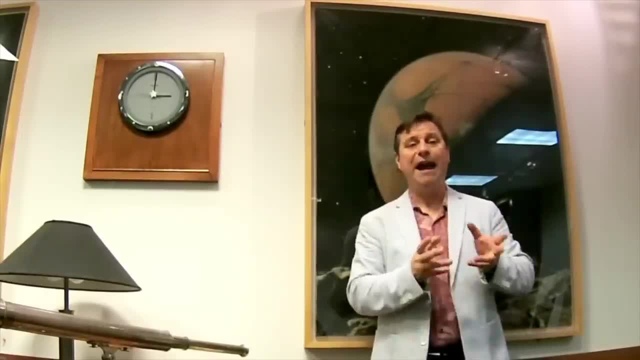 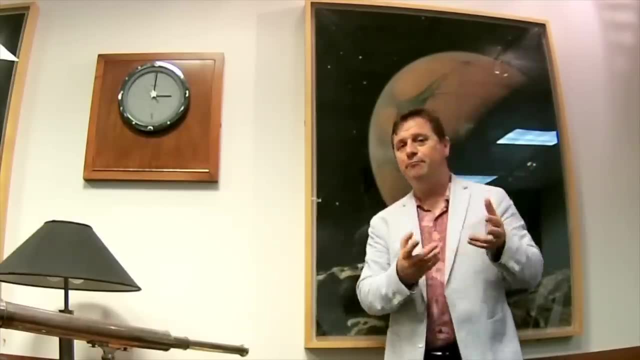 year at the same time of year And in the patterns of the stars. we can link them together with little lines that we pretend that they're there. We can group them together, make pictures out of these dots and then we can call them. 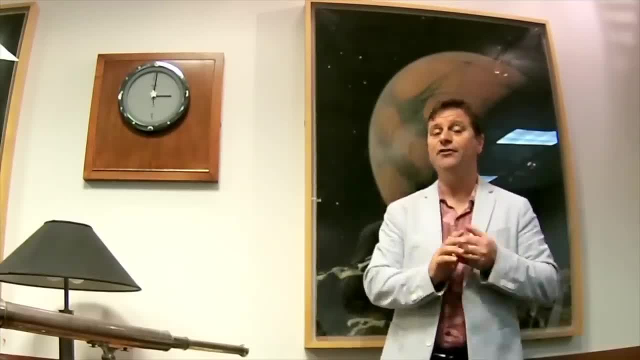 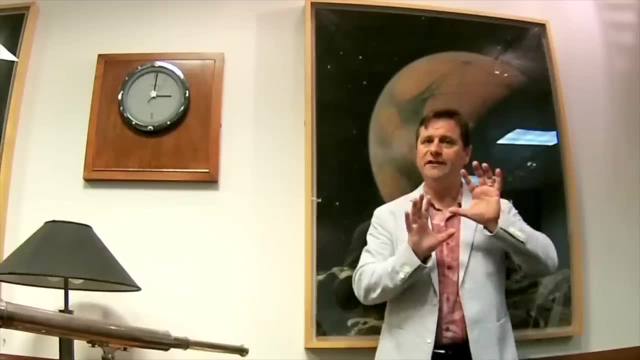 constellations. A constellation is an apparent grouping of stars in the sky. They don't necessarily have to have any relationship to each other- the stars don't- but they just are in the same direction of the sky. And when we look at constellations, there's some familiar ones that we know of. 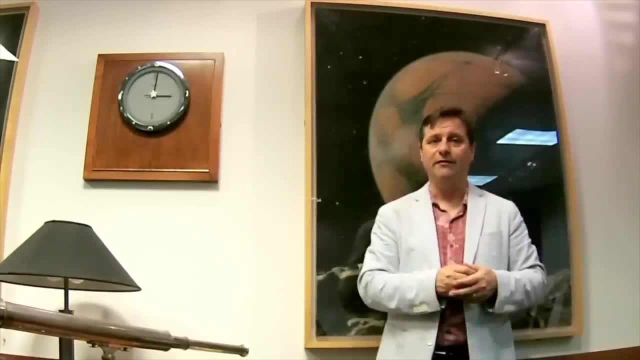 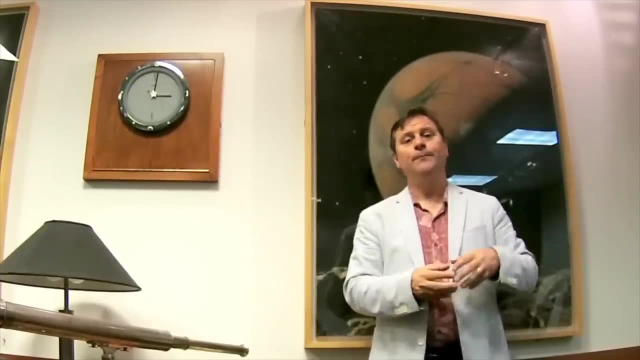 Such as Orion, with the three belt stars and the four around it, and then you have the Big Dipper, which is part of the large constellation Ursa Major, the Big Bear. Well, if we look, how many stars can we see? if we look up in the 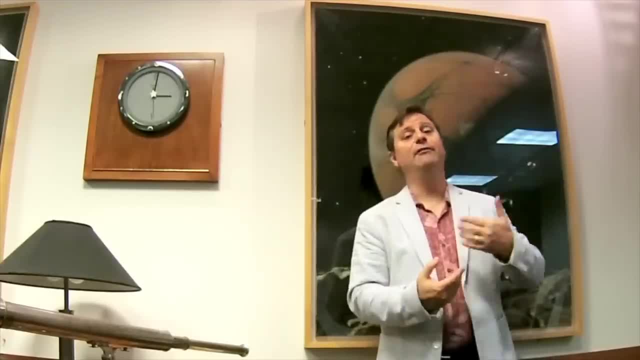 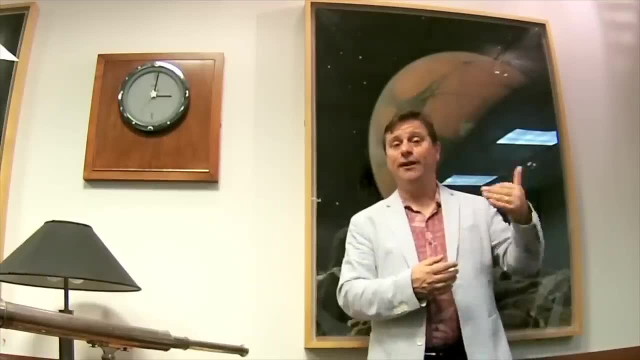 sky and all these pictures of constellations. Typically, if we were in a purely dark location and we have a massive power outage and there's no lights in the sky anywhere, you'll find that there's roughly about 6,000 stars in the entire sky that you can see without the aid of a telescope. 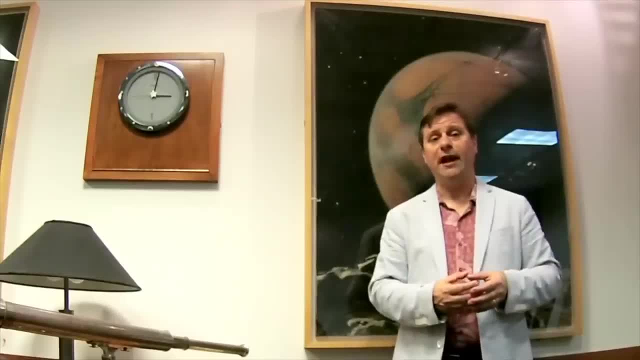 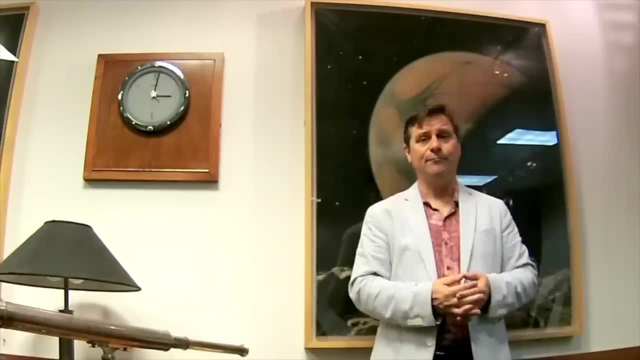 That's a lot of stars and if you go to someplace really dark you start to lose track very quickly of how many stars you count In an urban environment. you might be lucky to count a hundred stars In a very dense urban and light polluted. 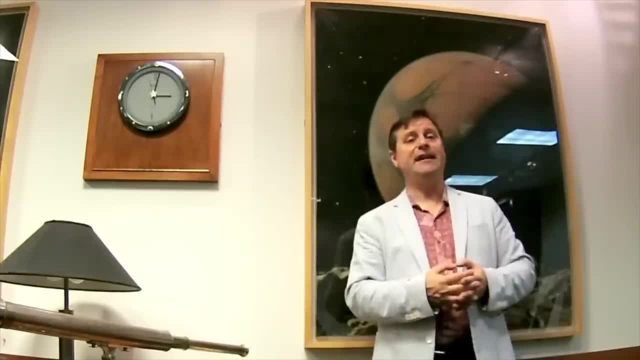 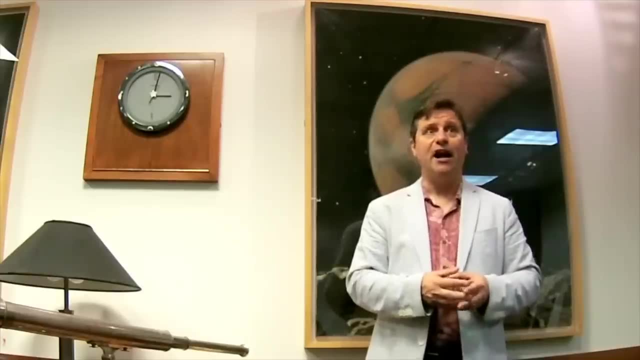 environment, you might get five or six. So light pollution has taken away our ability to see many of the stars and actually identify the constellations. Up until the 1950s and 60s, basically, the constellations were there for everyone. 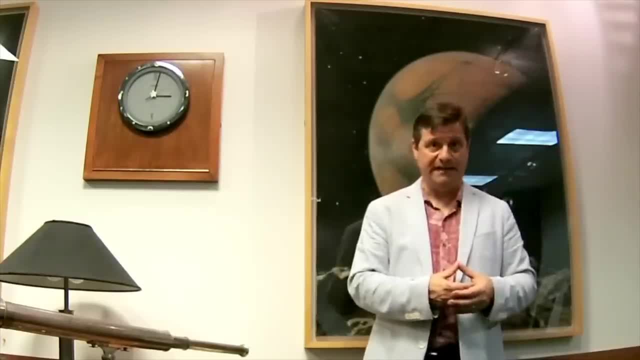 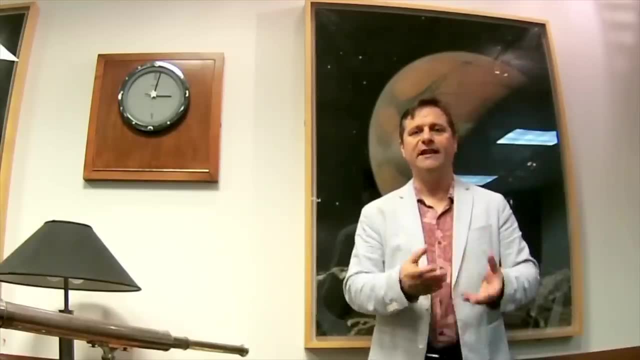 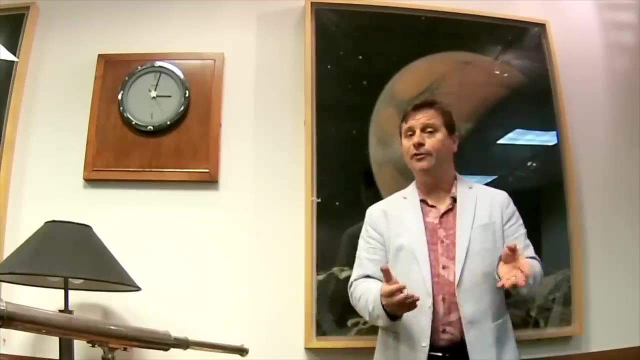 to see. but as modern society has become more illuminated in terms of street lighting and outdoor lighting that never gets turned off, we start to lose that light, because the light gets reflected to the ground, to the sky, and causes sky glow, And so sky glows prevent us from seeing constellations. However, if 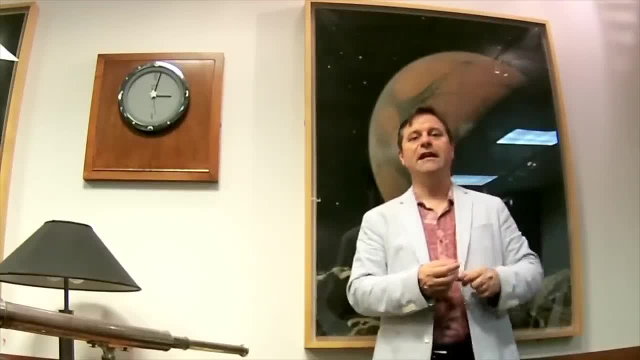 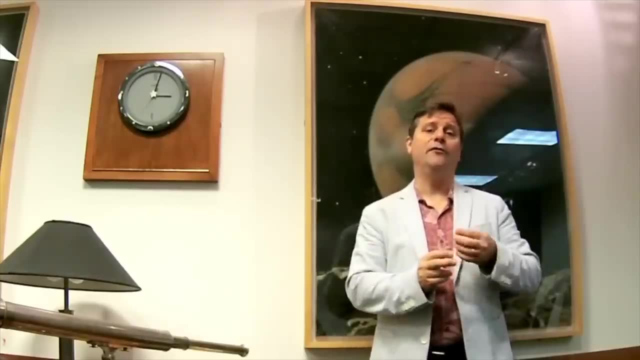 you're part of a class, get outside of town, go someplace dark and see the stars and try to see if you can pick out those constellations. So some prominent constellations are those that we call the zodiac. The zodiac are 12, or, if you. 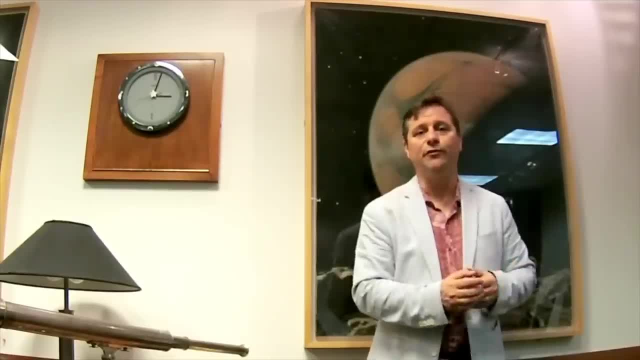 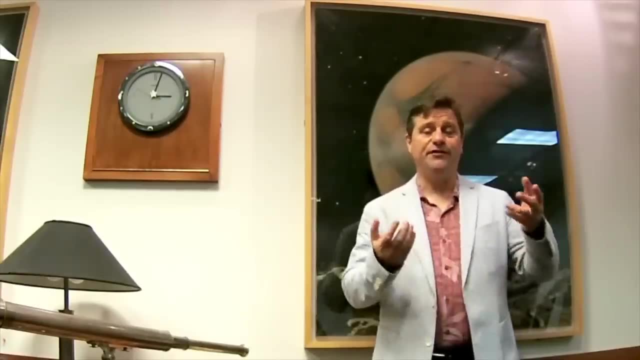 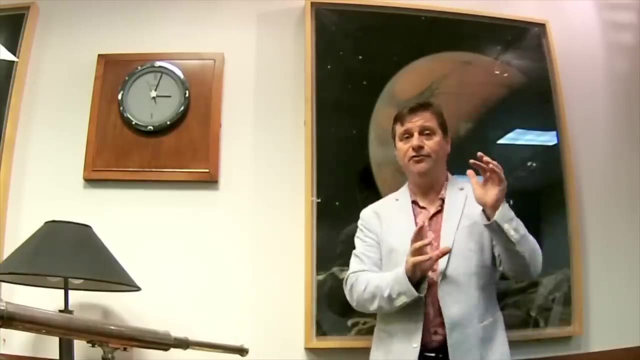 wish 13 constellations through which the Sun moves throughout a year. So we can try to find our way around the sky, and there's many ways to do so. One way that we can find our way around the sky is simply look for these constellations, these agreed-upon pictures in the sky. 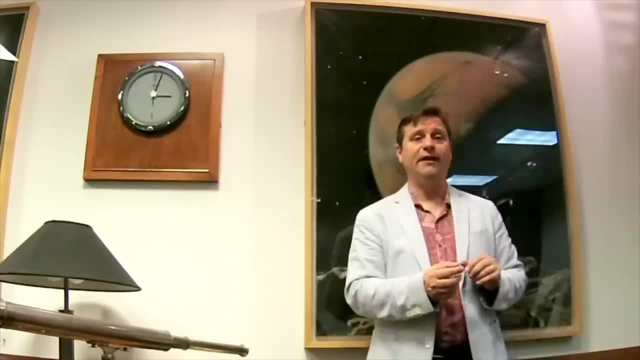 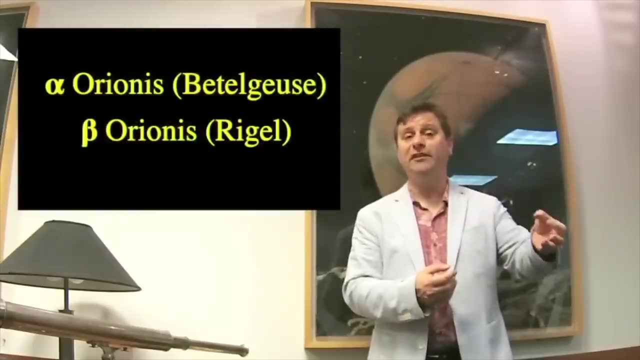 like, such as Orion, Orion, the brightest star in Orion. we would call that Alpha. The second brightest star is Beta, So the brightest star in Orion. its name is Betelgeuse and we have to add the Greek letter Alpha to give it, to say that it. 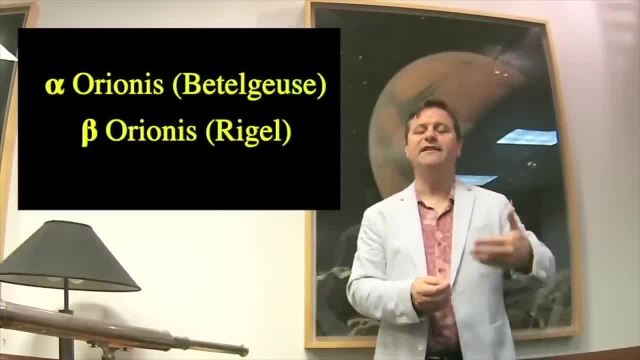 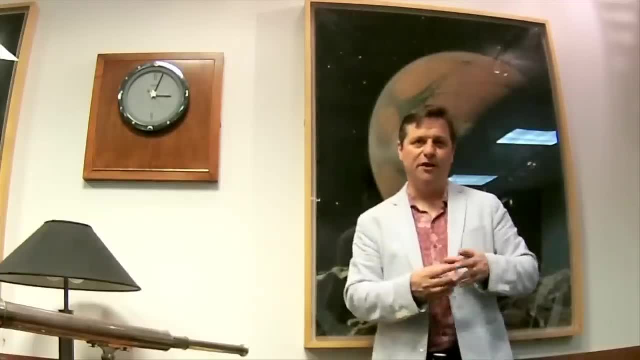 is the second brightest in the constellation, and Rigel is the second brightest in that constellation, and so we designate it with the Greek letter Beta. So that's pretty much what you see for many, many, many stars and constellations. There's a couple that are a little weird, but in general the 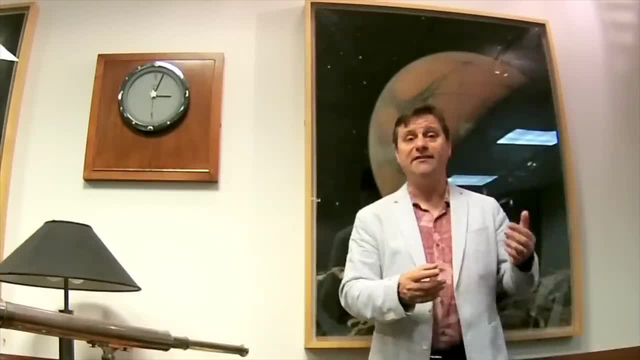 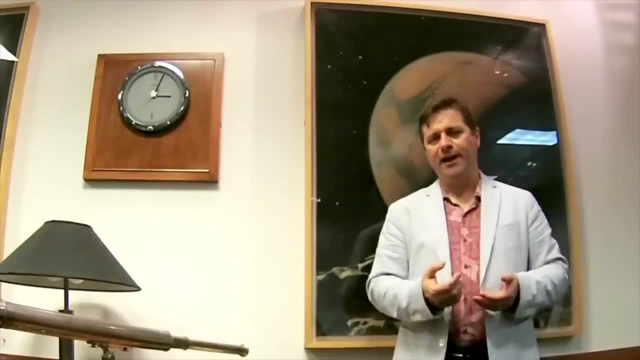 brightest star is Alpha, the second brightest is Beta, third brightest is Gamma, and so on, And then the brightness is go to numbers after you run out of Greek letters. So when we look up at this, that's one way of kind of navigating our 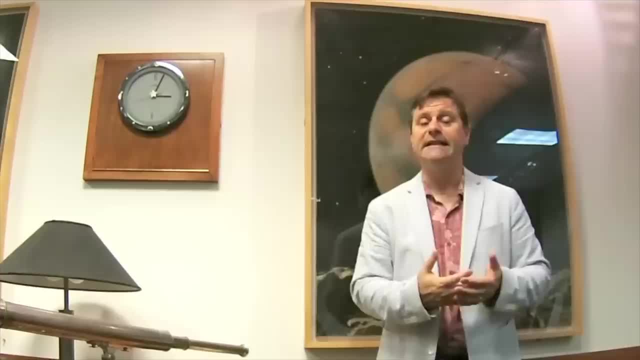 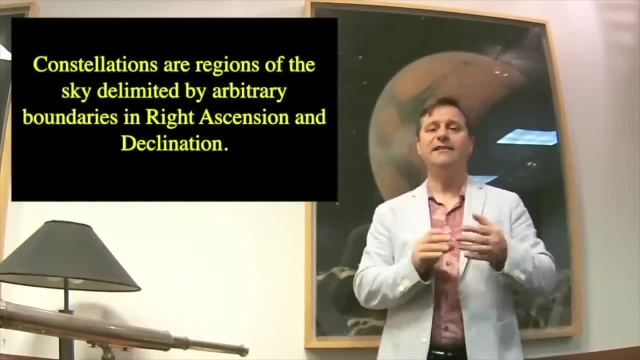 way around. but you have to know the constellations, and that's a big problem. everybody does and not everybody has a laser pointer and maybe they're too difficult to find. So we have a new definition for constellations: Constellations. 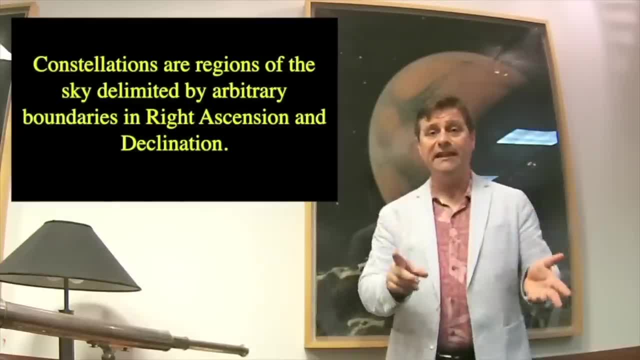 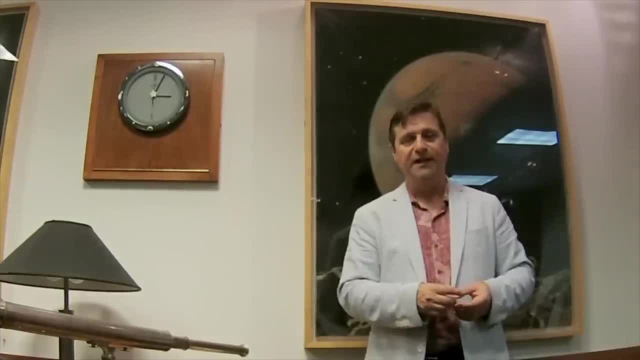 are a region of sky that's delineated by common agreement, And the common agreement is with the International Astronomical Union. So what are those things that are in the sky that we call constellations, and how do we get to agree where they are? 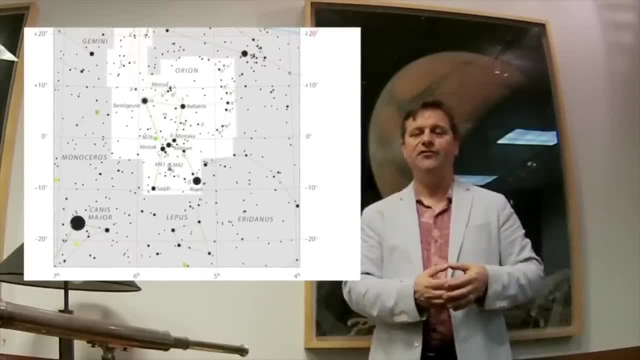 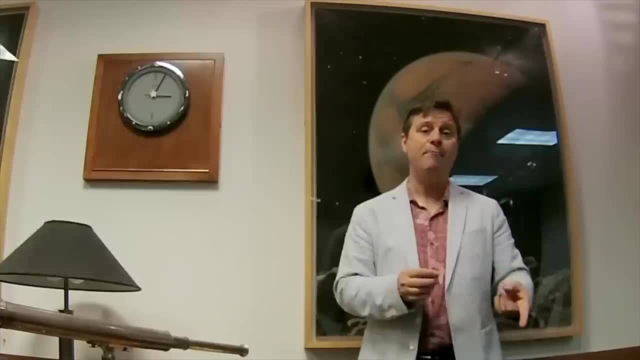 Well, we've actually created a coordinate system, Just like there's latitude and longitude on the Earth to help us find places, and latitude and longitude are frequently used by map makers and governments to actually delineate the boundaries of their locations on the surface of the Earth. 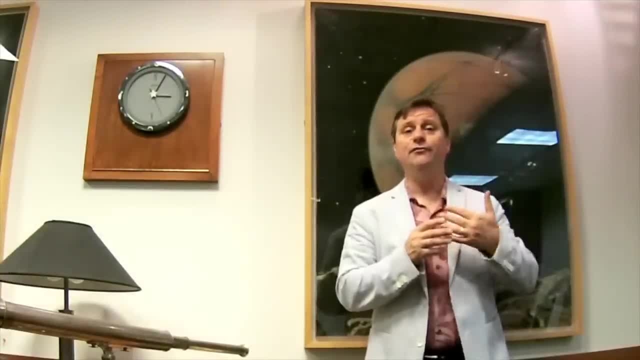 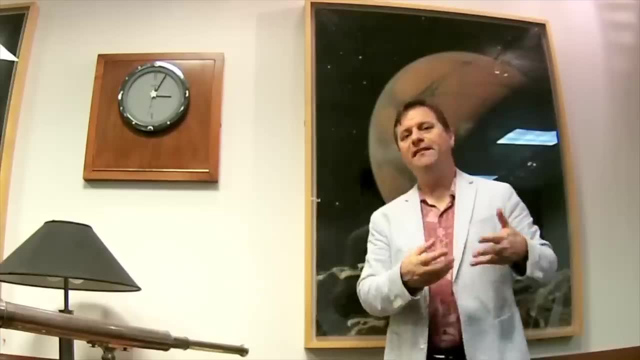 So if we take this natural thing, the latitude and longitude of the Earth, and we extend it out into space and we pretend that it is on the sky, we think then, therefore, that the sky looks like a big dome, It looks like if you're in some place, extremely. 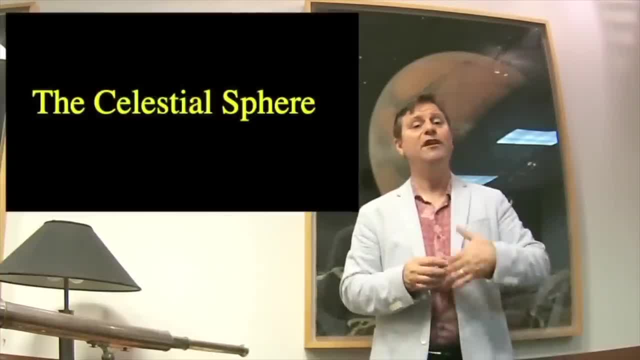 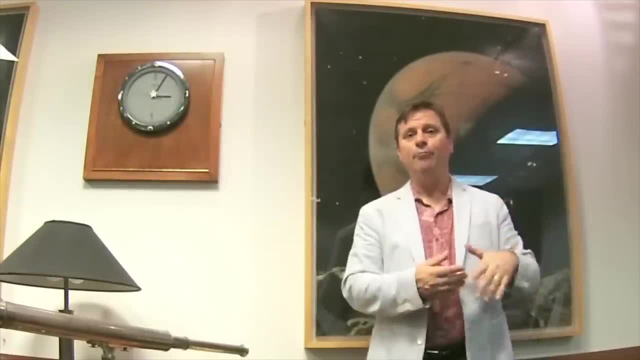 dark. it looks like an enormous dome is over you, And we call that dome the celestial sphere. It's an imaginary dome. There is no celestial sphere, but it looks like one to us. So since it looks like one to us, we can pretend that it has. 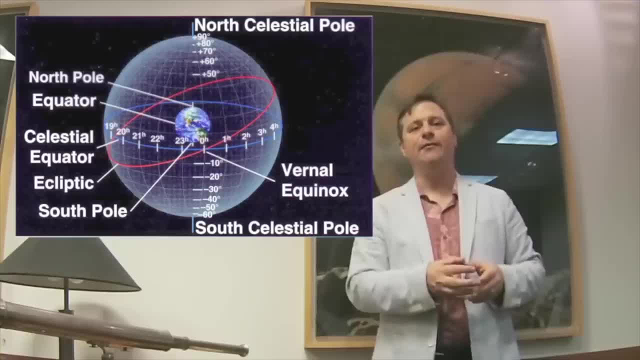 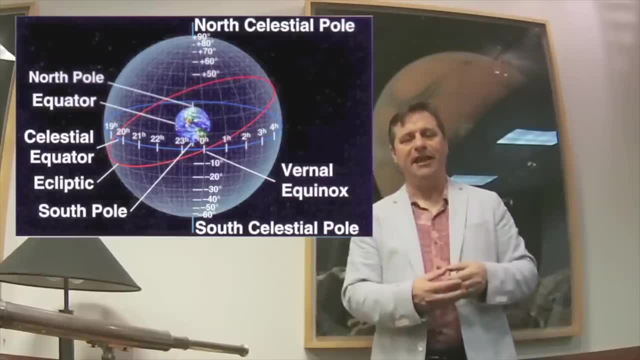 a coordinate system on top of it. So there are two basic elements to this coordinate system that I'm going to call the equatorial coordinate system. They're called right ascension and declination. So right ascension is the effect of the nature of sorry. 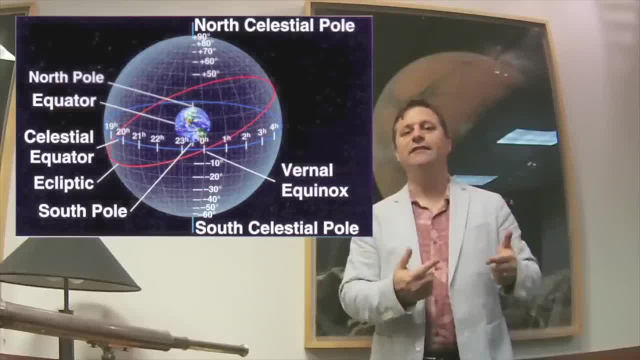 it's like latitude, I'm sorry, it's like longitude. So right, ascension is like longitude on the sky and declination is like latitude. So the Earth's equator set out into space. if you were on the Earth's equator and looked straight up. 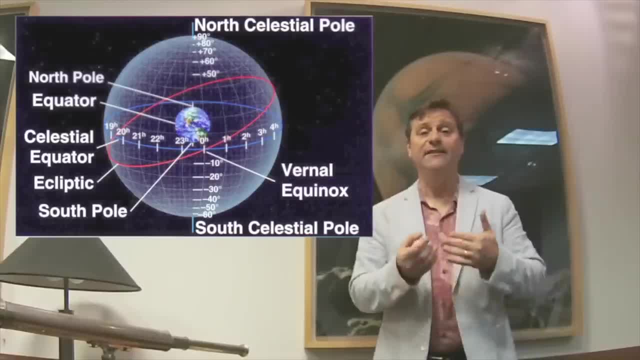 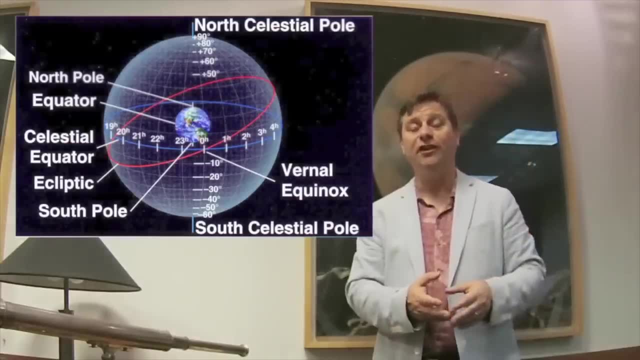 you would be looking at the celestial equator, And the celestial equator is declination zero And if you went 90 degrees up from the declination, you would be at the north celestial pole, And that's where you would be if you were at. 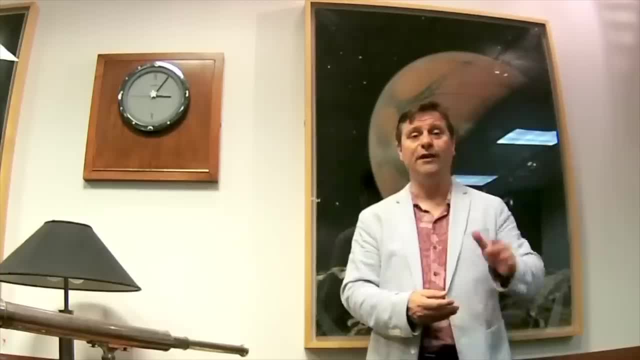 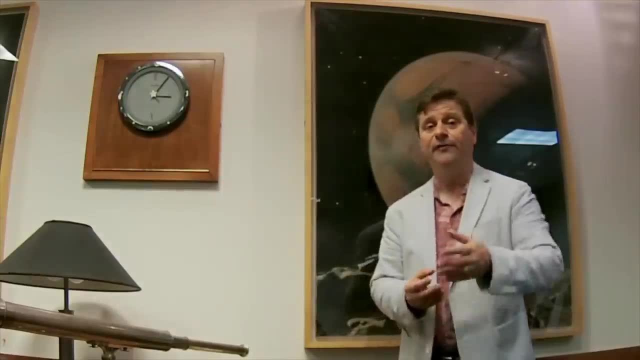 the north pole of the Earth and looked straight up, you would see the north celestial pole. And if you went south 90 degrees in declination from the celestial equator, you would be at the south celestial pole. So declination is just like latitude, but it's. 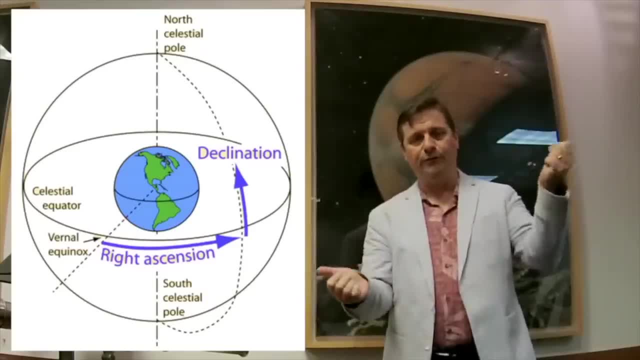 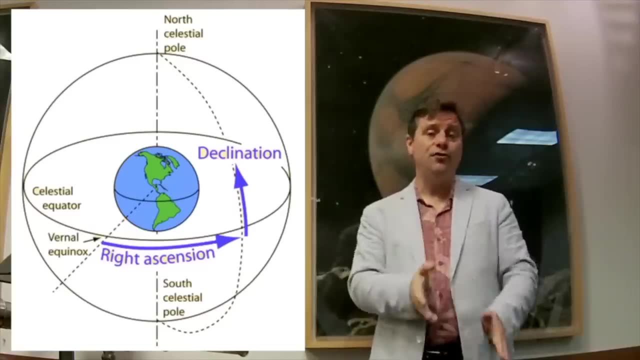 projected on the sky. So that's pretty easy to see. There's poles to it and there's an equator to it, just like that. So with latitude I mean with longitude, it's a little different. The longitudinal idea is called. 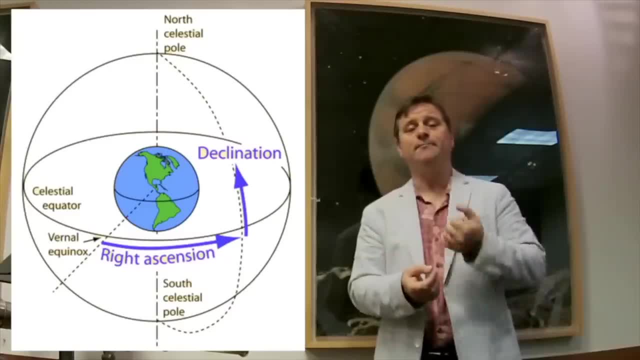 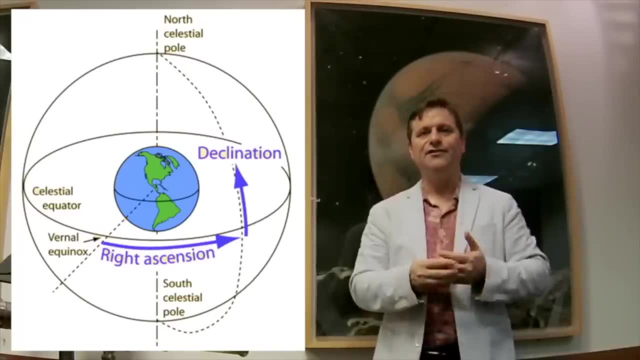 right ascension And unfortunately it's not measured in degrees. it's measured in hours, And hours are 15 degree units. So you 365 divided by 24 is 15, so you get these 15 degree increments, And the reason for that is that the Sun 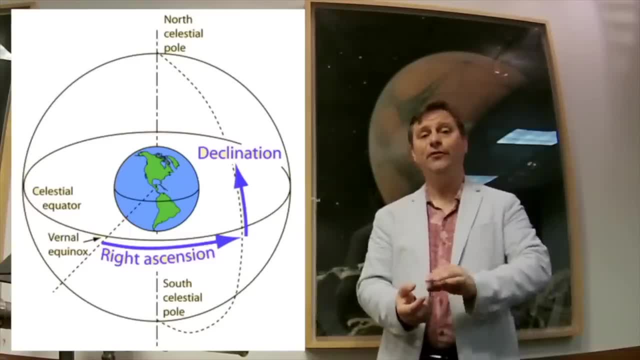 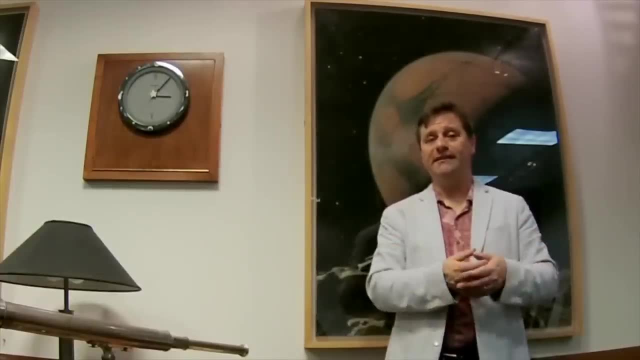 goes around the Earth every 24 hours, so it seems to actually move about one hour, And that's what it looks like it does. So what we have is that if you want to see when a star is going to rise, you look at its. 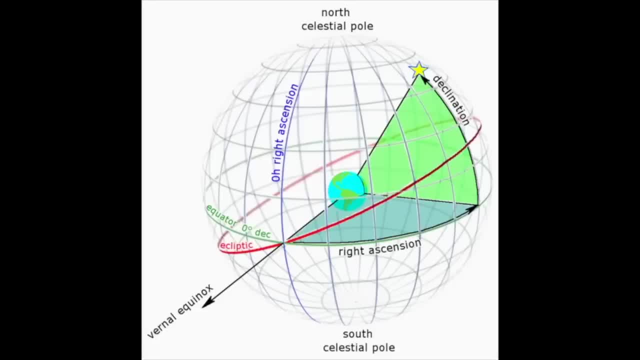 right ascension and that tells you the time with respect to the Sun. So if you know where the Sun's right ascension is, you know where the star's right ascension is. you can determine the time just by looking at their coordinates. 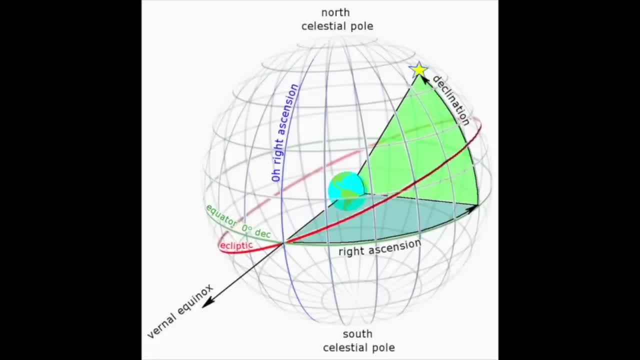 So right, ascension can have any zero point, just like longitude can have any zero point. there's no real zero point to it. So we choose a point on the celestial sphere where the zodiac intersects the celestial equator, And that point is called the vernal equinox. 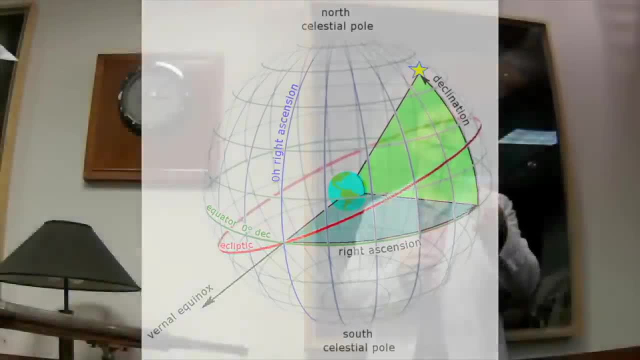 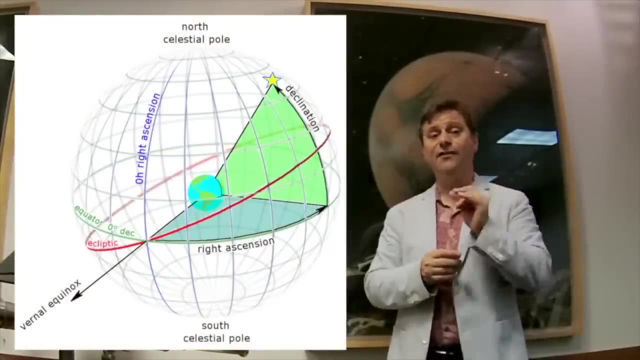 And that's the place in the sky where the Sun lives at roughly March 20th or 21st or 22nd. So on those days the Sun is on the celestial equator. it is rising above the celestial equator as it marches its way. 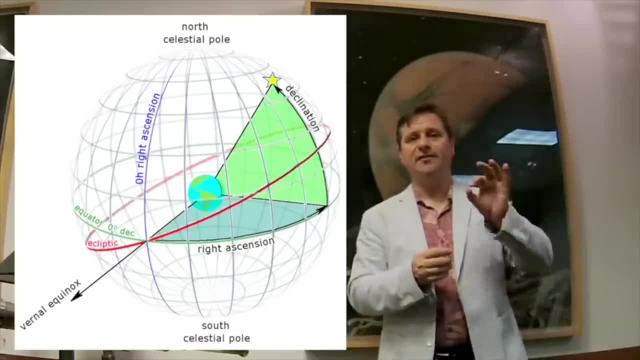 around the sky and we get the Sun as it's our designated point And it's called the vernal equinox, because that's when the Sun is right on the celestial equator and that's where we define the zero point for right ascension. 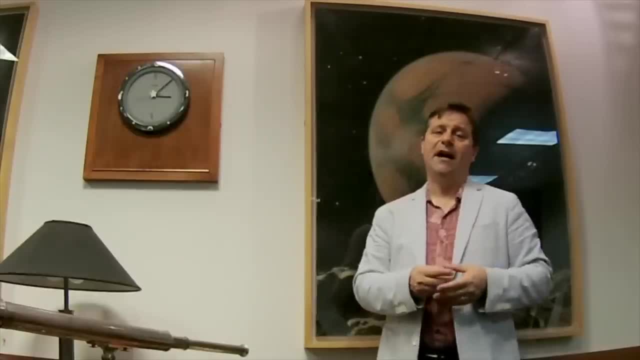 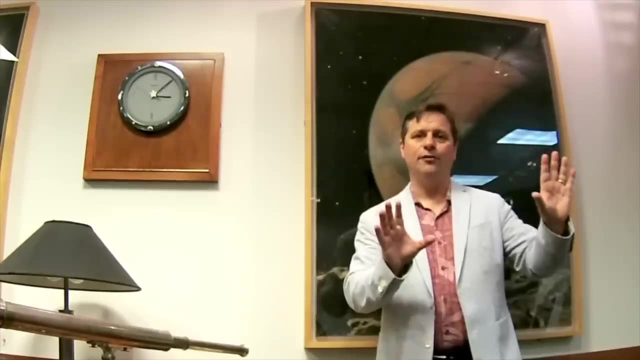 And it goes eastward from there. In any event, this is one coordinate system and that's tied to the stars, because if you look out into space, the celestial coordinate system stays fixed with respect to the stars, just like latitude and longitude stay fixed with. 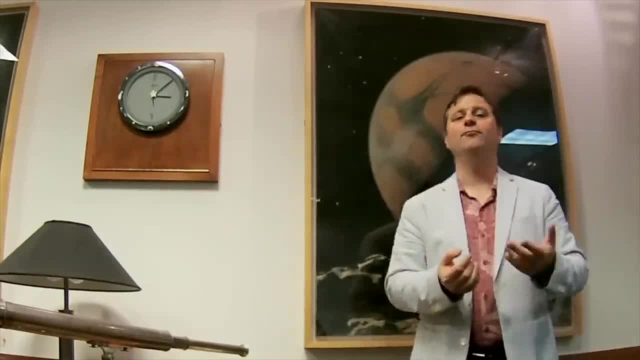 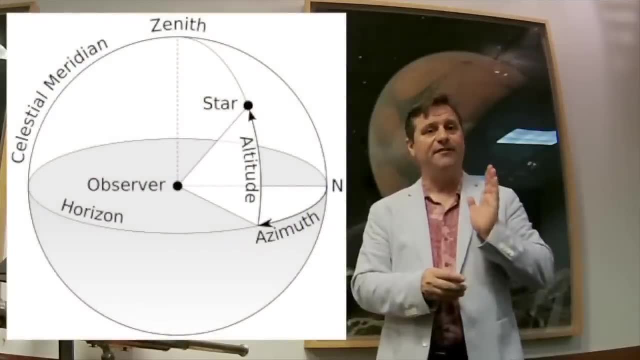 respect to the Earth. Now there is a different coordinate system that's much more helpful to us if we're just going stargazing in our backyard. It's called the altitude azimuth coordinate system. If you face due north, that has an azimuth angle of zero, and if you go to the east, 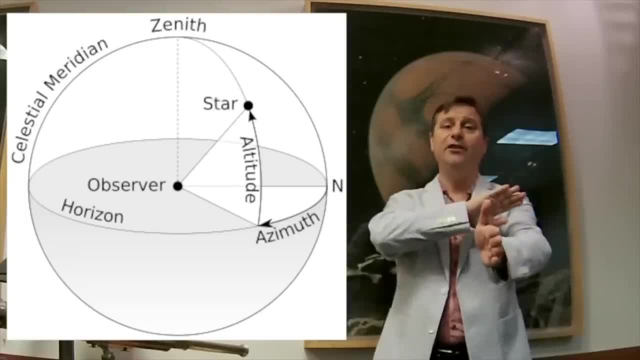 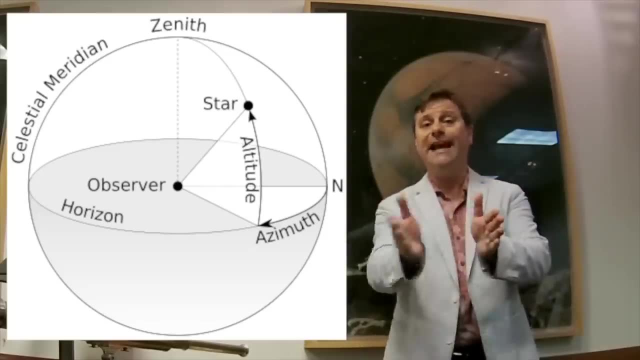 it'll be: 90 degrees is east, 180 degrees is south, 270 degrees is west and back to 360 degrees is north. So it's like, think of that. you're measuring an angle around the horizon, So then you have another. 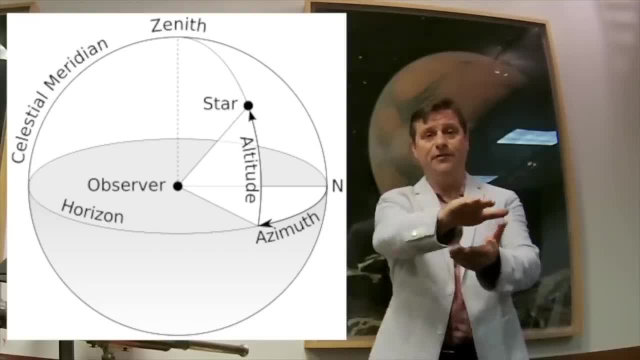 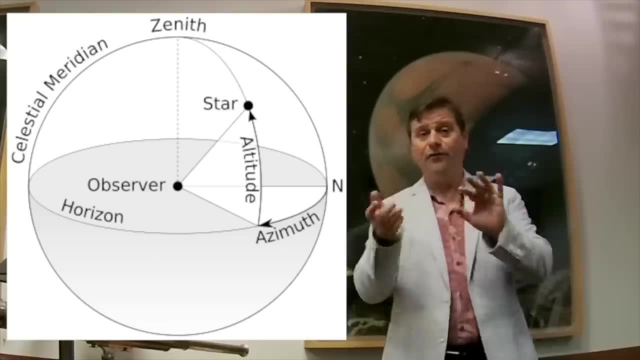 angle, which is elevation or altitude. So altitude is: if it's on the horizon, it's at zero and 90 degrees up it's at the zenith or at the top of the sky. Now, stars move through this coordinate system. 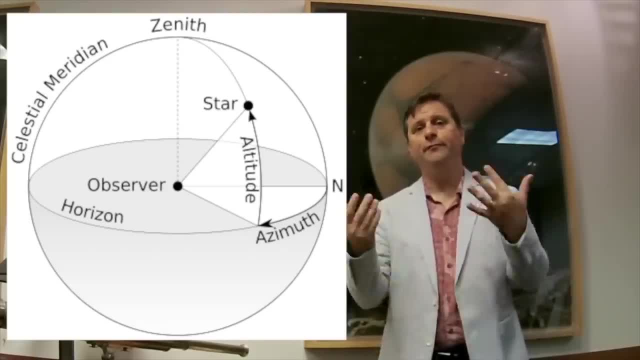 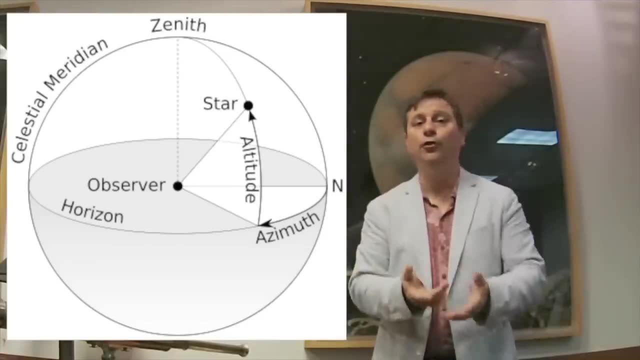 So the altitude and azimuth coordinate system is with respect to the observer, not with respect to the stars. So they're two different coordinate systems and the altitude and azimuth is good. if you want to say, hey, this is about 30 degrees up from the horizon due east, It's like okay, but that doesn't. 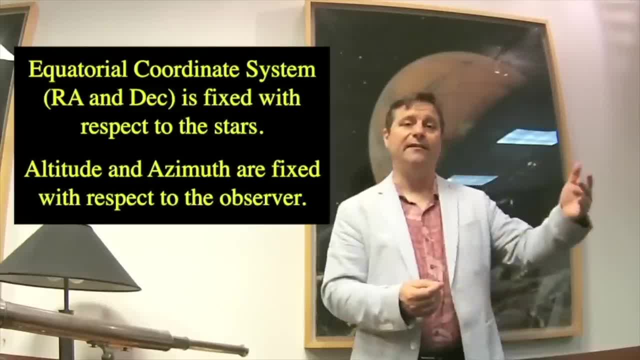 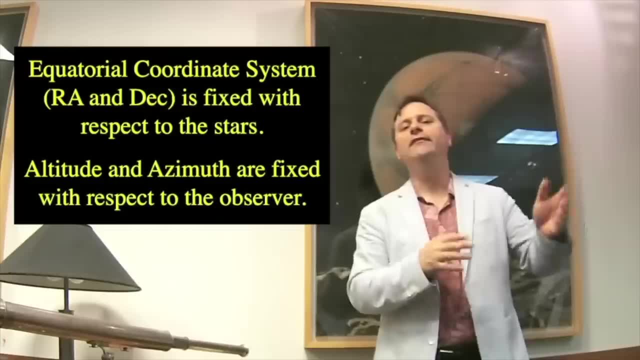 help you if you're trying to tell somebody where something is and you live in New York and they live in Montana. So if you're on the phone with somebody in Montana trying to tell them where this really cool comet is in the sky, you can't use. 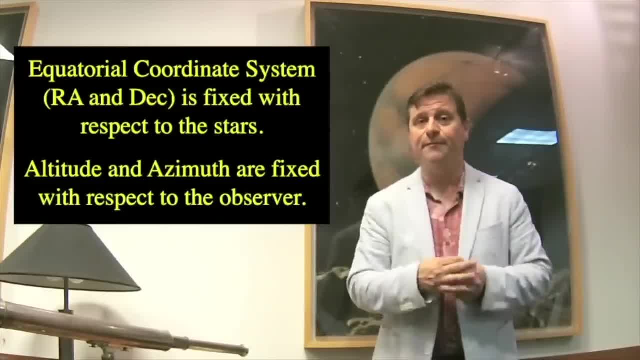 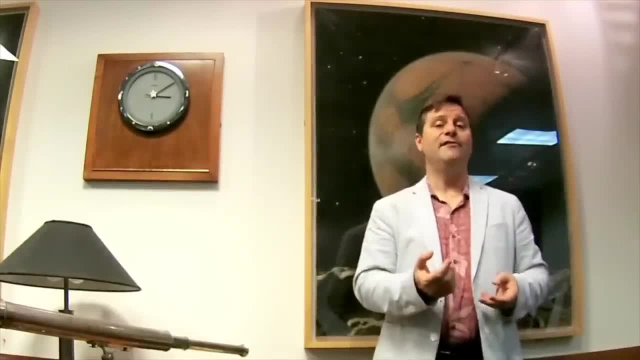 altitude and azimuth. You must use the equatorial coordinate system and show them where it is in right ascension and declination. So there's some basic things. Astronomy is the study of the things in the sky. We're going to be studying planets, stars, galaxies and the universe and our 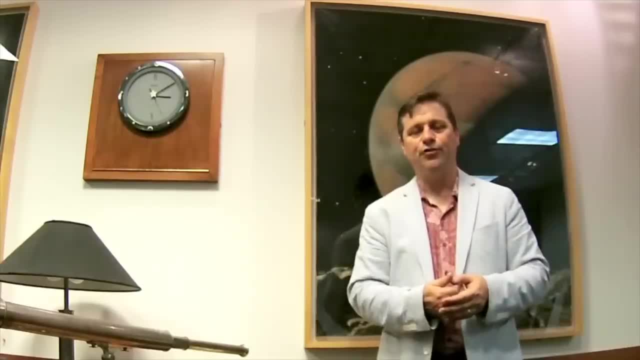 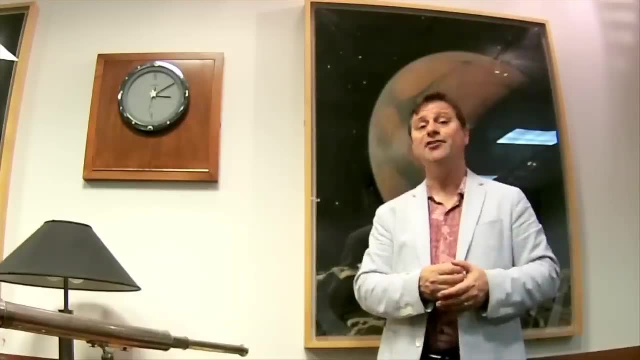 first step is looking at the sky. We see constellations which are groups of stars in the sky. They're given proper names, such as Betelgeuse and Bellatrix, and Rigel and Polaris, which is the north star, and all. 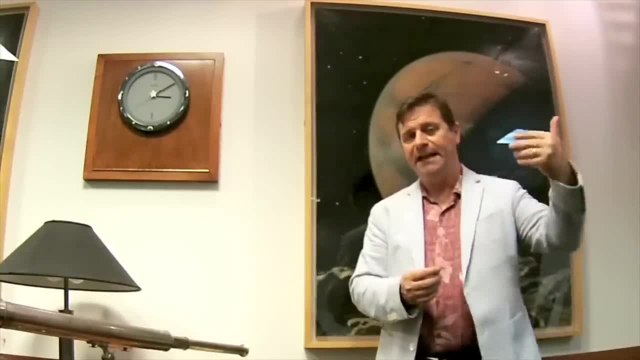 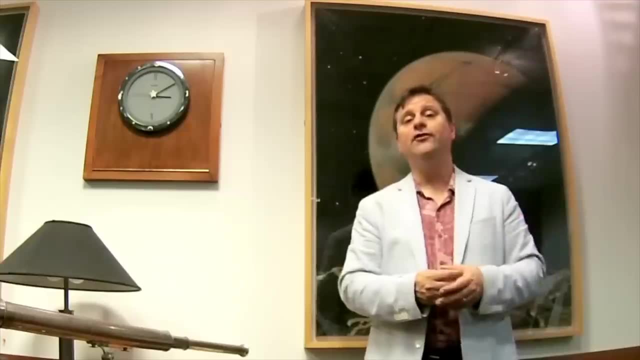 sorts of other names, And they have proper names as well as designated names, like the Alpha Orionis or Beta Orionis or Alpha Ursa Major or Beta Ursa Major, where the Greek letters determine their brightness, and always the first letter in the Greek alphabet is the brightest one. Also, we then 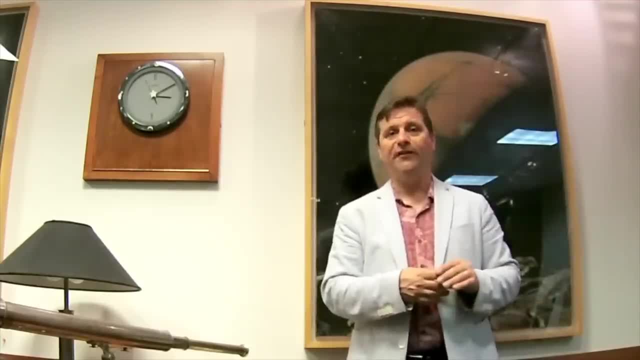 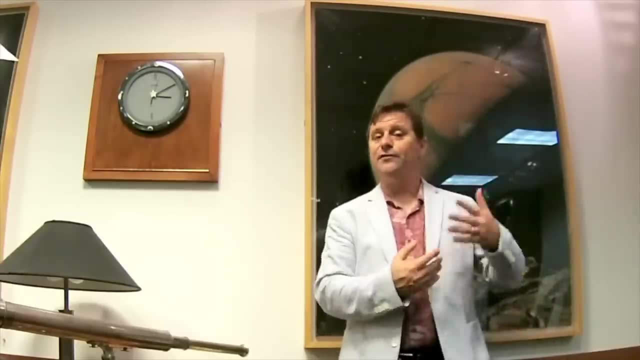 have coordinate systems to help us find things, And this is important because you look up in the sky and you always want to tell somebody: hey look, I saw this really cool thing up in the sky, This is where it is. And so you tell them using coordinates. 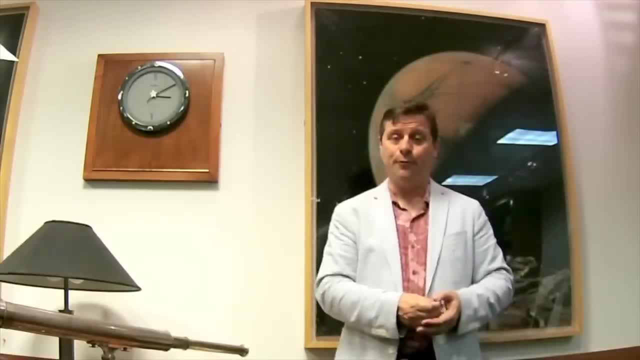 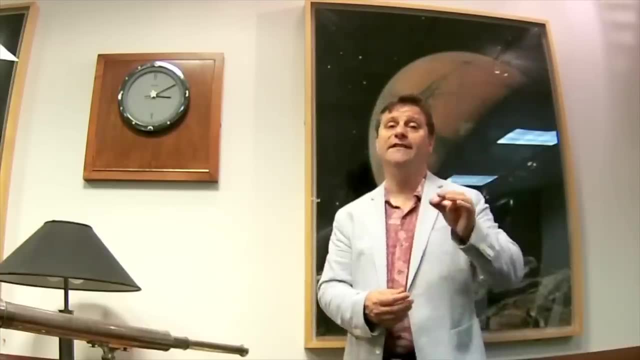 If they're standing right next to you, you can use the altitude and azimuth coordinate system. If they're on the phone or the internet with somebody far, far, far away and the thing hasn't even risen yet. but you want to see it after you've had. 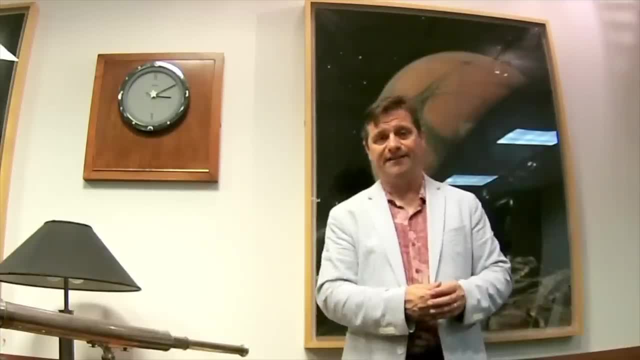 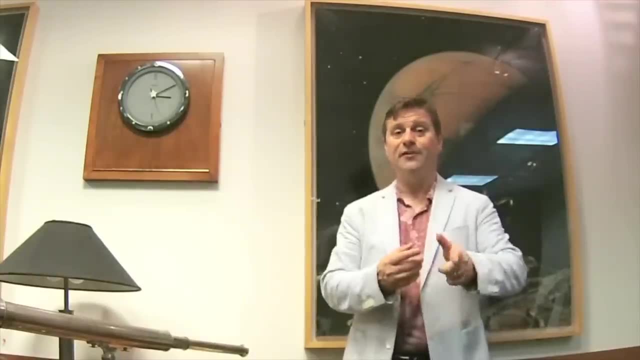 sunset or you've had sunrise and it's time for them to have sunset, then you would explain it to them using the right ascension and declination coordinate system, called equatorial. So that is our beginning and we're going to do. 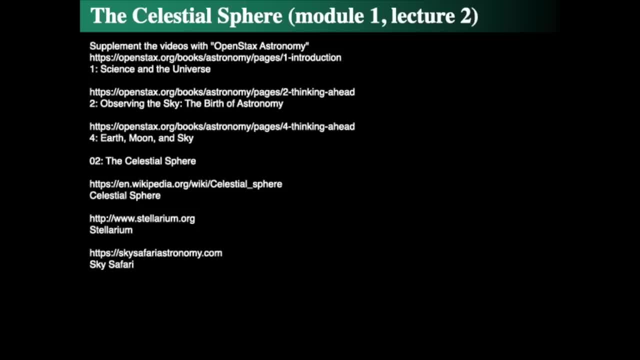 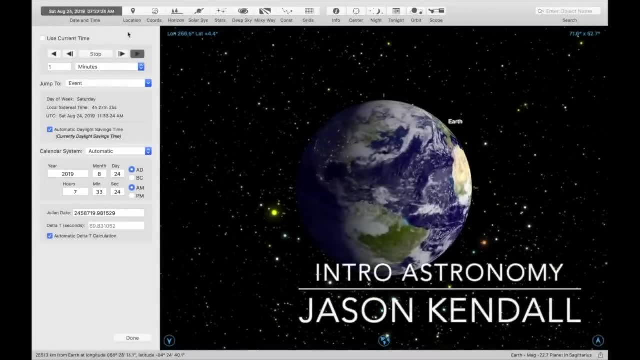 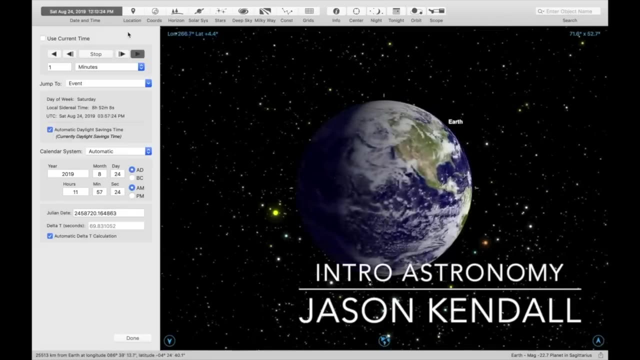 more soon. See you soon. Hello, this is Jason Kendall, and welcome to the next of my introductory astronomy lectures. I'm going to go back and redo some of my older lectures that I did a long time ago in order to bring in some good stellarium. 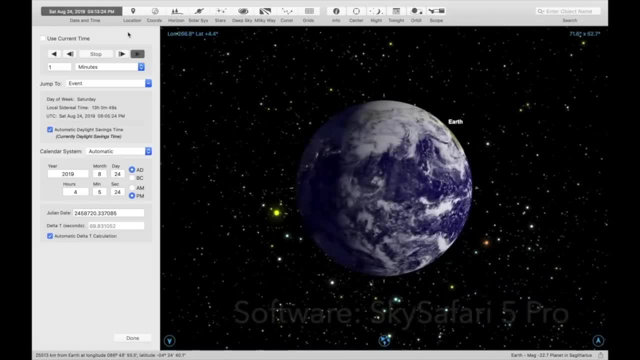 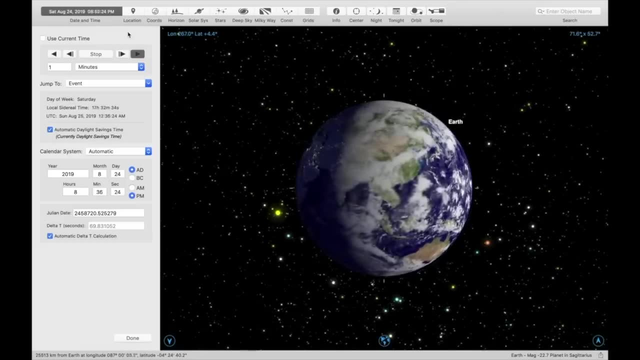 simulations to kind of help us understand things. And the first thing I'm going to look at here is the celestial sphere. So let's understand what the celestial sphere is and how we can visualize it. Well, first and foremost, we have to remember: 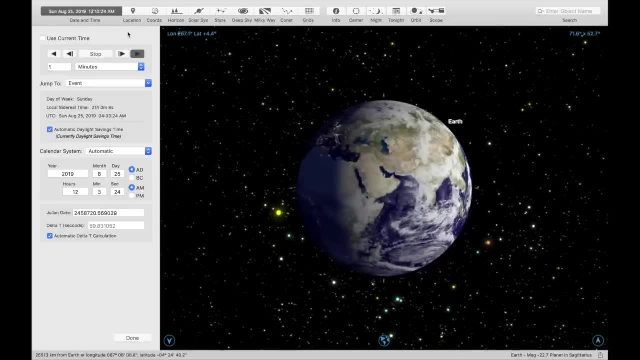 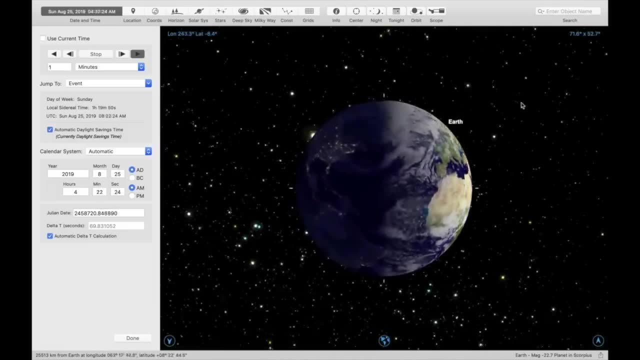 that we live on the Earth and the Earth is spherical. It is a ball. It is a huge ball orbiting in space and it's orbiting the Sun at some distance of 93 million miles away And if we turn around we can see there. it's over there. 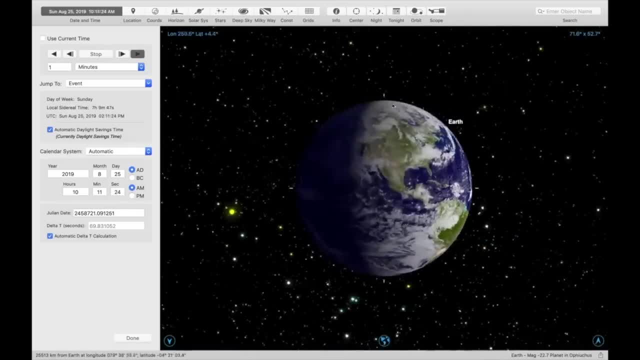 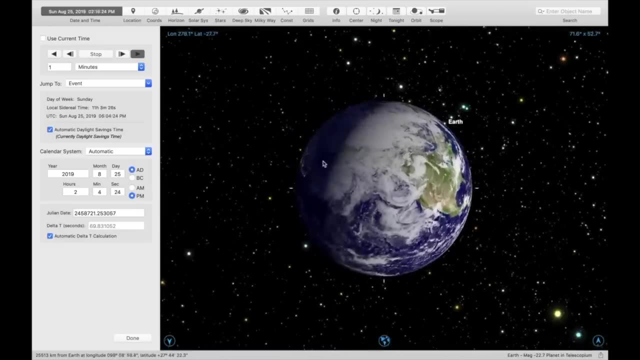 And we see that on one side of the Earth it's illuminated by the Sun and the other side is in shadow because it's facing away from the Sun. And the Earth is not flat, It is a ball, It is spherical, So as it rotates, 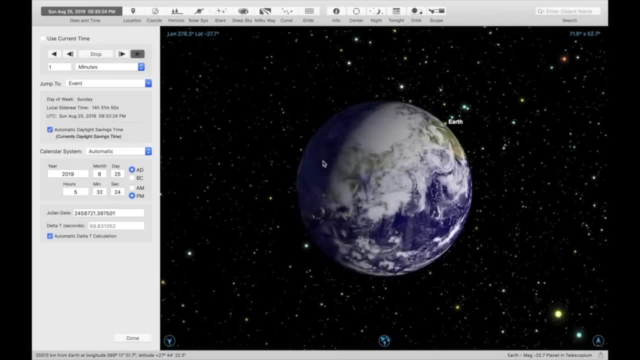 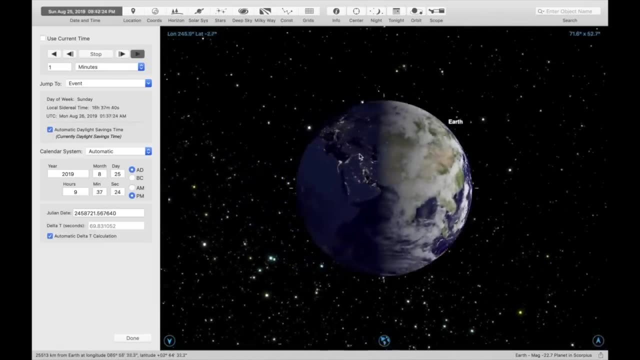 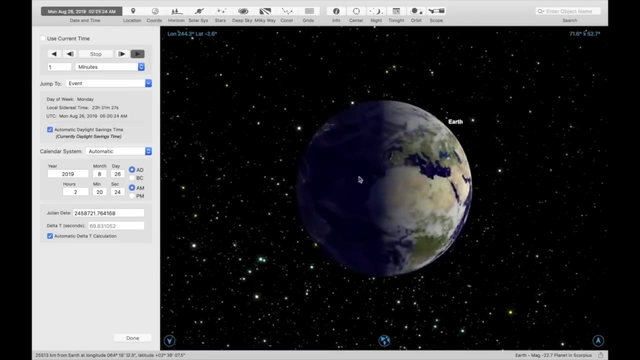 whatever's in the sky is different for different people. So if we look at the, if we just look at, say, on this side, we see for the demarcation between night and day as it goes through sunrise. Now the simulation, of course, is kind of having some trouble here, but whatever. 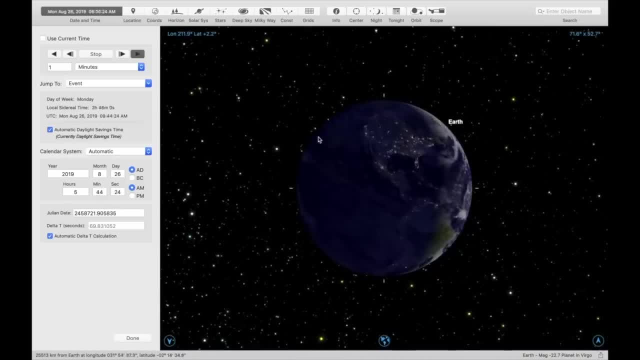 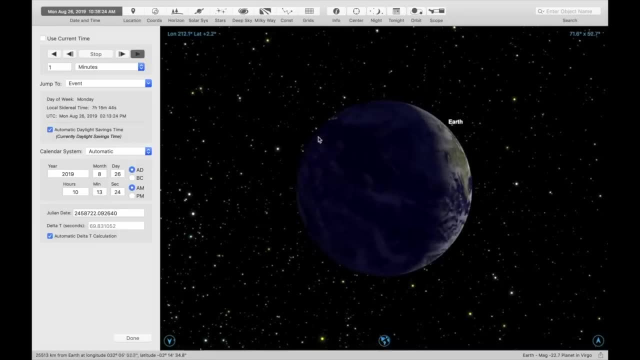 We can see that. if we look at nighttime side, we see that as the Earth rotates, the position of the continents, and therefore anybody on them, changes with time, And so therefore things that are in the sky change with time. So it's not like 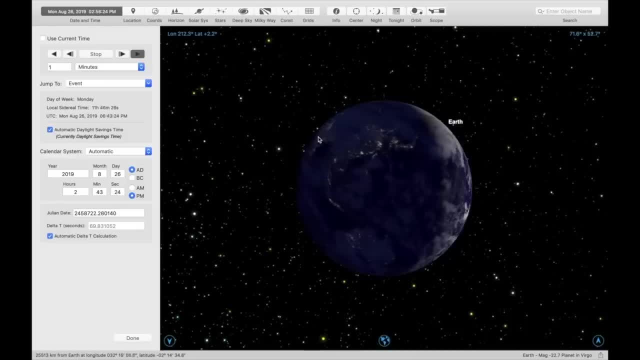 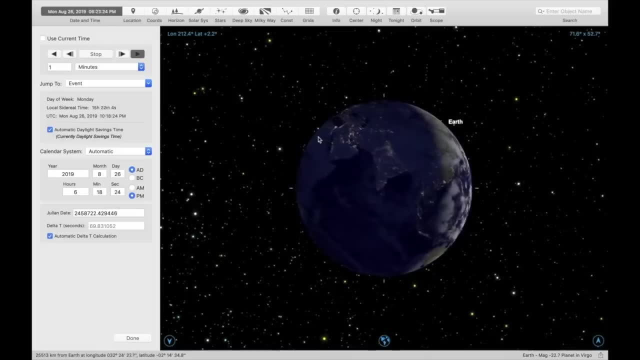 that the sky doesn't change. In fact, in some ways it does. In a lot of ways it does, But from our perspective, we see the Earth and we perceive the Earth as not moving. However, it is rotating on its axis And as it rotates on its axis, 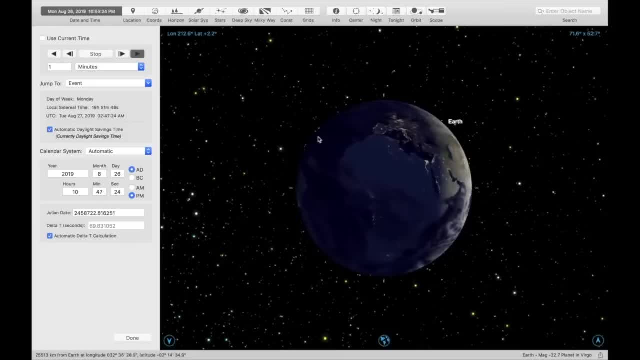 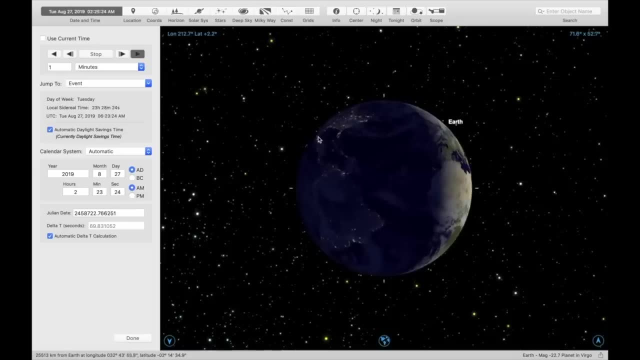 what we see in the sky appears to change. It's exactly the same thing as if we were driving in a car and we feel like the car is not moving because it might be going straight down a long road at like 90 miles an hour. 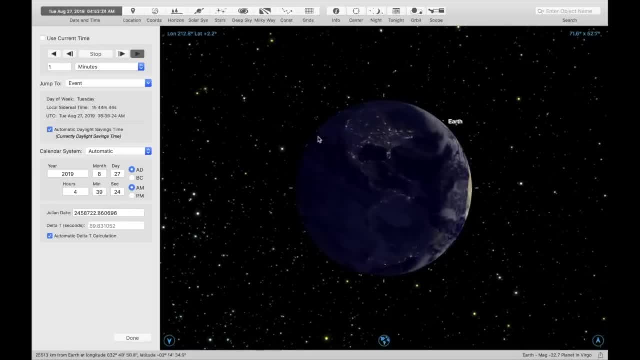 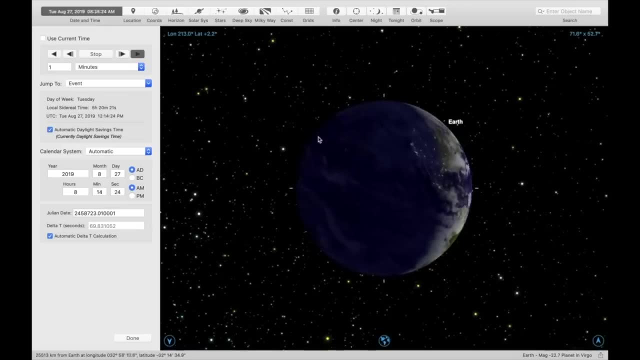 if you're going really fast, you're going west and all of a sudden you're looking outside and you see everything zipping by you. So you know that you're moving only because you got in a car and someone's driving that car. But if you 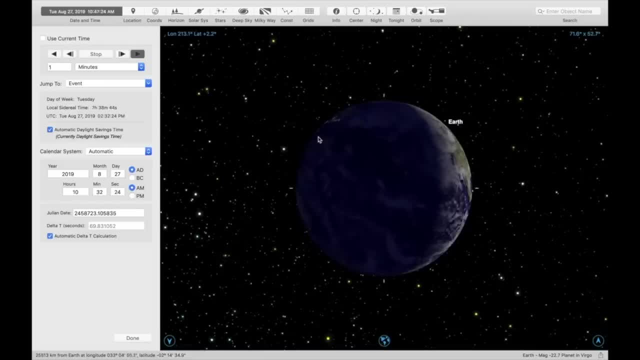 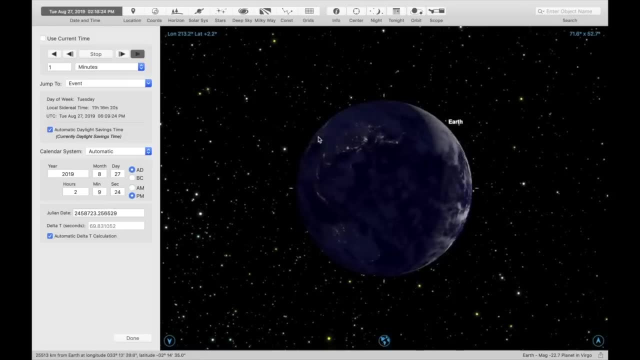 didn't notice that, or maybe you were on a train. the train appears to be still with respect to you, And if it's a really, really smooth track, then the outside world appears to be rushing by and you seem to be standing. 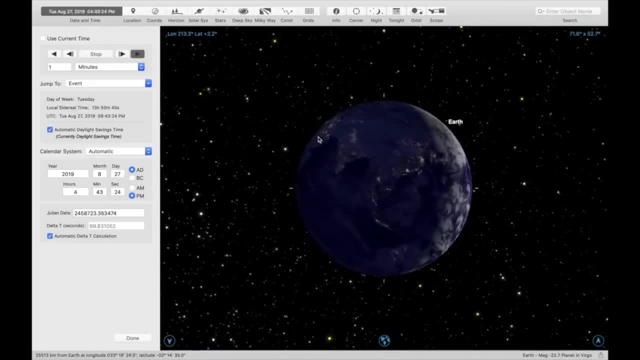 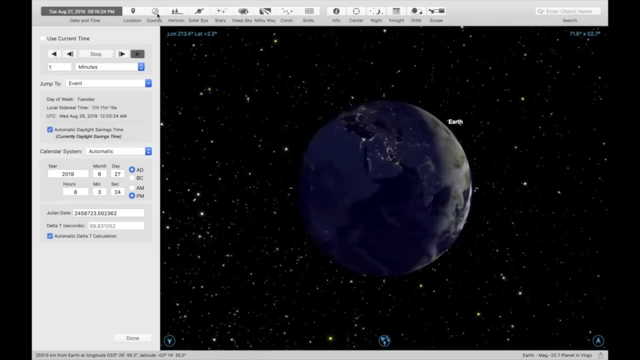 still, And that's the effect that we're having on the Earth. The Earth rotates on its axis, so therefore we see the sky move. So from this simulation we don't see the sky move, But let's actually go and check out what we. 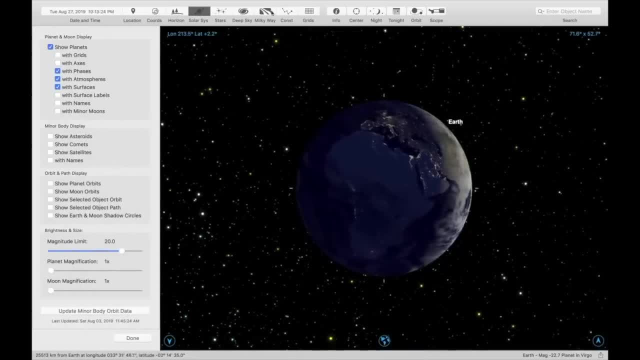 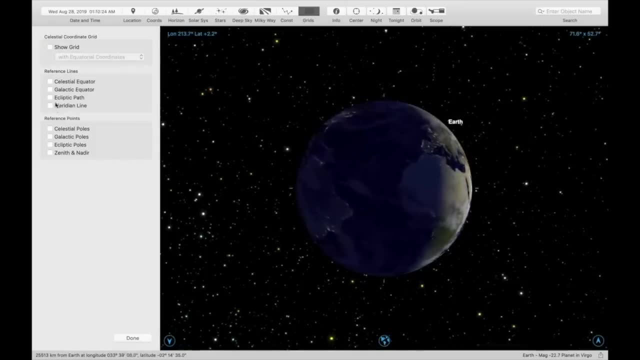 can learn about looking at the nature of our planet. This is our solar system, and I'm going to go look at the various grids and I'm going to turn on the celestial equator grid. Well, not just yet. I'm going to look at the solar system. 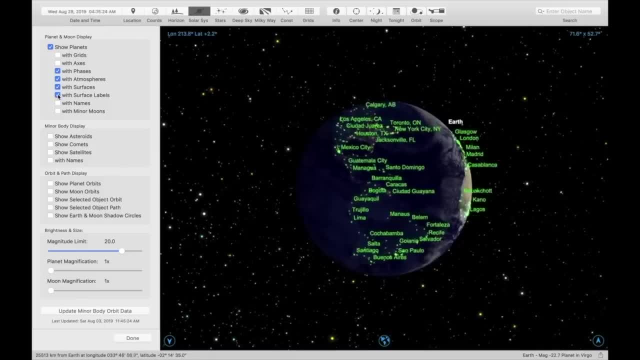 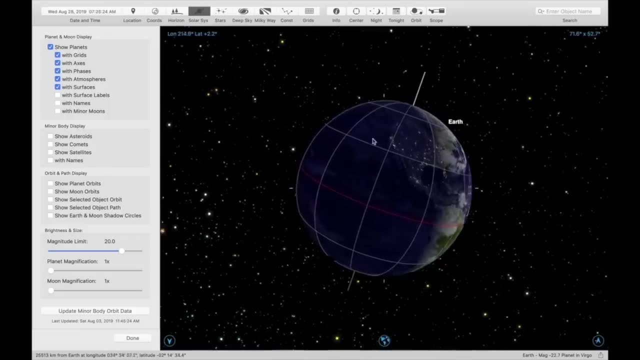 coordinates and I'm going to show the surface labels and the grids and the axes. So the axis of the Earth's rotation is this stick that appears to be sticking out of the North Pole and a stick that appears to be sticking out of the South Pole. 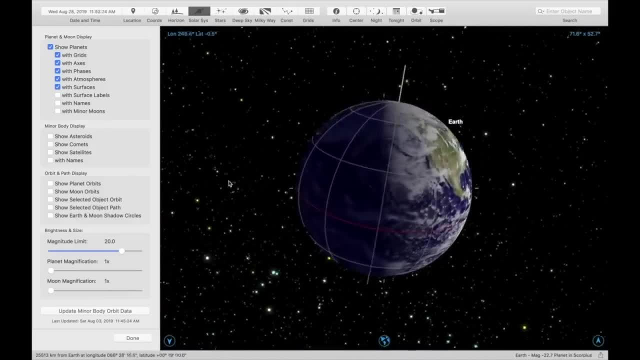 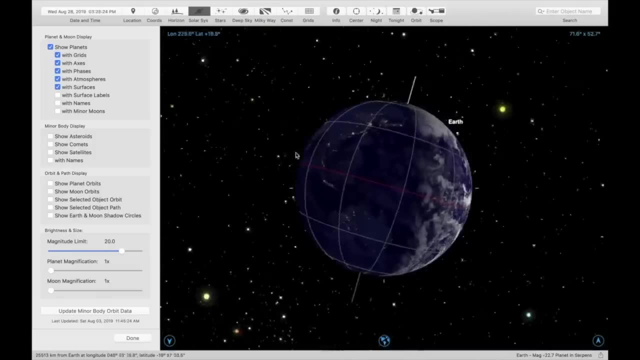 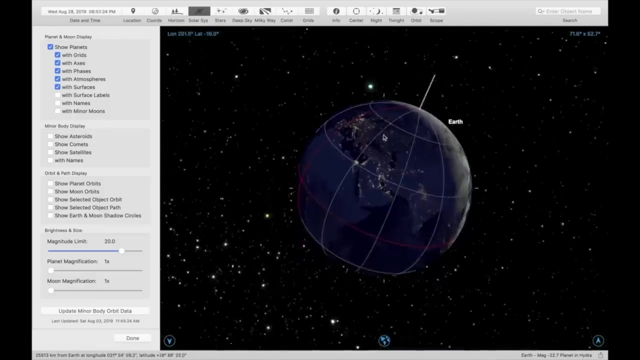 That is a line that goes through the center of the Earth, an imaginary line upon which the Earth appears to spin, And so that's called the Earth's rotational axis. There's also another slight little axis that is in tiny glowing marks, and that is well, I guess, if we twitched it just right. 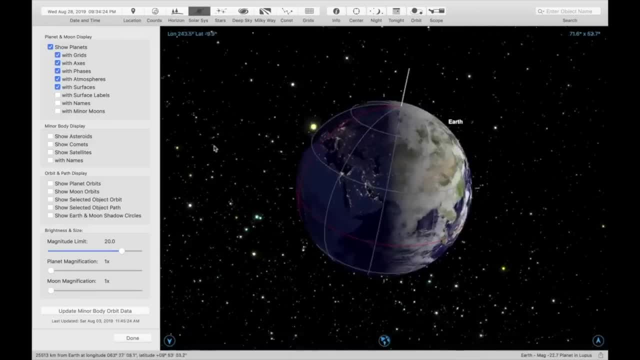 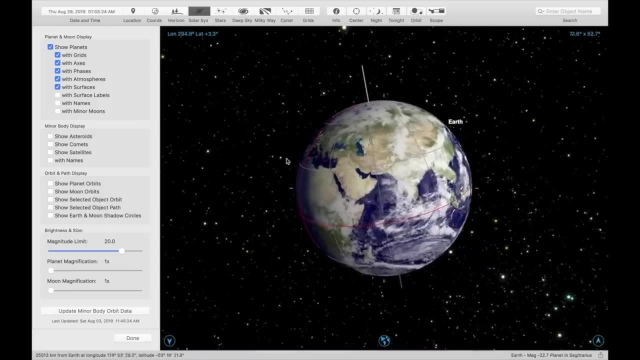 we'd be able to see that 23.5 degree tilt. But really the Earth's axis is pointed, it has its own rotational axis, and there it is, And we have a series of grid lines, and those grid lines are latitude and longitude, The red line going across the 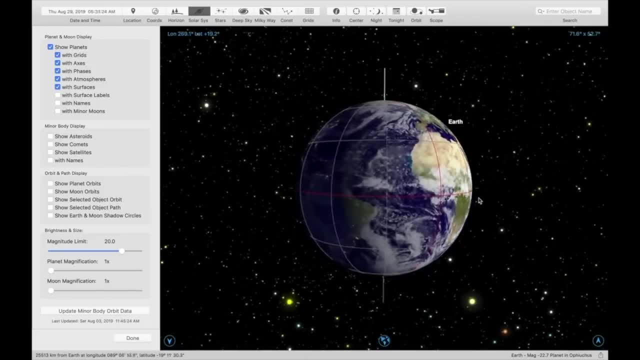 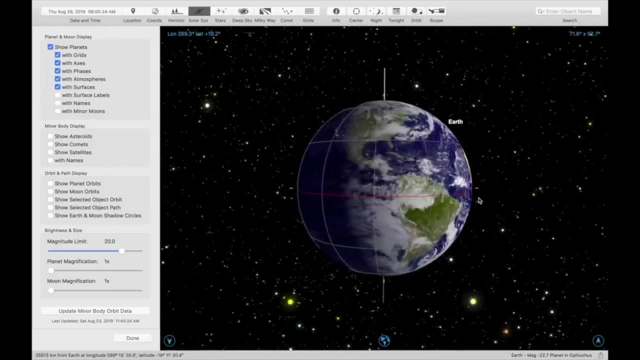 middle of the Earth, right across the middle, through Africa and across South America, like that. that is the equator, And the Earth's equator is at what we would call zero degrees latitude, And if we go up to the North Pole it would be. 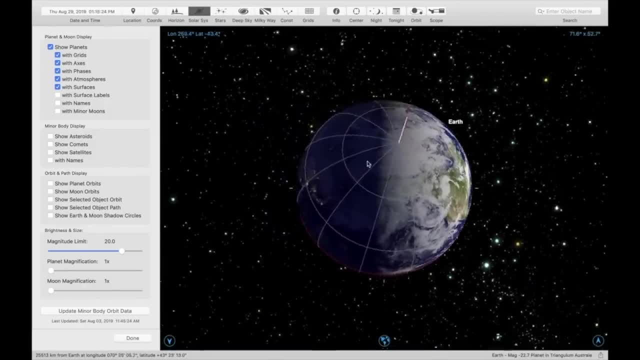 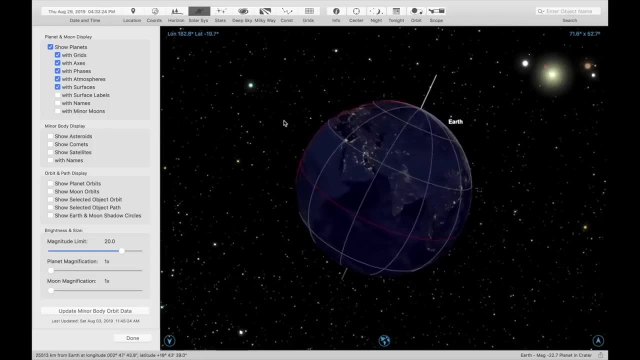 90 degrees north latitude. Now, if we go around, we also see there's a special set of longitude lines which go from the North Pole to the South Pole, and those longitude lines show the position on the Earth's surface, That red line that runs through Greenwich, Connecticut. 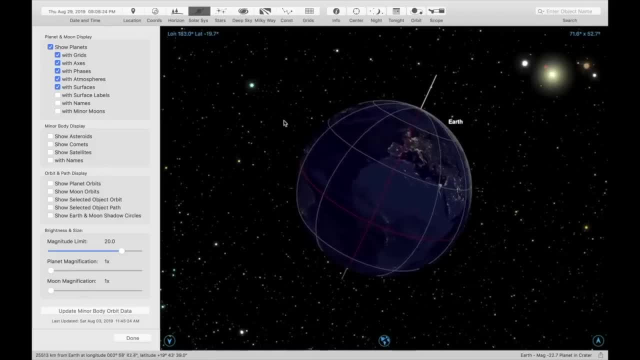 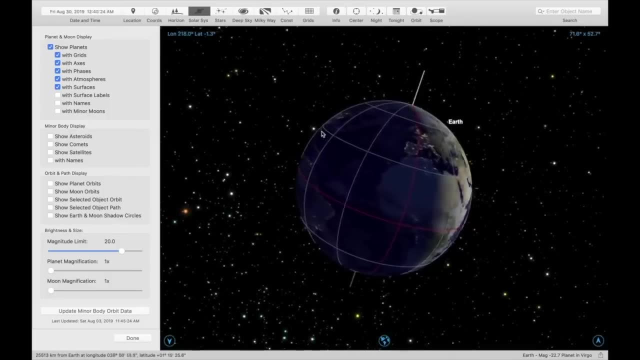 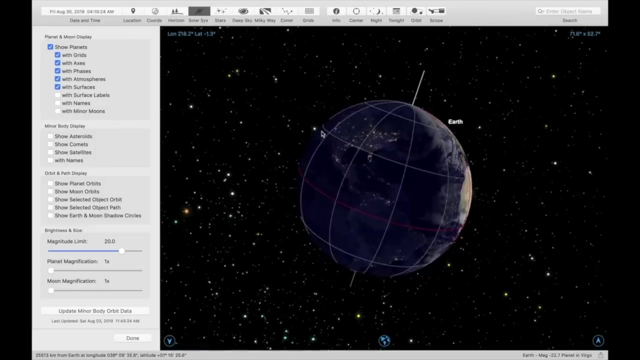 demarks the beginning of the coordinate system for latitude and longitude, for longitude specifically, And everything to the east is larger in longitude and everything to the west of that is less than longitude. So our natural thinking is that: imagine that we took the grid of latitude and longitude. 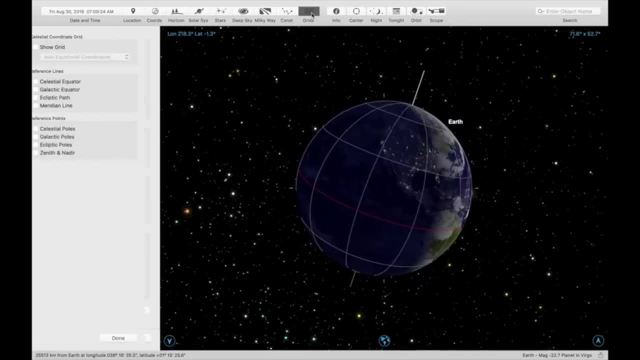 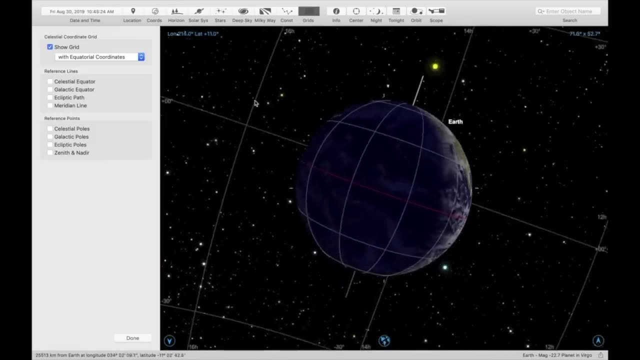 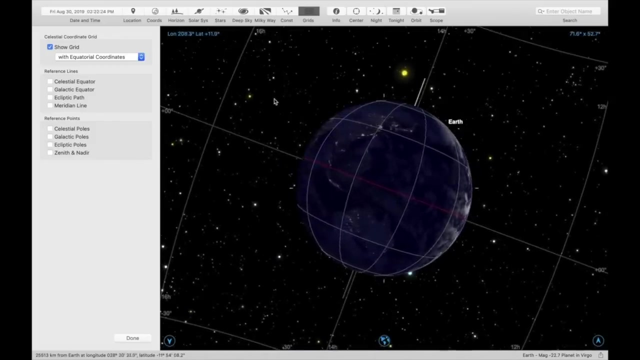 and extended it out into space. If we did that, we would be using what are called equatorial coordinate systems. So the equatorial coordinate system is an analogy of the Earth's latitude and longitude out into space And if I line them up just right, you can see that the Earth's equator 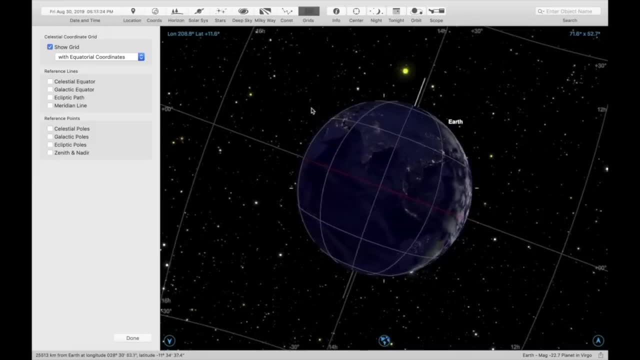 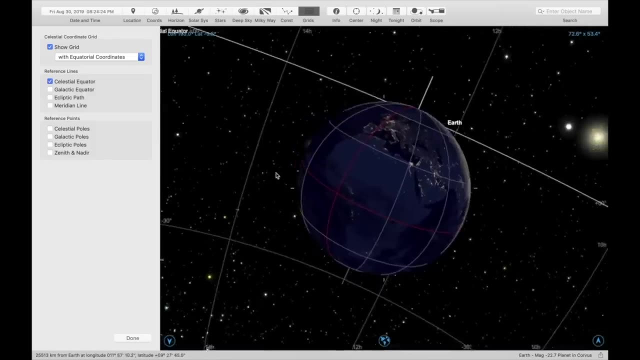 which is the red line, directly corresponds to the celestial equator, which is now bright. So I'm going to brighten and dim it. and brighten and dim it. And the celestial equator is the bright line that goes across the middle of the field. I'm going to zoom out just a little bit, The middle. 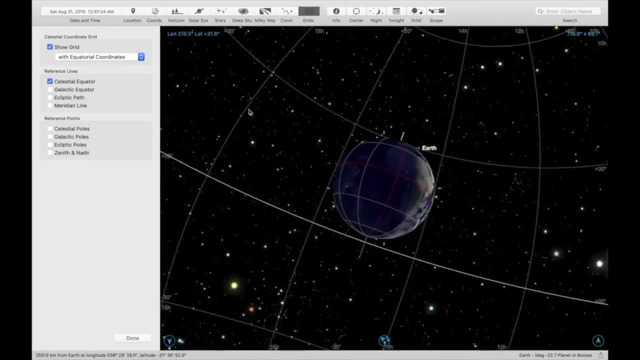 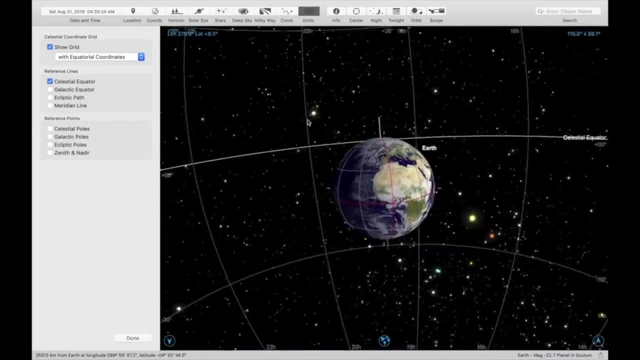 of everything in the sky. This is a grid that's on top of the sky, So we can think of the. I'll show you why we're even doing this in just a second. But the celestial equator is the imaginary extension of the. 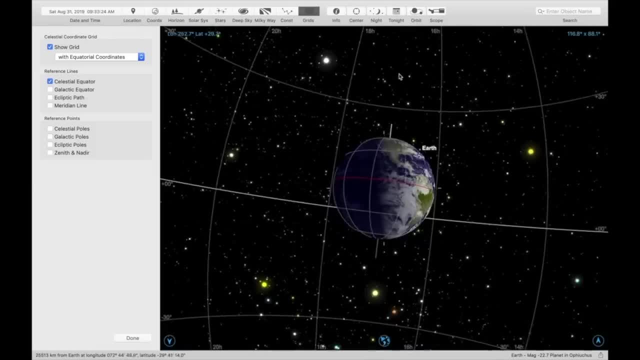 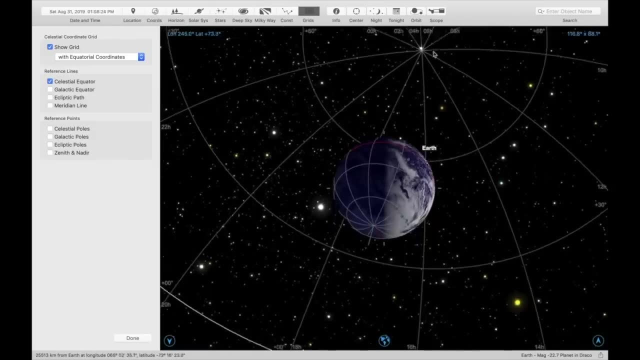 Earth's equator out into space. Now, if we look straight up from the North Celestial Pole, from the North Pole, where that line seems to be pointing, and that line points at what we call the North Celestial Pole, So that is, the NCP, or North, 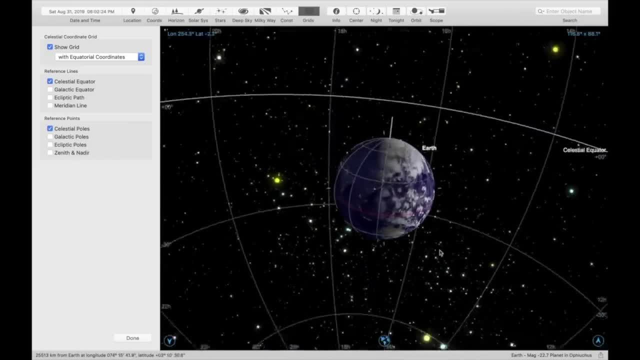 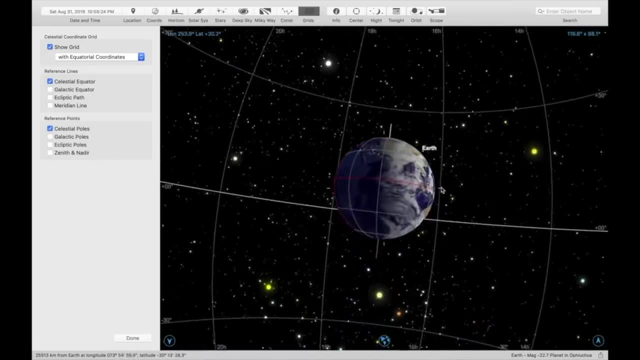 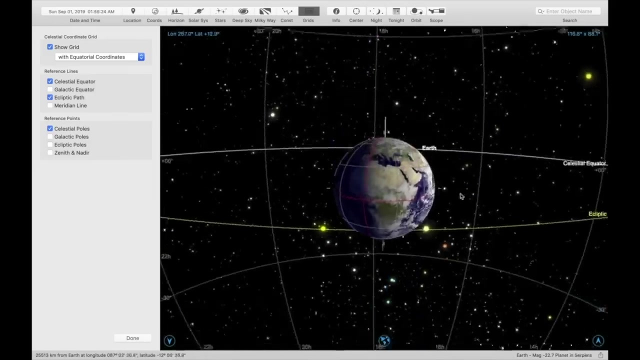 Celestial Pole, And there's also a South Celestial Pole where the southern Earth's axis points towards, which is the South Celestial Pole. Now, there's also a path upon which the Sun rides, and that path is called the ecliptic. So the Sun and all, and 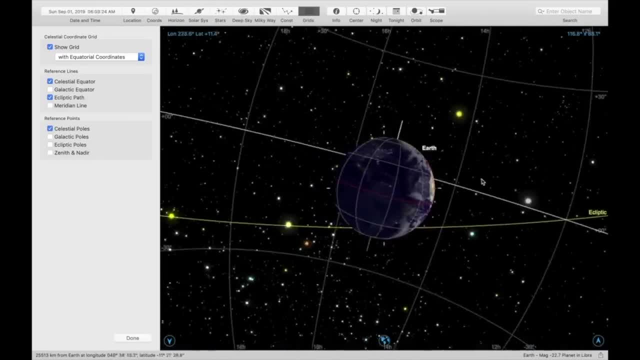 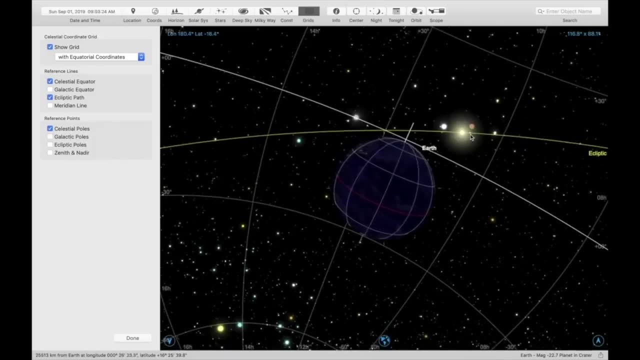 roughly all the planets appear to ride on the ecliptic, which is a path in the sky. So if we were to watch the Sun over the course of a year and see where it is in the sky, we would see that it's roughly well, it's always on the ecliptic. but the planets themselves 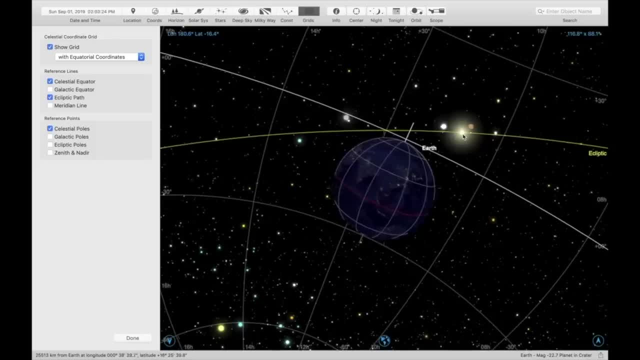 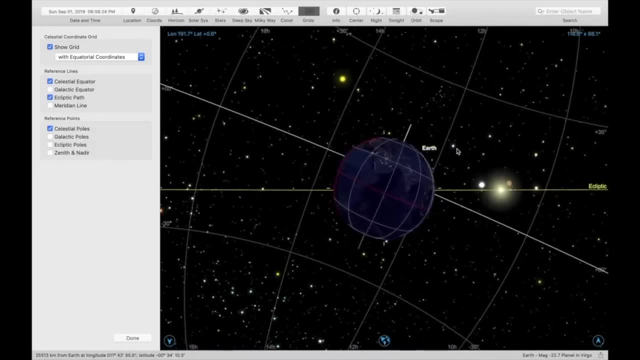 would be roughly close to the ecliptic itself. So we have this interesting coordinate system, which is on the stars and is an analogy with respect to the Earth's latitude and longitude. But notice how the Earth as it rotates, latitude and longitude go with it, but the Celestial Equator does. 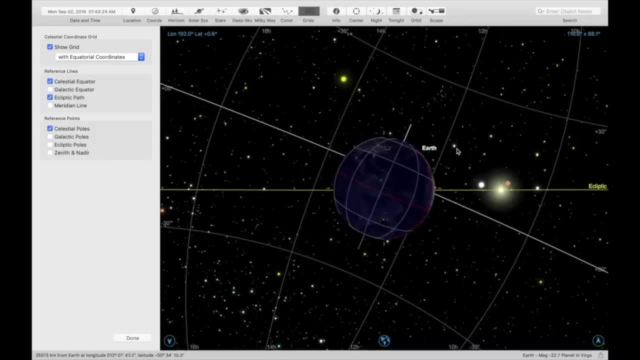 not change. So now, if we look at it slightly differently from a relative point of view and we go onto the surface of the Earth, then we see a completely different appearance. But I just wanted to make sure you understood that we have these coordinate systems which can be thought of as extending. 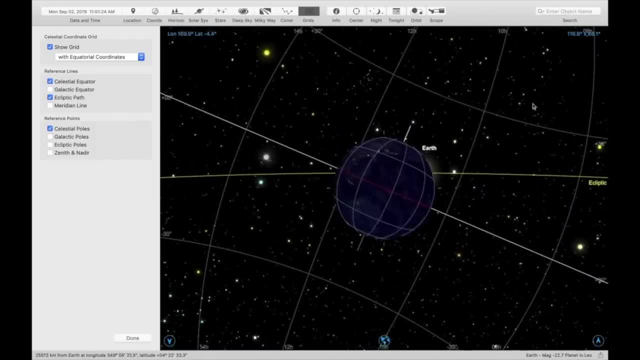 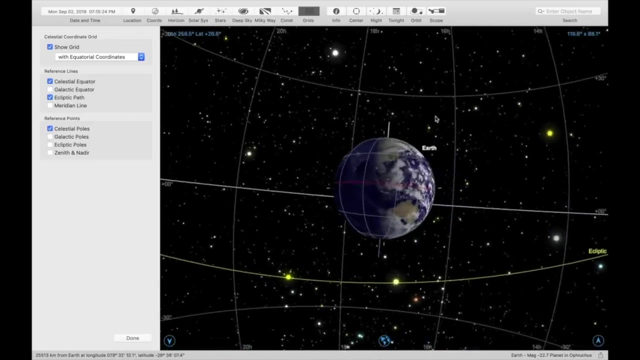 out into space. Now the latitude-like lines in the Celestial Equatorial coordinates are called declination and the longitude-like lines in the Celestial sphere are called right ascension, And so if we click on, say, some star or something, we will get the information about that star and it will 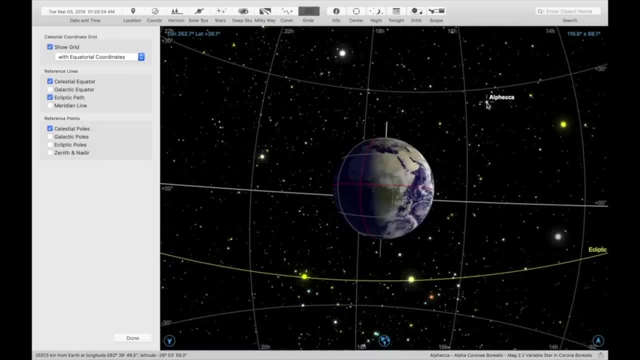 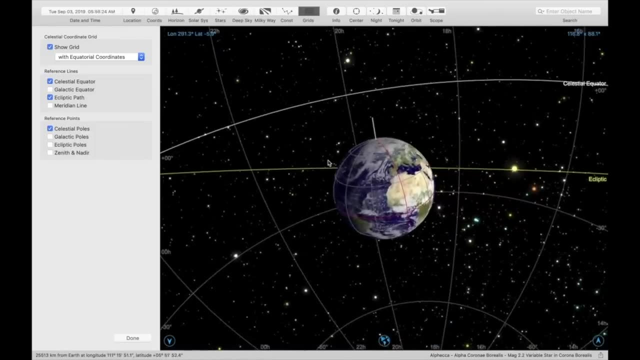 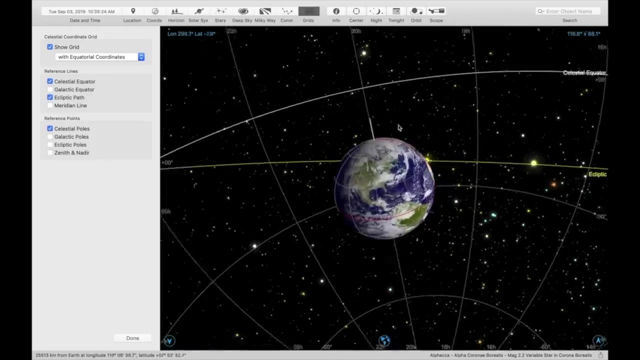 show what its latitude and longitude are, specifically its right ascension and declination. So that's interesting about those particular things, and notice that the latitude and longitude are fixed on the Earth and the Celestial coordinate system appears to be fixed on the 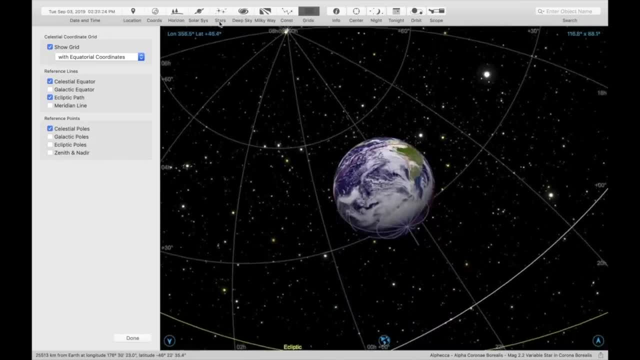 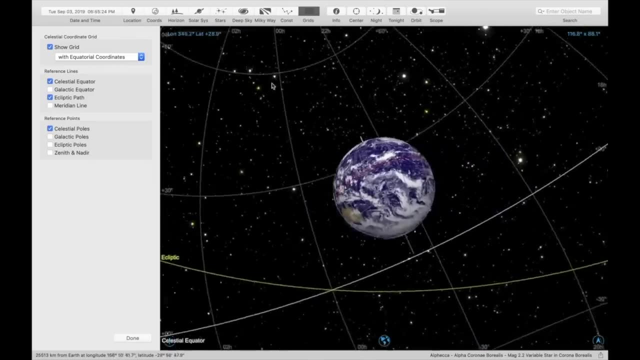 sky. So the sky is not the limit, but you can think of it as a grid that is superimposed in front of you or along with the stars. And why do we call it that? This is this imaginary concept called the Celestial sphere. 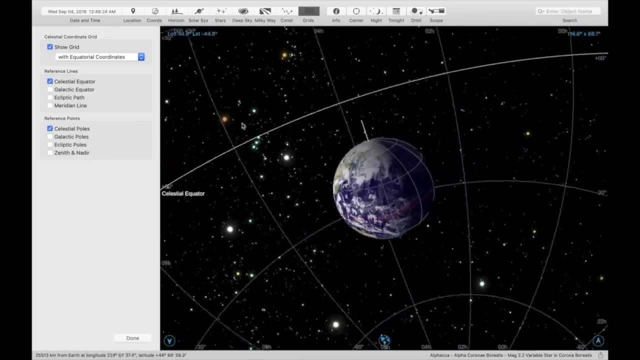 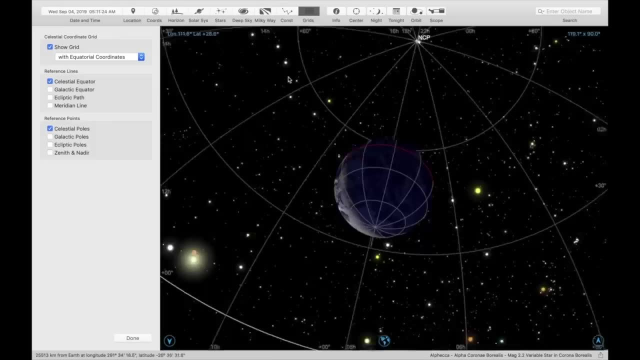 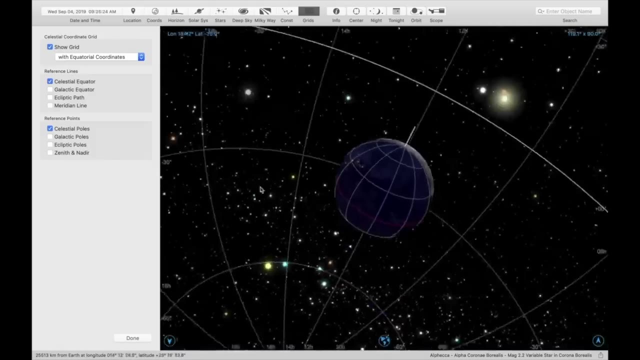 I'm going to turn off the ecliptic for this purpose, But the Celestial sphere is an apparent sphere that surrounds the Earth. That surrounds the Earth and appears to be above, below and all around the Earth, and what it appears to be is a grid or coordinate, or the apparent. 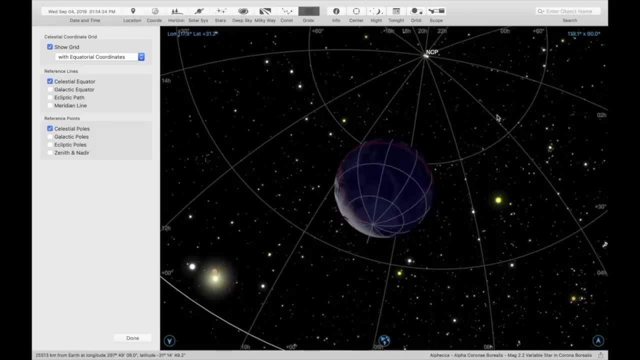 feeling that the sky is a grid or a sphere on all above us upon which the stars and planets appear to move, And so that's actually a pretty interesting way of thinking about it. But let's actually now dive in deep and go take a. 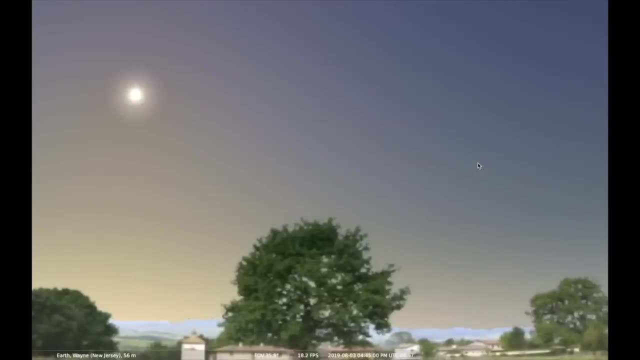 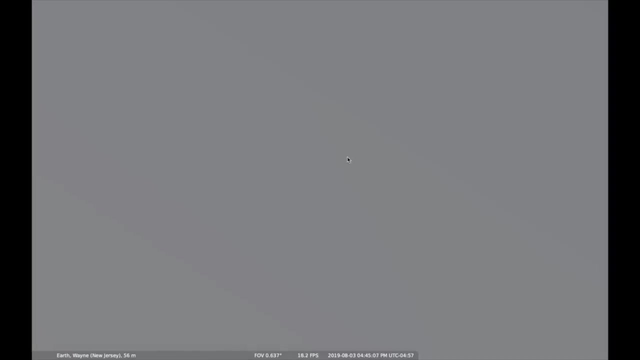 look at a different way of looking at it, which is a different piece of software, which is called Stellarium rather than Sky Safari. I'll close that off. And so now we're looking specifically at the hold on. let's zoom on out. So now we're looking at: 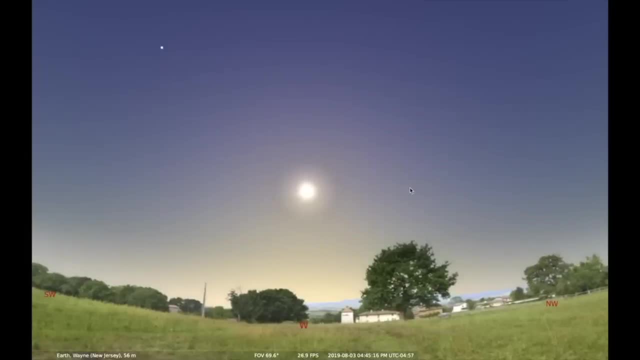 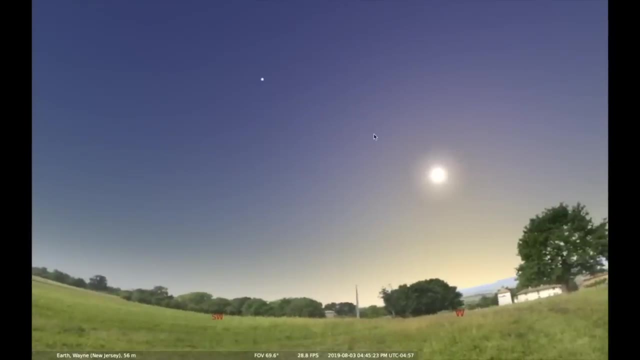 a software called Stellarium. the other one's called Sky Safari And we're looking at roughly today's time and date And if you look, we see the sky above us and around us and we can determine two different coordinate systems on the sky And the first coordinate 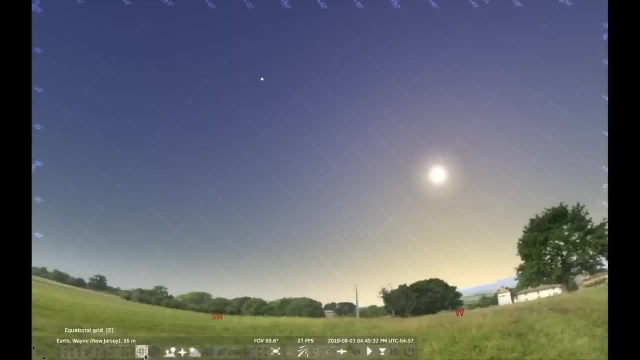 system we're going to talk about again is what we call the equatorial coordinate system. And there's the equatorial coordinate system we saw before, but now we're looking at the sky, as though we're looking at it from the ground. 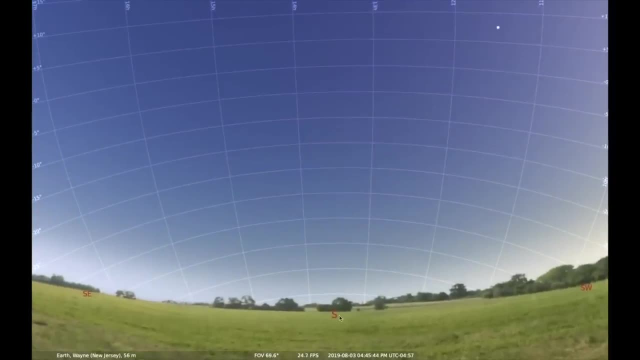 So if we look at it as though we're looking at it from the ground and we face, say, south from, say, somewhere in New Jersey, I'm just going to speed up time a little bit and watch what happens, Because now the Earth is rotating. 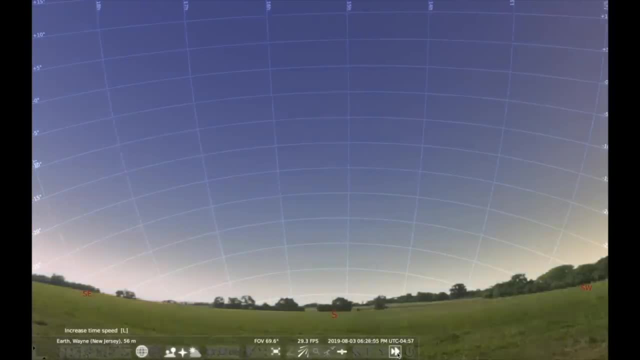 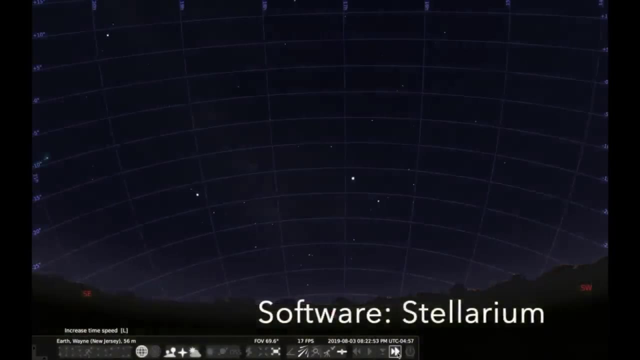 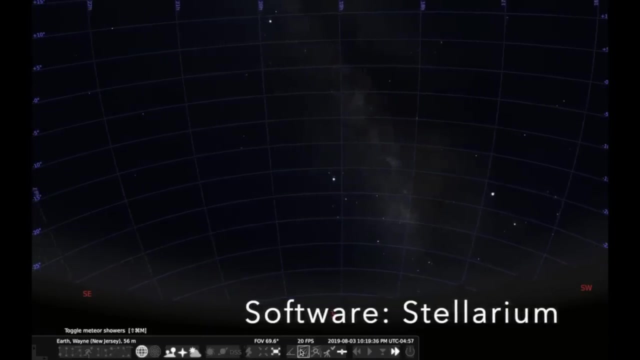 the celestial sphere or the celestial coordinate system, the equatorial coordinate system, appears to move in the sky, But remember that the celestial coordinate system is in front of the stars, which themselves don't move. So if the stars don't move, then what we have is: we have a. 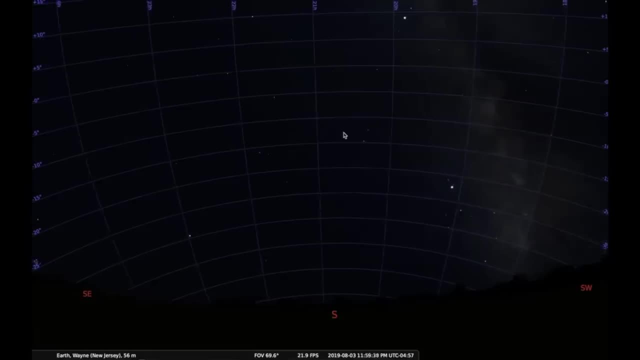 series of grid lines that are in front of the stars, And so the stars themselves appear to be attached to the grid lines, or at least as deep in as we want to go. We can go in as far in as we want, but that's a little crazy looking, so let's slow. 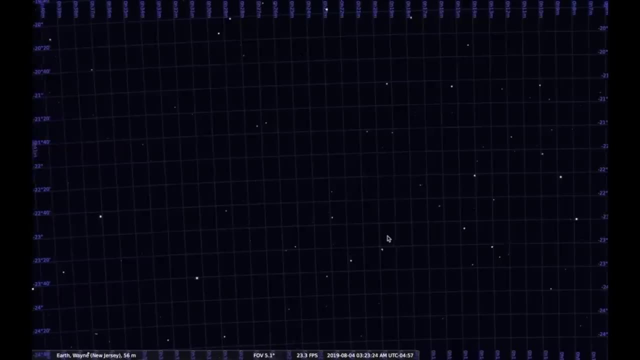 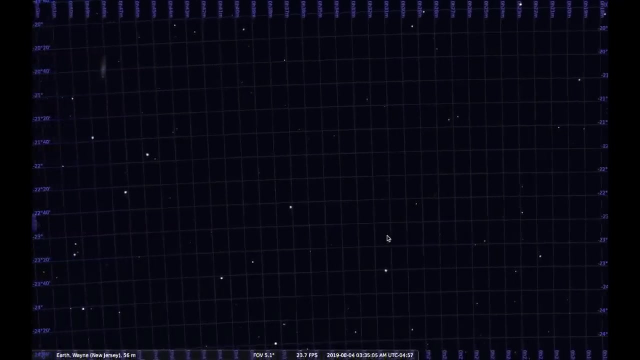 things down nice and slow. So you can see that individual stars- those are like moons or something that are zipping by, or asteroids, or actually probably just satellites, Earth satellites. So we have objects that are on the celestial sphere, that are enmeshed. 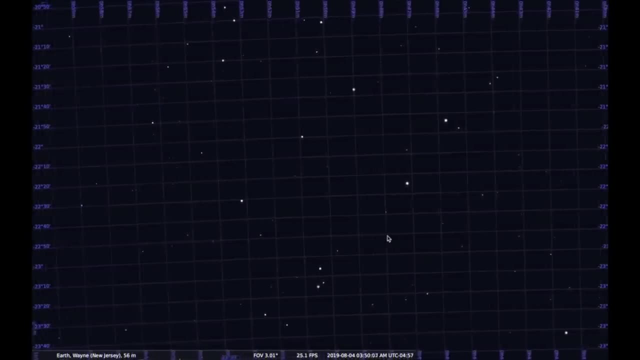 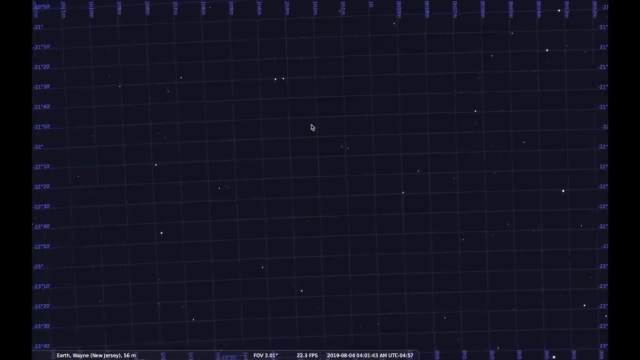 inside of this grid that we call right ascension and declination. Up and down on the celestial grid is declination and left and right is right ascension. So if we then zoom way back out, we're getting close to 4 AM. 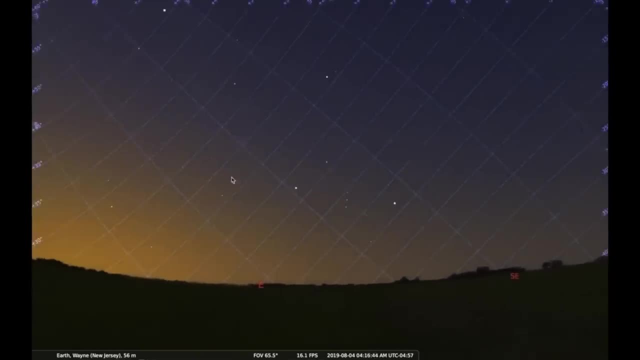 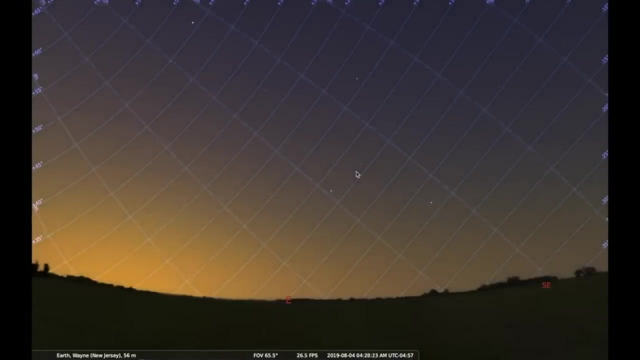 and that's getting close to sunrise. And as the sun rises in the east we see the grid slowly moving with it. There's the constellation Orion rising in the east. in early August. We don't see it very because the sun is close to it, But notice. 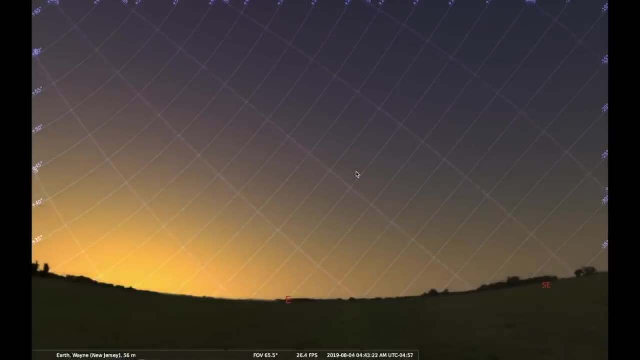 that, as the stars rise in the east and set in the west, we actually look at this object that we call the celestial sphere, and these grids are there for it. So why do we use this? What's the purpose? Well, it's to help us find our way around the sky. 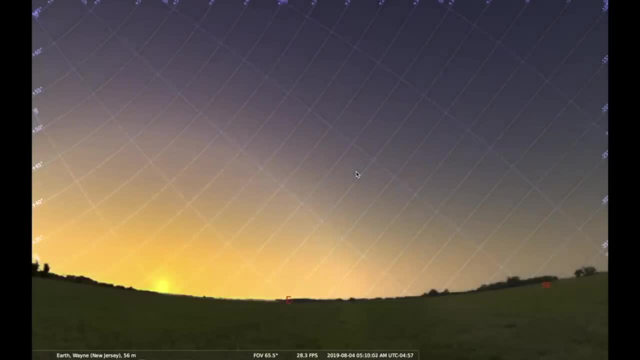 and find things in the sky. So what I'm going to do now is that, as the sun goes up, I'm really right now interested more in the locations of the stars rather than the sun, and the sun's very interesting, But I'm going to turn off. 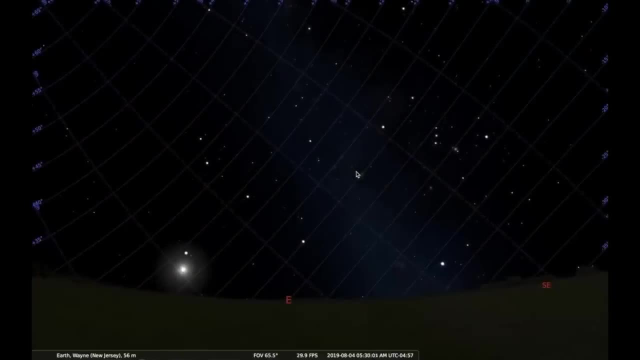 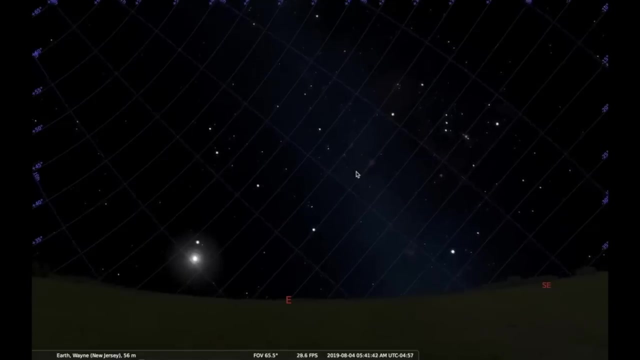 the atmospheric effects of stellarium, so it allows us to always see the stars. And so I've done that for a purpose, and the reason is I want to actually look at how the effect of the celestial sphere has on the motions of the stars in the sky. 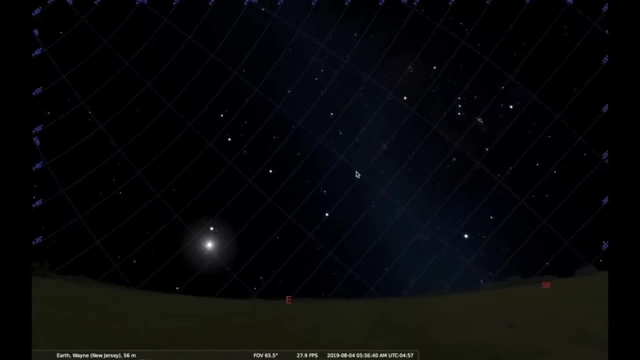 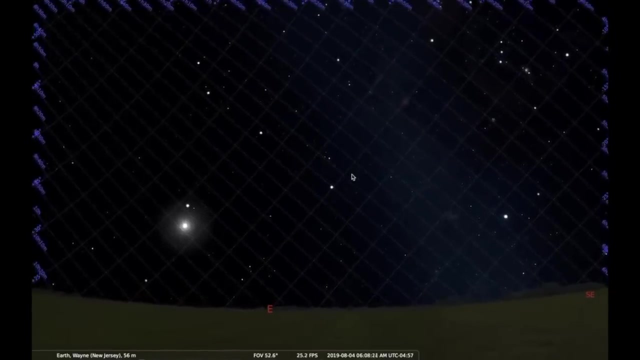 So notice, as we look at these objects, everything does appear to rise in the east. But when you say rise in the east, what do we mean? It doesn't rise straight up, does it? The stars aren't going straight up, They're going off at an angle. 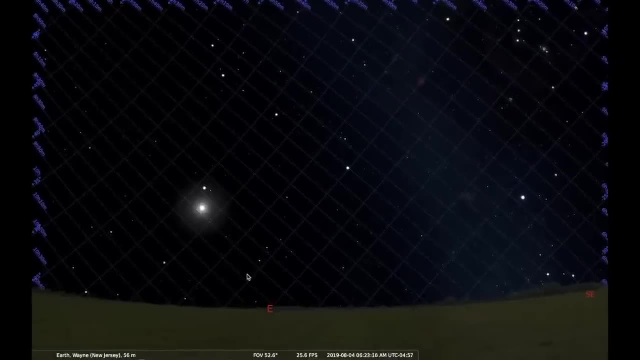 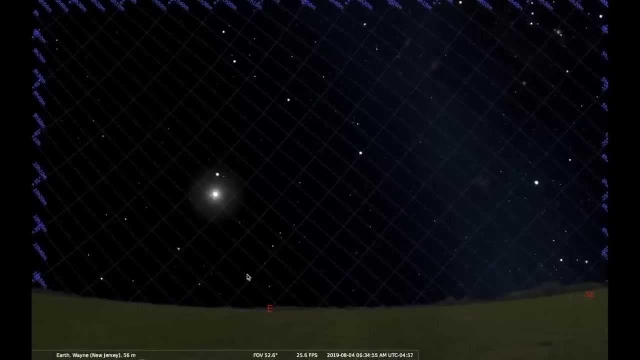 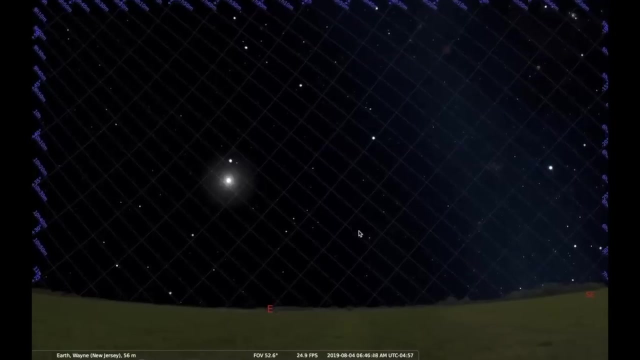 And what angle is that? They follow the grid lines. In fact, since they're attached to the grid lines, the grid lines just seem. they're not rising, they're going off to the side. So as the stars move, they follow the lines themselves And in fact they follow the 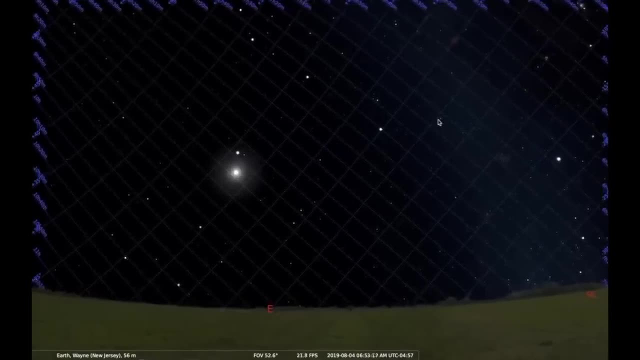 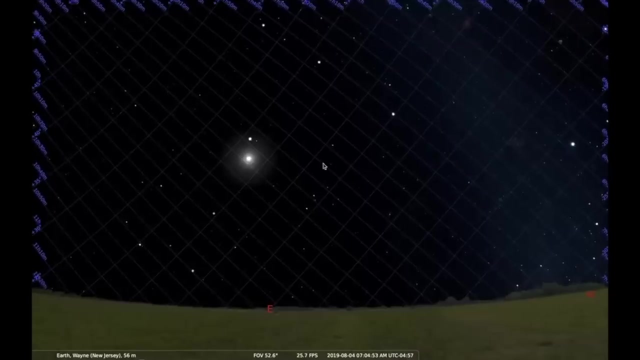 declination lines, which are going up and to the right, are the lines upon which we can see things moving, Or at least that is the apparent motion. Now, the lines that are going this way, the right ascension declination lines, those lines are: 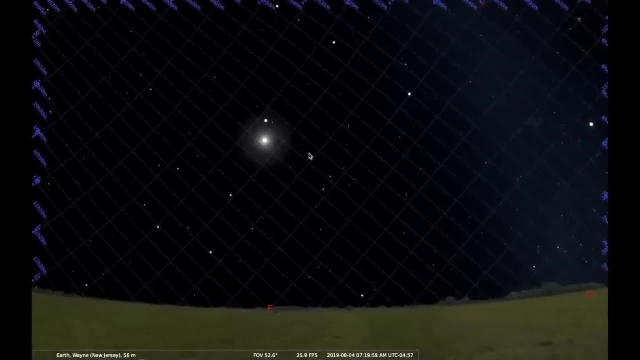 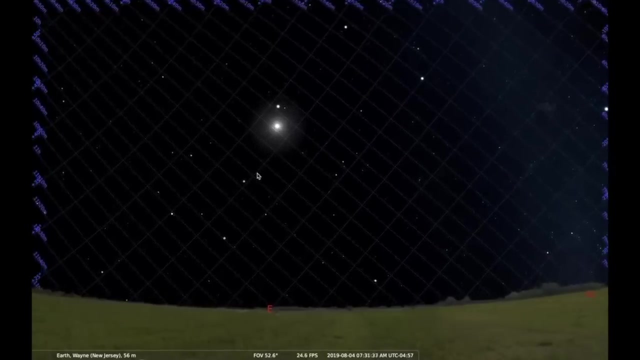 the ones that demark how fast, how long it will take for it to move from one point to another. So if I just let my mouse sit there in one location, we can see that star actually approaching. I think it's not actually a star, I think it's a planet. Yes, it's Mars. So we can see how. 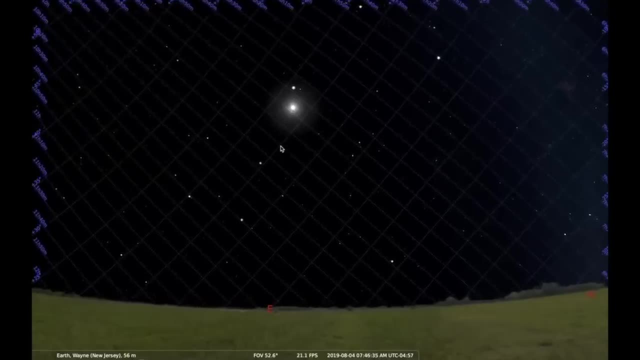 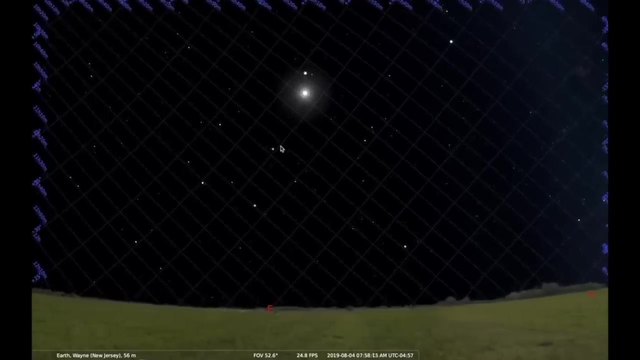 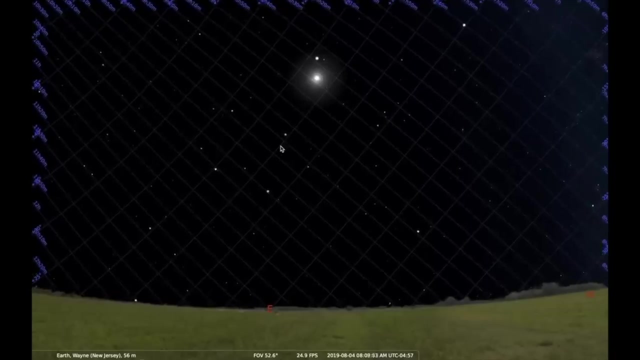 Mars will move with respect to the sky, And so if I place my mouse there, and because the distance between two of the lines is 10 minutes of right ascension, it takes 10 minutes of time for Mars to span one box length on there. So that's. 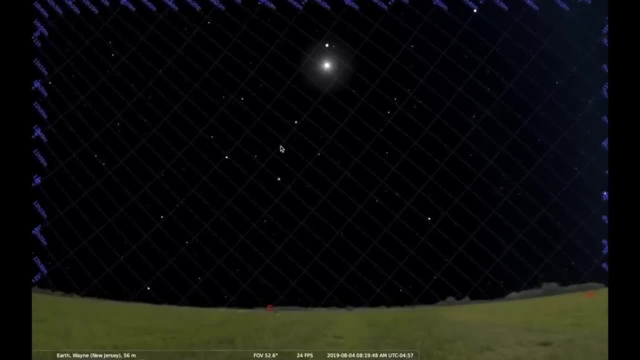 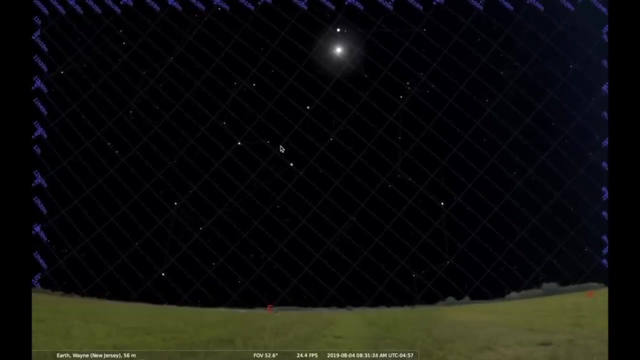 what those things mean. Alright, but our key thing is that let's actually now see what we mean by approaching the stars, And maybe this will help. I'm going to turn on the constellation lines to kind of keep things moving And notice that the constellation Leo over 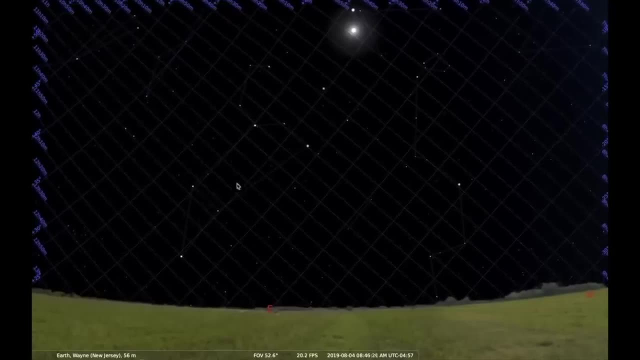 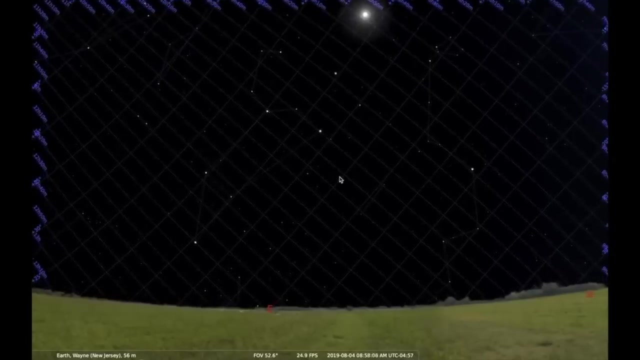 here, Leo the Lion, which is this one? here, Leo the Lion, stays fixed with respect to itself. The stars are not moving with respect to the grid, nor it is in the river, nor it is in any other constellation. The stars themselves. 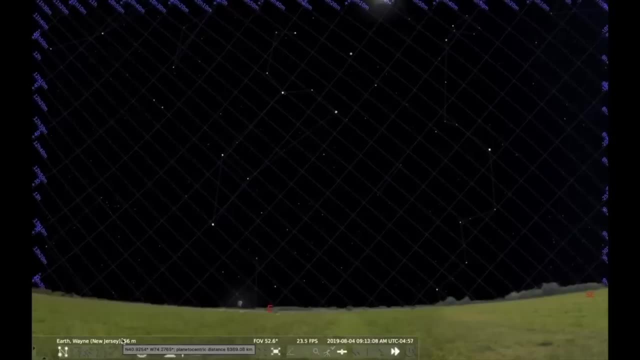 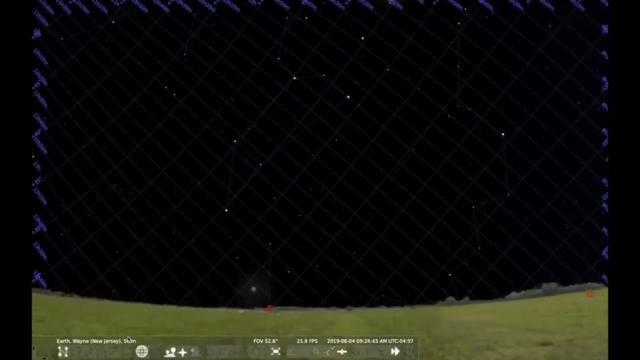 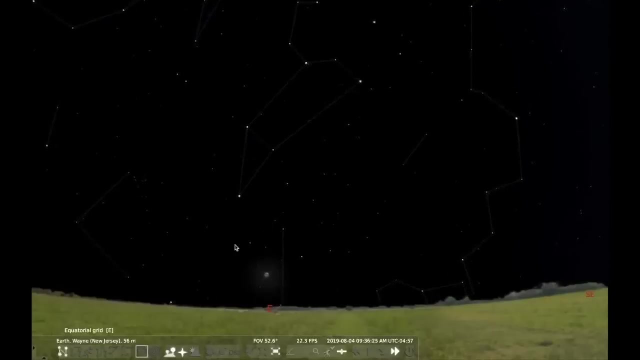 do not appear to be moving with respect to the constellations, And that's important to know, because when we actually do look at the nature of the stars, we have to. we want to know, we want to actually see how they behave when they rise in the east and set in the west. There's the moon coming. 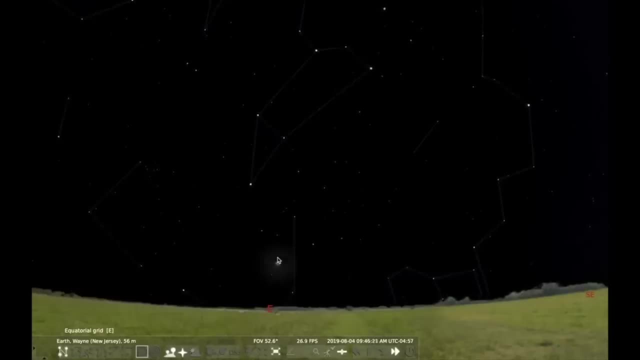 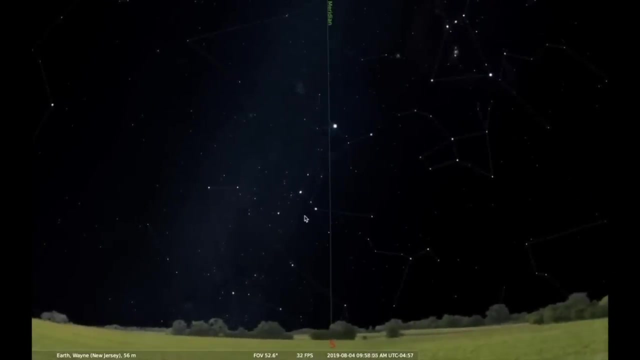 up, but notice that the stars appear to be moving up and to the right when they rise in the east. If we look towards the south, there's our meridian line. again, I turned it on and we turn. the meridian line actually tells us a very interesting thing about the nature of 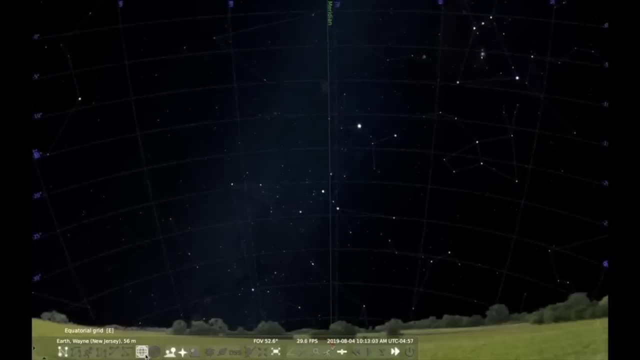 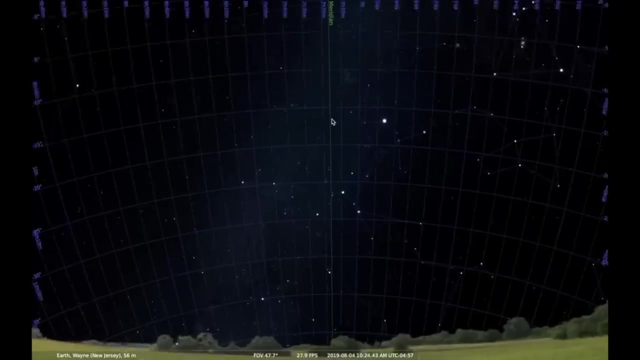 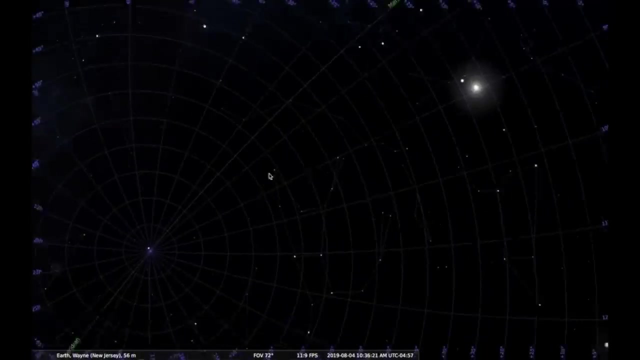 the equatorial coordinate system, because the meridian line goes from due south to the zenith overhead and then all the way to due north. So let's actually zoom out to see what I mean by that. So there's straight overhead and then down to the north And notice what an interesting thing is. 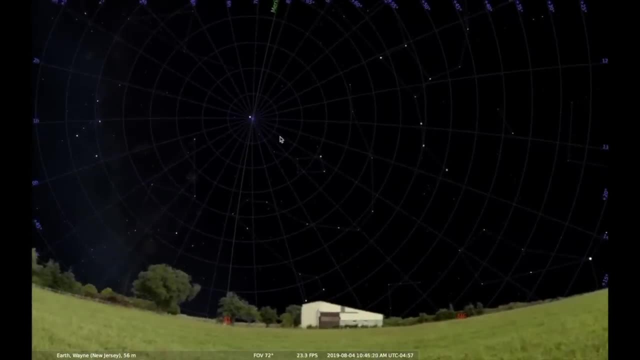 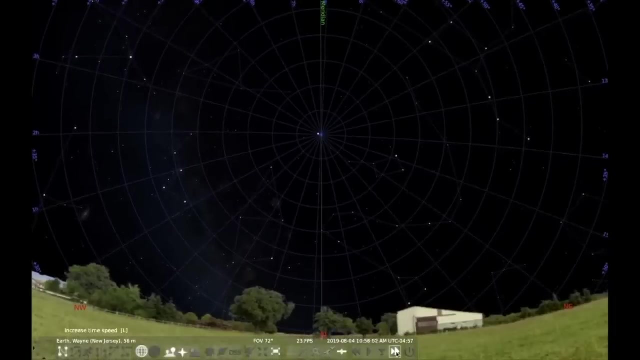 is that since we went straight overhead, we now see that the north celestial pole, which is towards the north, actually does not move. So the north celestial pole, we can spin time a little bit faster to see what happens, and as it kind of dizzies around, we see 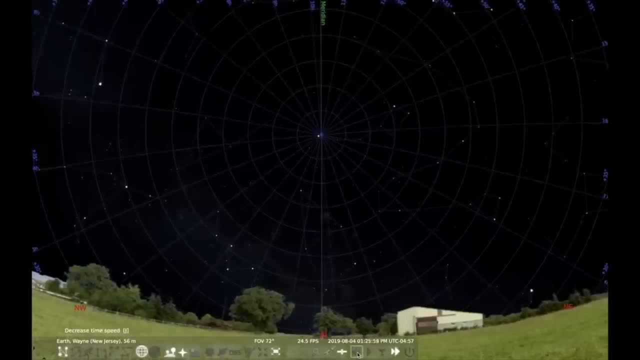 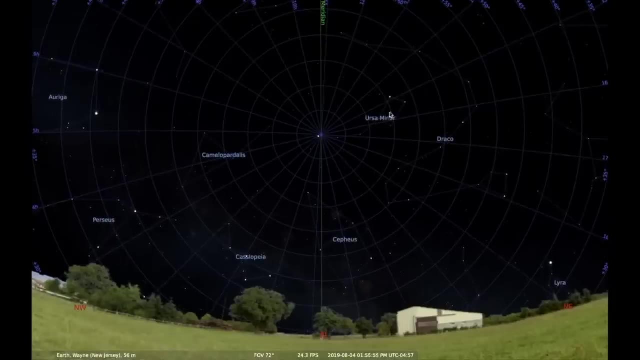 there's the north star, or the star Polaris, which is in the constellation Ursa Minor. In fact, I'll turn on the constellation names just for enjoyment purposes. There's the constellation Ursa Minor, which is the little dipper, and so you can see what I mean. There it is. 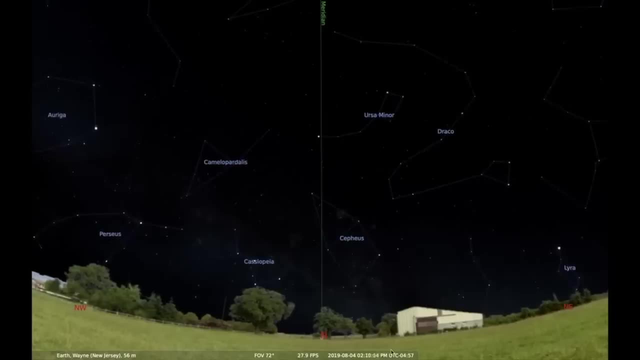 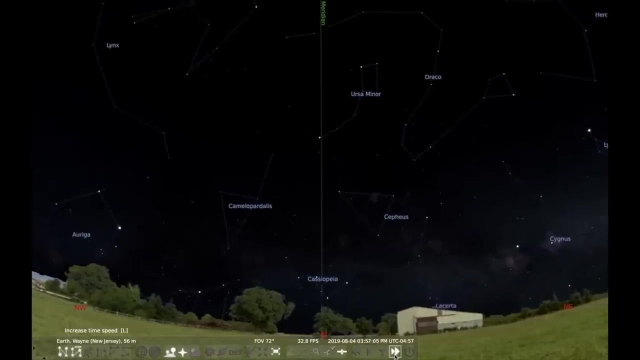 the little dipper is moving and the north star does not appear to be moving with respect to the north celestial pole. So notice I've sped up time. so many many minutes are going about. an hour is going by every few seconds, so we can see. 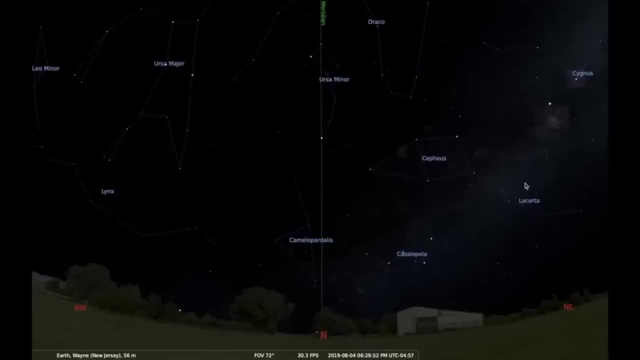 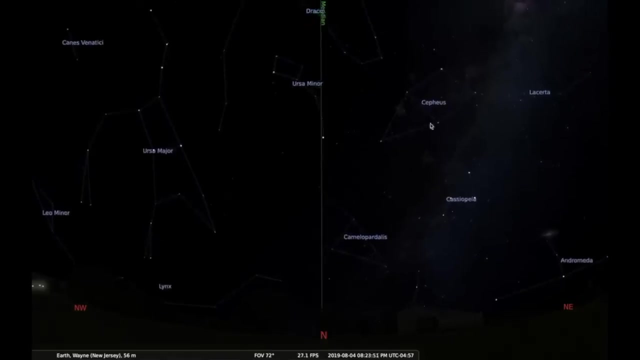 that, as the stars rise in the east and set in the west, there are some stars that are pretty special, like all the stars of Camelopardalis and the stars of Ursa Minor and the stars of Cassiopeia and the stars of Cepheus and some of the stars of Ursa Major. 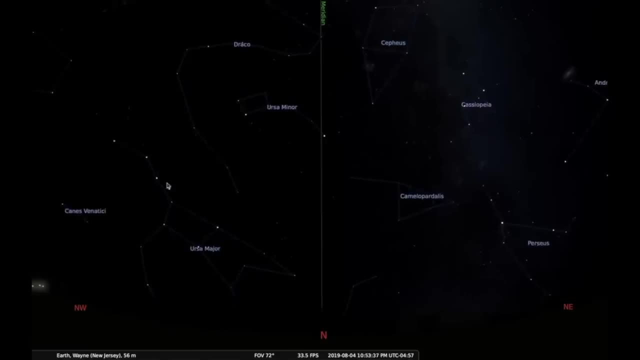 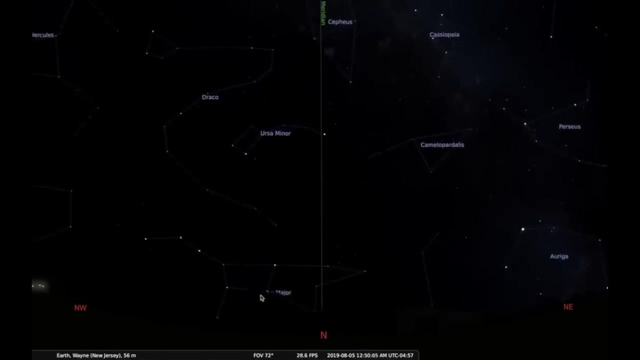 They never set. So notice that the stars of Ursa Major, the big dipper, particularly. look how low it gets to the horizon. for people in Wayne, New Jersey, It never gets below the horizon. Such stars are called circumpolar stars, The stars of 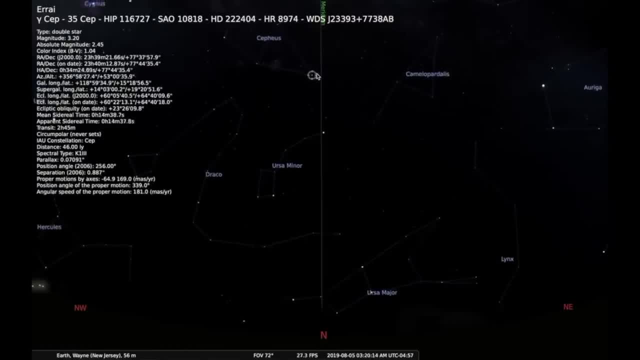 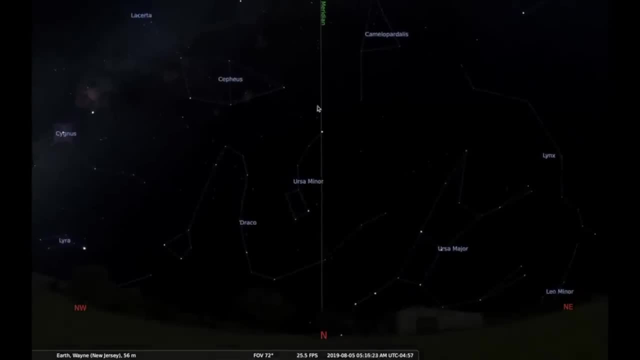 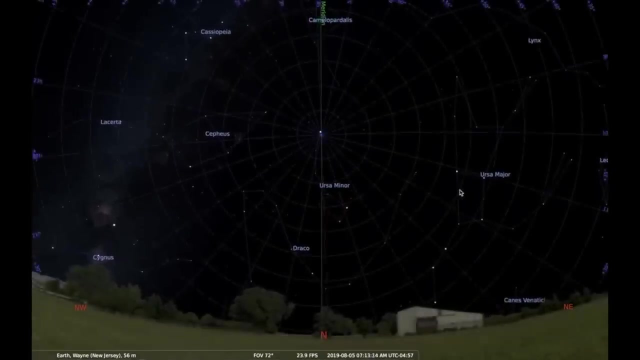 Ursa Minor are circumpolar. The star Eri in Cepheus is circumpolar, meaning they go around the north celestial pole and they never set. So let's turn the grid back on to see more interesting stuff. So there's the north equatorial region. 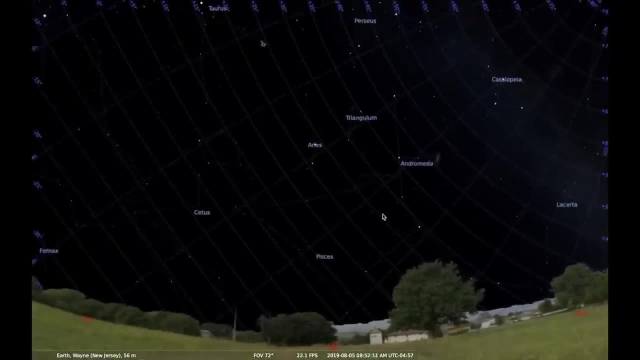 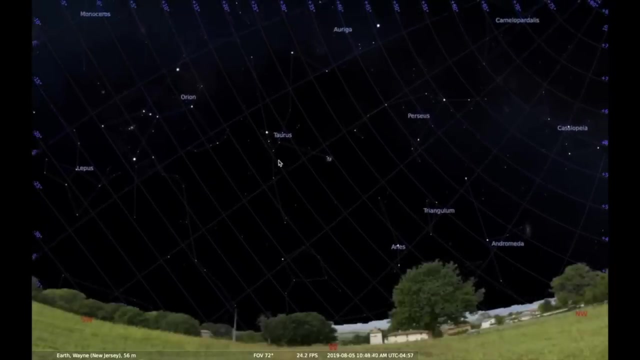 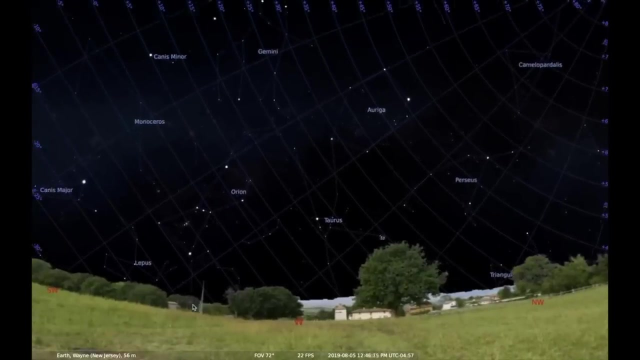 and now we go and look due west and as we see things, looking due west, we see the constellation Taurus coming straight at an angle. And what is the angle with respect to the horizon If we look due west and go straight this way, make an angle from the horizon up to the celestial? 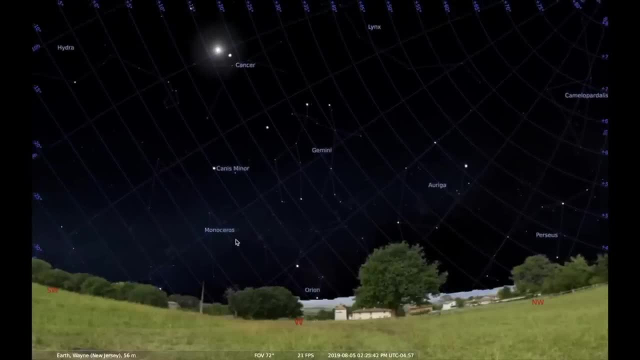 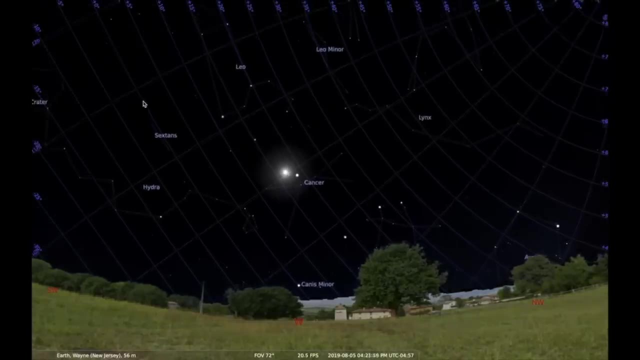 equator, this angle between the celestial equator and the horizon at due west or zero degrees. the celestial equator is here. what we see, let's see if I can turn that on. no, that's the ecliptic, and maybe 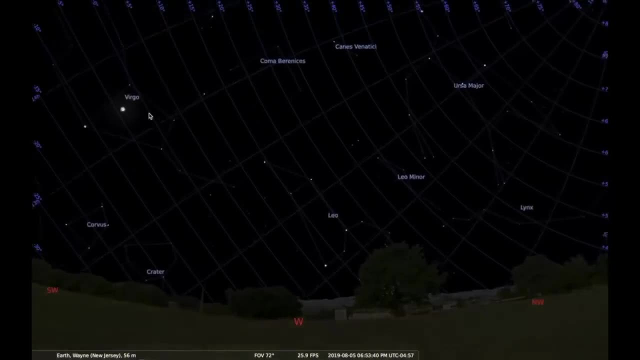 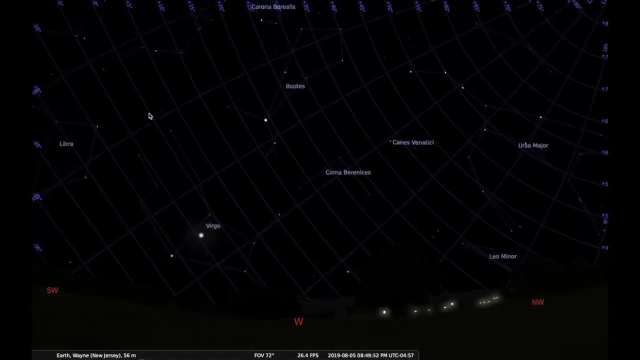 there's, where's our celestial equator? Okay, let me see if I can find it again. there it goes, But in any event, we see that- oh, I think I lost it- we have the angle between the celestial equator which is here, which is zero degrees. 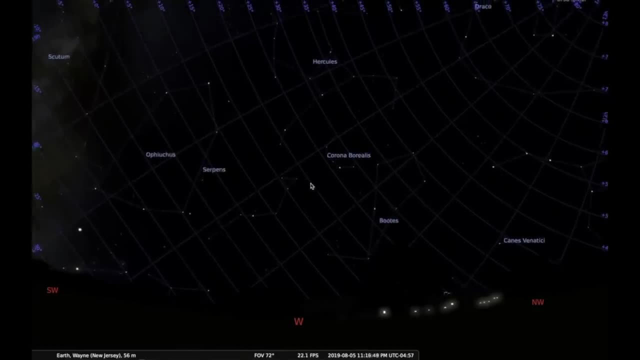 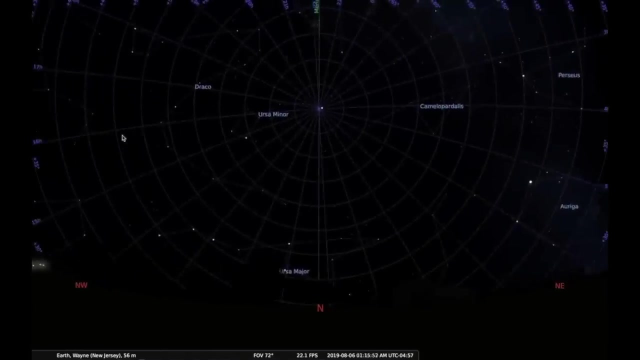 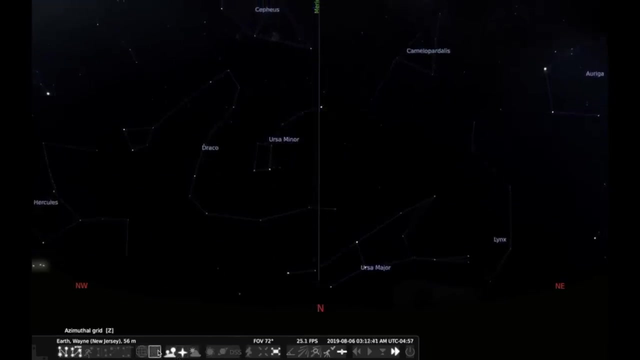 declination and the horizon is equal to 90 minus the altitude of the north celestial hole. Well, what do we mean by altitude? Well, for just a second, let's turn off the equatorial grid and turn on the azimuthal grid. Now, the azimuthal. 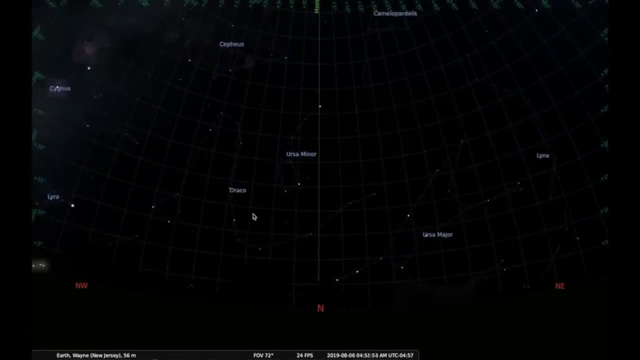 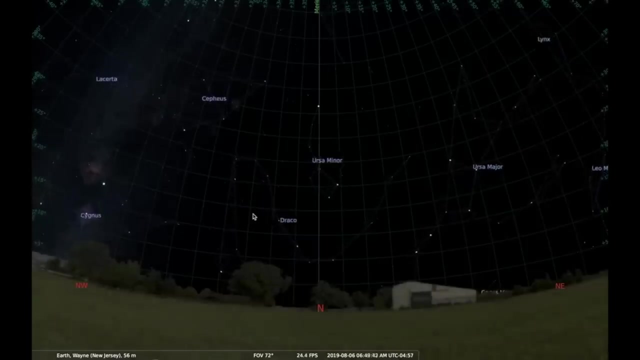 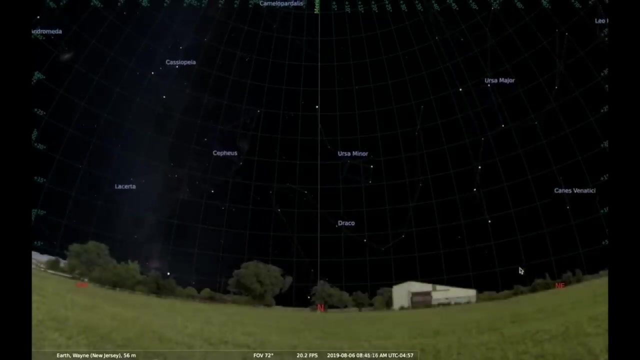 grid shows the position of the stars with respect to the horizon. Now, this is your perspective that you see on the sky. So this is a grid with which the stars are moving according to. But now what do they move? They say, well, each of the lines from the horizon up. 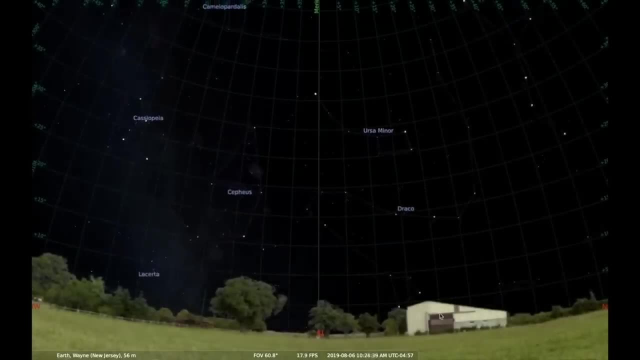 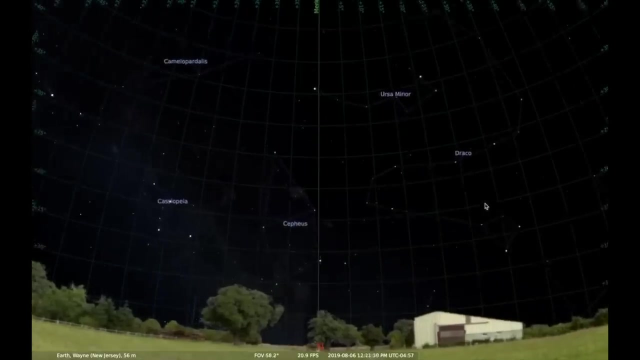 is a few degrees of altitude, So it can. if it's at the horizon, it's zero degrees altitude. there's five, ten, fifteen, twenty degrees above the horizon in altitude. We can go as high as we want, but as soon as we get all the way to 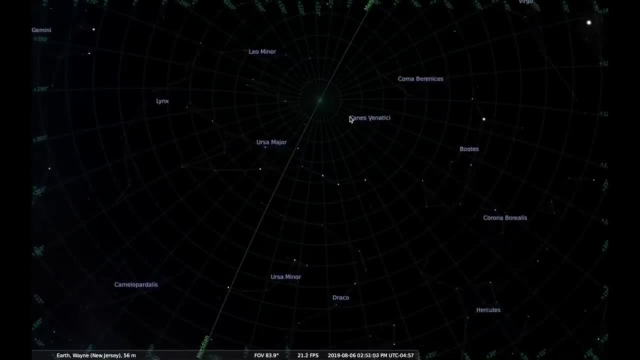 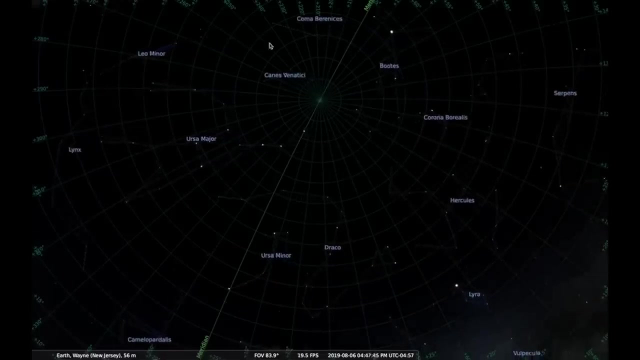 straight overhead. we see, straight overhead is the zenith, And the zenith is the place that is directly overhead. That's what we call the zenith, And you can see that all of the altitude lines kind of go all the way to the top And there goes the 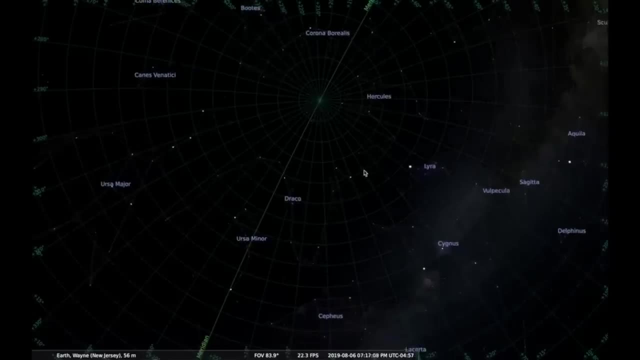 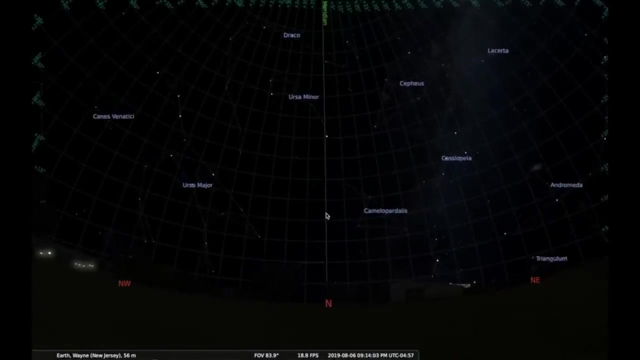 stars of Hercules are about to pass through the zenith And we see that there's also this other line, the meridian line. And the meridian line says, let's say, we go to the right. So this is five, ten, fifteen, twenty degrees to. 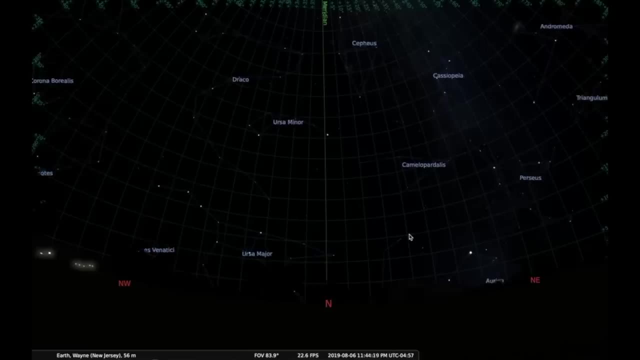 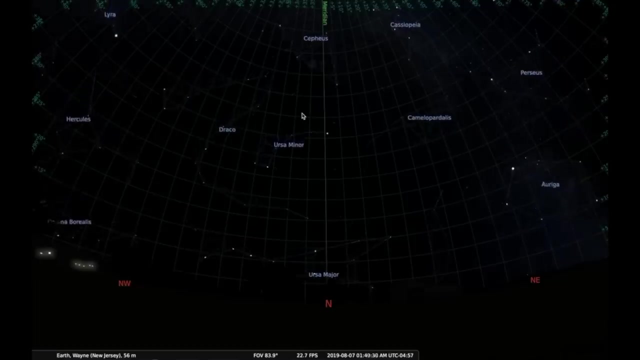 the right all the way around, from north to east, to south, to west, to northwest and back, And so that is called azimuth, And your azimuth angle is how many degrees from north to the east you're looking So we can find things in the sky. 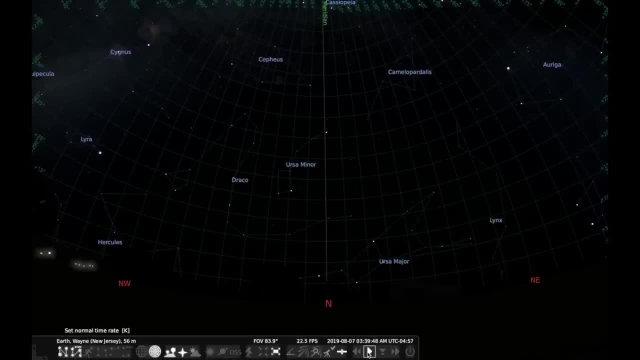 if they're going at a normal rate, like normal rates, like this is normal one second per second- then things don't move very fast. However, they move fast enough so that the altitude azimuth system doesn't work over time for showing people things. 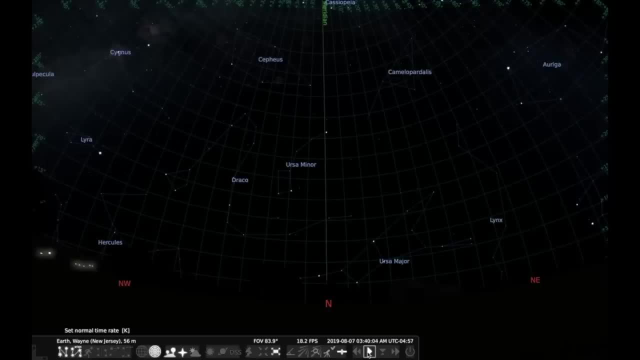 Also, it doesn't work, if you're looking for things, that you're trying to tell a friend in another location to go look for something. So let's say there's something really interesting happening right now, on August 7th, at three o'clock in the morning and you want to tell somebody. 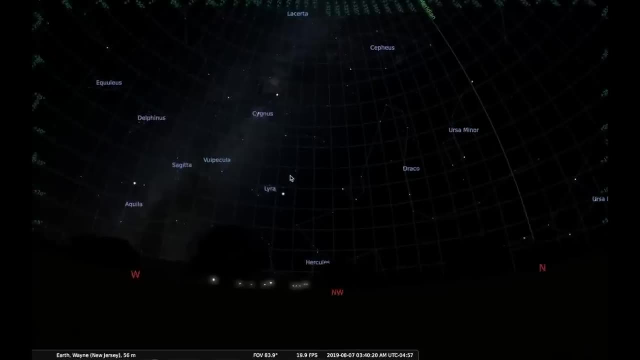 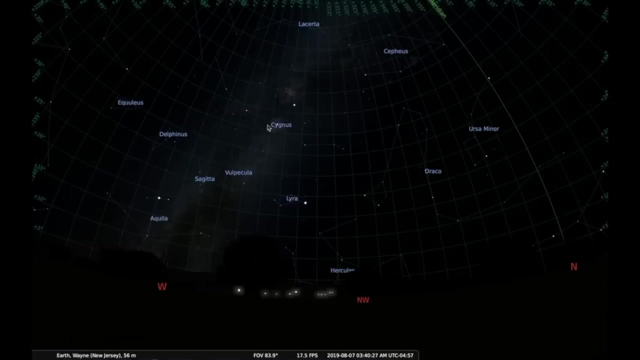 that's very far south of you what to go look for. So right now, at three o'clock in the morning, maybe there's a star that's exploded or something. Maybe there's a supernova that's happened. There's a milky way in the background, so maybe it happened. So we're. 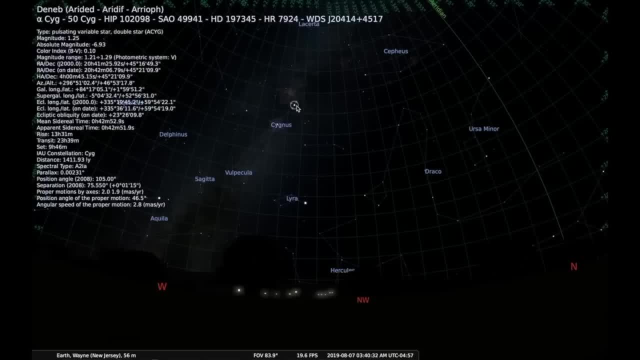 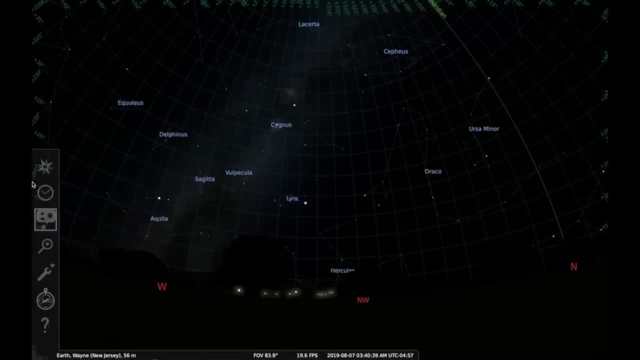 going to say: your friend says, wow, what's happened with the star Deneb? Something is flaring or something happened in Deneb, or maybe you just want to point out the star Deneb for your friend, And your friend say lives. 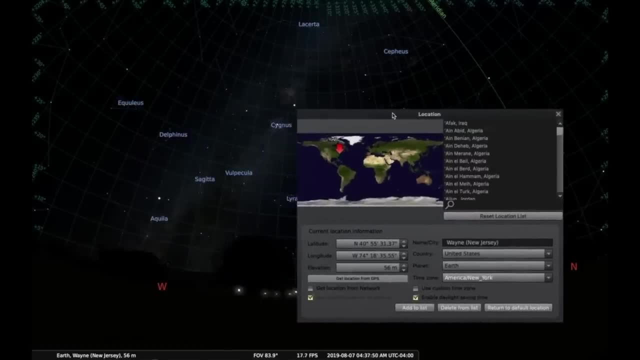 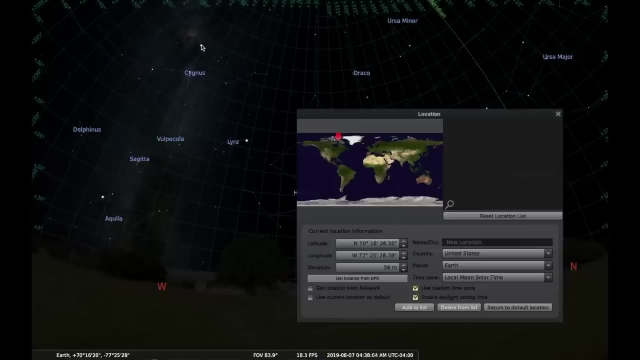 in a different location on Earth. Maybe your friend lives very far north, really far north, almost to the northwestern territories of Canada, So you tell them to go outside and look and wait a second. something's different about that. Notice what happened. The star Deneb is now very, very, very far. 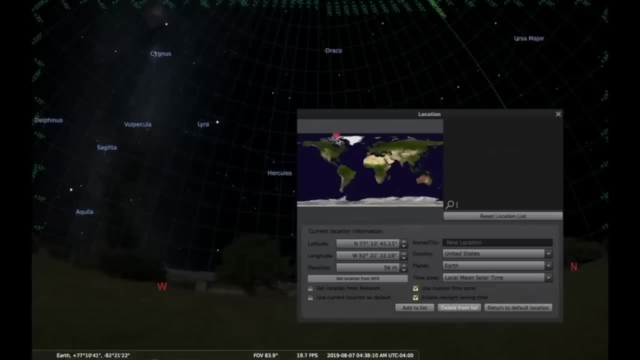 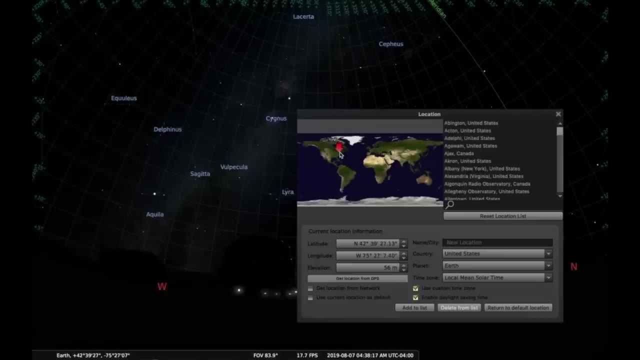 north. Let's see if I can find. or at least there it is, You can see it has a totally different location on the sky, So the star Deneb is much higher in altitude than for people that are here. It's also got. 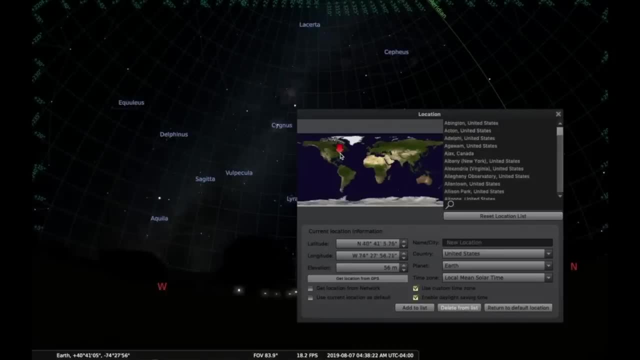 a different location in the sky, for the horizon as well, because of their different position on the Earth. So Deneb has a much higher altitude. but if we go very far, let's say we go all the way to the north end of Greenland- Notice that we're way. 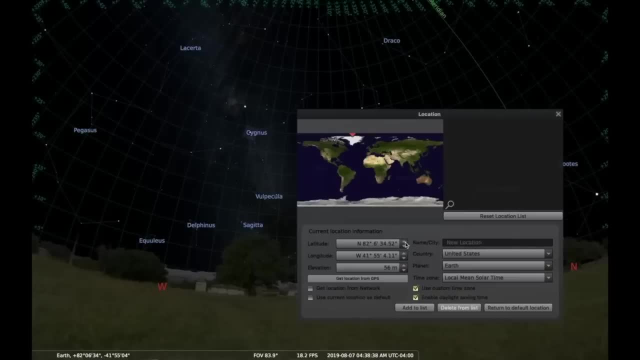 up north, very far north, even farther. Let's go all the way as far north as we dare. And if we go north, north, north, north north, and maybe we go a little bit further back west or something, Let's go see if we can push it back. 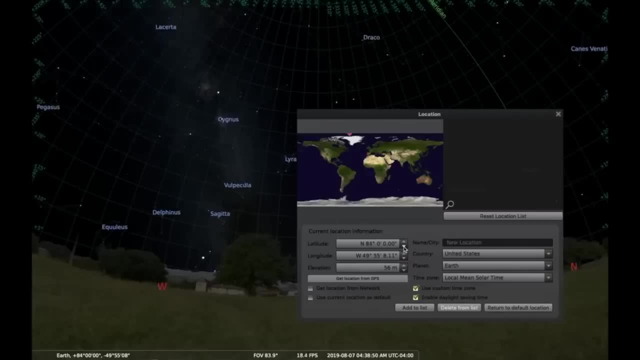 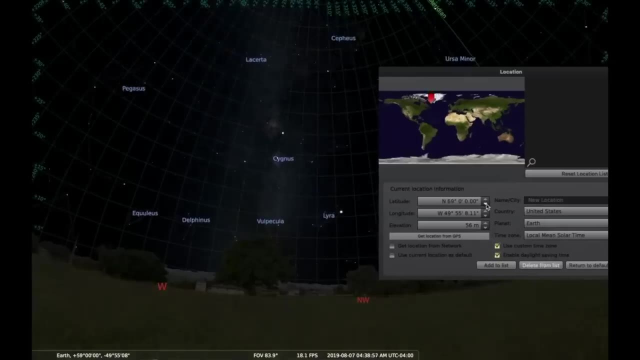 Notice that as far north as we are, we actually can't, we actually don't see too much difference. So actually, there we go, Let's pull. let's go farther south in our altitude, Go back over to New Jersey, and there we go, Let's actually just go straight north from. 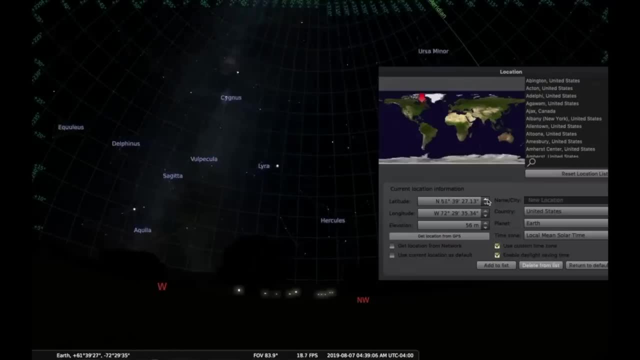 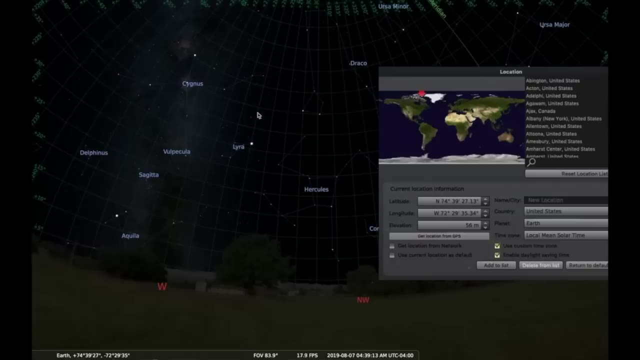 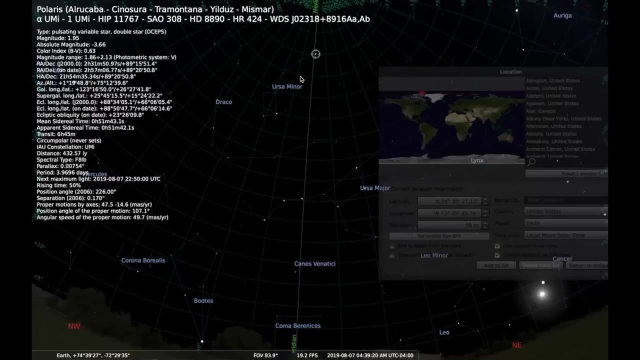 New Jersey and see what happens. Interesting huh. Notice how we go straight north and the altitude of Deneb has changed. But actually let's now take a more interesting look and go all the way over to the Little Dipper. So there is our favorite star, Polaris. So Polaris is here. 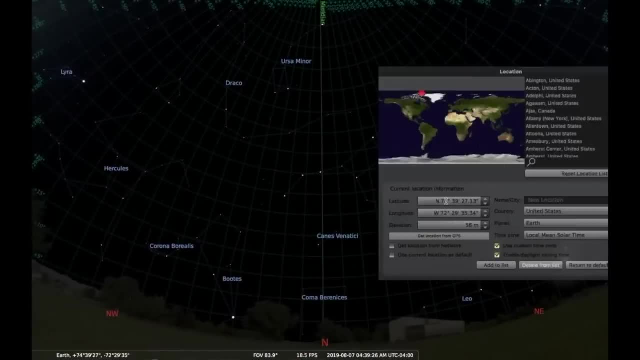 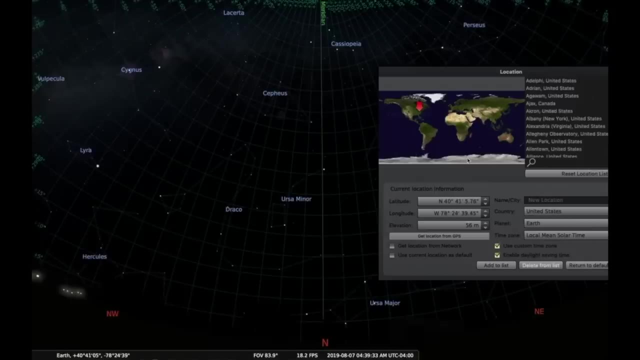 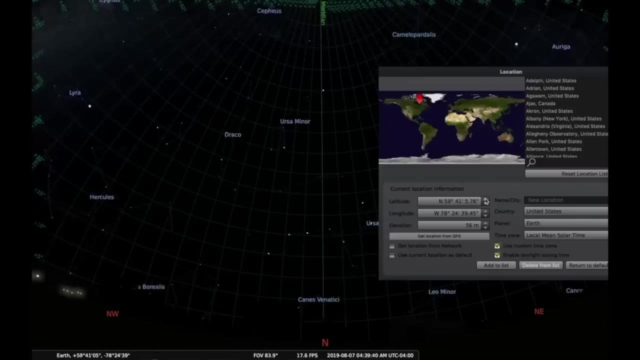 and now we're very far north. but let's change our location on the Earth and we'll start here, Somewhere in central, in the middle of the United States, and then what we're going to do is travel northward, And as we travel northward on the United States, we see that the 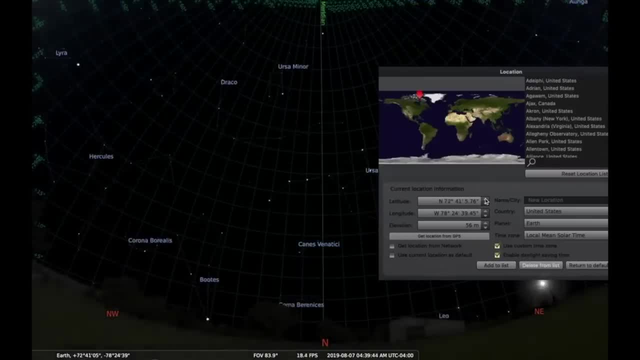 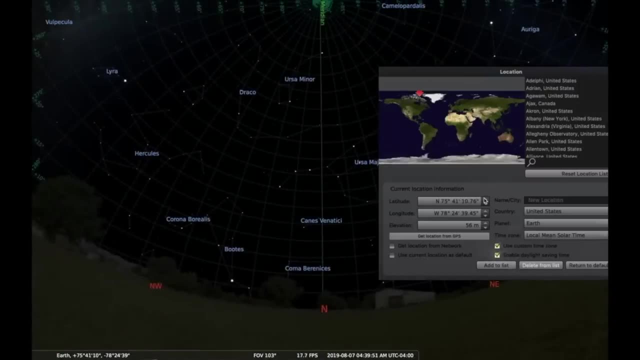 north star. it gets higher and higher and higher off the horizon until we finally get all the way to. we get all the way very, very north: 80 degrees north latitude. What's going to happen when we get above 80 degrees north latitude? 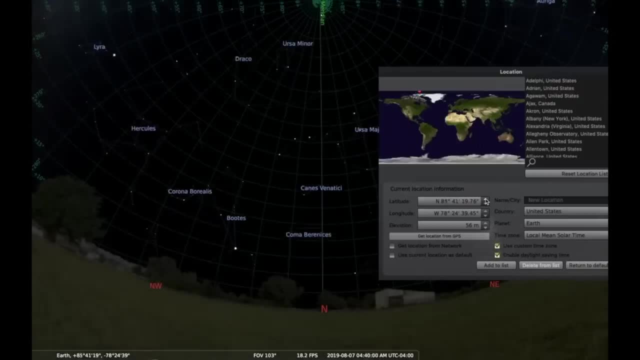 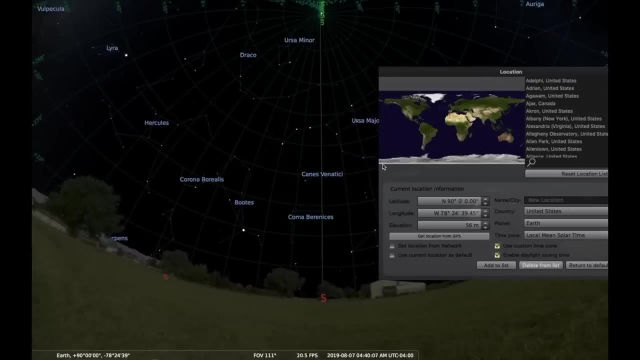 So 75,, 80,, 80 degrees north latitude keeps going, up, up and finally, once it gets to 90 degrees north latitude, that is the North Pole. The North Pole is 90 degrees north latitude and when you're at the North Pole, things look really. 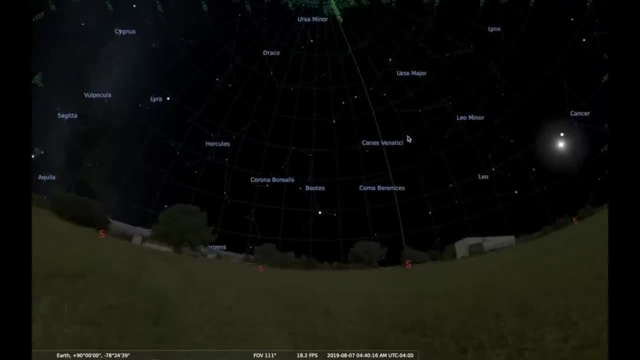 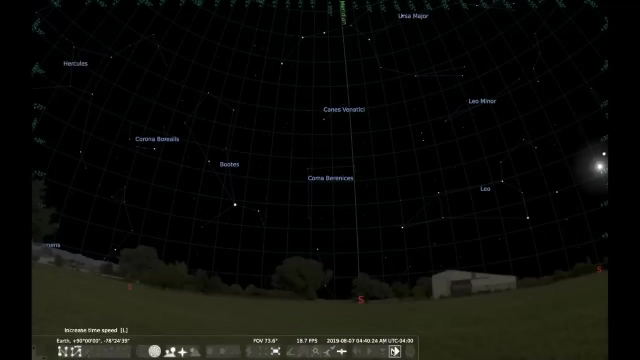 different. So let's close this out for just a second, And I'm going to just actually let time go a little faster and we'll see what happens. So I'm looking what looks to be south, at the North Pole, but if I just 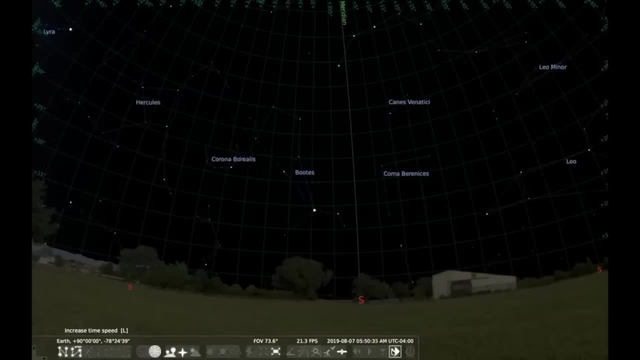 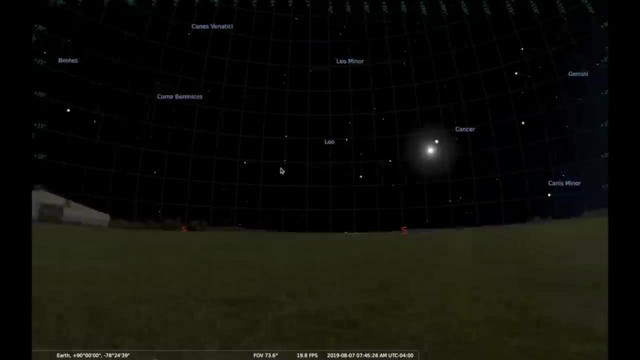 kind of let time go, notice how the stars. what are the stars doing? They don't rise, they don't set. They actually stay at the same altitude. None of them are rising And even interestingly, I'm going to tag the sun and follow the sun around As I follow the 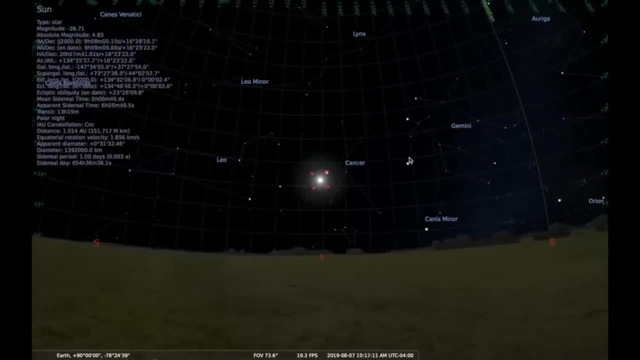 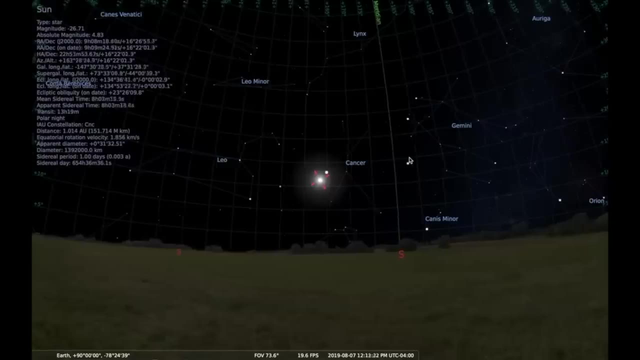 sun around. notice how it's going around the horizon, and every direction is labeled S for south. When you're at the North Pole, there is no other direction but south. There is no east, There is no west, There's not even a. 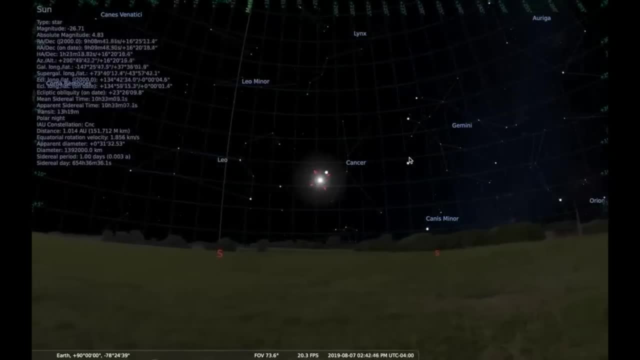 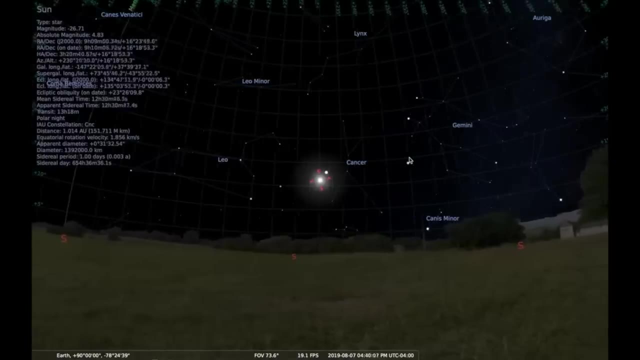 north anymore. When you're standing directly at the North Pole, the only direction is south. And notice what's happening with the sun. It's neither rising nor setting All of the stars, they just keep orbiting. And that's because, when you're 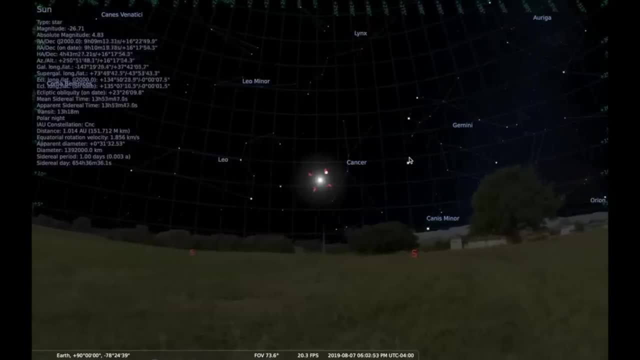 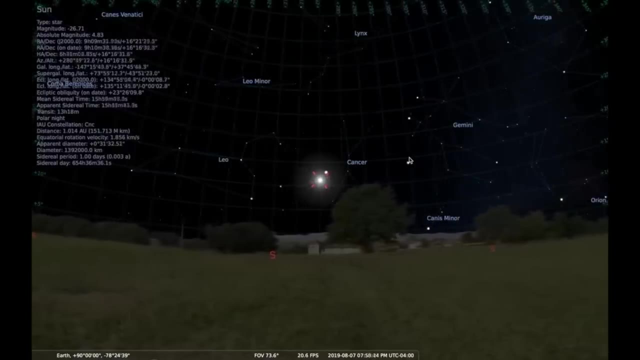 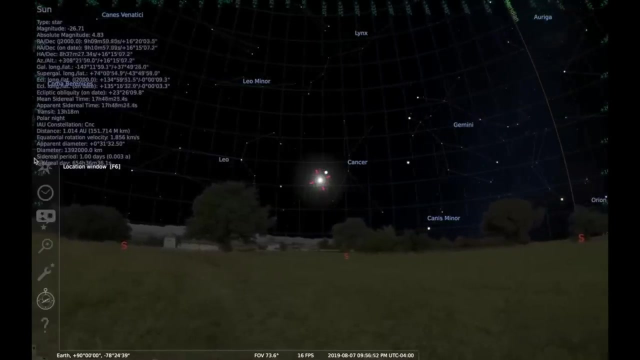 at the North Pole. your horizon is directly below the axis of the Earth's rotation, So nothing can rise or set because of your altitude, because of your latitude. So let's actually take our trip and we're going to go back south again And I'm going to reduce our 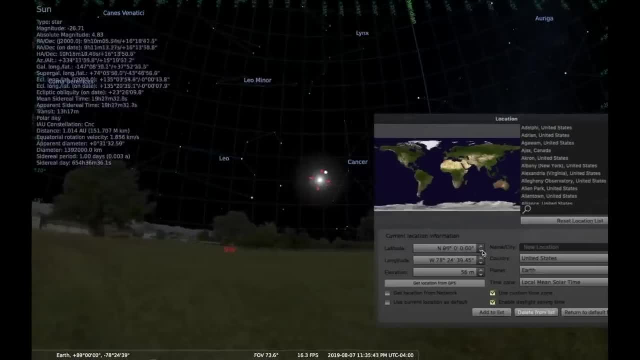 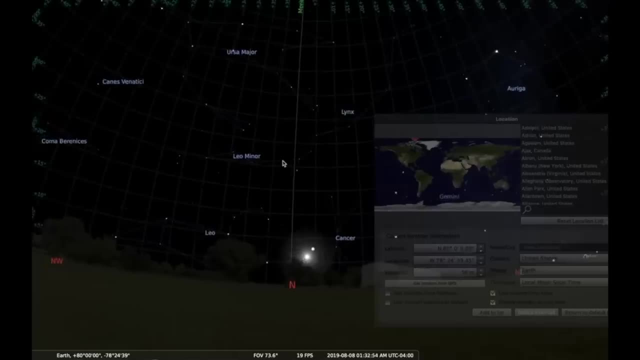 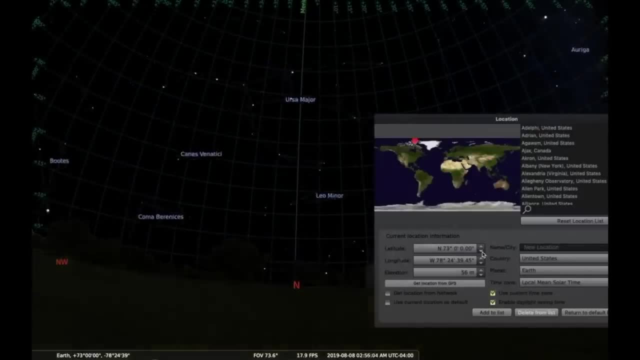 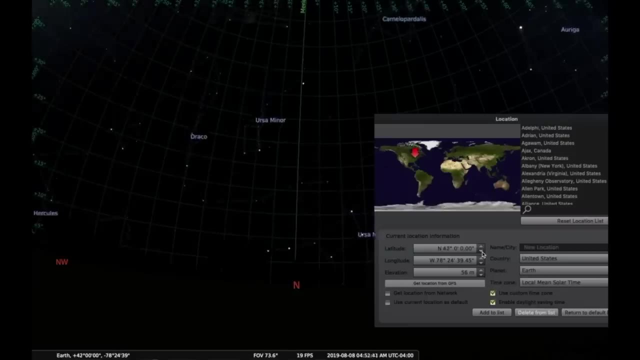 go back in here And here we go. Let's go down south, And as I go further and further south, we see that the stars that are circumpolar are fewer and fewer, And so now that's roughly our latitude, my latitude in New York City, And let's keep. 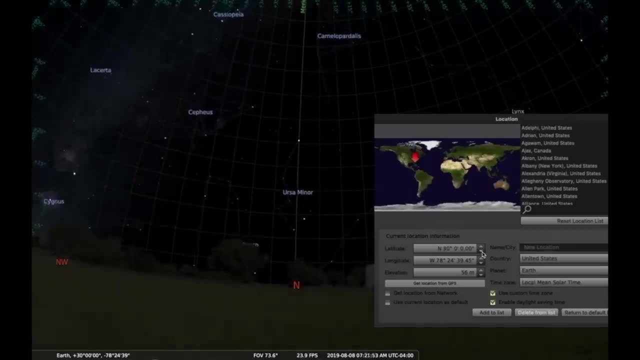 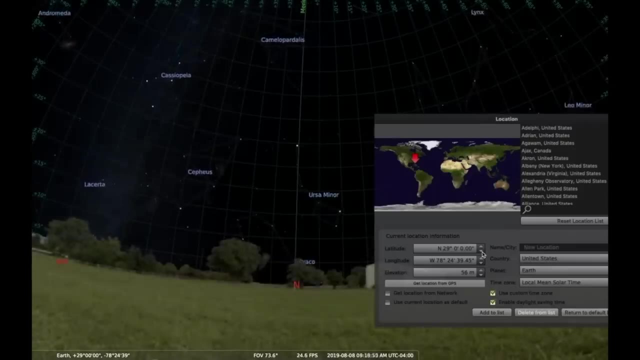 going further and further south. I'm going to take it all the way down, to, say, the southern tip of Florida, which might be 29 degrees above the above the above the equator, And let's keep it going further. If we go below, into Cuba, it's about 25. 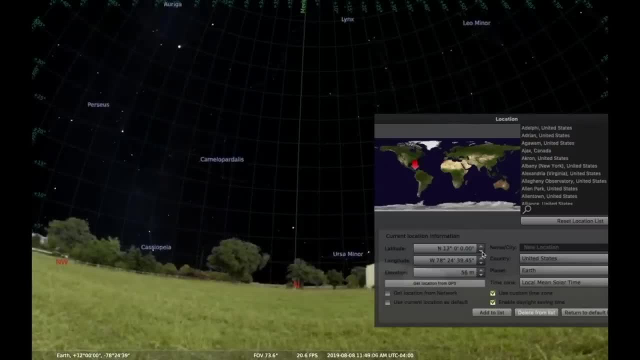 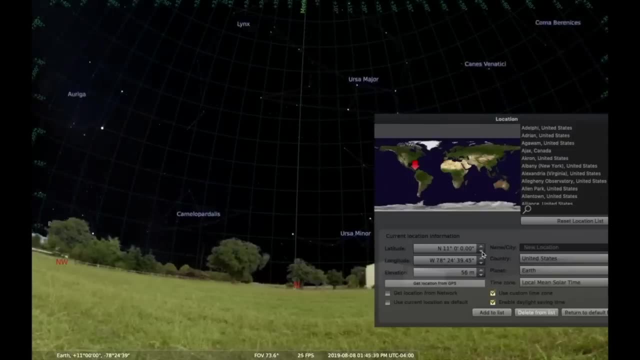 degrees. If we go all the way down to say, oh, we're looking roughly in the Panama area, Panama might be only 11 degrees north of the equator, And so notice what happened with the north star. The north star is really low to the horizon. 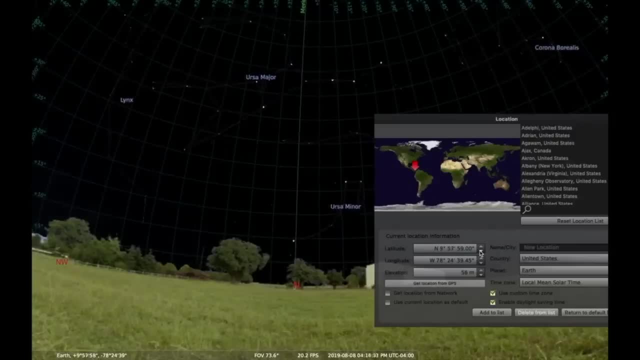 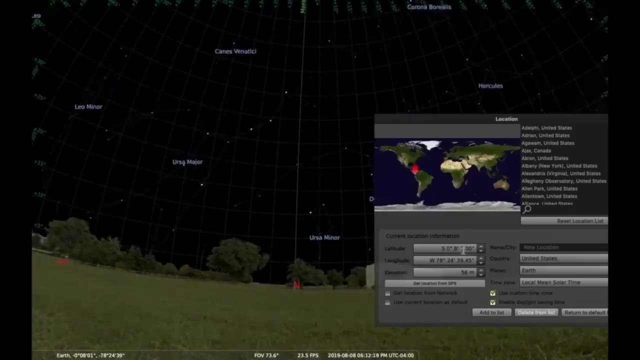 And so we keep going lower and lower and lower And watch what happens. That's interesting. So let's descend, descend, descend, descend, descend, descend until we get to the equator. So now, if we're at the equator, we have another interesting thing. 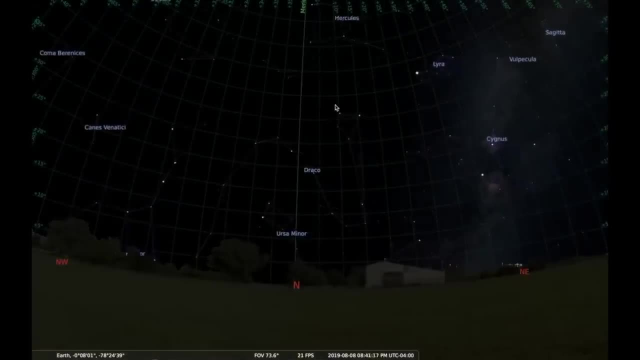 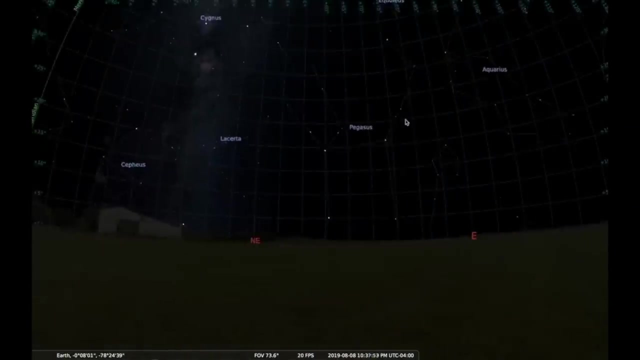 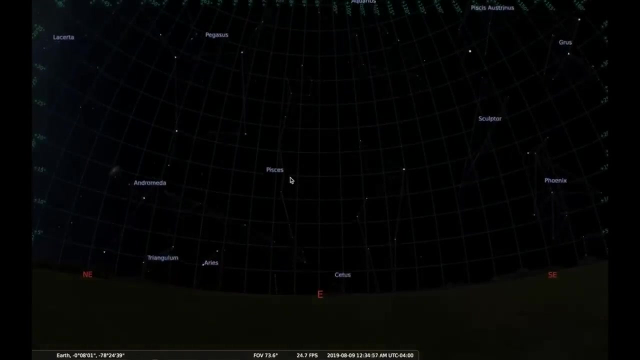 that occurs, Notice. the north celestial pole is on the horizon, The stars go straight overhead. But now we've got something very interesting. Let's look east, due east. Remember in New York City area how the stars rose at an angle to the horizon, But at the equator they rise straight up. 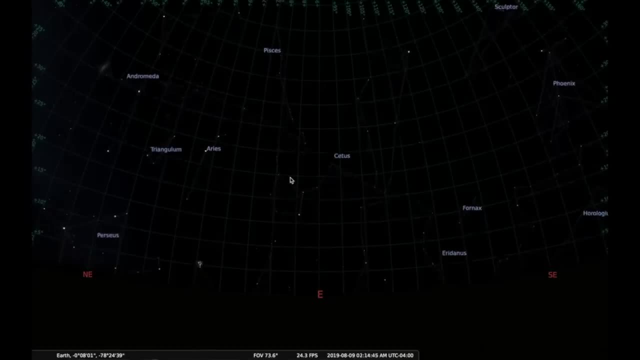 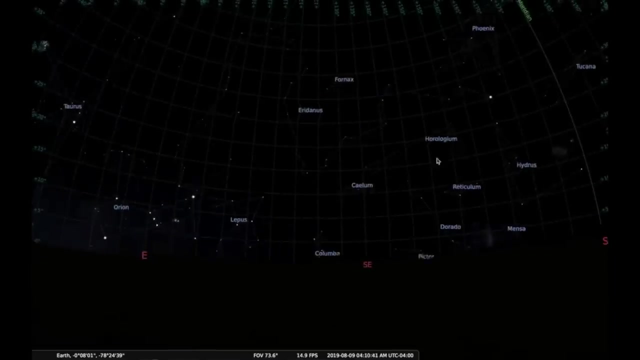 from the horizon. Everything, when it reaches the horizon, raises straight up. Isn't that interesting? So look at everything going straight up from the horizon. Now, as you go further and further south, when it rises off the horizon, that curve just goes immediately. 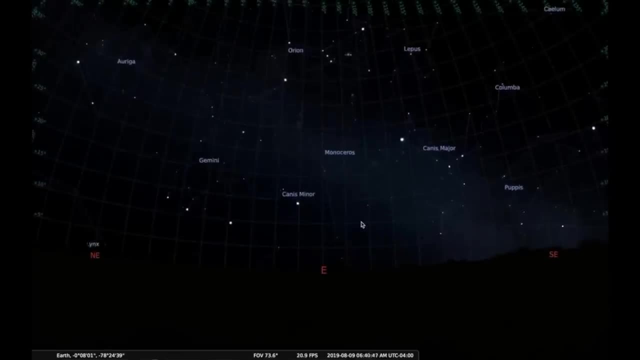 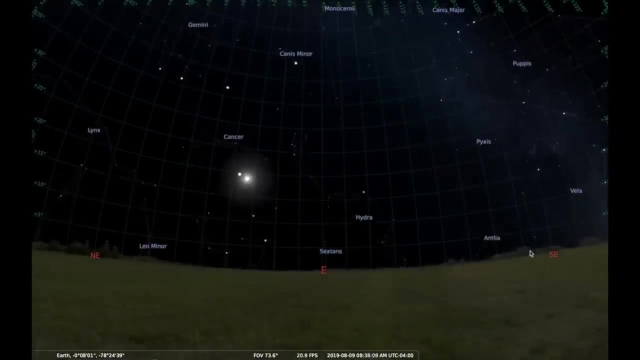 turns it, But if we're looking due east, due east, the stars rise directly up from the horizon. The angle that these things also do is the same, but if they're on the celestial equator they will not veer left or right. 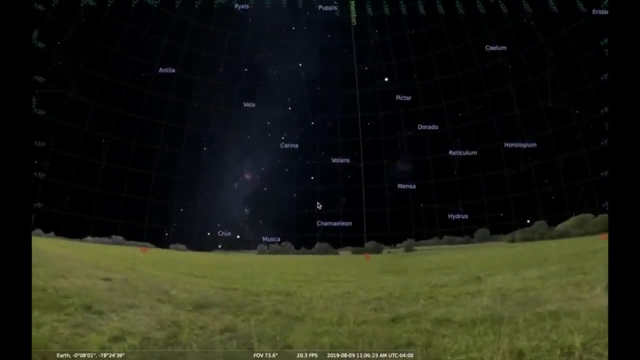 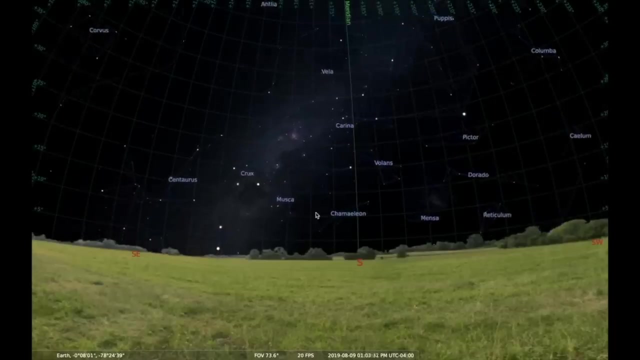 Notice. as we look further and further south now we see something interesting. There are constellations that you're probably not familiar with: Musca, Chameleon, Volans, Dorado, Mensa, Reticulum Crux. That's, the southern triangle Circinus. 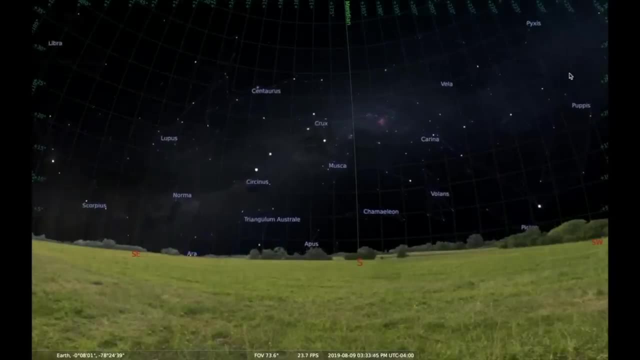 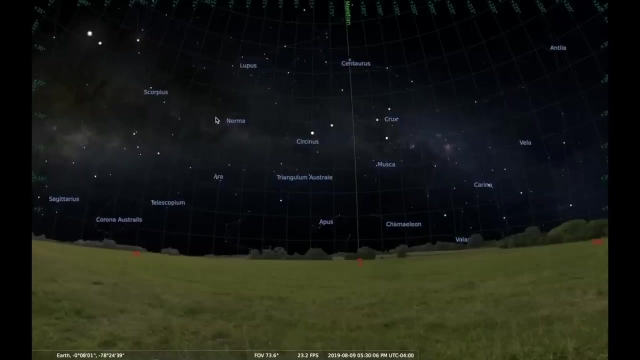 Lepus, you might know, Pupus you might know. But these are all stars. There's Scorpius there Now. Scorpius is interesting. It's very, very, very low in the horizon for us down in New York City, But when you're at the equator it can get very. 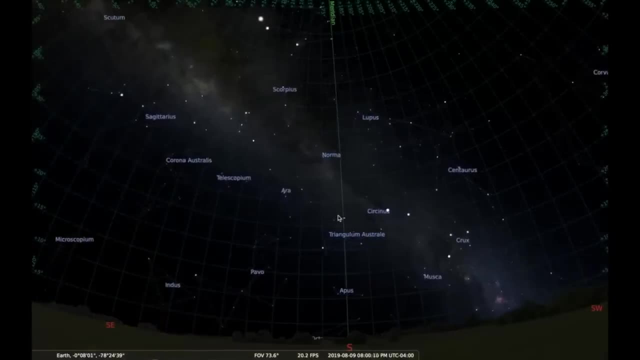 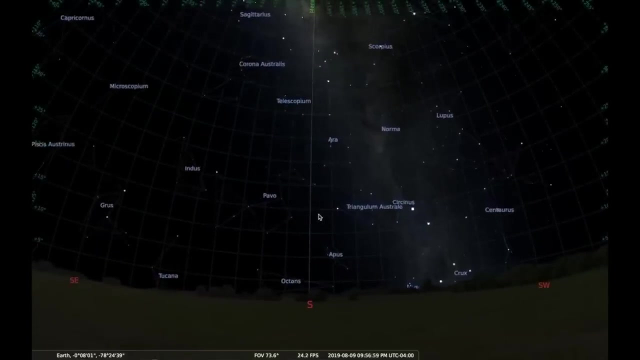 high off the horizon. Look how high that is. It's getting up to 60, 70 degrees off the horizon. So if you're on the equator, you get a good chance to see the things in the center of the Milky Way, which is really beautiful, Alright, so 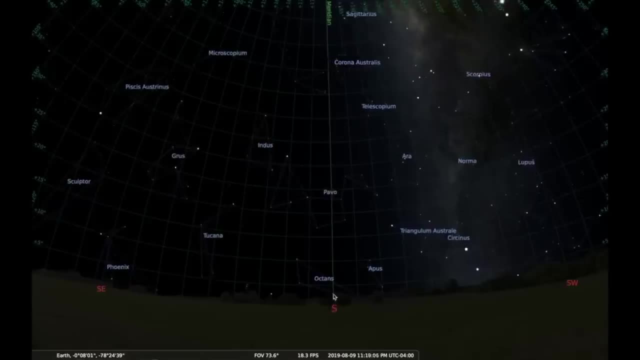 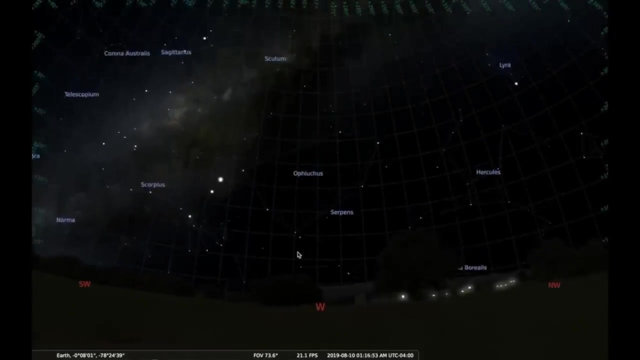 when you're looking south, we see that the south celestial pole, where everything seems to be rotating around, is there. and then we go look at the west and we see things again descending straight into the west. Now let's try a little game. We're going to look to the south this time and we're going to 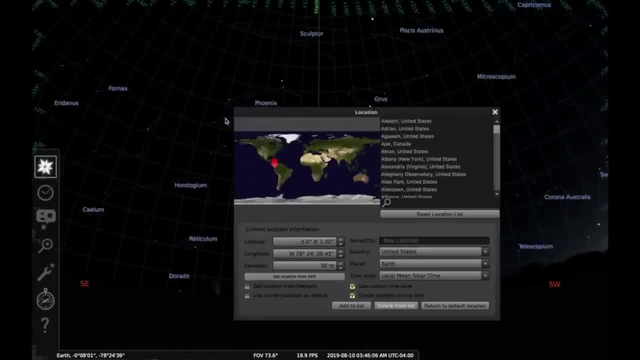 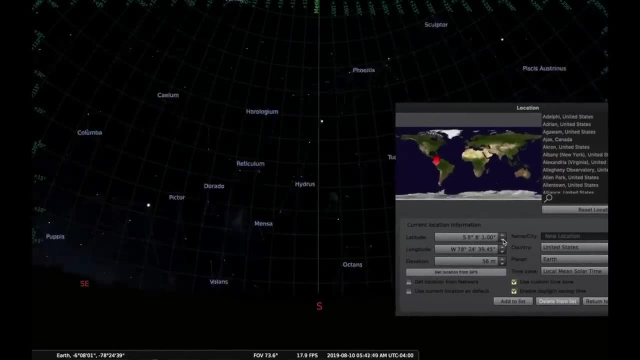 continue our walk on the Earth south. as I change the location of our direction, our location on Earth, I'm going to continue going south and notice what's happening. I'm going to keep going south and I'm going to stop in just like 30 degrees south. 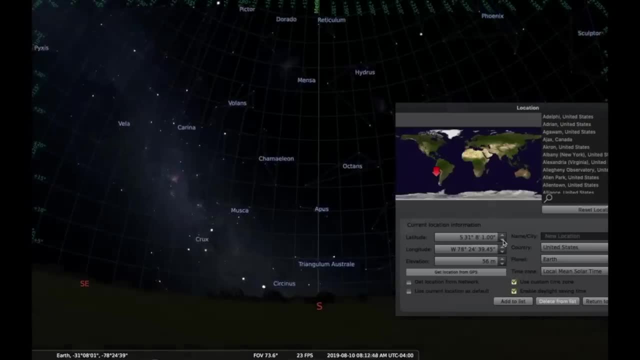 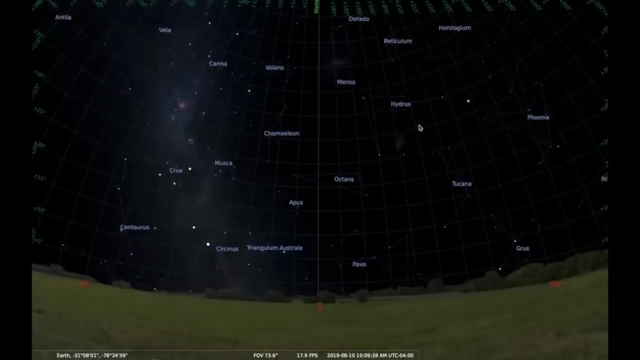 So now I've gone 31 degrees south. Interesting, That's like looking north from 30 degrees north, except now we're looking south. So let's see what's happened on the rest of the celestial sphere. We see this whole thing. 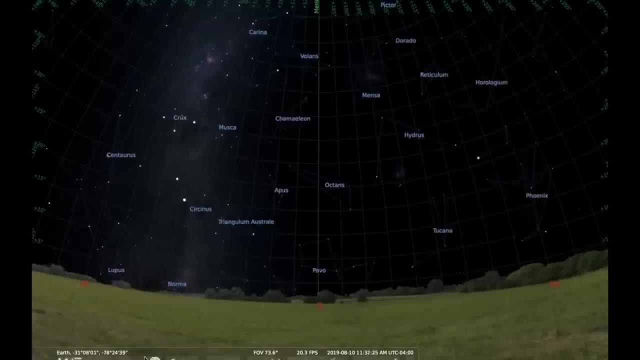 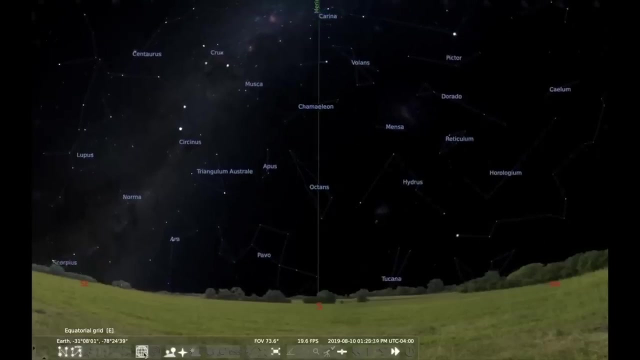 We now understand the nature of right ascension of the altitude in azimuth, showing how things rise and set and their altitude off the sky and their direction around the horizon. But I'm going to bring back the azimuth, the equatorial grid, Now. last time we looked at this from the 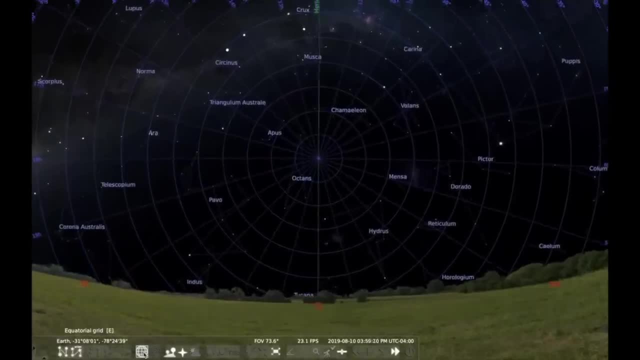 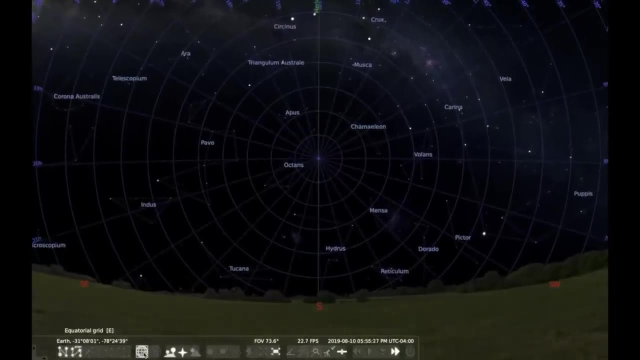 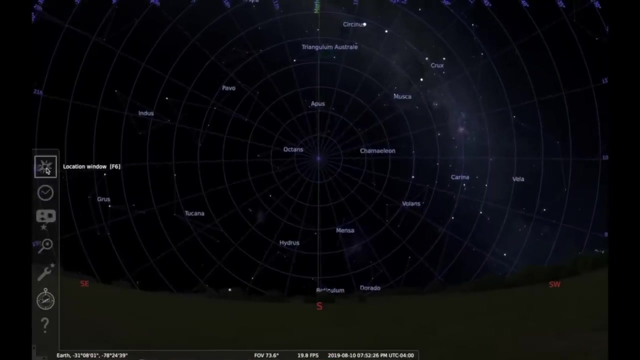 equatorial grid standpoint, we were looking north And we were looking to see the north star, But now we're looking south, So we're seeing the south celestial pole. The south celestial pole is the place that around which all stars in the southern hemisphere appear to rise and set. 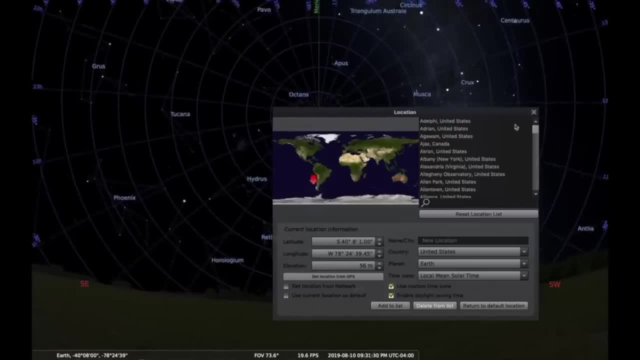 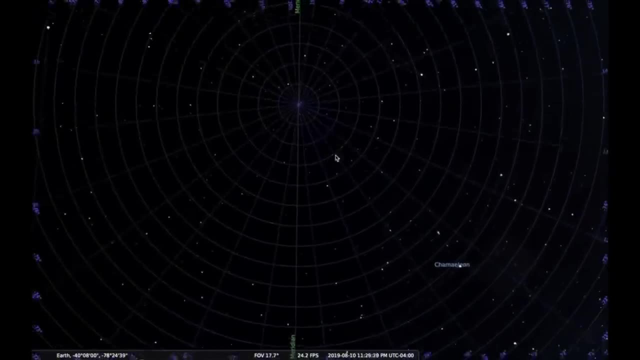 So I'm going to go a little further south. Let's go to 40 degrees south just to help have a little bit of fun. But the problem is that there really isn't a north star of the south. There really isn't, I mean there. 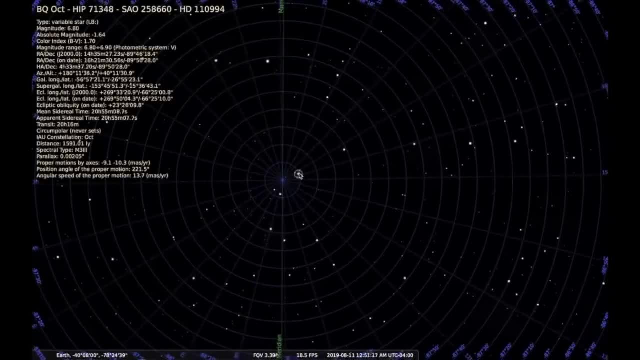 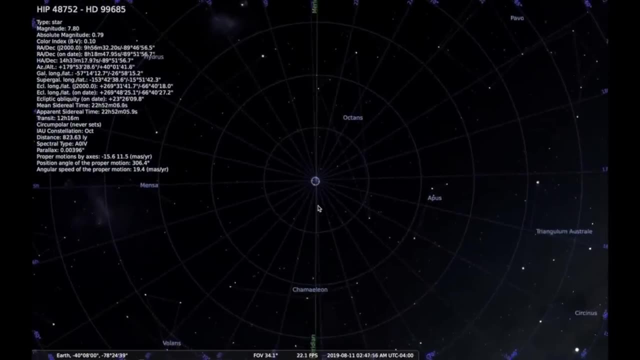 are stars, of course, that are nearby, but they're very, very faint. This is a very faint star of magnitude 7.. That's a magnitude 8 star. There are really no truly bright stars that are close to the south celestial pole, So what people do instead is that they use 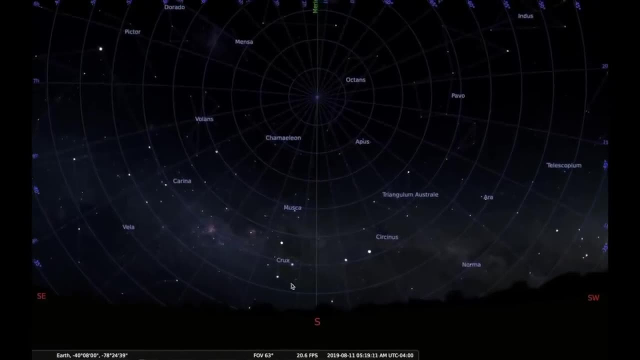 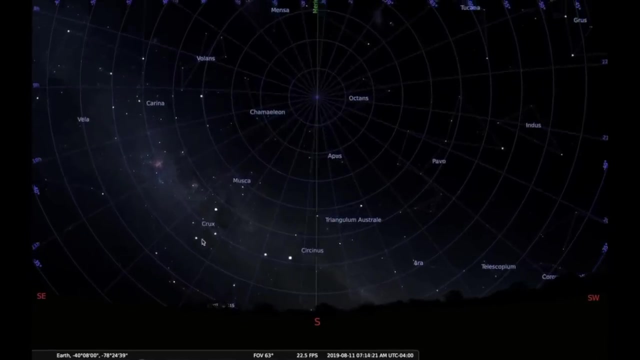 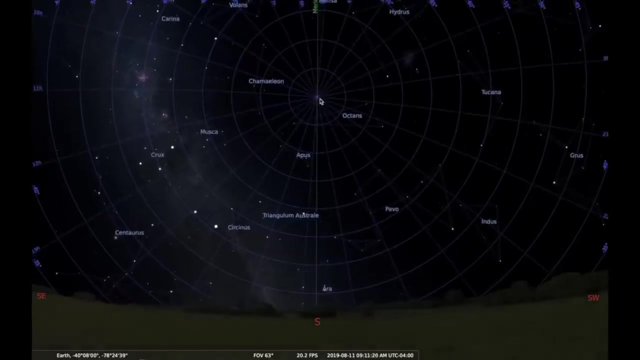 in the southern pole. they use the constellation crux or the southern cross to point at the south celestial pole. So all you have to know is the angle between these stars and the south celestial pole and know how far off you've got to kind of joggy it to get there Because it's not pointing directly at it. 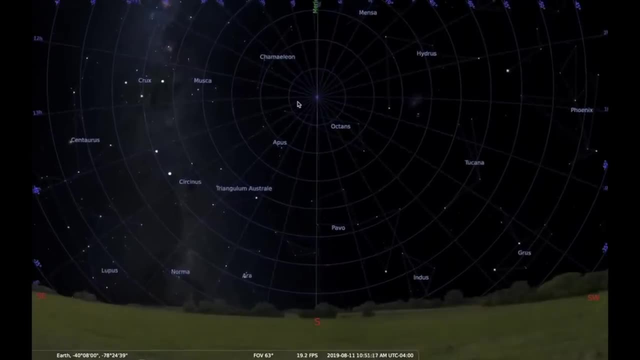 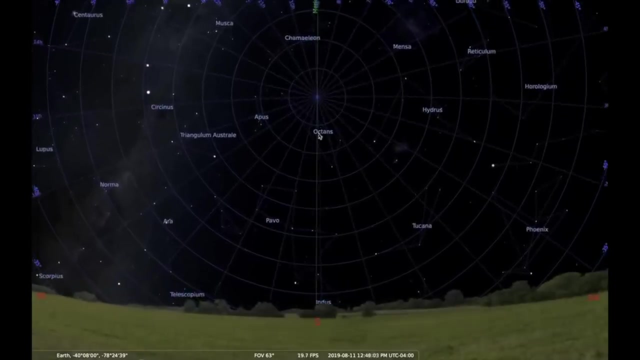 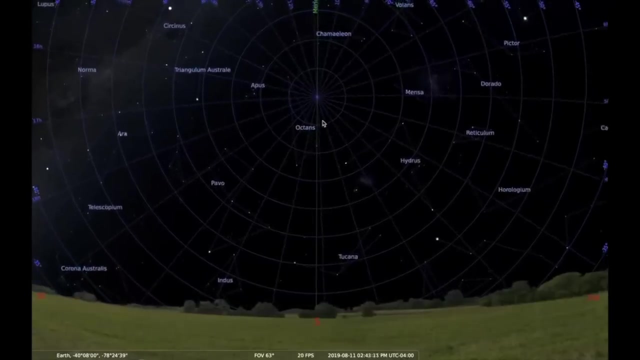 is it? You can see that that's pretty clear. But the southern cross points roughly at the south celestial pole, and so that can give you your latitude. In fact, your latitude is the altitude of the south celestial pole or the north celestial pole off of the horizon, If it's the south celestial. 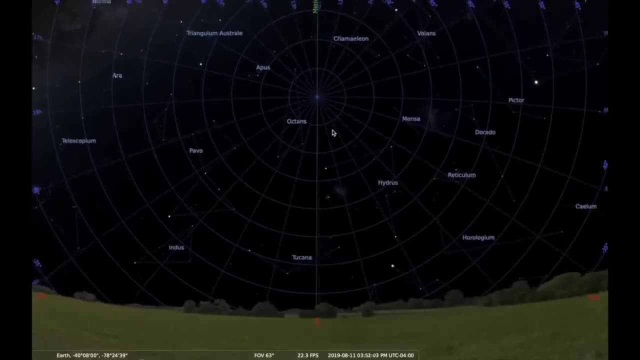 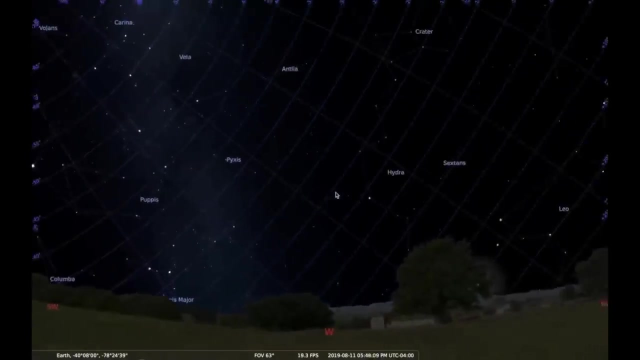 pole that you're looking at, then you have a negative latitude or a latitude below the equator. If it's north, then it's the other way. So now let's go look to see what happens when stars set in the west. This is different. 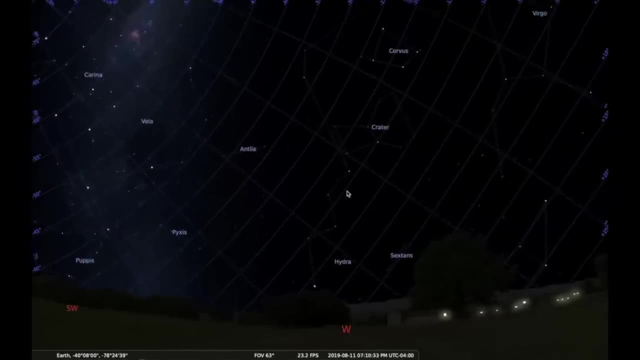 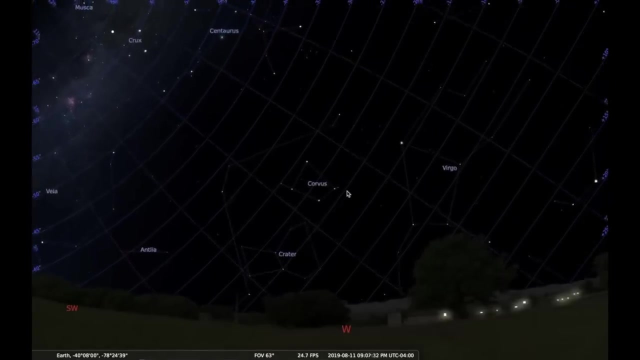 The stars when they set in the west and the south, say in Australia or South America or Southern Africa. notice how the stars appear to set from the right. The angle that they make to the west is originating from the upper, right to your upper. 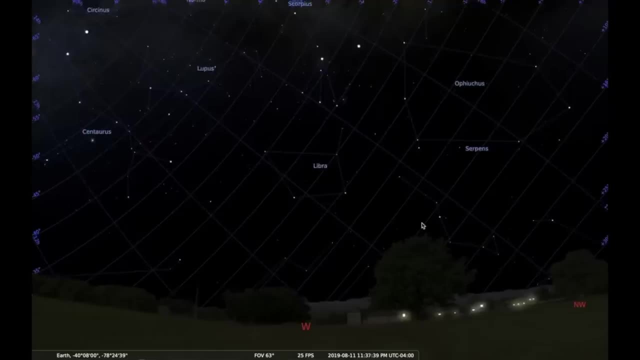 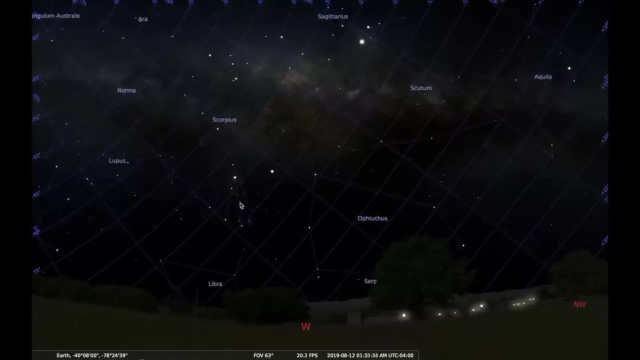 right and then they go down to the lower left. So the stars themselves are kind of seen backwards in how they rise and set, And some familiar constellations are upside down, like Scorpius and Sagittarius and Aquila and Australis. They're all these. 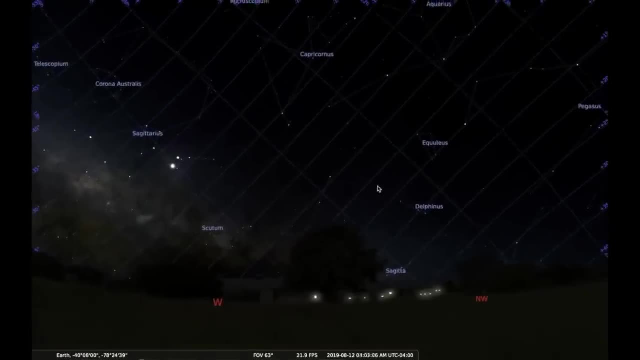 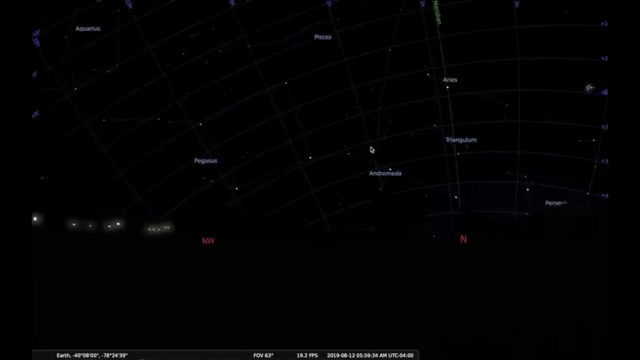 constellations that we're very familiar with that are now apparently upside down, according to Northern Hemisphere observers. Well, let's look for the north star. If we look for the north star, we're going to be out of luck, Because the north star is below the horizon and we 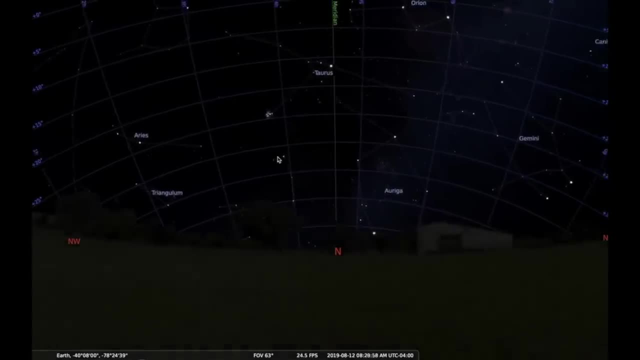 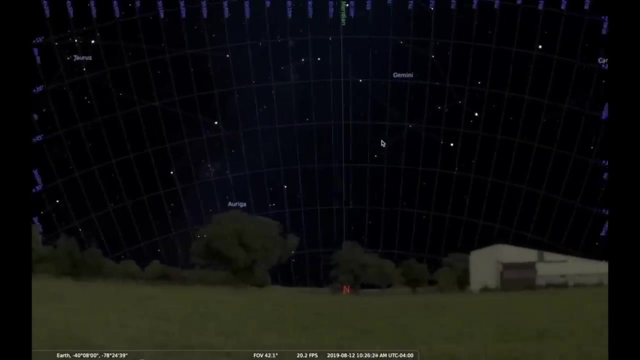 can't even see the North Ursa Minor, the Little Dipper, And even still weirder, there's Orion, which is now upside down, according to a Northern observer. There's Gemini that's going there, Taurus the bull, and the Sun is, of course, moving across. 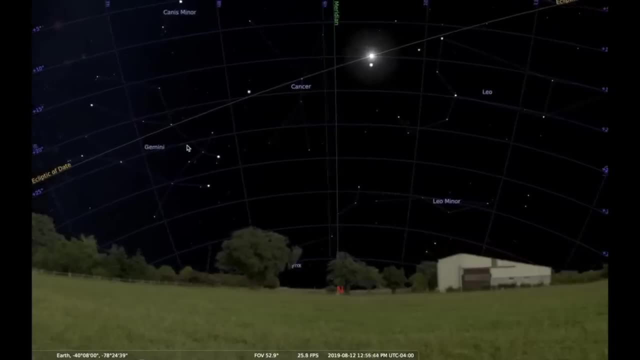 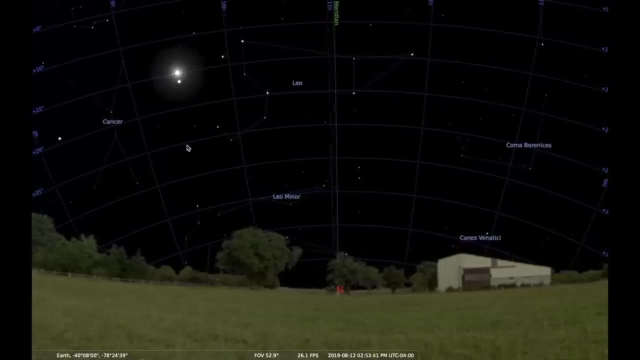 So I think we can bring back the ecliptic just for enjoyment. There's the Sun passing along the ecliptic And the ecliptic itself is fixed with respect to the stars. but we'll turn that off for now. Actually it's. 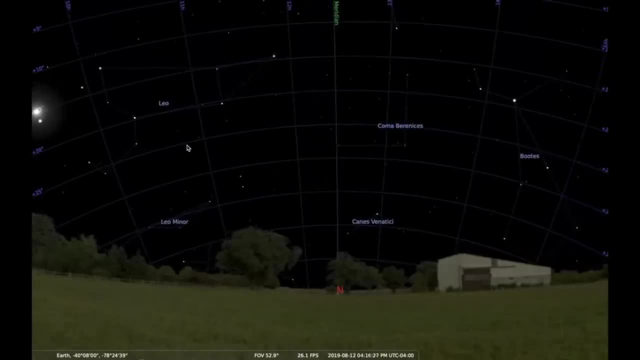 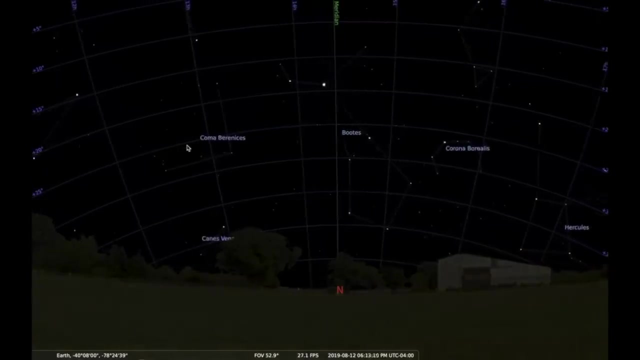 yes, So we have Leo the lion upside down, according to a Northern observer, but that's just fine. But notice, we cannot see the north star. There are no circumpolar stars to the north for Southern Hemisphere observers, But there are circumpolar stars. 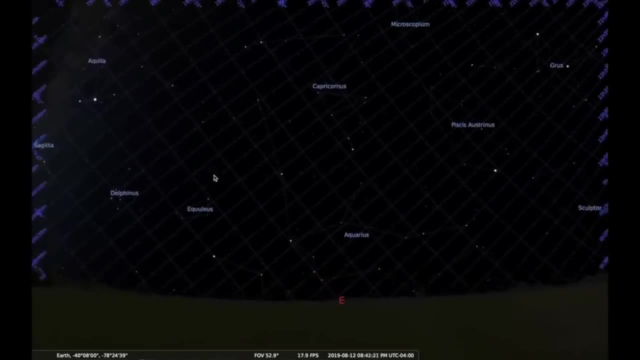 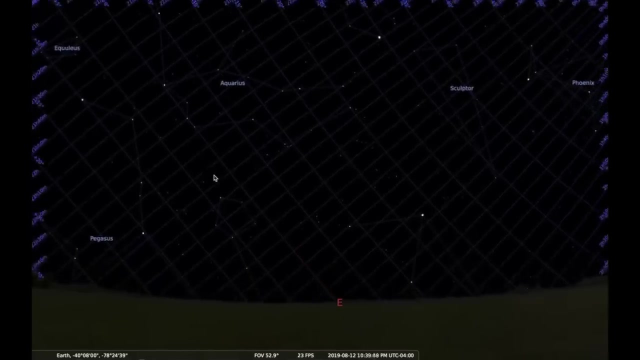 to the south for Southern Hemisphere observers And notice stars in the Southern Hemisphere. they rise in the east but they go in the upper right. So your latitude is of course, the altitude of the Southern Celestial Pole, and that's the whatever latitude this is. 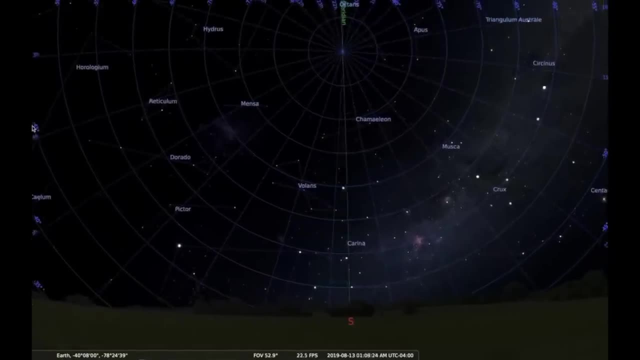 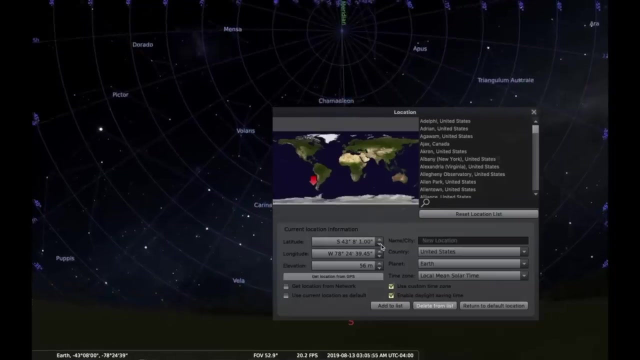 that would be about 40 degrees off the horizon. Again, if we wanted to play the game and go all the way to the South Pole, we can do that, And if we do, we have to go all the way down. dun, dun, dun, dun, dun, dun dun. let's keep going. 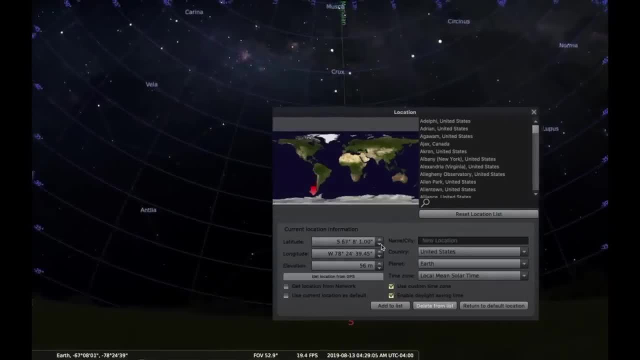 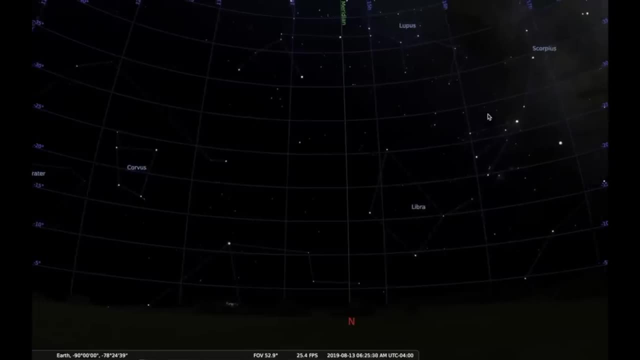 all the way down to the South Pole. let's go all the way down. let's see how fast it takes. I keep clicking until at 81,, 82, and then we're at the South Pole, Again at the South Pole. nothing rises or sets. so if you're down there in the winter and the Sun is below the horizon, you have 24 hours of night for 6 months. So the Sun never rises for 6 months. The day is 6 months long at the South Pole. 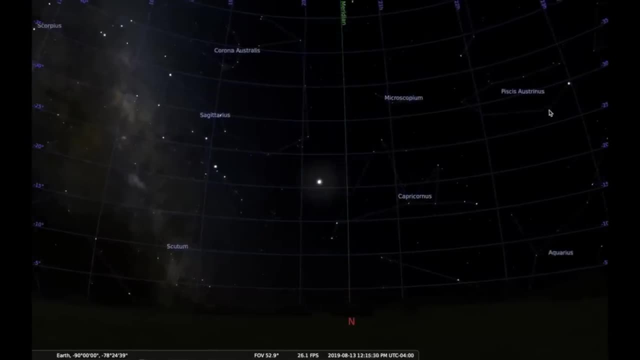 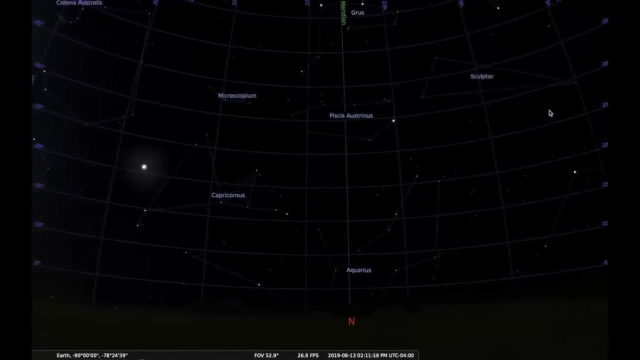 The night is 6 months long at the South Pole, The same with the North Pole, which is really fascinating. Either it's day or it's night there, and there's no rising or setting of the Sun. Alright, let's take it back to our normal. 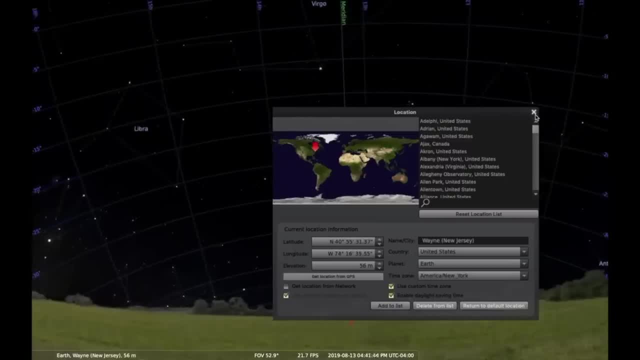 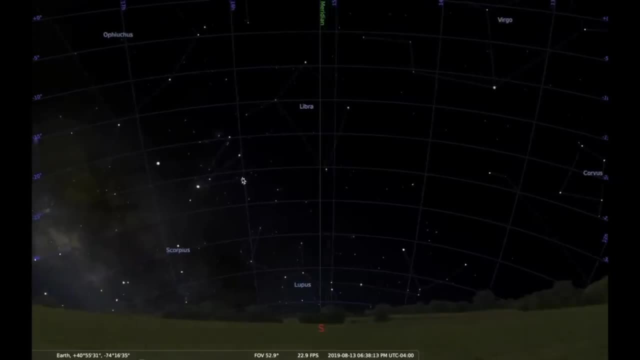 location and bring it back to our default location, which is in North America, roughly New Jersey, And if we look South we don't see the South Celestial Pole and there's Scorpius, back in its normal place for us New Yorkers and New Jerseyers, And we go. 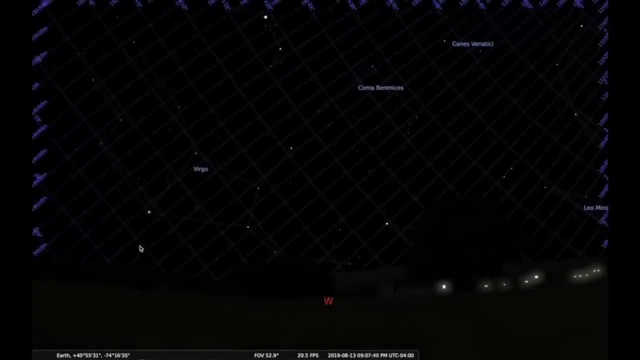 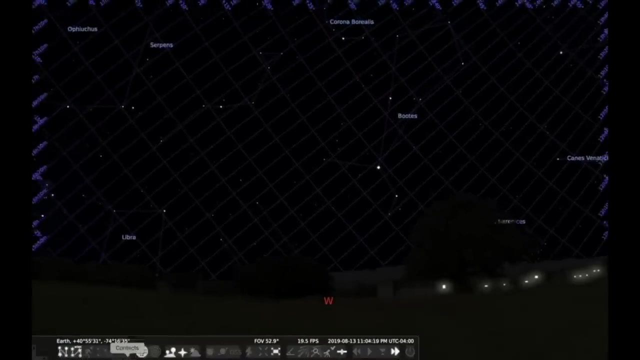 we look to the West, we see it kind of setting in the way we expect it. So then we go back over here and there are a number of things that we can chat about again. but the most important thing is, as we look out into the night sky, we see that this thing called the Celestial 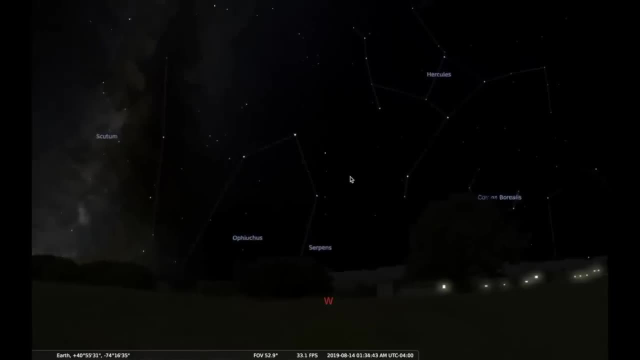 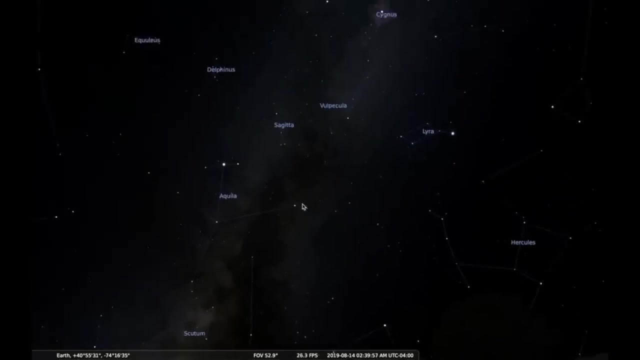 Sphere exists. And so what do we do with that Celestial Sphere? Well, first let's turn the time to a normal, and now I'm going to go all the way over here and I'm going to say: we'll look at the constellation Lyra. 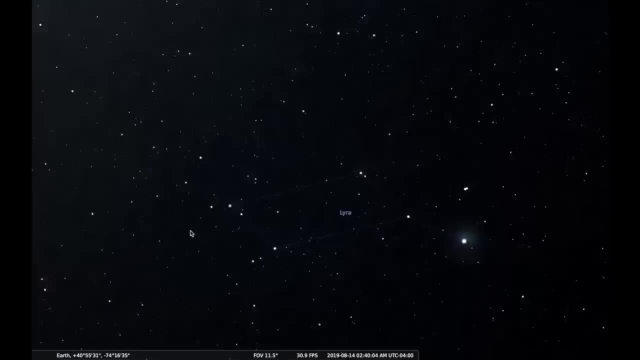 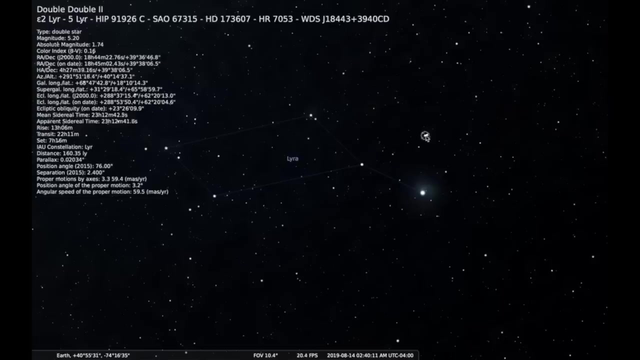 Lyra the Liar And I'm going to zoom in on constellation Lyra and I'm going to go all the way over to a famous double star which is Epsilon Lyra, the double-double Epsilon Lyra, And if we look closely at its coordinates, we see R? A. 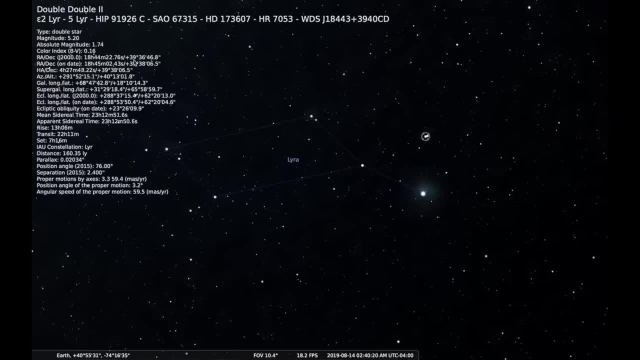 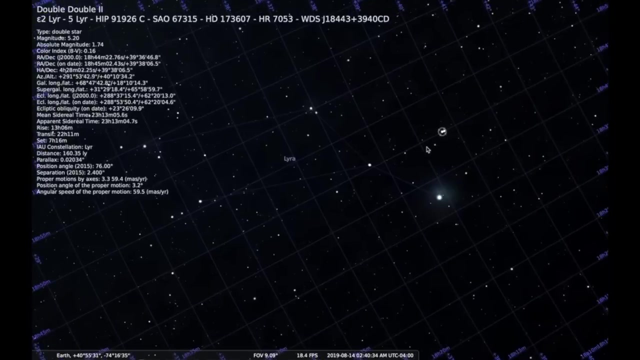 and 18 hours 44 minutes and a declination of plus 39 degrees 36 minutes. But why does that matter? Because if we go back and turn on our equatorial coordinate system again, we see that that is the exact coordinates of Epsilon Lyra. 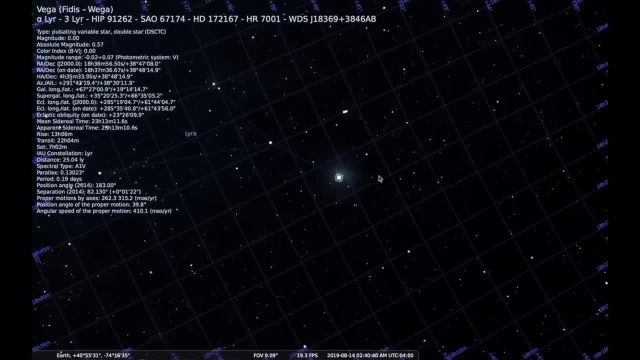 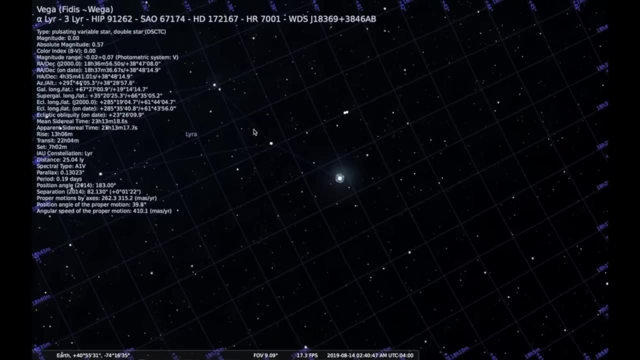 or let's just stick with Vega, because Vega is easy to find. Vega is one of the brightest stars in the sky, So Vega is a very, very bright star with a right ascension of 18 hours and 36 minutes and 56 seconds. 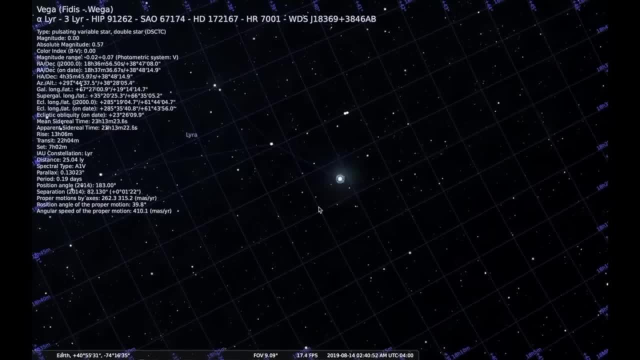 So 18 hours and 36 minutes means this is the line for 18 hours and 35 minutes. There's the hour and there's 18 hours and 36.. And then what's the declination? The declination goes up this way until we get to. 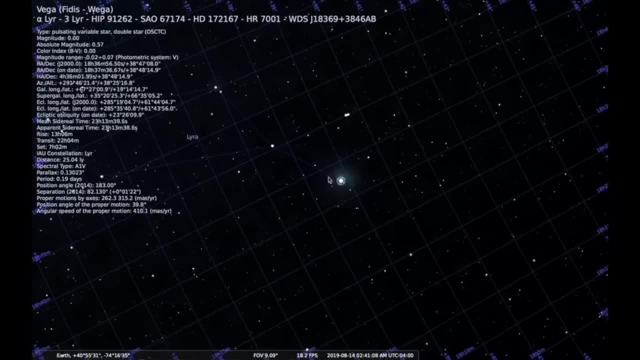 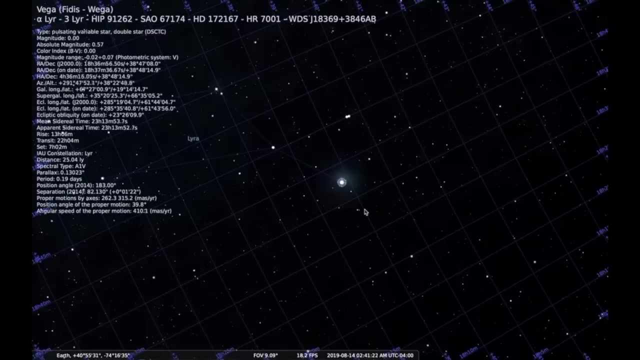 38 degrees. So here is declination 38 degrees, here's declination 39.. This is 38 degrees and 37 arc minutes. So because the coordinate system, the equatorial coordinate system, is fixed with respect to the stars, Vega's right ascension and declination. 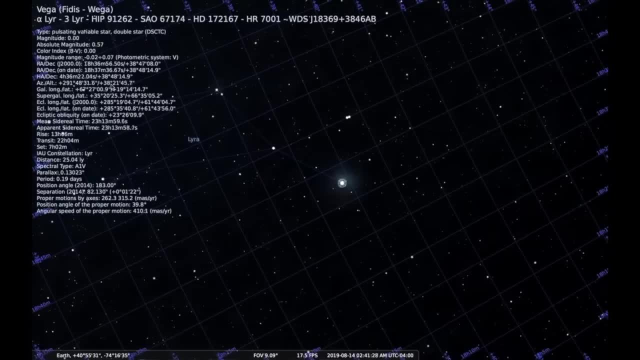 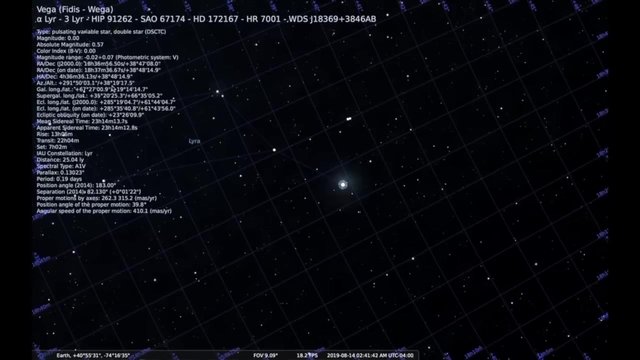 does not change, even as its altitude and azimuth change. Notice, the altitude is changing and the azimuth is changing. That's because, as the Earth rotates, the altitude and azimuth change. They must change because the height of the horizon is changing And accordingly, where it is along the sky, up from the horizon. 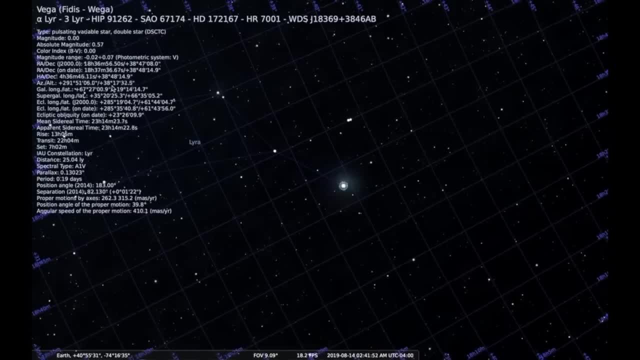 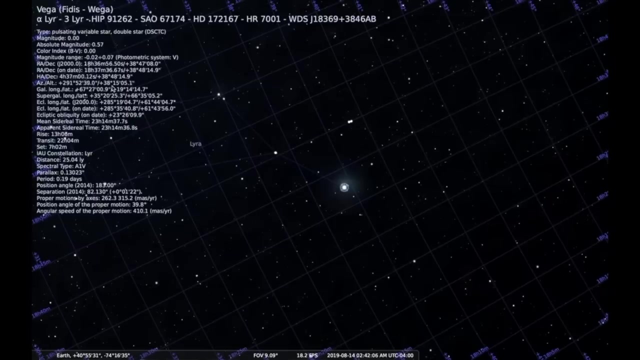 changes as well, But the right ascension and declination is fixed. So we have a longitude and latitude on the Earth and we can think of the celestial sphere, which is an imaginary sphere above us, covered with a coordinate system called the celestial equatorial coordinate system that is fixed with respect to. 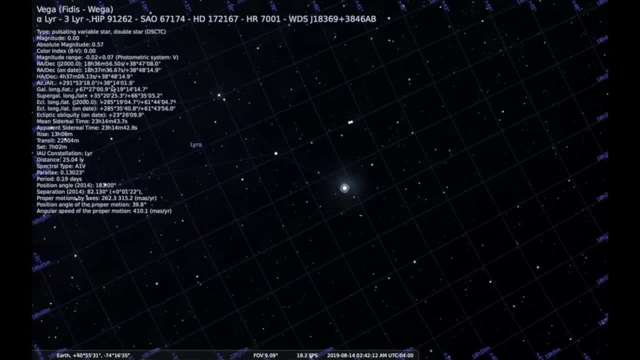 the stars And we can think of the stars as put on a big celestial sphere, which is of course imaginary. but that helps us to do a coordinate system And that tells us where things are in the sky, So we can use altitude and azimuth. That's very helpful for observers on the ground. 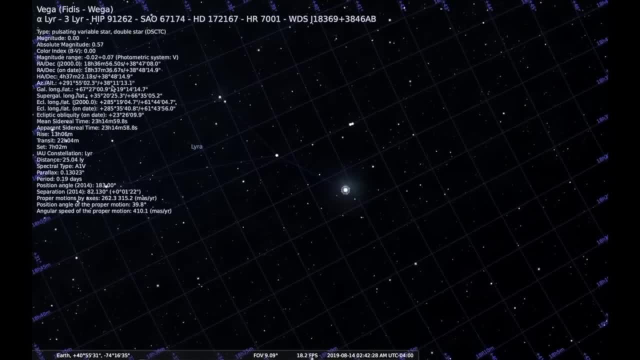 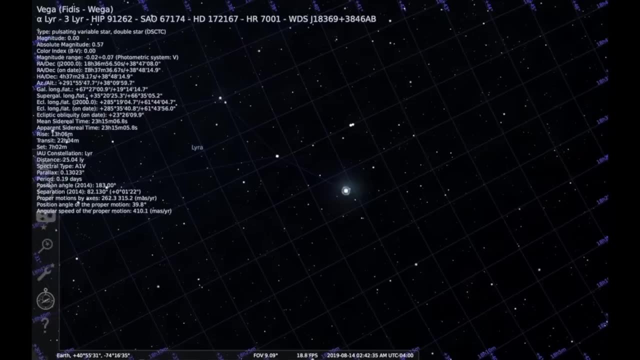 But the right ascension and declination is really good if you want to know really where something is and you want to tell somebody where it is also. Be that as it may, let's actually change it. Let's show you what I mean. 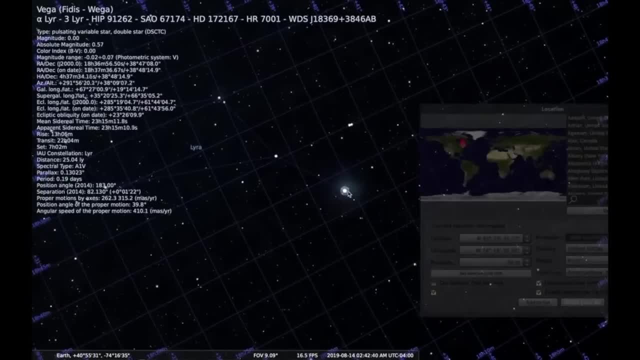 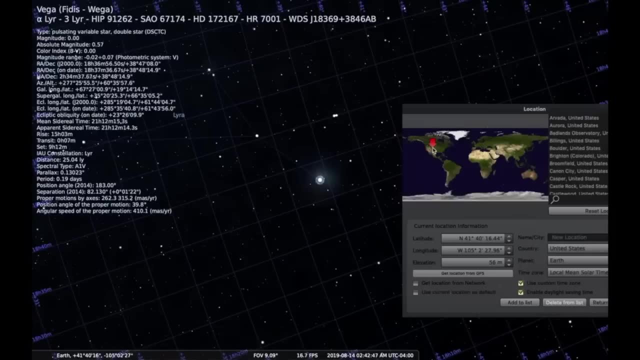 So now I'm going to change the location. I'm centered onto Vega and now I'm going to change my location to somewhere further west, Say out in Colorado. If we go out in the west, we see that it seems to have rotated, which seems like things have changed. 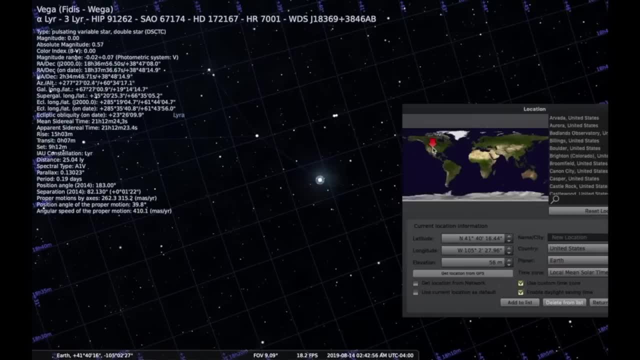 But notice that the altitude has changed and the azimuth has changed, but the right ascension and declination have not. So the altitude here and the azimuth here have changed and if I go to say Mexico, definitely the altitude has changed and the azimuth. 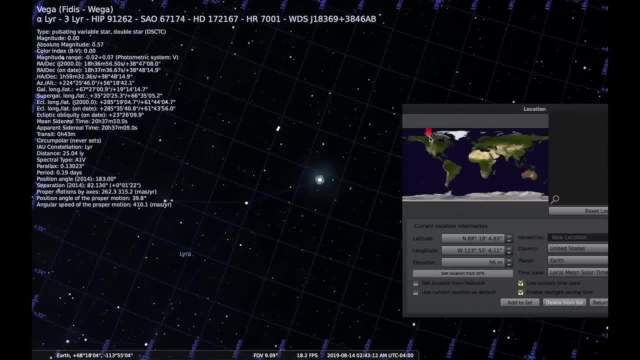 has changed. If I go up to Canada, the altitude has changed and the azimuth has changed, but the right ascension and declination have not. So that coordinate system- right ascension, declination and equatorial coordinate system- is perfect for telling people exactly where to look, because you don't necessarily know. 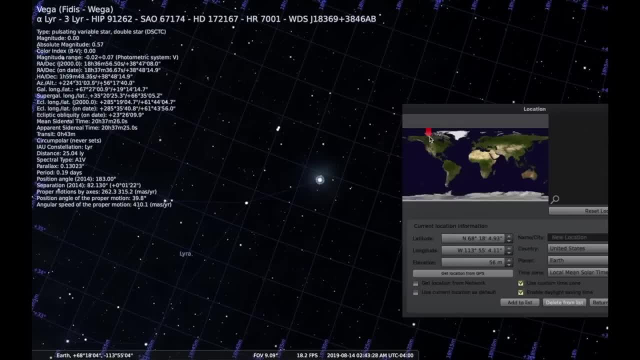 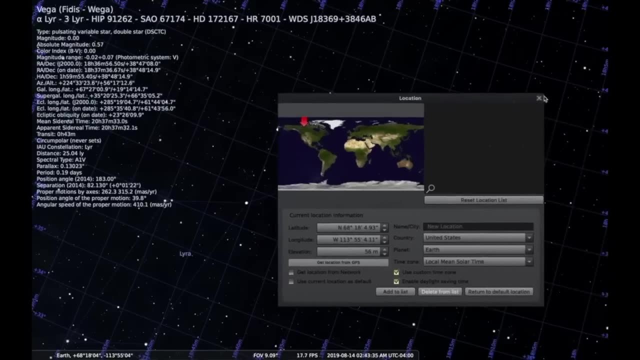 what somebody else's altitude and azimuth are for, say Vega. That actually helps us find where things are in the sky and that's their important things. So you would go out to a friend and say, well, look above the horizon and look for that bright star. 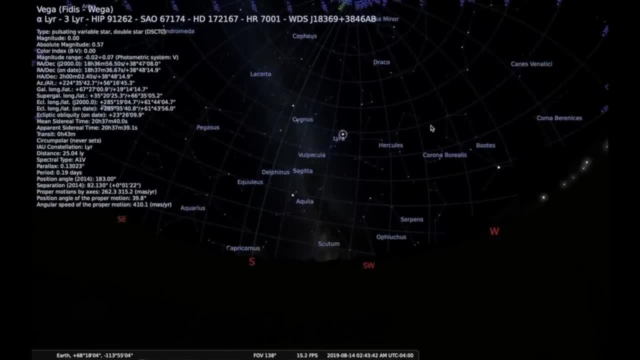 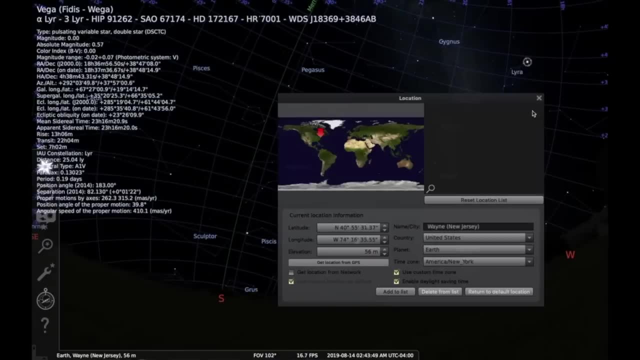 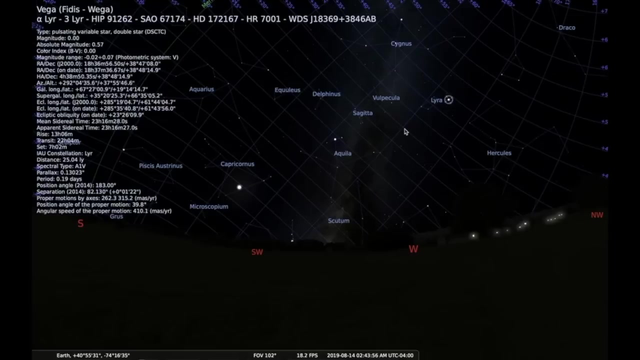 That's going to be kind of difficult because they might have it in a different location than you. In fact, look how different it is to go from northwestern Canada to New Jersey. It's radically different. So the place in the sky for Vega is very different for two people on Earth. 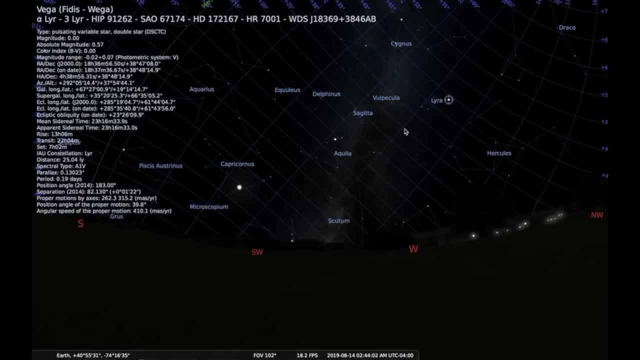 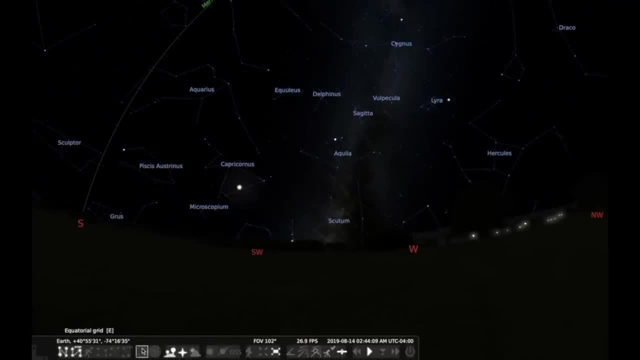 And that's because the Earth is a sphere, and because it's a sphere, different observers have different locations that they can look at. So this is an introduction to how we find things in the sky and what we're actually looking for when we go hunting around for stars in the sky. 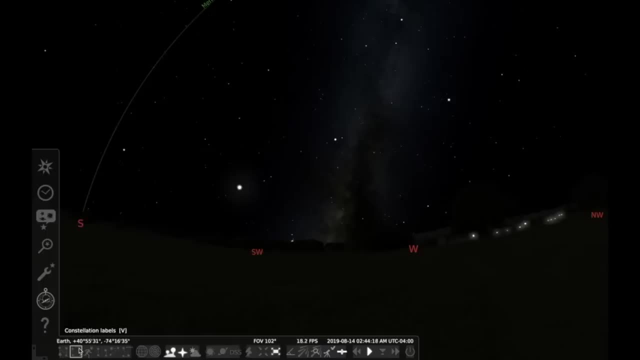 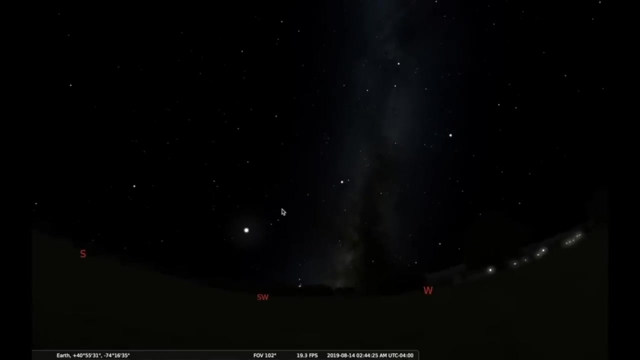 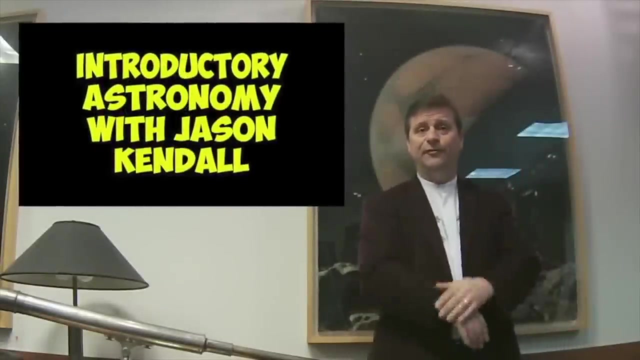 and we can see that the stars themselves are fixed with respect to a coordinate system that we call the equatorial coordinate system and that helps us navigate the sky on the celestial sphere. Hello, my name is Jason Kendall and welcome to our second lecture on astronomy, which is going to be a lot of fun. 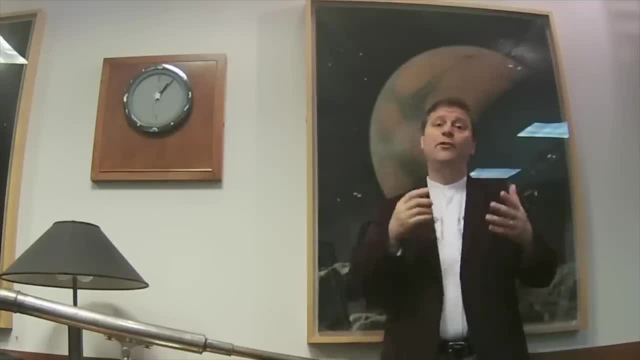 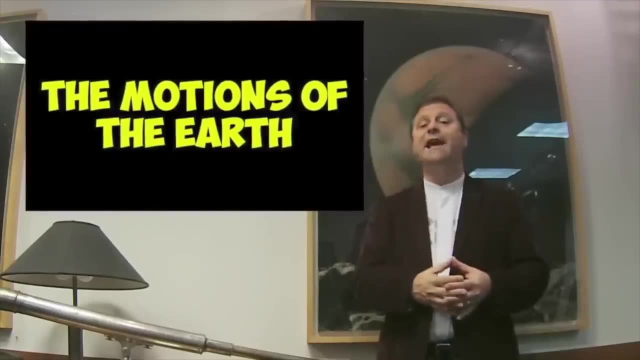 We've got lots of things to talk about. Well, today, what we're going to be talking about is the orbit of the Earth. The Earth's orbit around the Sun and the rotation on its axis are some of the most fundamental aspects of astronomy. It was one of the greatest puzzles of all time, and trying to understand the motions of 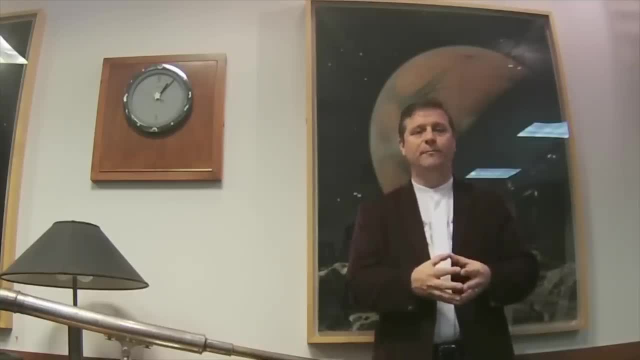 the stars with respect to the Earth has been a great puzzle for most of humanity, So I'm just going to go blow through it as though it's settled science, which it is. So the orbit of the Earth is effectively divided up into two basic pieces: The orbit of the Earth around the Sun and the rotation. of the Earth on its axis. We call the rotation on the Earth on its axis the solar day, and it takes 24 hours, by definition, for the Sun to come back to the same place in the sky, and that's what we call the solar day. And that's high noon. 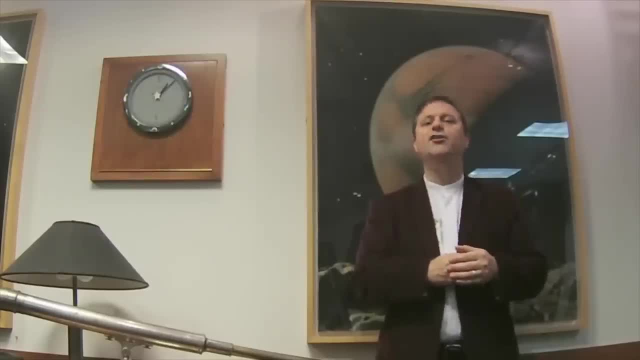 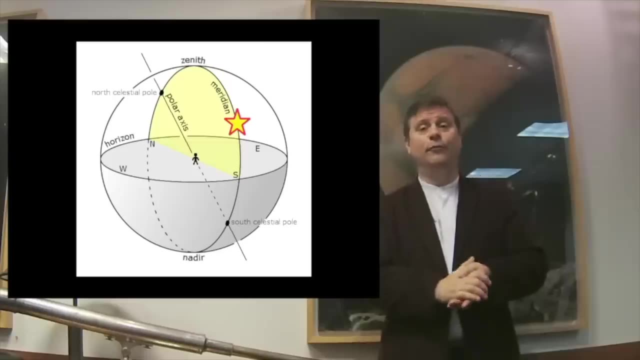 to high noon or midnight to midnight. typically we think of high noon because that's when the Sun, when we look due south, it's directly on what we call the meridian, And the meridian is an imaginary line that goes from due south to straight. 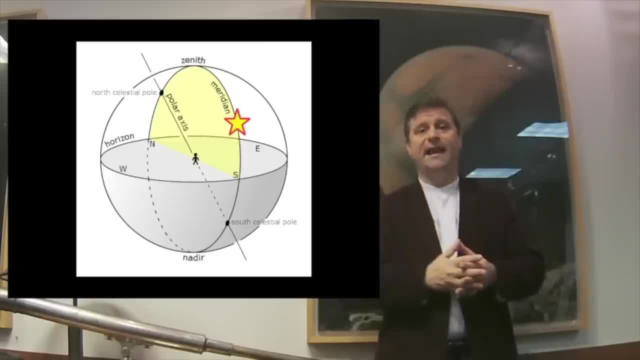 overhead of the zenith through due north, And so when the Sun passes- that typically at noon- we're a little bit off there because of the equation of time, which I won't get into, but that's pretty much the definition. When it gets back to 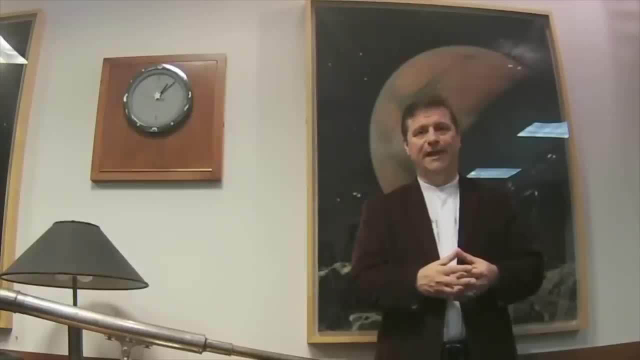 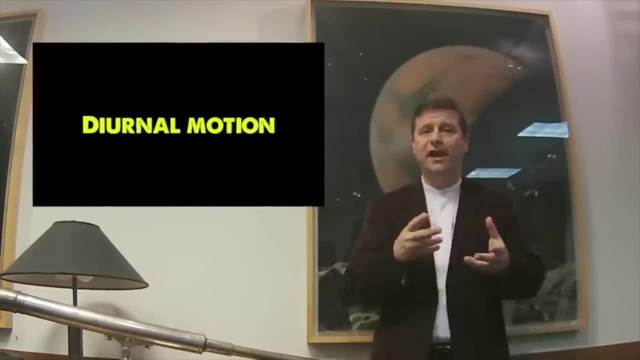 noon at that time. that is the definition of the solar day. Well, there's another thing that we can call this. it's the diurnal motion, and diurnal means two types of changes. So the diurnal motion of the rotation of the Earth on its axis produces 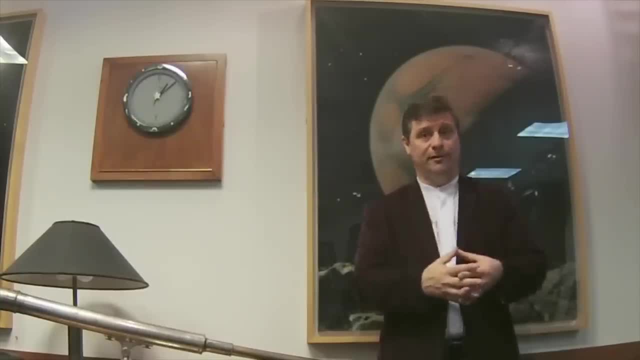 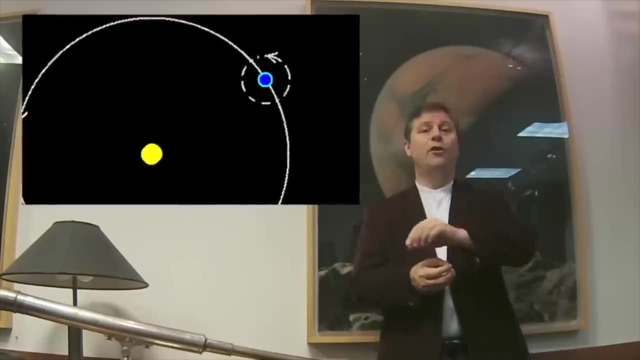 day and night. So there's two things: diurnal, that's what we call the diurnal motion. Well, as the Earth rotates on its axis, we also know that it goes around the Sun on its orbit. So if the Sun's here, 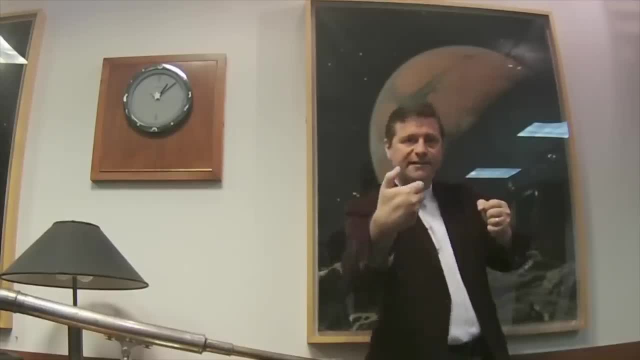 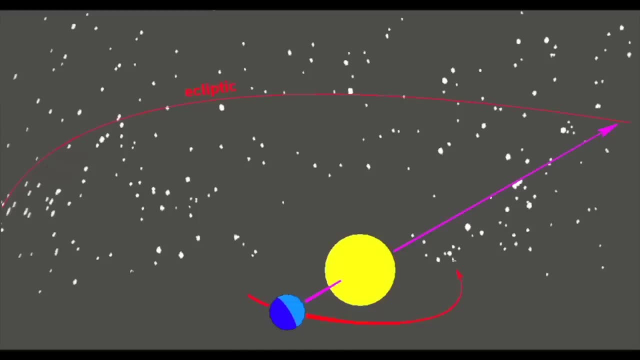 and the Earth is there as it goes around. here we have the Earth rotating on its axis as it goes, So the exact location of the Sun in the sky changes with time, And so what we'll find is that if we plotted the exact position of the Sun in the 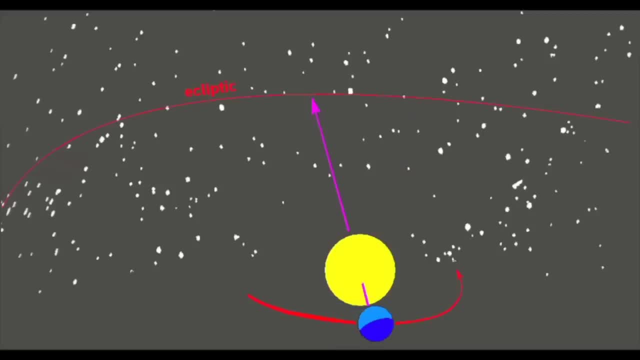 sky. with respect to all the background stars, we find that the Sun appears to be changing its position. Well, it's because, as the Earth goes around the Sun, the stars that are up at midnight are different ones, So the Sun is apparently in front of other stars. We can't see that, but we can infer. 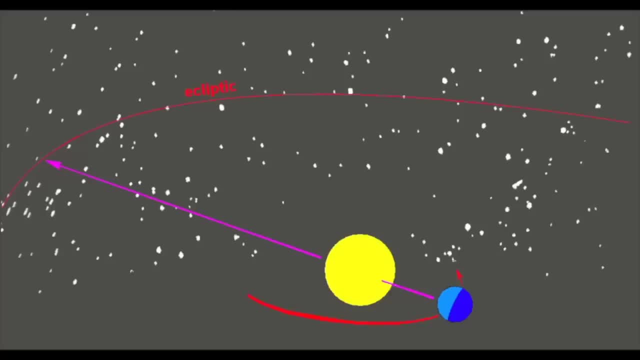 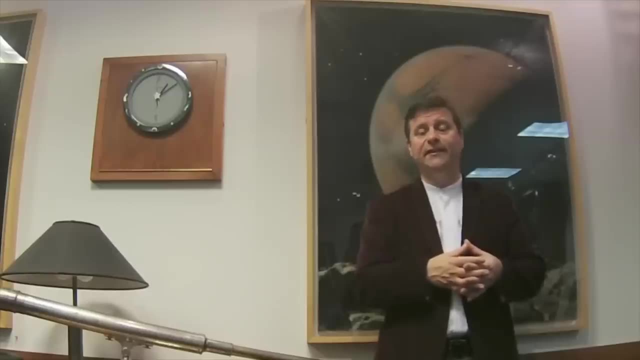 it because we know where the Sun rises and where the Sun sets and we can see the stars right before sunrise or the stars right after sunset and we can determine roughly in the sky where the Sun is And then we can establish that And what we call that path, that the Sun seems. 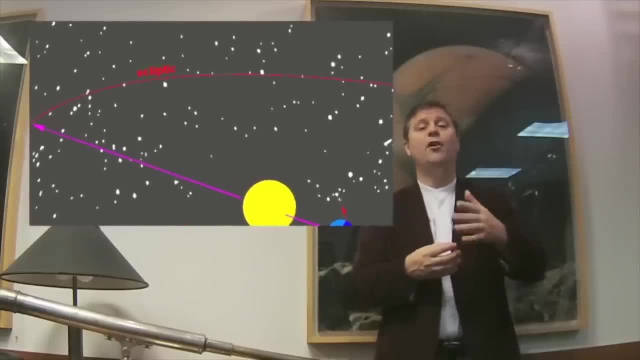 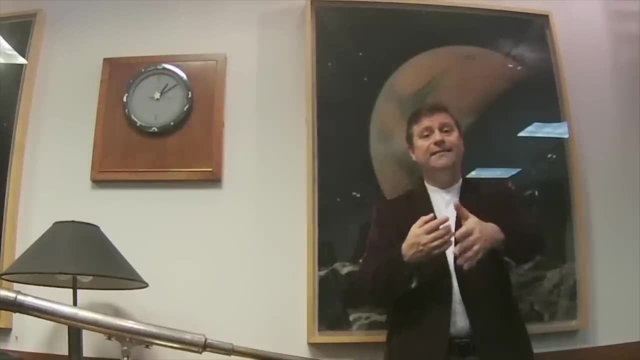 to make with respect to the background stars. we call that path the ecliptic, And so it's a definition of where the Sun goes in the sky. Well, as the Sun travels around the sky, this is an Earth-centered view. we can look at the Earth-Sun. 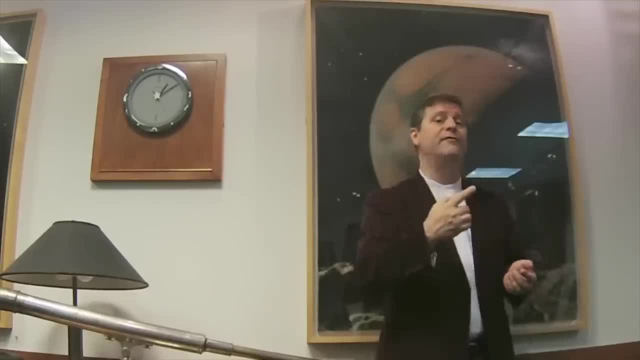 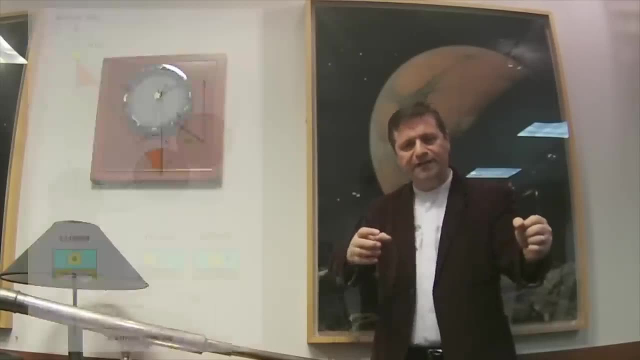 traveling around the sky or, equivalently, as the Earth travels around the Sun. we find that as the Earth rotates on its axis, as the Earth moves, it rotates a little bit further. So there's two definitions of the day. There's the normal solar. 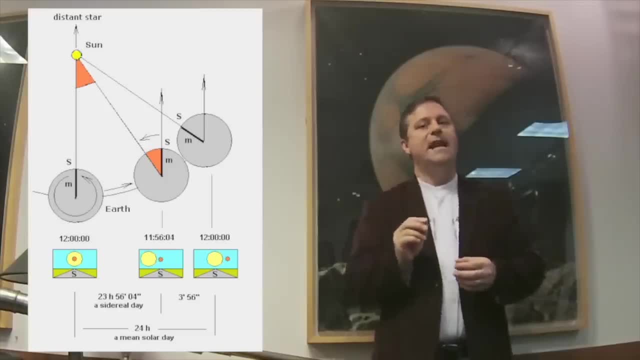 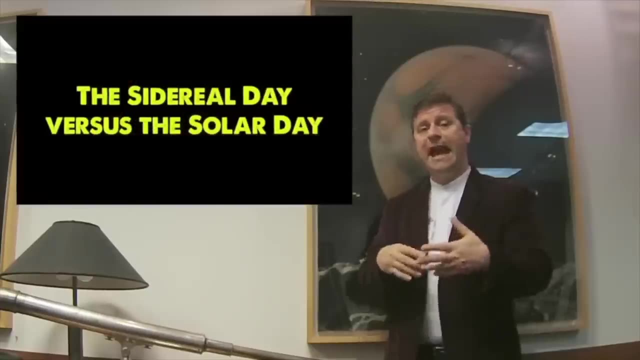 day, which is noon to noon, and then there's a different day, and we'll call that the sidereal day or the day with respect to the stars. So instead we look up at night and trace when a particular star crosses the meridian. we'll find that the sidereal day is actually shorter than the solar day. The sidereal day is 23 hours 56 minutes and about 4 seconds. So that means what's happened is: why does the solar day and the sidereal day differ? It's because the Earth moves a little bit. 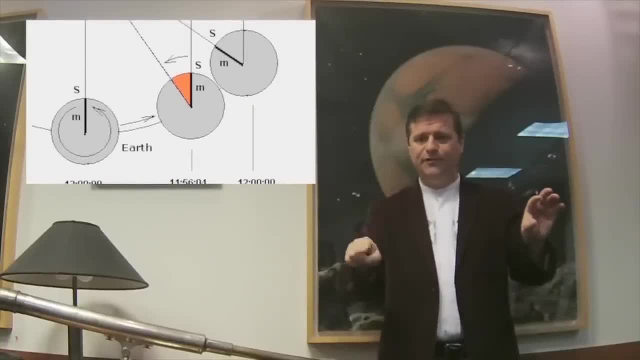 So if this is the solar day and this is the Sun and this is the Earth as it rotates around on its axis, it changes. So it'll change a little bit to here, and if we think of this as where the direction of the, 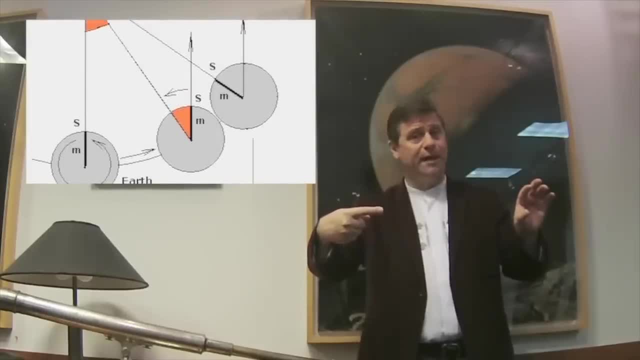 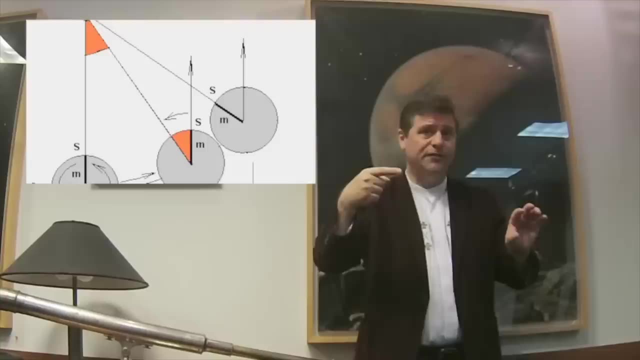 Sun is at 24 hours, 23 hours and 56 minutes later. the Earth has moved a little bit in its orbit, And so the stars that are in the background way over here- those stars- are in the same position, But now we've got to go a little bit further in order to get the Sun in the same. position in the sky. So therefore the sidereal day is shorter than the solar day by about 4 minutes. because the Sun goes around the sky roughly 1 degree a day, because there's 365 days in a year and 360 degrees in a circle, so it 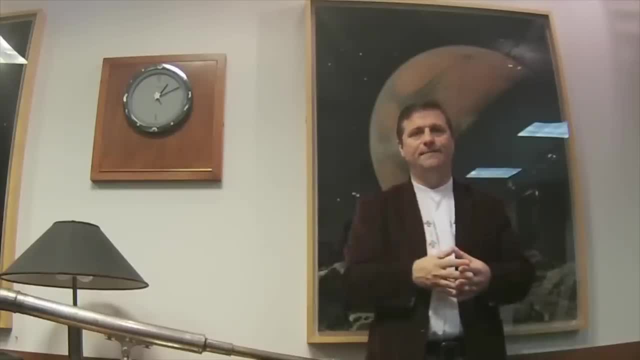 goes roughly 1 extra degree, so it has to move that degree Anyway. so those are our two definitions and they're kind of important to remember because if you want to watch things in the sky, there's two ways to do it. 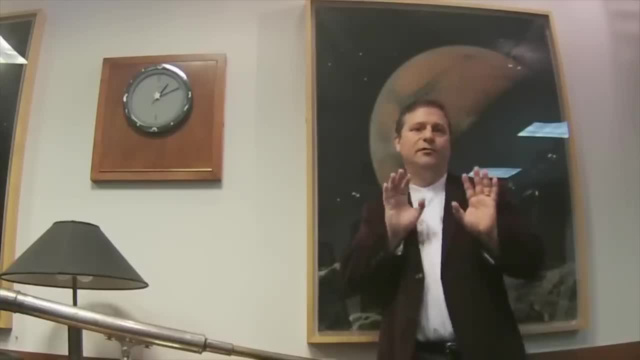 You can either wait for the Sun or, if you want to take pictures of things, you want to look at them in terms of their sidereal time, which is, when do they arise and set. Okay, so those are our two basic motions. as a result, 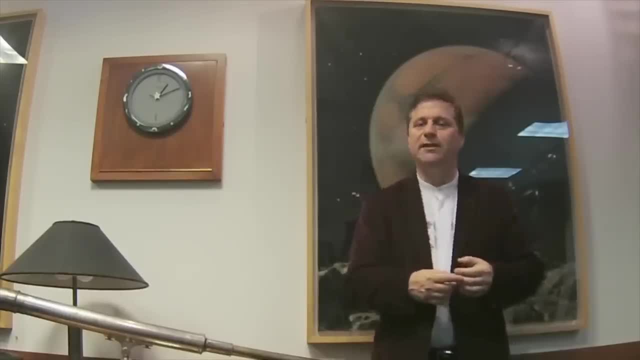 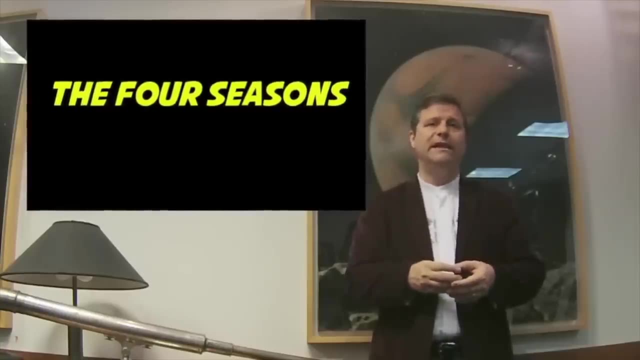 of the Earth going around the Sun. But there's this other thing that people keep talking about, which are the seasons. You know we have climate change, but seasonal changes are things that we see more frequently. So what are the reasons for the seasons? 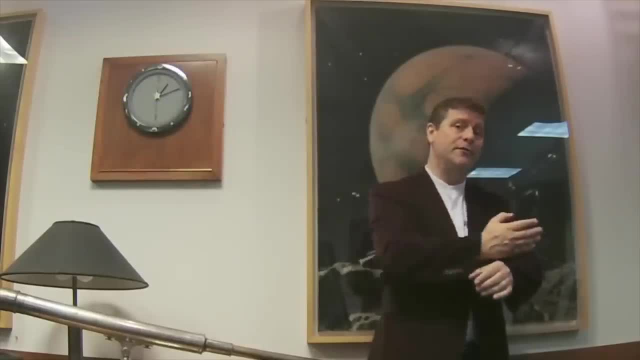 And as we watch the Sun go around the Earth, or more specifically, as the Earth goes around the Sun, we see some interesting effects. In the wintertime in the northern hemisphere, on Earth, the Sun appears low in the sky at noon. 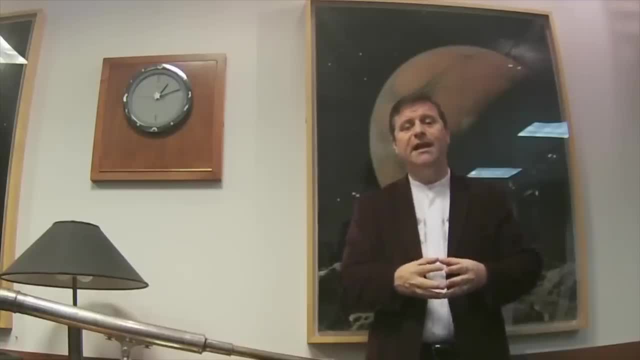 And in the summertime it appears high in the sky at noon. And that's because the Earth's rotation axis is not the same as its orbital axis. So once again we can think of the Earth going around the Sun like this. and so it makes like a disc, makes like a plane. 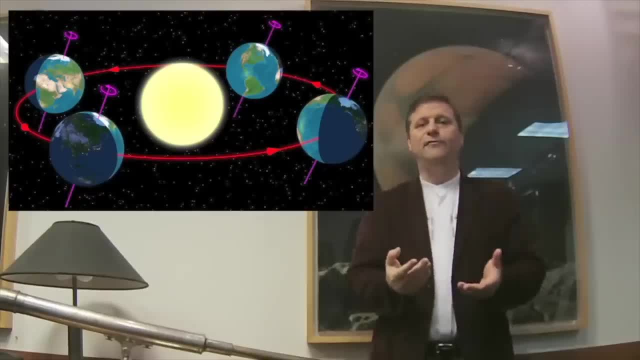 And we can make an arrow going out of it. Think of an old photograph or an old disc with a spindle going through it, and the spindle is the axis for the disc, Or even a top, if you will. So the disc of the plane of the Earth going around the Sun has an axis and then 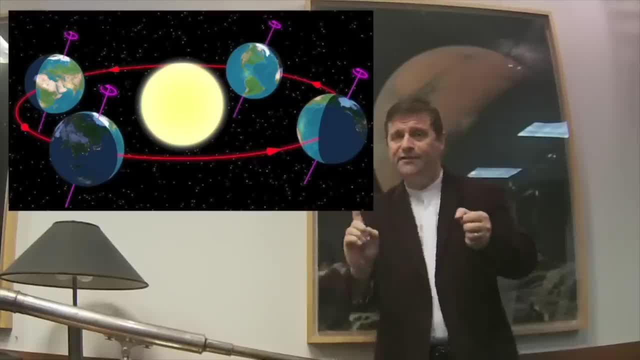 the rotation of the Earth's axis is tilted. So as the Earth goes around, here's the axis for the orbit. the axis for the tilt stays fixed, Just like a top. The top's orbital, the top's spinning axis always stays up. That's why a top doesn't fall down. So as you spin, 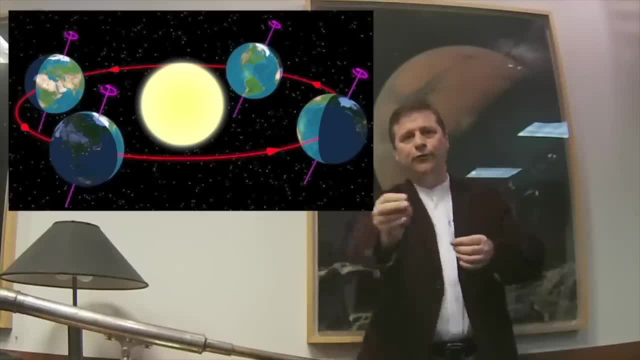 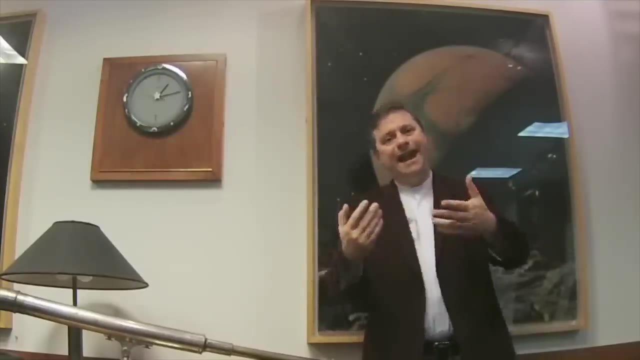 the top, it doesn't fall down. So as the Earth goes around the Sun, the orbit, this rotation axis, always stays pointed in the same direction, And then the width is different by 23.5 degrees from the orbital axis. So that is the beginning for the explanation for the reason. 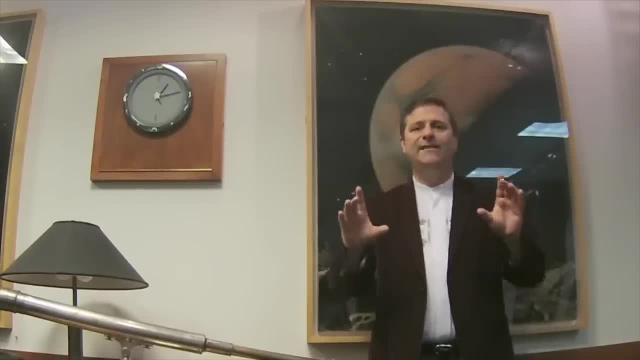 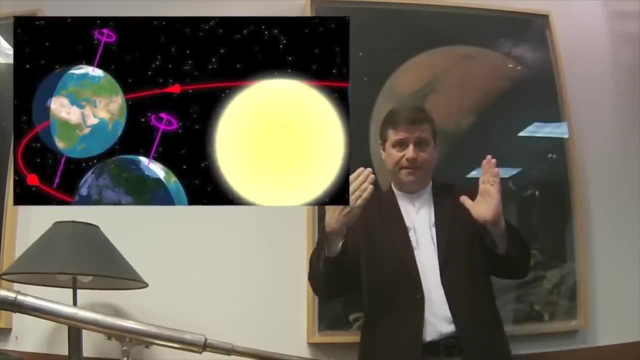 for the seasons, And really what we can think of is that at the times of summertime, if the Sun is here and the Earth is here, the Earth's axis is pointed towards the Sun. Now, in the wintertime, the Earth's axis is pointed away from the Sun. So what does that matter? That matters because in the summertime the Sun is high overhead and so the light from the Sun doesn't get spread out as much on the surface of the Earth in the Northern Hemisphere. But in the wintertime the same amount of sunlight. 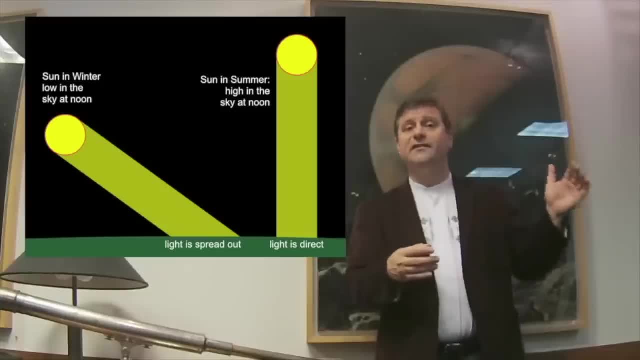 gets spread out over a larger area because the Sun is at a lower angle in the sky. So the Sun's light is spread out over a greater area. so it doesn't receive as much sunlight per square meter on the surface of the Earth. So therefore in the wintertime it's. cooler And in the summertime it's warmer because the solar radiation all of it falls onto a smaller area, So the per unit area, So it doesn't get spread out as much. If it's straight overhead it gets spread out hardly at all. The reasons for the seasons, therefore, are: in the wintertime, the total amount of energy received by the Northern Hemisphere is less than that in the summertime, So there's more light. First of all, the days are longer. Oh wait, how's that? working, The days are longer and the light is more intense, So therefore it can stay warmer in the summer. In the wintertime the days are shorter and the light is spread out, So it never gets the chance to get as much light and so therefore it's cooler in the wintertime. 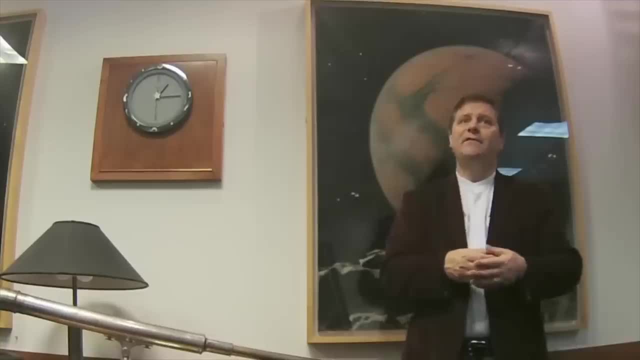 And of course, in the Southern Hemisphere, everything is flipped. So what we think of then is say, okay, let's relate these two things. The first thing is remember the path that the Sun seems to make in the sky. we call that the ecliptic. That's the same as if the Earth is going. 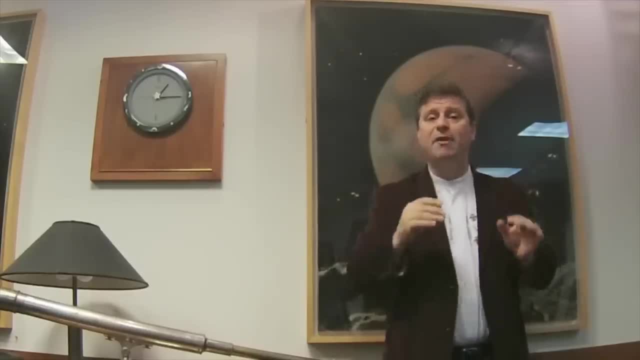 around the Sun or the Sun is going around the Earth. We can pretend either way, But the path that the Sun appears to make with respect to the background stars is called the ecliptic. However, that's not the same thing as the path that something appears to take. 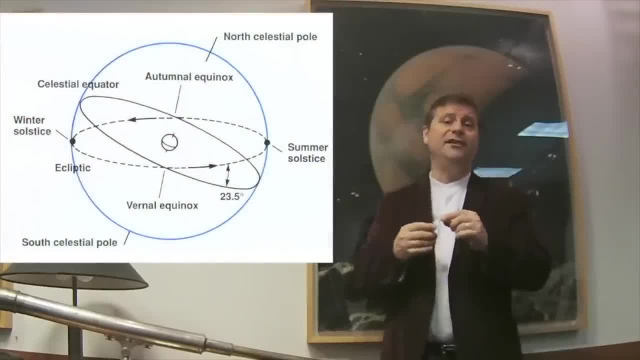 if it's on the celestial equator. The celestial equator is the Earth's equator projected out into space. So the tilt of the Earth's axis means that the celestial equator is not the same thing as the ecliptic and they intersect at only two points And we call those. 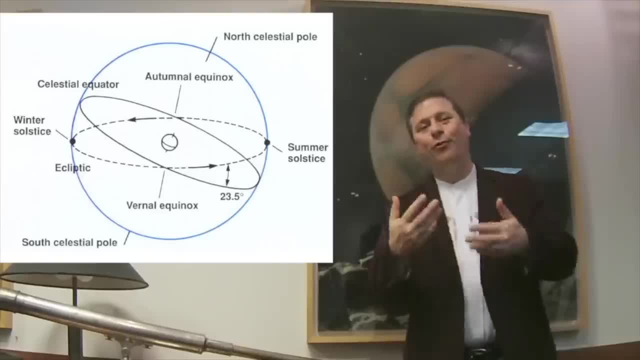 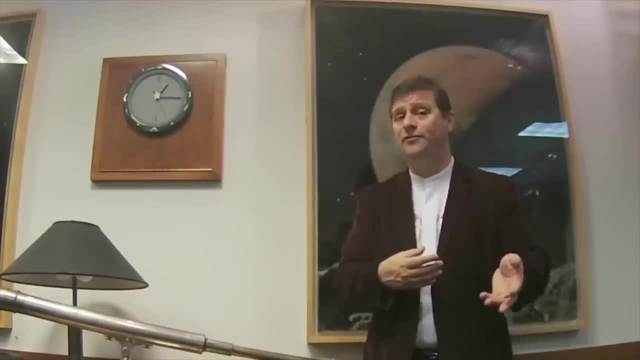 points, the equinoxes, So the four points that we always remember. we say the vernal equinox and the autumnal equinox, there's the summer solstice and then there's the winter solstice. So here's the idea: is that when the Earth is in the 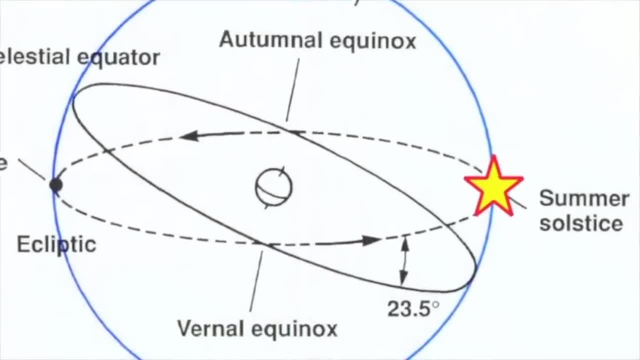 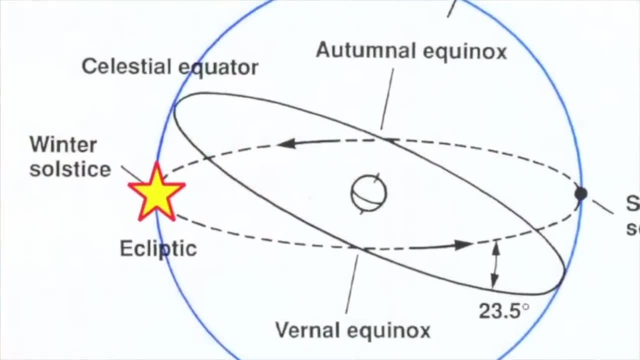 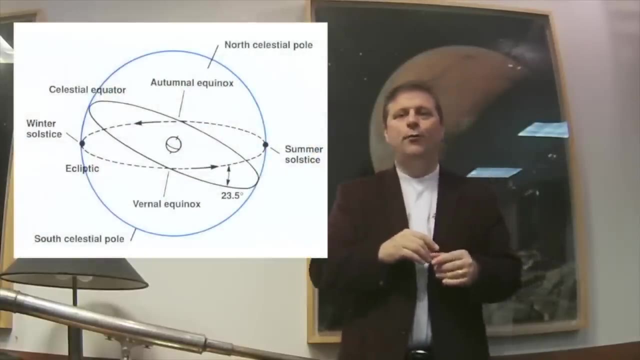 summertime the Sun is above the celestial equator by 23 degrees, And when it's in wintertime it's below the celestial equator by 23 degrees, And at the equinoxes it is exactly on the celestial equator. So we have 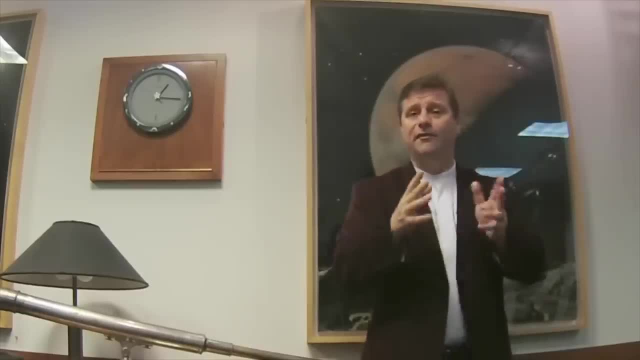 as it travels around. we call the vernal equinox the beginning of the. well, it seems to be. it's a natural place to think of the beginning of the year And, in fact, astronomically, it's kind of the way we think about it. it's the beginning of the year because that's where two orbit 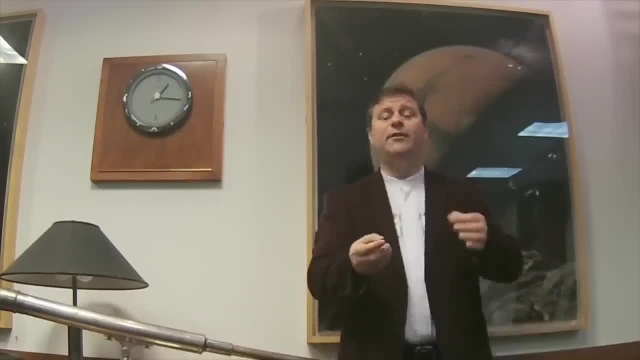 that's where? well, it's a very important point because it gives us the reference point between the ecliptic and the celestial equator. So the seasons, therefore, are caused not by the distance between the Earth and the Sun, but because of the angle of the tilt of the Sun. The distance of the Earth and the Sun actually doesn't change that much, because the Earth's orbit around the Sun is almost perfectly circular And in fact during the northern hemisphere- winter- we're closer to the Sun by a lot. 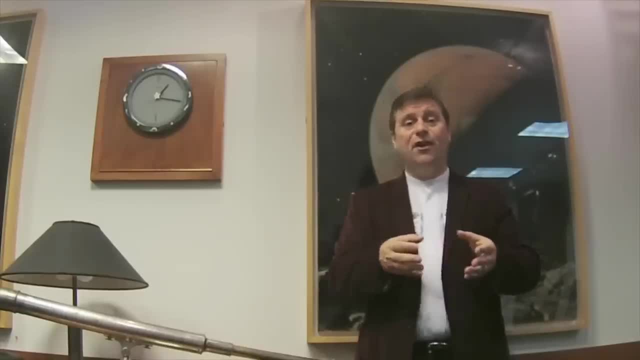 by a considerable amount of distance compared to the summer. So if there was a distance problem, then we would always see that the winter would be hotter. Now, this doesn't I mean if we were in the orbit of Mercury all of a sudden- 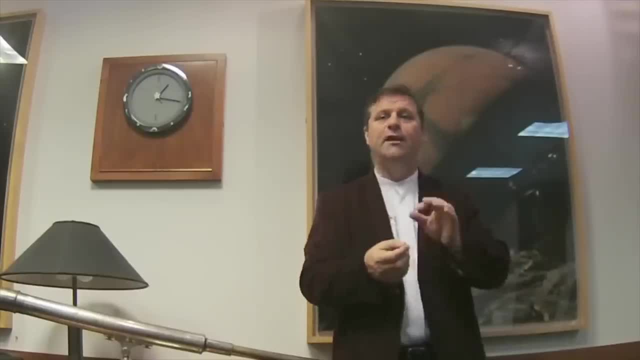 yeah, it would be hot. And if we were out by Mars, yeah, it would be cold. But the Earth's orbit is almost perfectly circular, so the dominant effect of the seasons is as a result of, simply, the tilt of the Earth's. 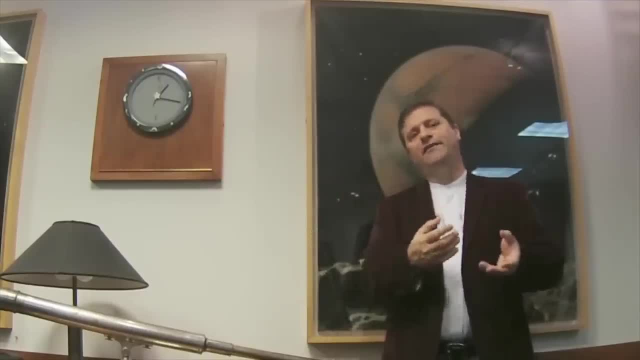 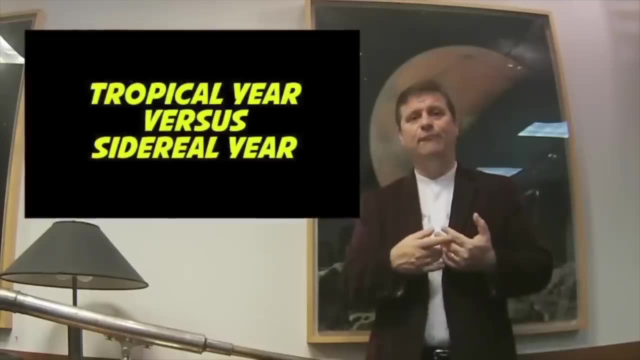 axis. Okay, so the next thing to think about is: okay, we can talk about the year then. I kind of alluded to it. What is a year? A year is season to season, And we call that the tropical year. 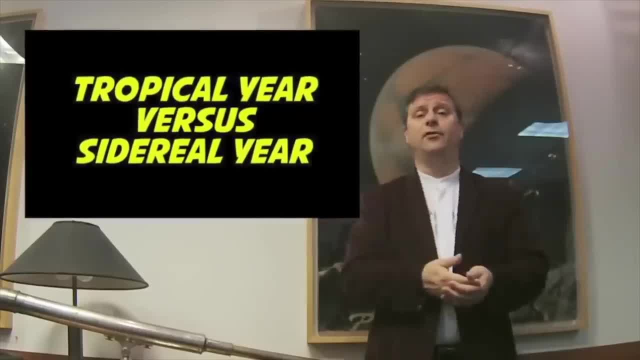 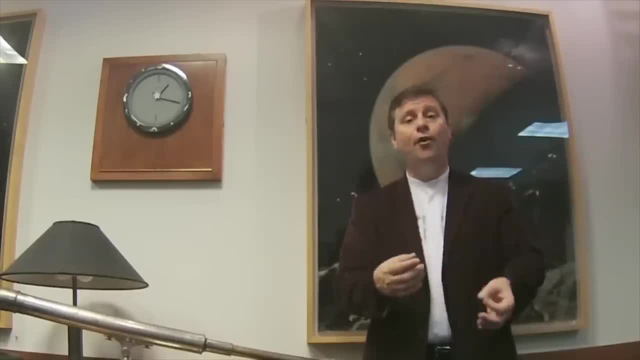 It goes from say we can call we the western culture, we say January 1st to January 1st. We could use vernal equinox to vernal equinox or summer solstice to summer solstice. All of those points are. 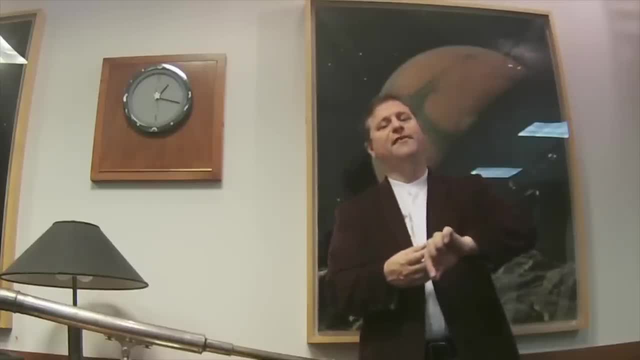 what we would call a tropical year, But we could also define it with respect to the sidereal year. Now, a sidereal year is when the Sun gets back to the same place in the sky with respect to the stars, as it did a year ago. 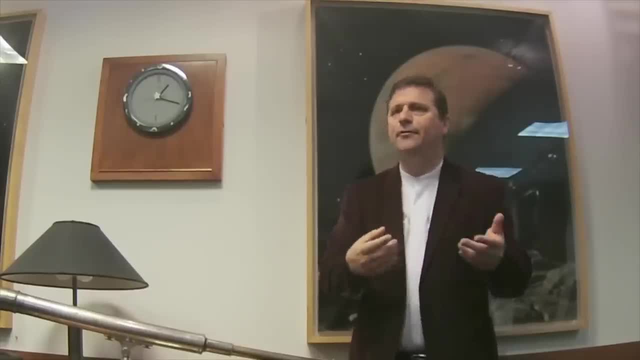 So the funny thing is is that might not sound like it's a difference because, all things being equal, all things being equal, they should be the same, But they're not. In fact, the sidereal year is about 20 minutes longer than the tropical year. 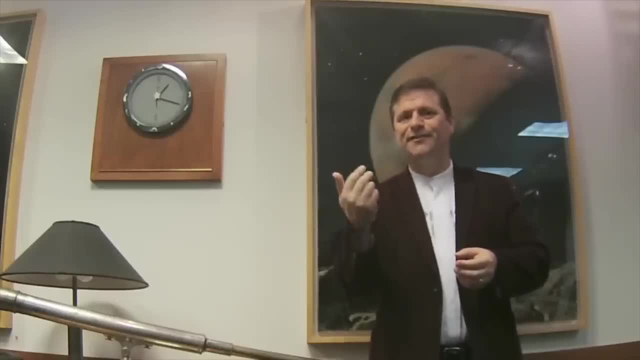 And the reason for that is because, yes, the Earth's spinning, But the Earth, just like a top, precesses. So note, remember, when you take a top and you spin it on a table, after it first starts off nice and steady, it looks really cool. it's a lot of fun if you have a really good. 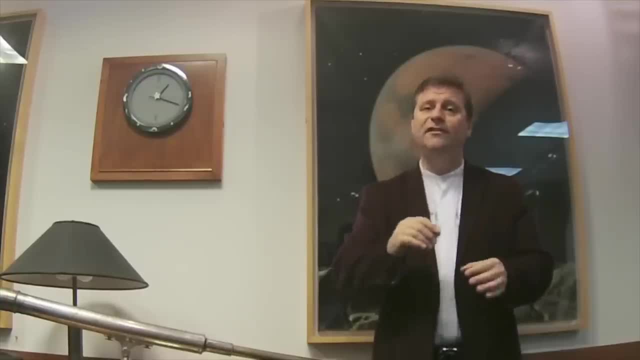 top. it'll spin for a long period of time But eventually the top slows down And as the top slows down, the top of the top starts to make a circle and starts to go lower and lower and lower, And it's not just rotating on the spin axis. 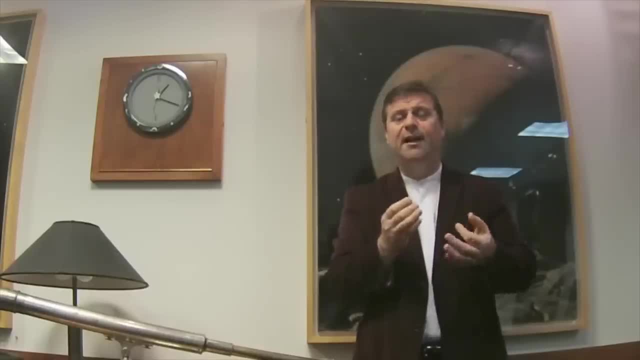 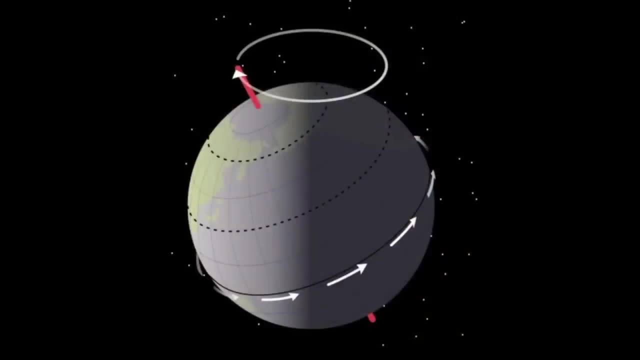 but now the direction of the spin axis is changing, That motion that we call precession, And so precession also happens to the Earth as well. So the Earth's spin axis changes with respect to time. Now, in a human's lifetime you're not going to see too much of a change, because the time it takes. 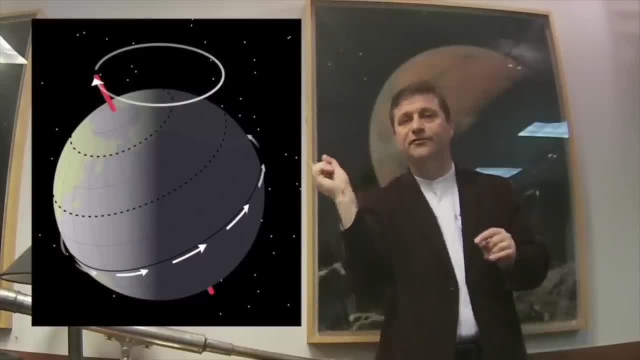 for the Earth's spin axis to change is about 26,000 years. It takes a long time for it to make one full spin. That's a long time to wait, But if we think about it that makes a really interesting set of. 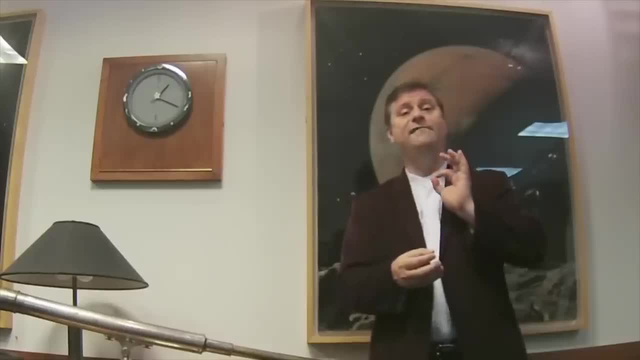 analogies throughout human history, Because 5,000 years ago, right about the time that Egyptians, the ancient Egyptians, were creating mummification, the North Star was not Polaris. Polaris sits today, roughly today, at the North Celestial Pole, which is the extension of. 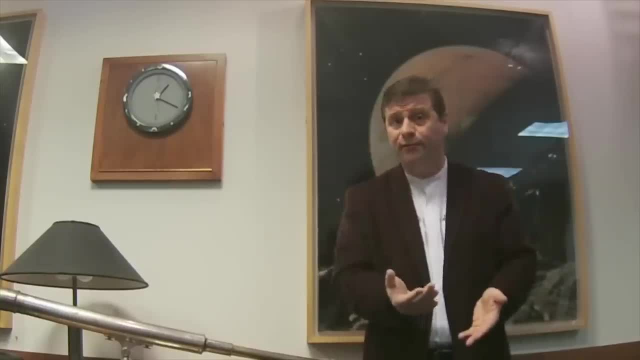 the Earth's rotational axis out into space. So if you were to be at the North Pole, lay on your back, look straight up. you would see all the stars going around you in the course of 24 hours with the North Star Polaris. 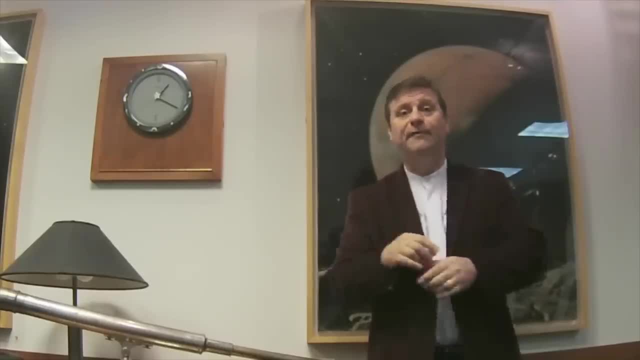 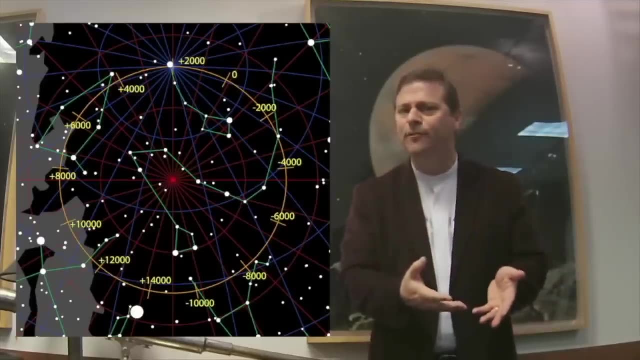 or Alpha Ursa Minor, straight overhead. Now, if you go back 5,000 years ago, at the height of the ancient Egyptian civilization, when they were beginning the mummification process for their pharaohs, that star was Thuban in the constellation. 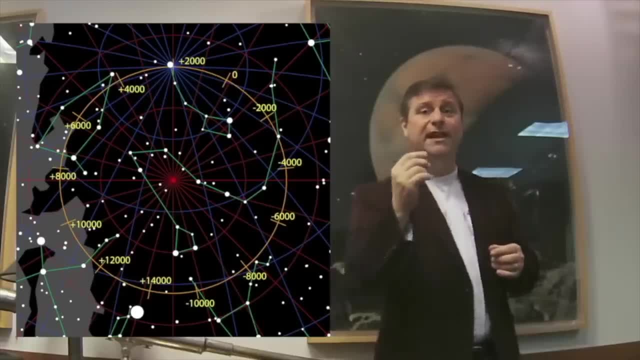 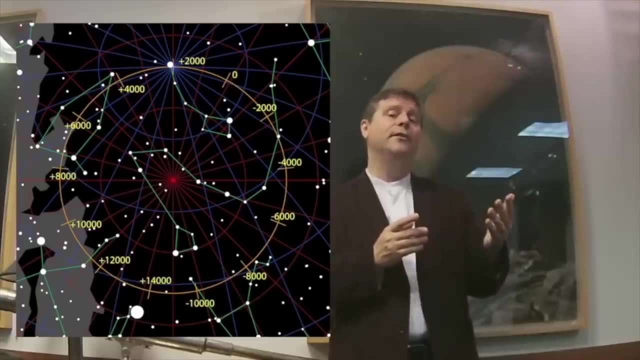 Draco, It was not the North Star, because the precession had not yet brought it to Polaris. And if we go back even further, say about 10,000 years ago or 12,000 years ago, the first inklings of the domestication of cattle 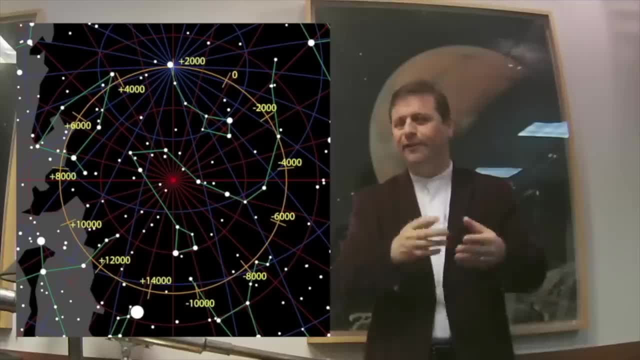 the founding of Jericho happened about 12,000 years ago, roughly speaking. So when we look at it well, at that time the North Star was the star Vega in the constellation Lyra, clear across the sky, a huge angular difference of about 46. degrees across the sky. That's a big, big, big angular difference, But that was 12,000 years ago. So therefore, if we were to go to sleep today and wake up in 12,000 years, the North Star would again. 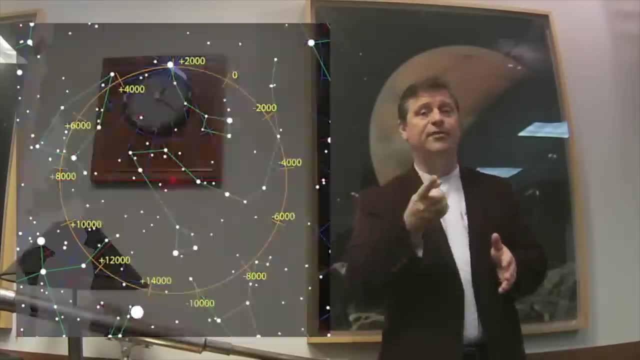 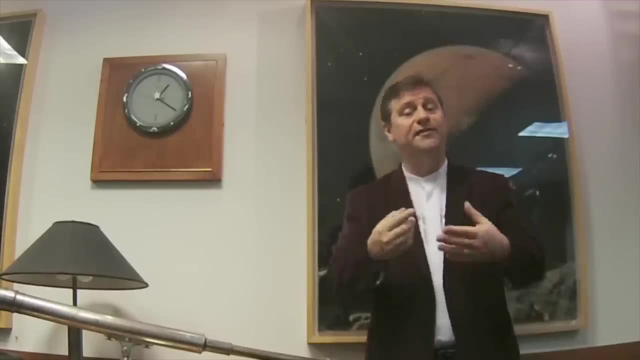 be Vega, So that's kind of cool, But it takes a long time for that precession to occur. Now there's also little tiny wobbles that are associated with that as well. It's not a perfect circle, because the Earth has a moon and that actually. 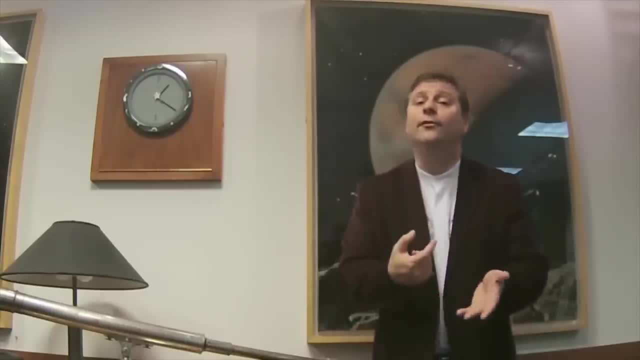 takes it around a little bit, But that's kind of the summary of the Earth's motions. So the Earth's motions are kind of complete here and we can talk about them in the following. We've got the Sun apparently going around the sky on what we call the ecliptic. We've got the Earth, the extension of the. 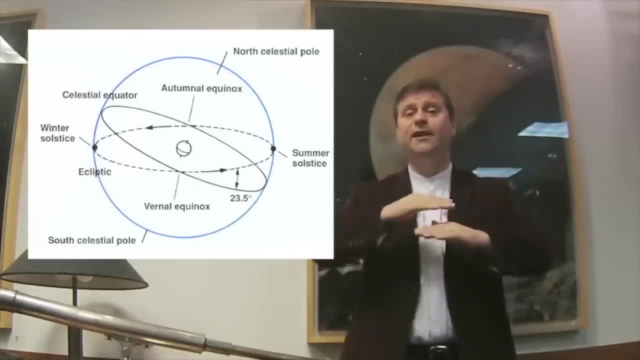 equator out into the sky and we call that the celestial equator. And because of the tilt of the Earth, the celestial equator and the ecliptic only intersect at two places: the vernal equinox and the autumnal equinox. 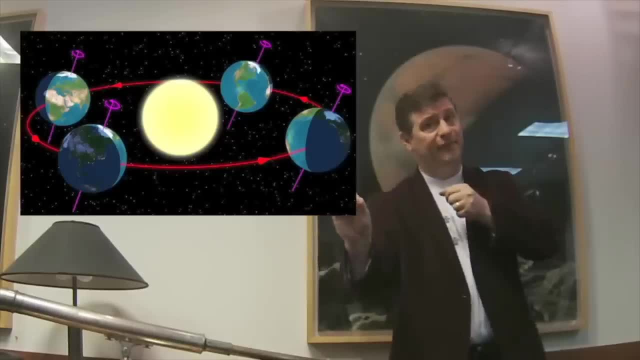 So, as the Sun, as the Earth goes around the Sun in a given year, the Earth's axis of rotation points only in one direction, and so, therefore, the seasons are caused by the directness of the sunlight on the surface of the Earth in that hemisphere. 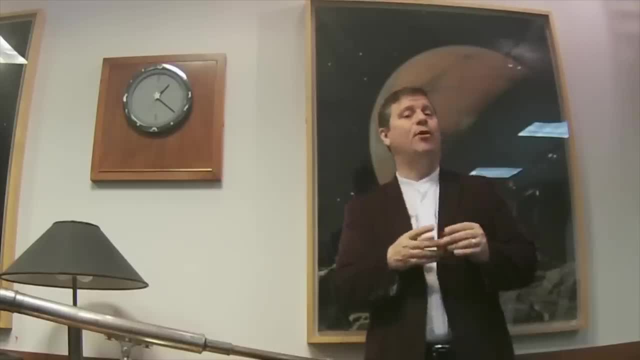 And, of course, precession occurs, and that's been part of human history. In fact, if you go way back and look at ancient Egypt and go to the Met over in New York City, you'll find that the ancient Egyptians actually made. 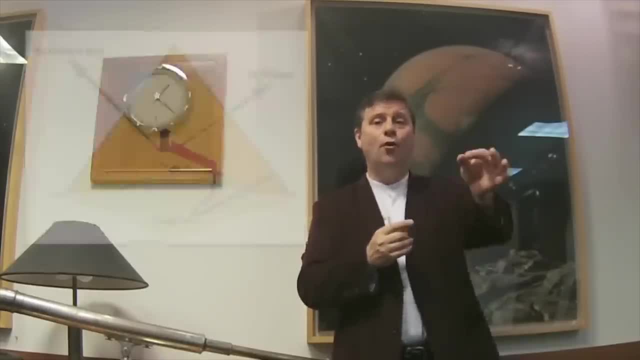 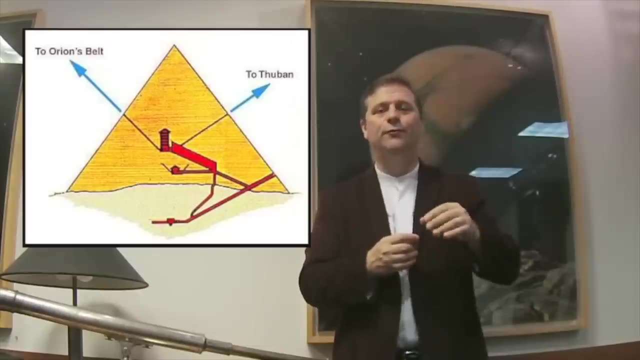 the Great Pyramids. There's a hole in one of them that if you were in the center of the pyramid looking out through this hole 5,000 years ago, you would see the star Thuban. Today you don't see the star Thuban, But back then the engineers 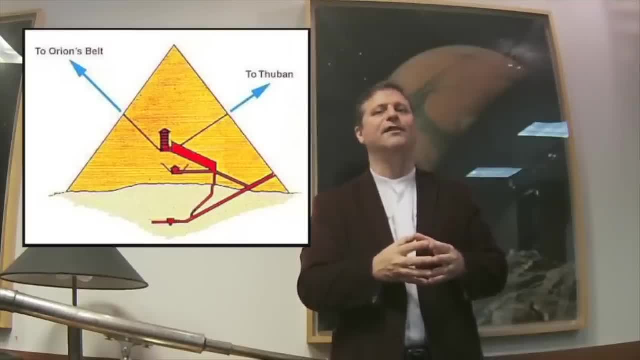 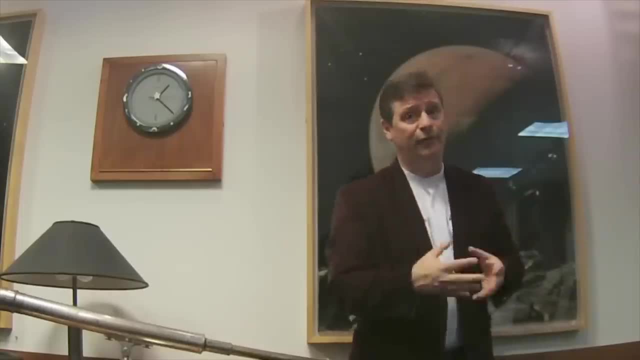 of the Great Pyramids made sure that the pharaoh would always look at that thing, even as he was mummified and deified as a god. So astronomy has had a big impact over time and these are some of the major impacts and those are some of the orbits of the Earth. 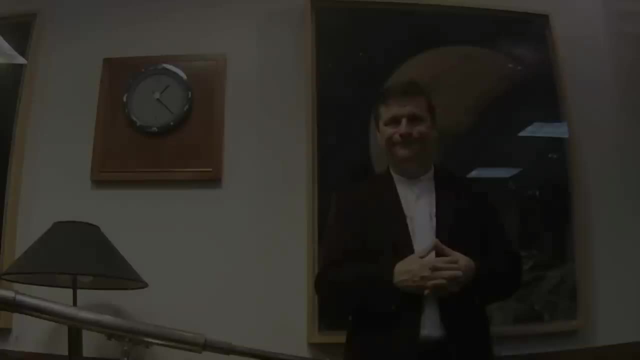 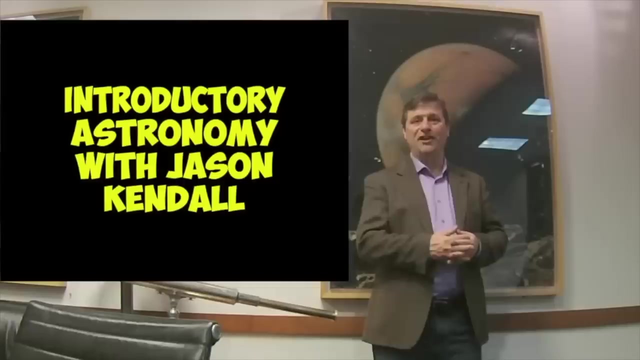 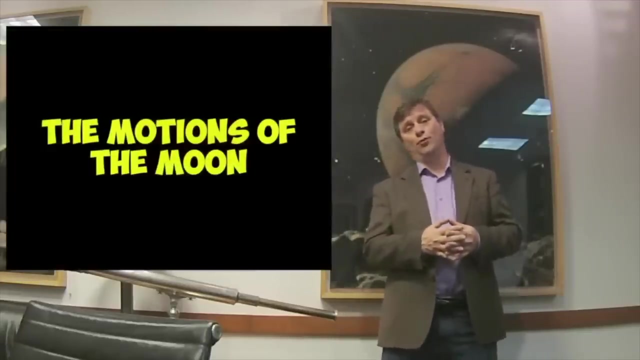 and some of its motions. We'll see you next time. Hello everyone, My name is Jason Kendall, and welcome again to another lecture on introductory astronomy. Today we're going to be talking about the motions of the Moon. Now, the Moon is very, very, very familiar to. 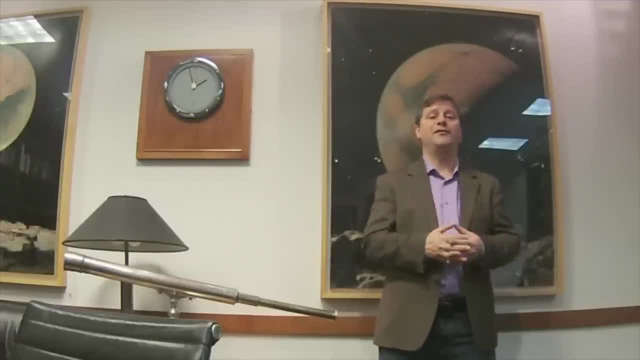 everyone. Everyone sees it in the sky. It's probably the most familiar astronomical object that we have that everyone knows about other than the Sun. The Sun and the Moon, and ostensibly the stars, are mostly familiar things, But the Moon is, of course, imbued with lots of 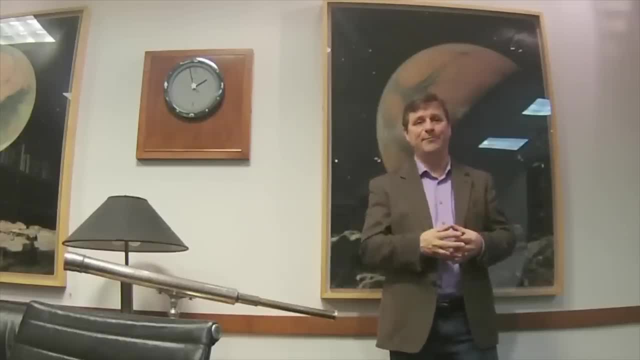 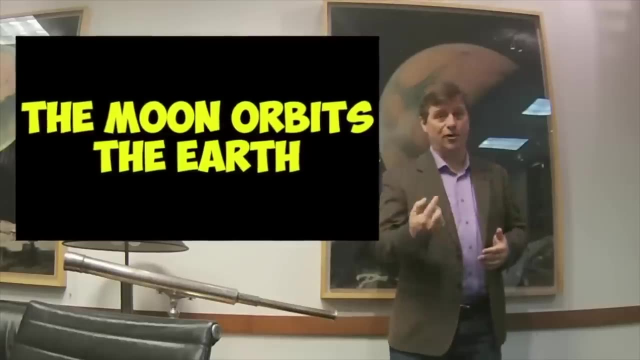 things from literature and culture, and so we can't escape its view. So let's talk about it for a bit. The first thing to understand about the Moon is that, well, it orbits the Earth, And as it orbits the Earth, it goes through what we call phases, because of the relative 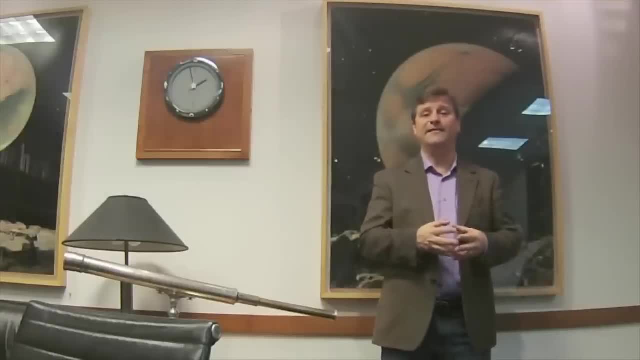 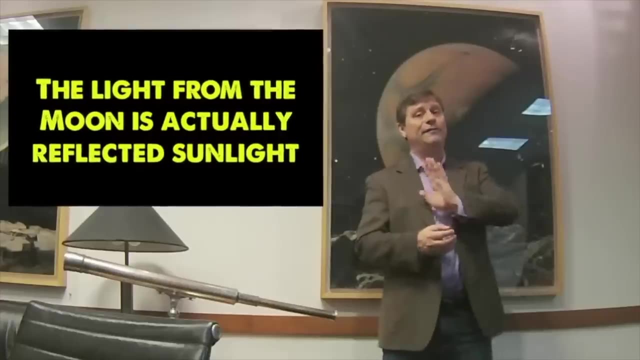 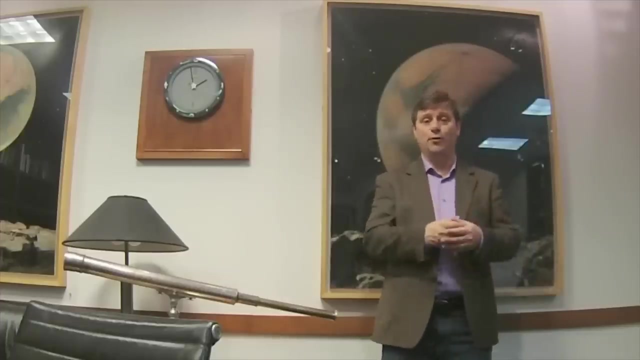 position of the Moon and the Earth with respect to the Sun's light. So the Sun shines on both the Earth and the Moon. The light reflects off of the Moon, and what portion of the reflected part that we see becomes the phase of the Moon. So always half of 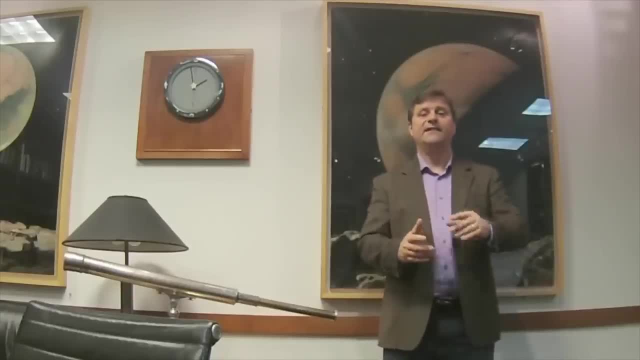 the Moon is illuminated by the Sun Always. Sometimes we see the entire half that's illuminated and sometimes we see only a part of it. Most of the time we only see a part of it And at very special times we see none of it. 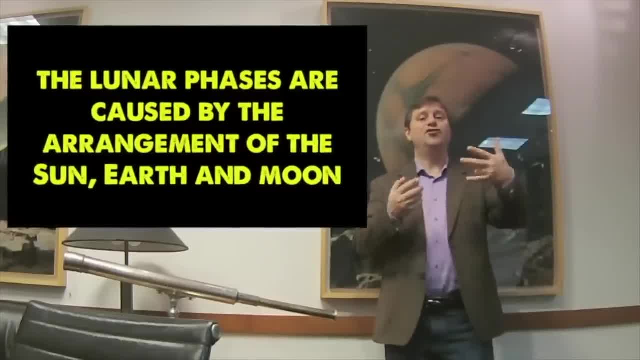 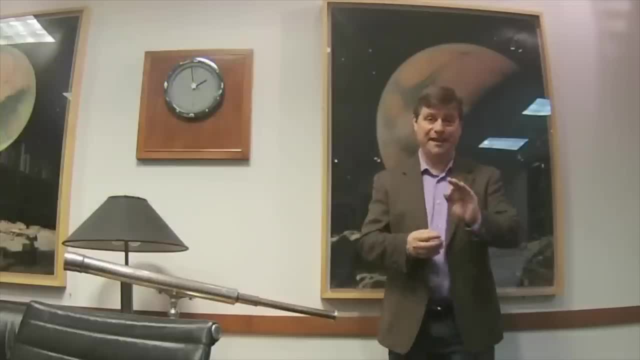 and that's called New Moon. So let's talk about the New Moon. Let's talk about the phases. So the geometry of the position of the Earth and the Moon dictates the phases. It has nothing to do with the shadow of the Earth on the Moon. 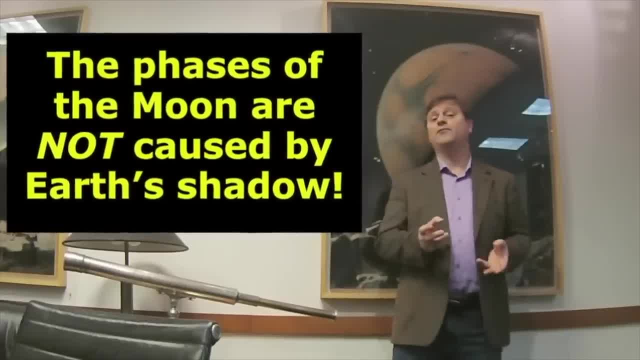 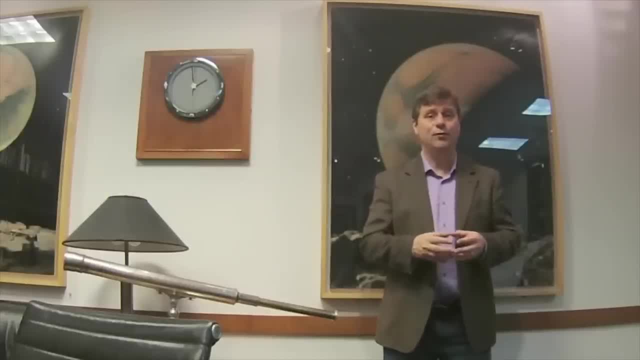 In fact, that's a really common misconception. It's one of the most common misconceptions of all- that the phase of the Moon is caused by the shadow of the Earth on the Moon, and that's simply not true. The shadow of the Moon is very large. 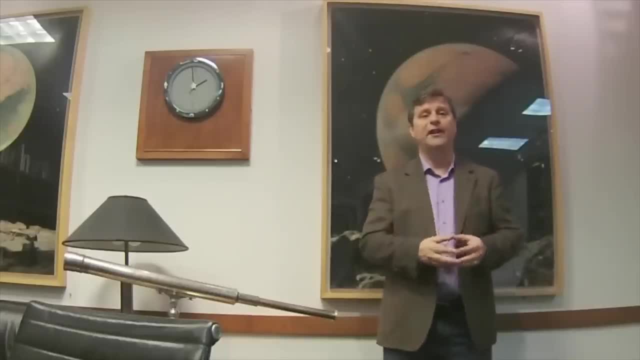 and when the Moon goes into the shadow, we call that a lunar eclipse. That only happens quite rarely, So let's actually look at what we see in the sky. So the first thing that we see is we call these things phases, and they go through. a whole cycle of phases throughout the month as the Moon orbits the Earth. in one month time It starts off as New, then it goes to a waxing crescent: a first quarter, then a waxing gibbous, then full, then waning gibbous and then after that. 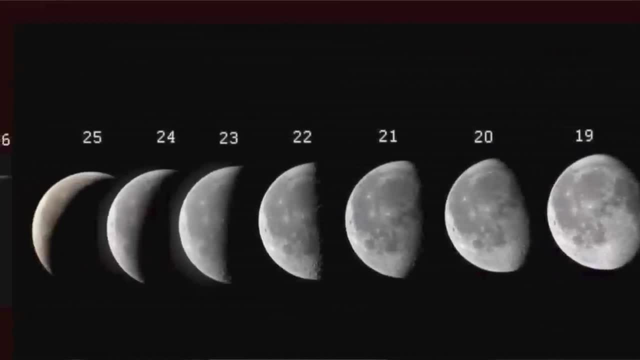 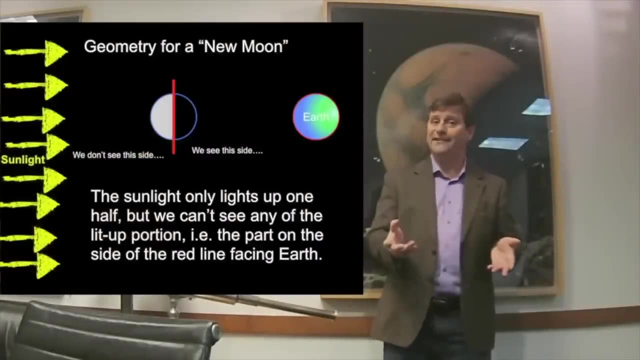 is third quarter, then waning crescent and then back to New Moon. So what are these things and what are their various geometries? Well, a New Moon is actually a Moon that you can't see, which is kind of a funny thing. 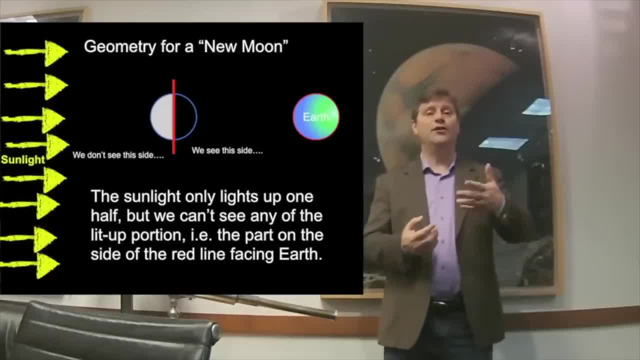 to think about. but the New Moon is the phase of the Moon, when the Moon is in the same direction as the Sun in the sky. So if it's roughly in the same direction, you're not going to see the Moon in the sky. 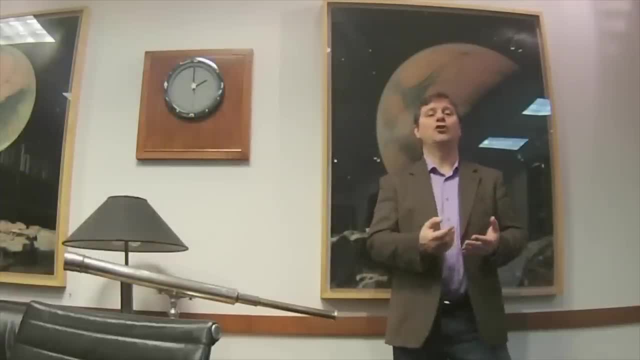 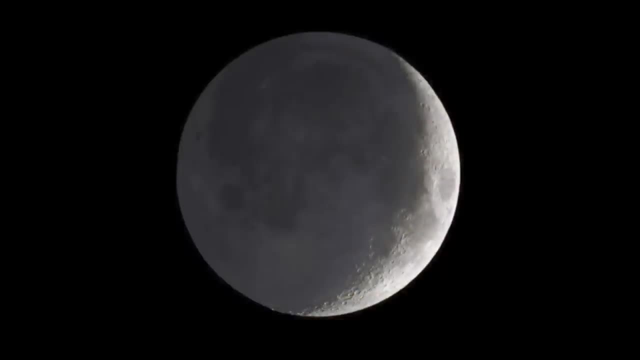 and so, therefore, it's called a New Moon. It's kind of an odd description, but that's what we call it. We call it a New Moon. Anyway, the first time you see the Moon is at what we call waxing crescent- A waxing crescent Moon. 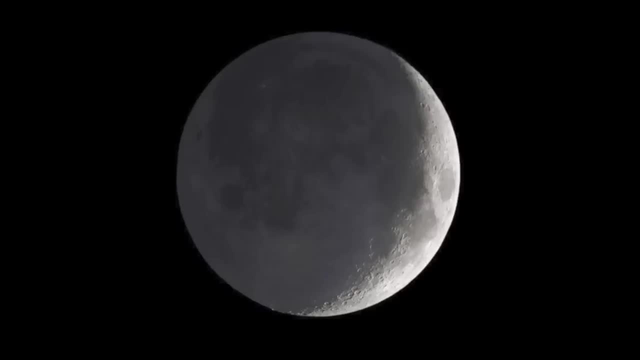 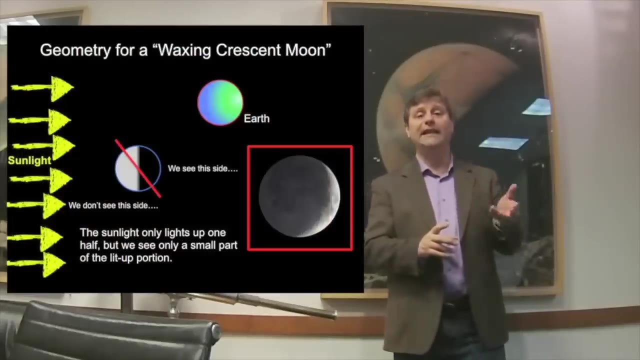 rises just after sunrise and then it sets just after sunset, So a waxing crescent Moon is only visible in the early evening, just after sunset, And it's just a portion of the Moon that we see. It looks like a croissant or a crescent, which is where that word in French gets its name: a crescent. 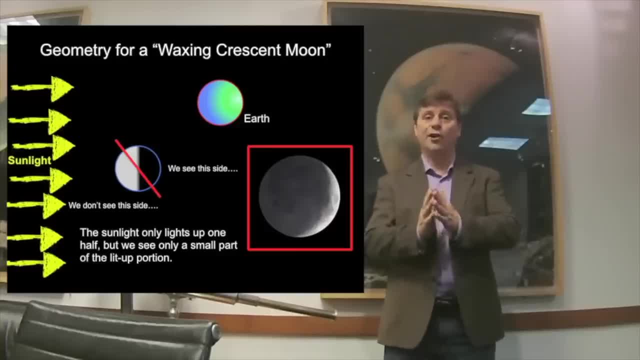 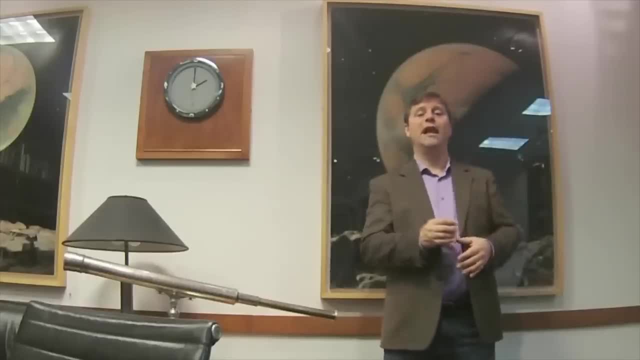 So the crescent Moon then appears to get larger and larger with time over the course of days, and then, a couple of days later, we see what we call a first quarter Moon. Now, a first quarter Moon to some people says, well, it's a half. 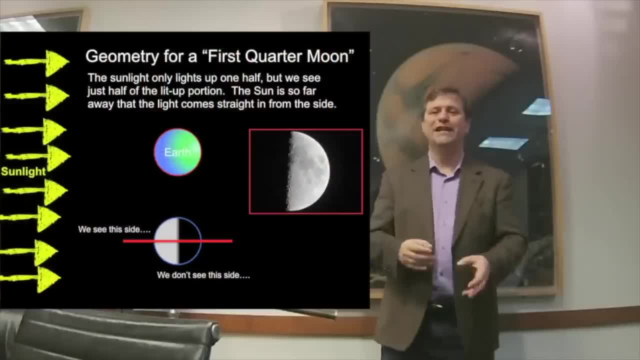 Moon. Well, it's not a half Moon. We call that a quarter Moon because we only see the light from one quarter of the Moon. Half of the Moon we don't see which is the far half, The near half. we see that side, but only half of the near half. 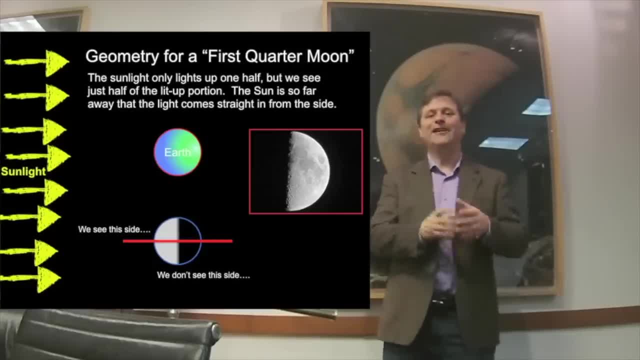 half of the near half is illuminated, so that's one quarter of the Moon. So that's why we call it first quarter. It also happens to correspond to when the Moon is 90 degrees around its orbit around the Earth, So that is a quarter of the way through its orbit around. 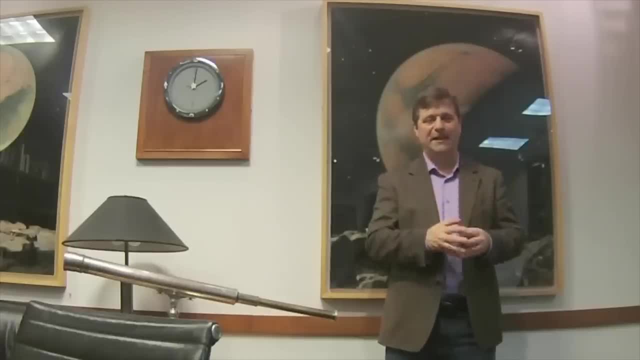 the Earth. so that's its first quarter And it's half illuminated. Alright, so a half illuminated Moon is called first quarter, just to be totally confusing, for no good reason other than why not? And after the first quarter Moon a few days later after the first quarter. 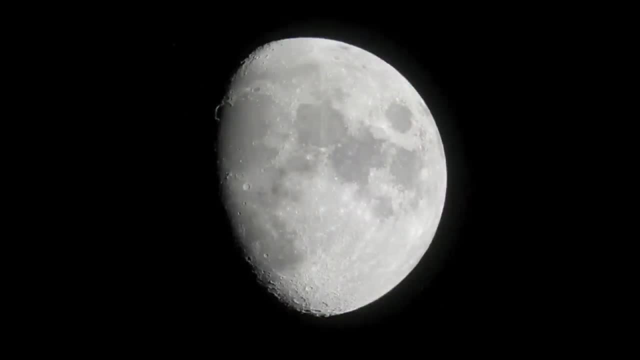 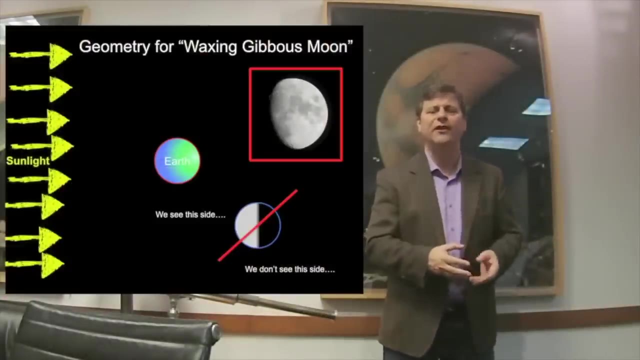 it's more than half illuminated. and when the Moon is more than half illuminated, we call that a waxing gibbous Moon. That's a funny word, gibbous, but it just means more than half illuminated. And as time goes on we get to a full Moon. 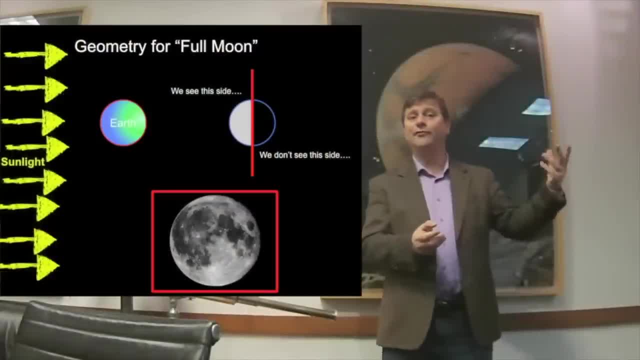 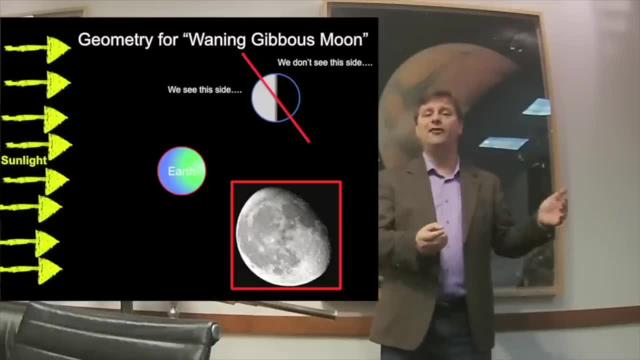 And a full Moon is fully illuminated. After the days after full Moon, then we have a waning gibbous Moon which again is more than half illuminated, and then we go through third quarter Moon, where it's half illuminated, according to how we see it. on. the Earth and then it goes to a waning crescent Moon and then back to new Moon. So that is the cycle that occurs every 29 days and we call that the synodic month. And the synodic month is the month with. 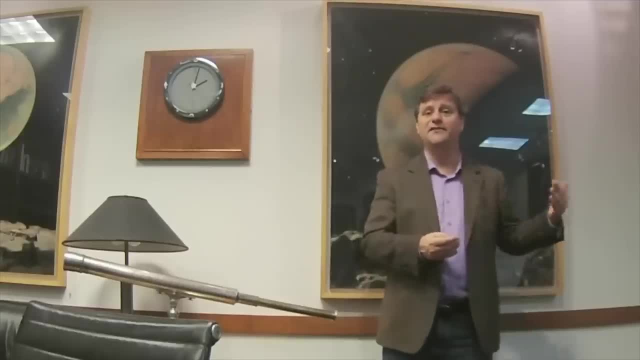 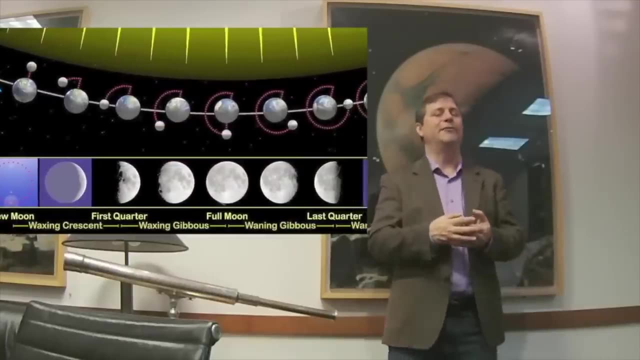 respect to the phases of the Moon. So the synodic month traces basically the Moon as it goes around the Earth from phase to phase. So we have to kind of reference the Sun inside of there. And so there's another definition we could use for the Moon and we would call that the sidereal month. 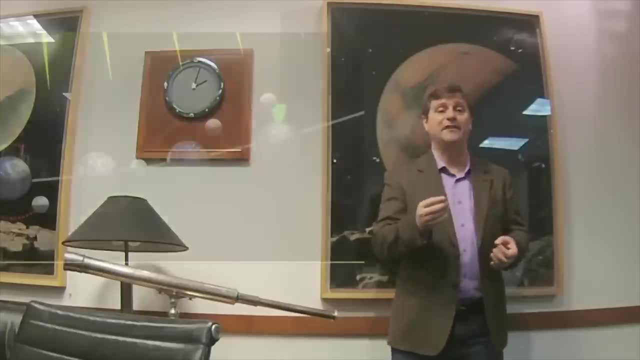 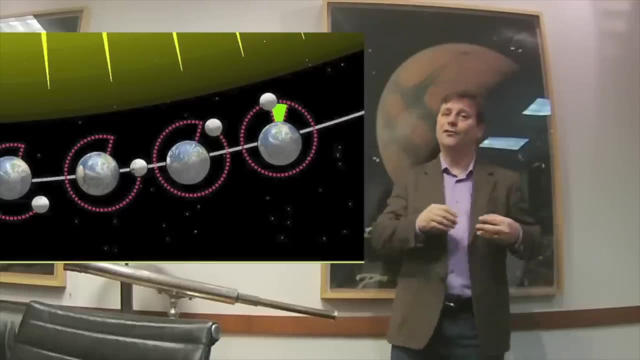 The sidereal month is the Moon's position in the sky with respect to the background stars And, of course, since the Earth is going around the Sun, as the Moon goes around the Earth and the Earth goes around the Sun, it's a shorter time for it to take. to get back to the same place in the sky with respect to the stars than it does with respect to the Sun, So the sidereal month is shorter by about two days, and so therefore, we get roughly 27 days as the sidereal month. Well, most people don't think of the sidereal month, so let's stick with. 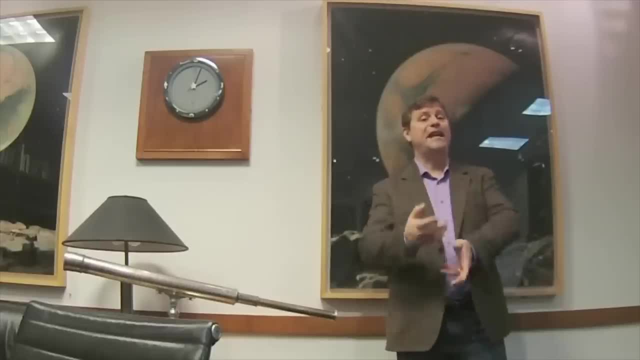 the synodic month, which is phase to phase. Now here's how the phases go. So sometimes you see that in paintings or literature or even just common thought, most people really think that the phases, the Moon's up all the time. They say, oh wow, let's go outside and see the Moon. 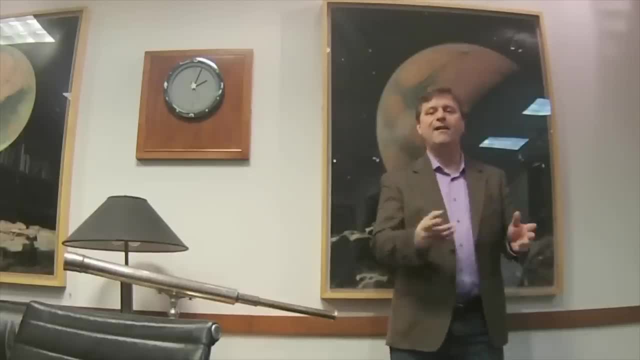 let's go see the Moon, And they always think of the Moon up at night. Everybody always says: let's go out and see the Moon at night. Well, sometimes haven't you noticed that you see the Moon during the day? They see it as a gibbous phase during the day And sometimes 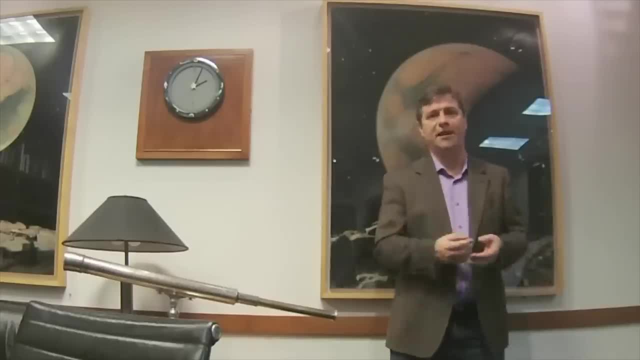 you don't see it at night and you go: well, where's the Moon? And you say, well, it's gotta be up, it's nighttime, it's the Moon. Well, the Moon is not always up in the sky at night. So let's look at the various phases As I alluded. 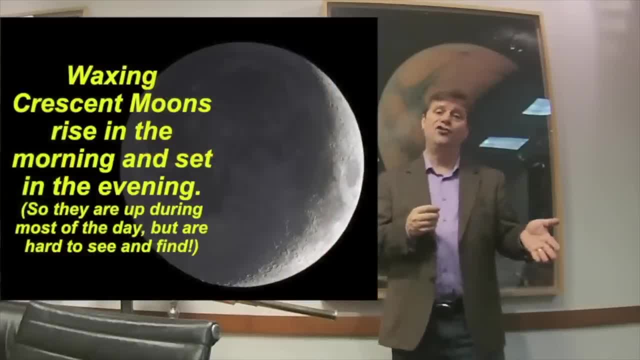 to before. the waxing crescent Moon rises just after sunrise. So it's up in the sky most of the day, but it's so close to the Sun that it actually is overwhelmed by the sunlight. And we can only ever see the waxing crescent Moon just after sunset, when it's low. 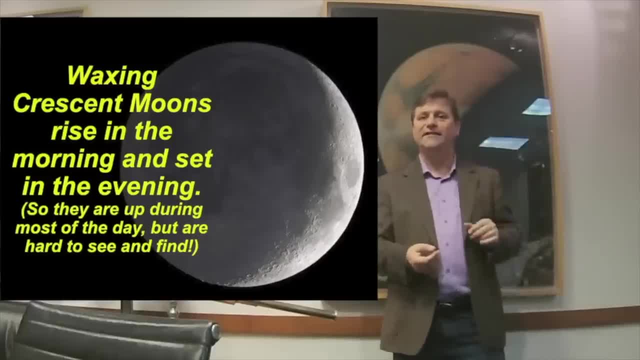 in the West and its curved portion is facing towards the Sun. Now sometimes we think of there's a line in Shakespeare where we call it the horned Moon or the horned Moon, So it looks like it kind of has got a. 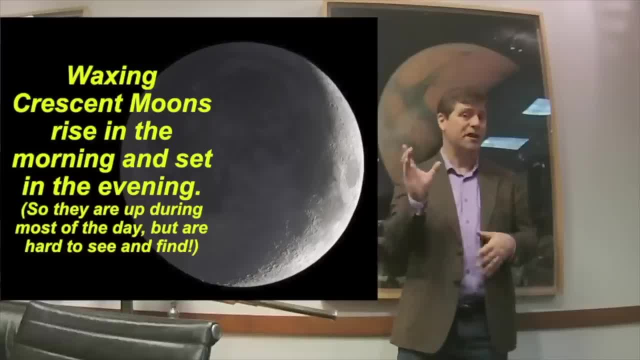 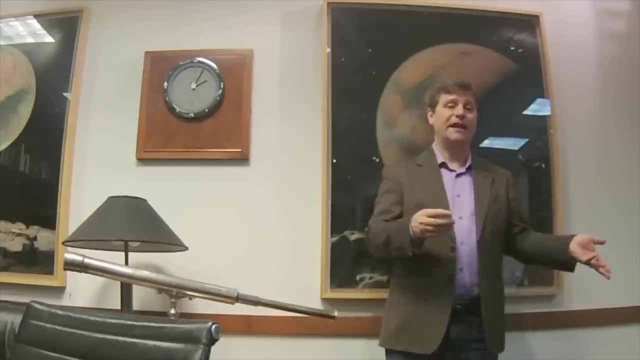 pair of horns, and that's another way of thinking of a crescent Moon. The horns of the Moon, when it's in crescent phase, point away from the Sun. Alright, so the crescent Moon rises in the morning and sets in the early evening. Now, when does the first? quarter Moon rise. The first quarter Moon rises when it's 90 degrees away from the Sun in the sky. That means the Sun is at noon, and therefore the first quarter Moon rises at noon, And so the first quarter Moon is high in the sky at sunset, and then it then. 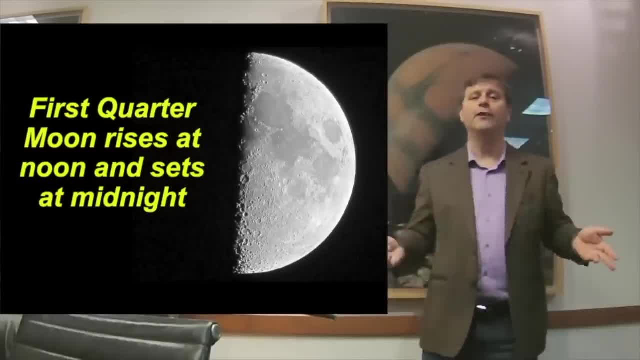 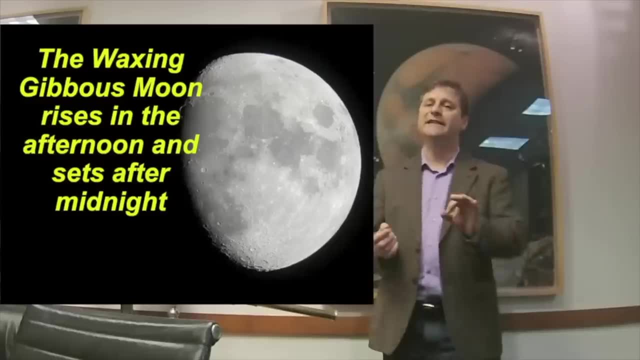 sets at midnight. So that's kind of neat. That's the arrangement for the first quarter Moon. Now gibbous Moons are up most of the night and most people think, ah, a gibbous Moon is a full Moon. But it's not a full Moon, It's more than half. 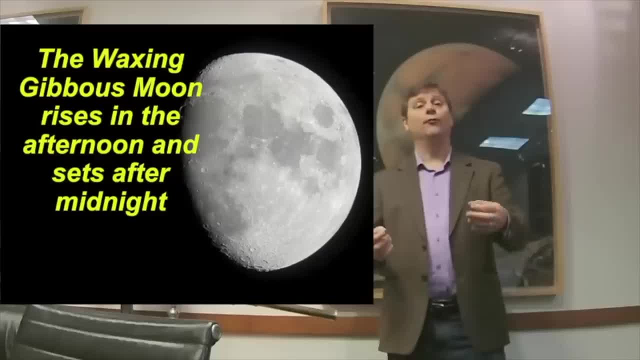 illuminated, but it's not full. A gibbous Moon rises after in the afternoon, So it rises at least in the afternoon. so as the Sun sets it's already up in the sky and we see it there, and it sets after midnight. That's a 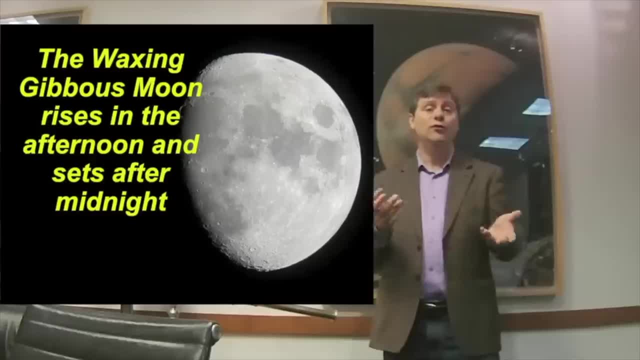 gibbous Moon And unless you really like stargazing, unless you like Moongazing, stargazing gets tough in these first, in these gibbous Moons, because it's up very much most of the night. So we are abandoning stargazing. 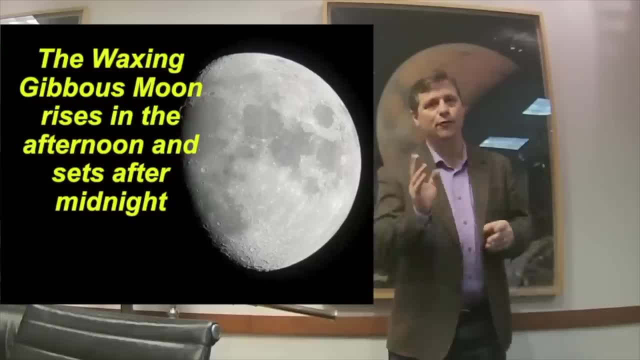 and looking for galaxies and quasars and also a nebulae when the Moon's up in a gibbous phase. but we can always go and take out our small telescopes and look at the Moon or our binoculars too. Alright, so the when we 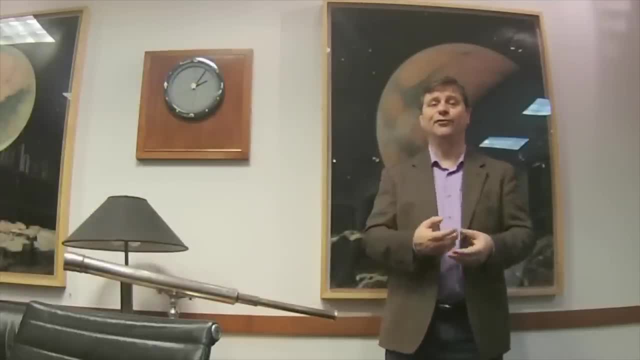 look at the gibbous Moon. it again rises after well after sunset. it's already been up in the sky, and so it's already been up in the sky as soon as sunset occurs and it sets well after midnight. Alright, so let's. 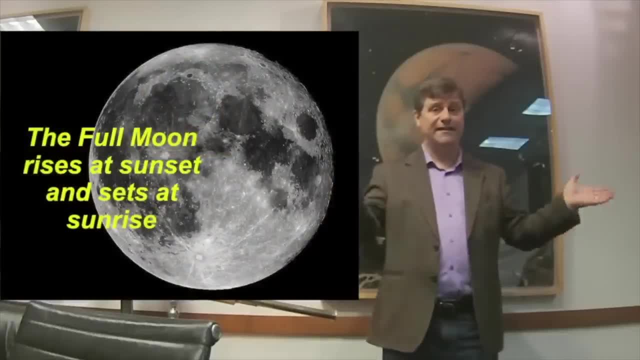 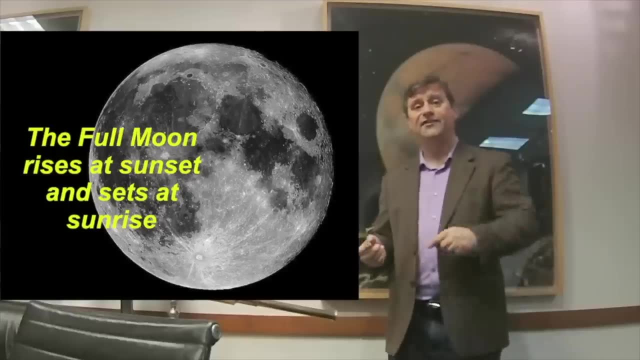 look about the full Moon. The full Moon is different. It rises, since it's exactly opposite the Sun in the sky. it rises at sunset and sets at sunrise, So it's up all night. That's the full Moon and everybody thinks, ooh, pretty full Moon, it's always wonderful. 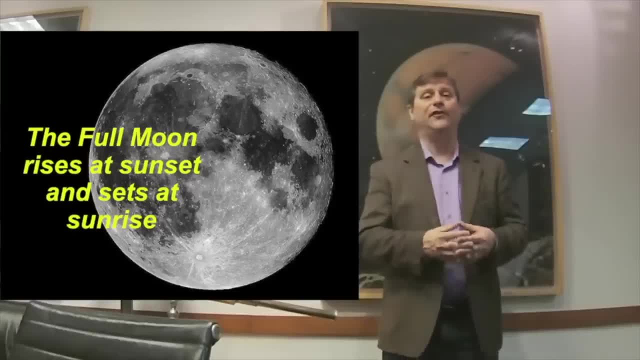 to go outside and look at the full Moon. it's beautiful and allows you to see some wonderful things, and everybody always has these wonderful superstitions about the full Moon, and that's to be discussed in a different time. Alright, so full Moons are beautiful. 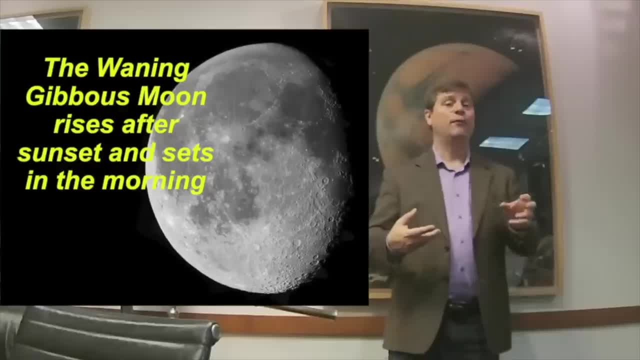 but then we go later, and so the waning gibbous Moon rises after sunrise. So you get a time in waning gibbous Moons when the Moon is not in the sky at all during the night time. So look at that. 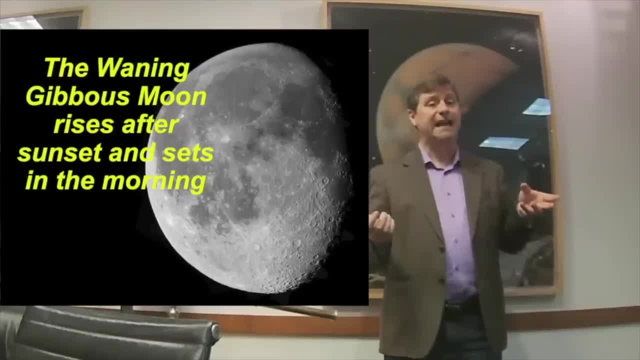 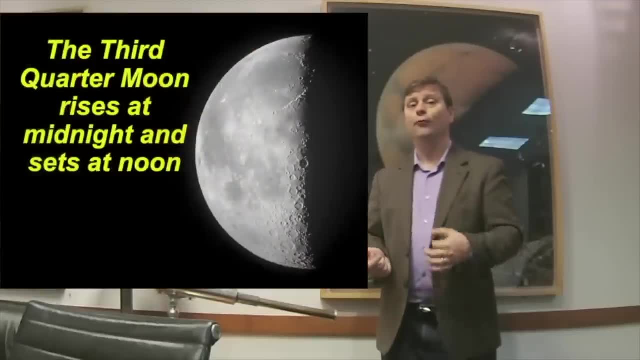 So you get the waning gibbous Moon. it rises well after sunset and sets well after sunrise. So that's the waning gibbous Moon. Third quarter Moon rises at midnight and sets at noon, So it's up for half the day. 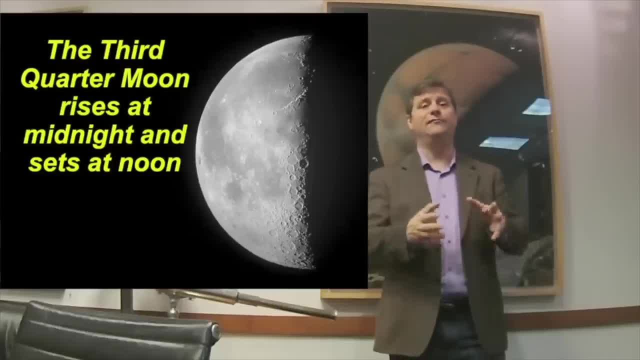 And it's very hard to see it when it's up in the morning. but you can probably catch it if you try in the early morning of the third quarter Moon, You can catch it and look like, wow, the Moon's up in the morning. Yeah, that's the third quarter Moon, Alright. 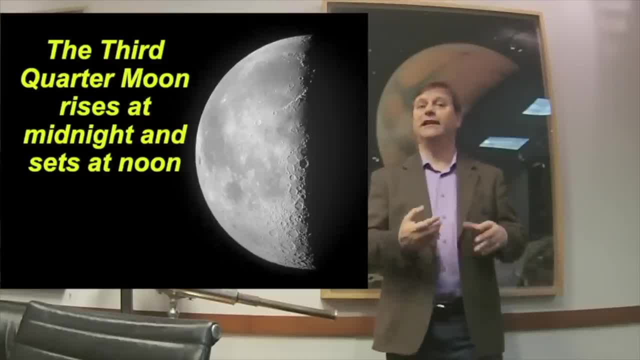 so the best time to do stargazing is usually for the evening. people who don't want to get up early in the morning is when it becomes third quarter Moon, Or even first quarter if you want to go late night, But third quarter Moon is always. 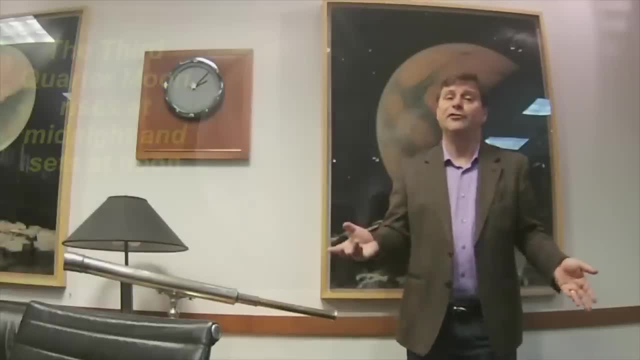 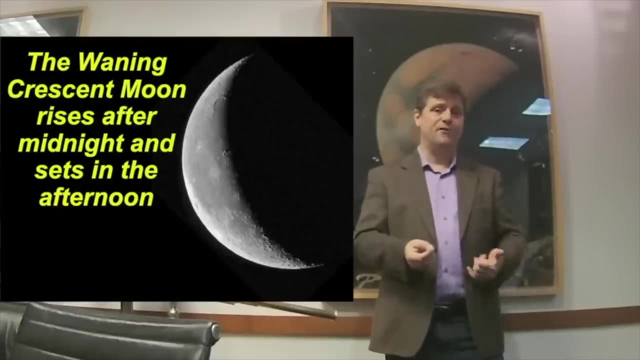 people's favorite time for stargazing, because hey, right after dinner go stargazing, right. So the crescent, the waning crescent Moon then rises very late at night, maybe 3 o'clock in the morning, well after midnight, and sets- well it sets. very far in the day, So it's actually up only a very short period of time at night before sunrise occurs. So it sets. if it rises at 3 o'clock in the morning, it'll set roughly 3 o'clock in the afternoon And then shortly thereafter the Moon. 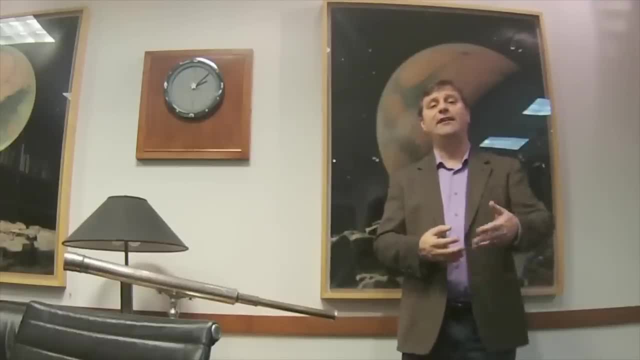 and the Sun will be roughly in the same position in the sky and you get new Moon Alright. so those are the phases of the Moon and their rough rising and setting times. Now we did discuss that people sometimes think that the shadow of the Moon causes 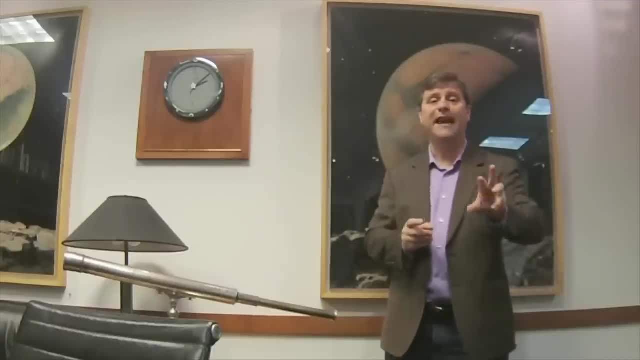 the phases, which is not the case. It's the geometry of the Moon and the fact that the Moon is spherical and the fact that the Sun can only illuminate one half of the Moon. Now, since these are big things- the Moon and the Earth are big things- they cast a shadow And so, since they 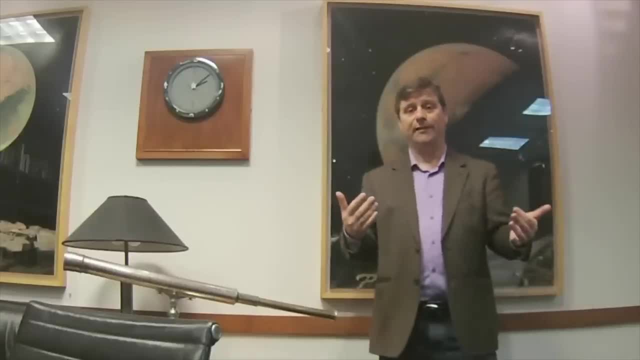 cast a shadow, they can pass into each other's shadow. Now it doesn't happen all the time, so you don't hear about them happening. they sound like more exotic events or important events astronomically, and that's because the Moon is not. 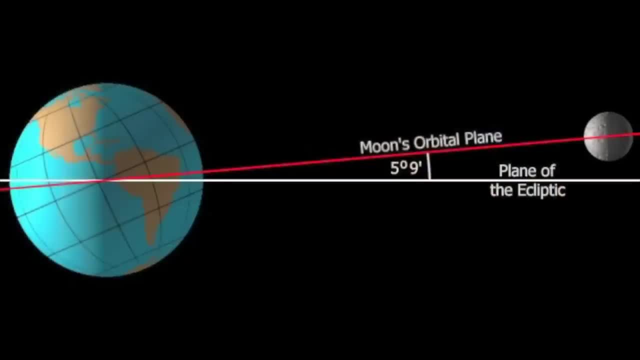 does not orbit in the same plane that the Earth goes around the Sun. The Moon's orbital axis is tilted about 5 degrees with respect to the ecliptic. The ecliptic again, is the path of the Earth going around the Sun. So since they're tilted, the shadow of the Moon 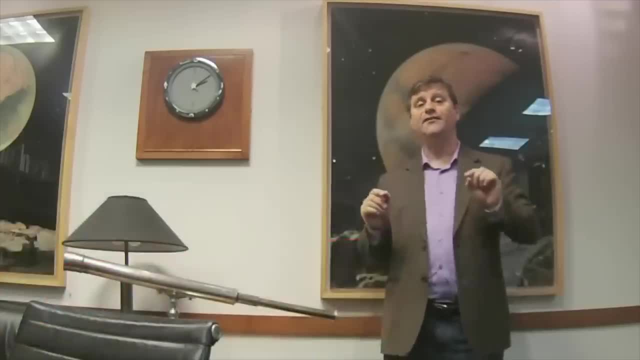 doesn't always hit the Earth, And likewise the Moon doesn't always pass into the shadow of the Earth. So these two shadows, or one of the objects, doesn't necessarily go into the other object's shadow very often. Let's talk about the first one, And the first one is what we'll call a lunar 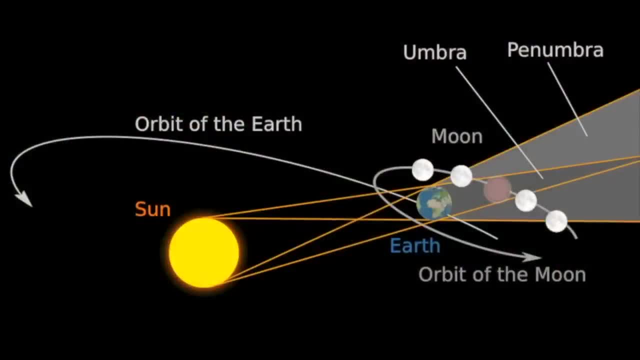 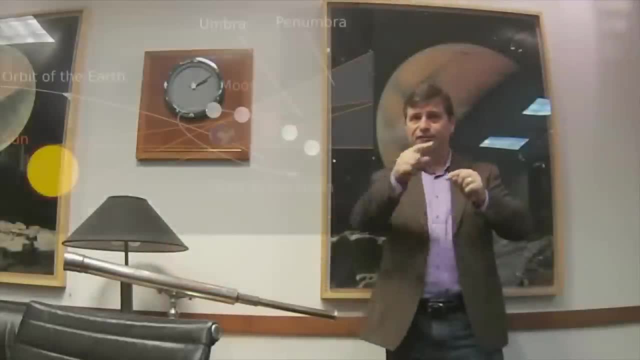 eclipse, And a lunar eclipse is when the Moon passes into the Earth's shadow. So that angle of inclination for the orbits has to be just right where the intersection of the Moon's orbit and the Earth's orbit around the Sun has to be just right and the Moon has to be 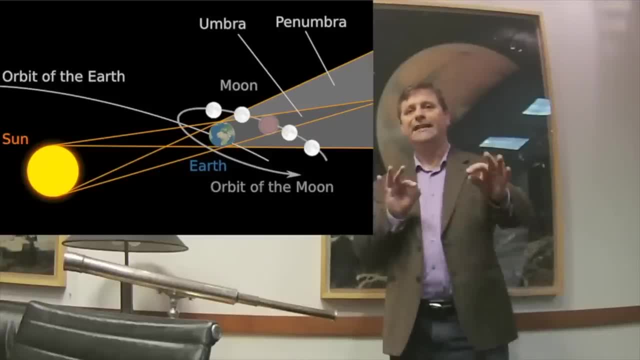 just on that intersection path. And when it is- and it happens to be- a full Moon, then the Moon can go into the shadow of the Earth And that's what happens, which we call a lunar eclipse. Sometimes it's a total lunar eclipse and you see a big chunk taken. 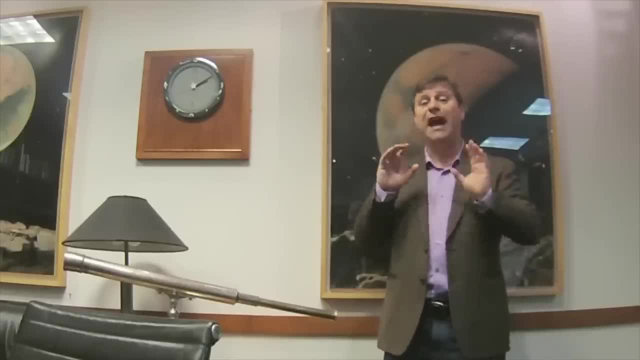 out of the Moon as it passes into the Earth's shadow and then it becomes a deep, deep, deep red from the refracted light of the atmosphere of the Earth landing on the Moon, and the Moon becomes so dim. even a full Moon becomes so dim that you can see stars right next. 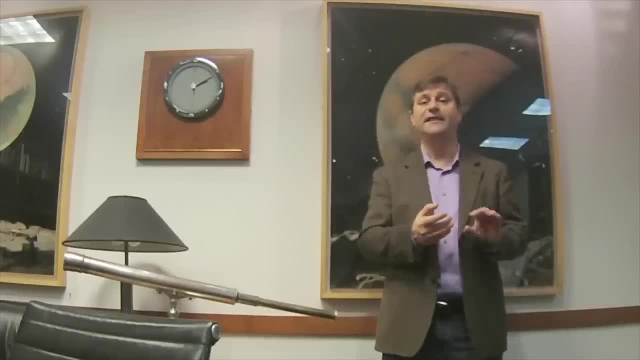 to the full Moon. It's a gorgeous, gorgeous sight and if you ever get a chance to see a total lunar eclipse, do so. It's a wonderful sight. Stay up all night if you can. I had the opportunity to actually watch it in the Caribbean on board. 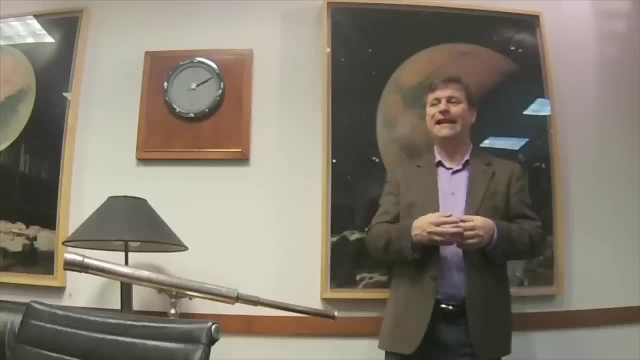 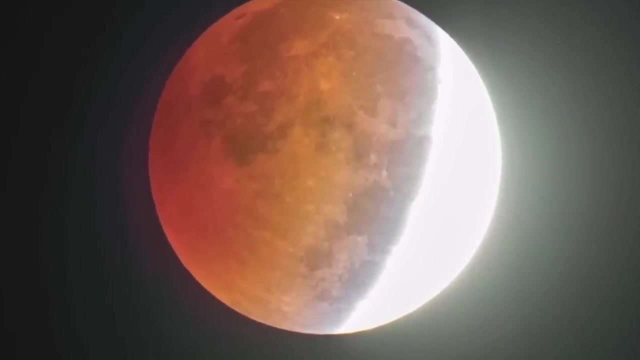 a cruise ship many years ago. It was wonderful to see In any event. so the lunar eclipse happens when the Moon passes into the Earth's shadow, And a partial lunar eclipse is when it only passes partway into what we call the umbra of the Earth's shadow. The umbra of the Earth's shadow is the 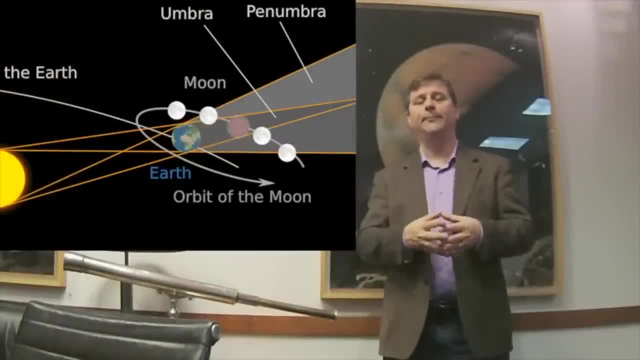 total shadow. If it passes only partially, we've got a partial eclipse. and it's a penumbral eclipse, meaning it gets partially dimmed because some of the light gets blocked by the Earth. Alright, what happens if it's on the other side and we're near New Moon? 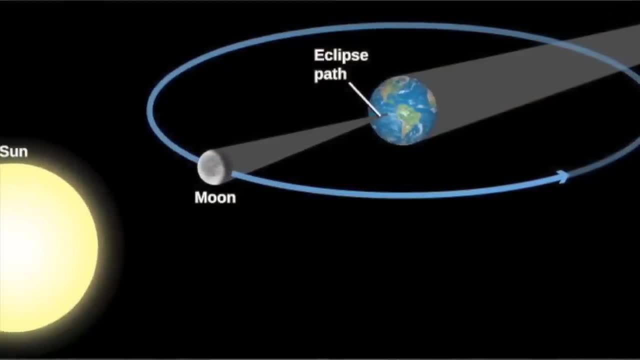 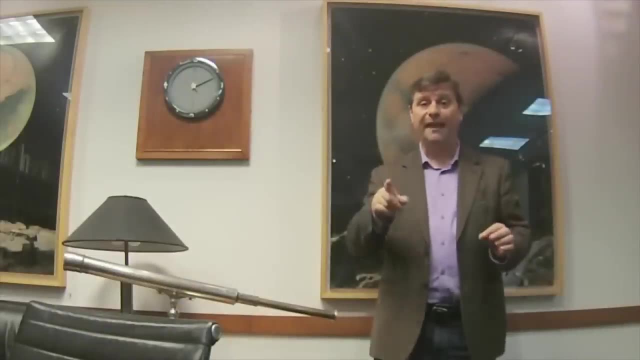 and all the lines, the intersection of the Earth's orbit around the Sun, the Moon's orbit around the Earth. they all intersect. What happens when they intersect and it's New Moon, Well then you can get a total solar eclipse. It just so happens. 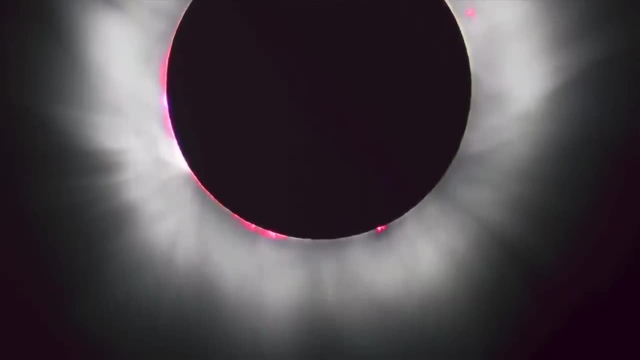 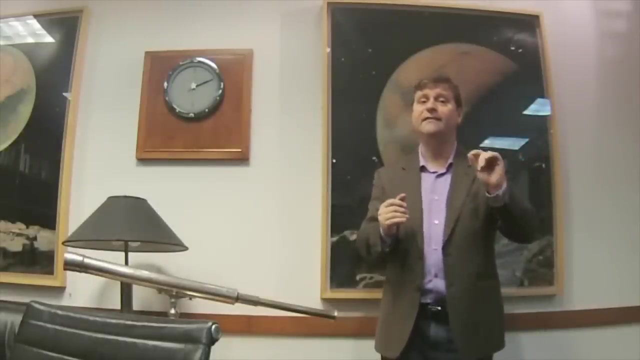 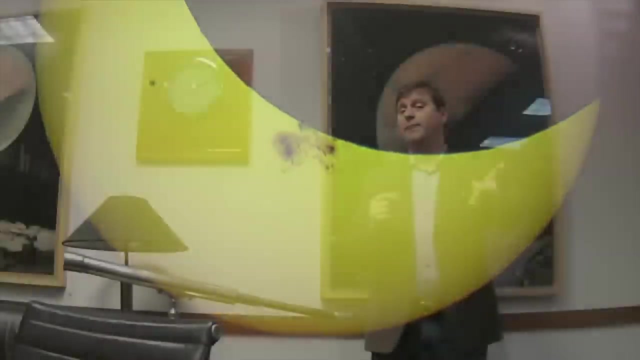 right now in the history of Earth that the distance between the Earth and the Moon makes the Moon have the same exact angular size in the sky as the Sun. The Sun's about a half a degree in size and so is the Moon, And if you want to check what I mean by half a degree, your thumb 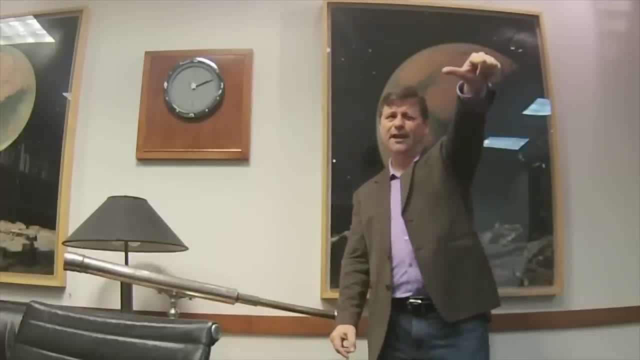 held at arm's length is about a degree. You close one eye and you look at your thumb: held at arm's length. that's about one degree, Which, if you want to know what that really means, try this: One degree and then two. 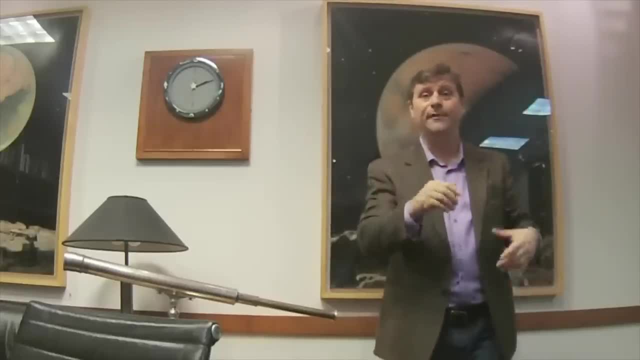 and then three, and then four, and you can go 360 times around, 360 thumbs around held at arm's length. And that means your thumb held at arm's length is about one degree. So the Moon is about half of that and so is the Sun They just so happen to be about. 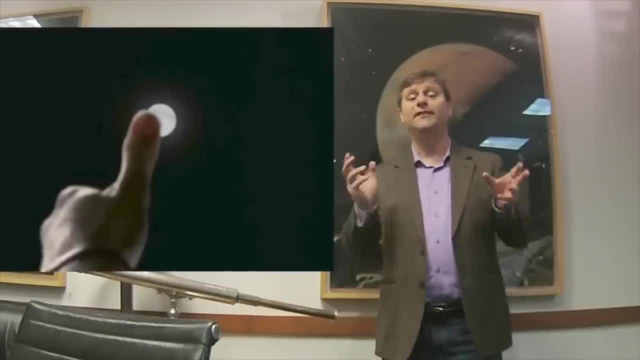 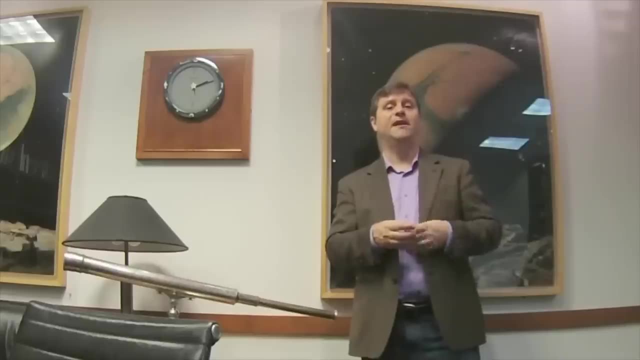 the same angular size in the sky, which means that the Moon can just completely block out the Sun, And when it does that, we call that a total solar eclipse. A total solar eclipse is when you're completely in the shadow of the Sun. Now, 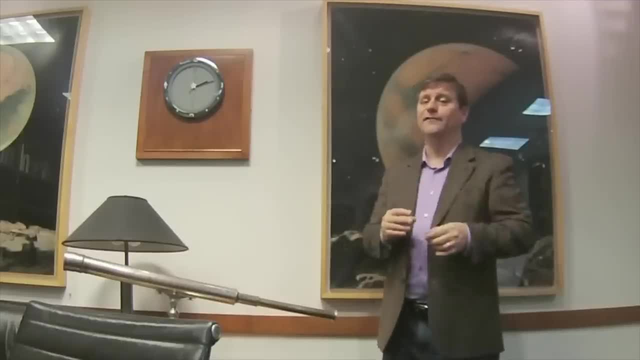 that's a very, very, very small shadow on the surface of the Earth. It tends to only be like tens of miles wide. So when the next one occurs, which will traverse across the United States on August 21st of 2017,, then you will see an amazing set of 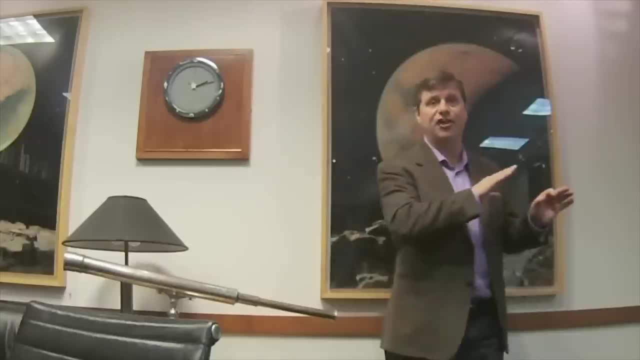 things Millions of people are going to go. try to be in the path of totality. as the shadow scoots across, As the Moon orbits the Earth and the Earth orbits the Sun, that shadow will move really quickly across the US. And if you're inside and down in the bottom of a mine and you can't do that, or 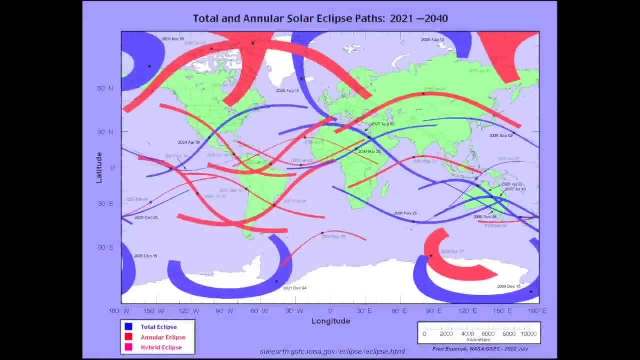 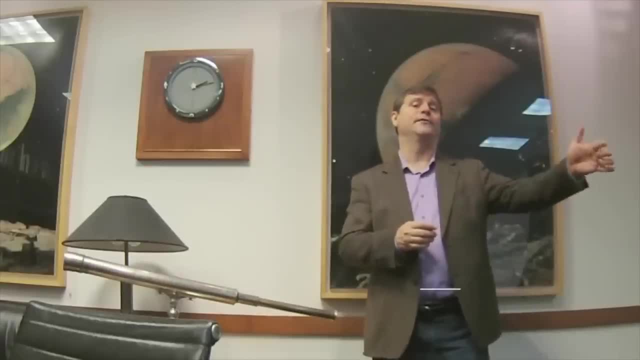 you can't break yourself away from your cell phone, then you can watch it again on April 4th of 2024.. So you'd have to wait a good seven years before you see another total solar eclipse in the United States, But there will be another one. Okay, so a total solar eclipse. 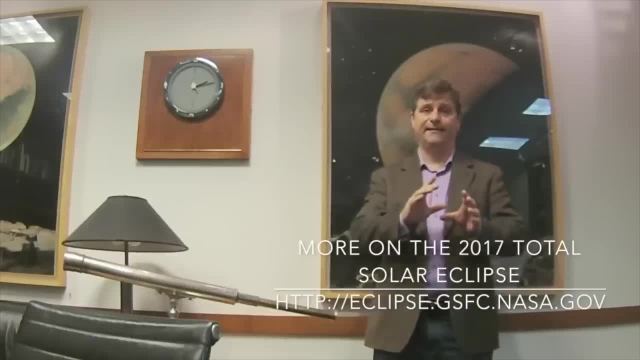 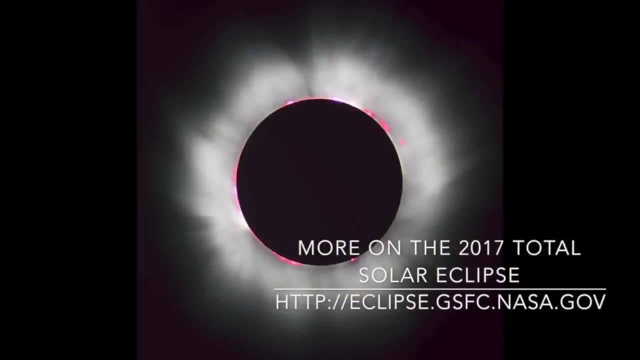 is when the Moon completely covers the Sun, And then there's all sorts of wonderful things that you can see when that occurs, such as the Sun's corona. you can see the chromosphere, all sorts of beautiful things, And, as people say, that are solar eclipse chasers, it's one. 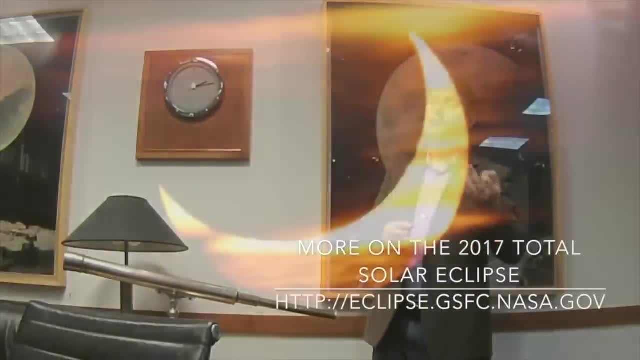 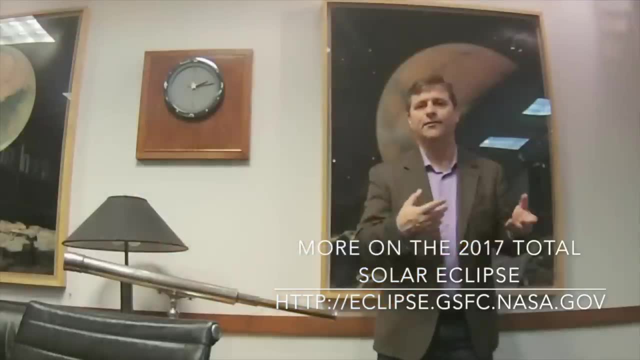 of the most gorgeous things that you can actually ever see. A partial solar eclipse is when the Moon only partially covers the Sun, and we would also call that a penumbral eclipse, meaning we only see, it's only partially inside the shadow. So a partial solar eclipse is also very dramatic. 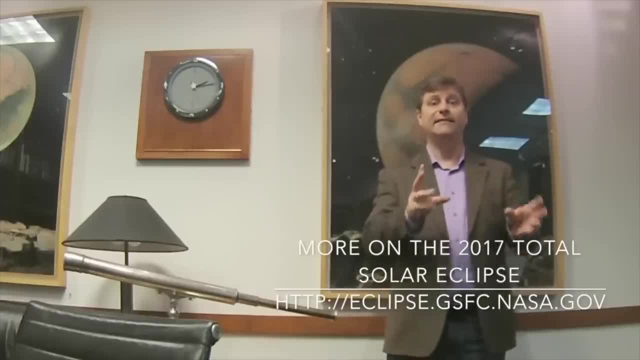 because it looks like a bite's taken out of the Sun and the sunlight dims. In fact, when a total solar eclipse happens, you can see stars in the day and creatures that normally go to sleep at night. they think it's nighttime and so they start going to bed. flowers begin to close. 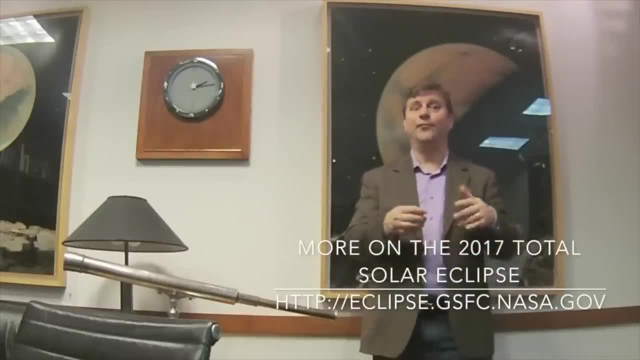 roosters crow. all sorts of strange things happen because animals think: well, it's nighttime, I'll go to bed. So solar eclipses are an amazing thing and I invite you to go. try to see one if one occurs near you. 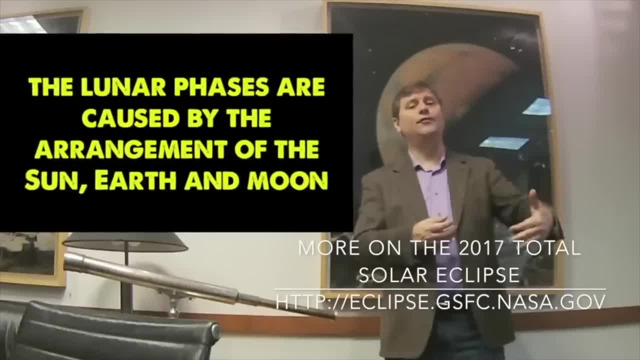 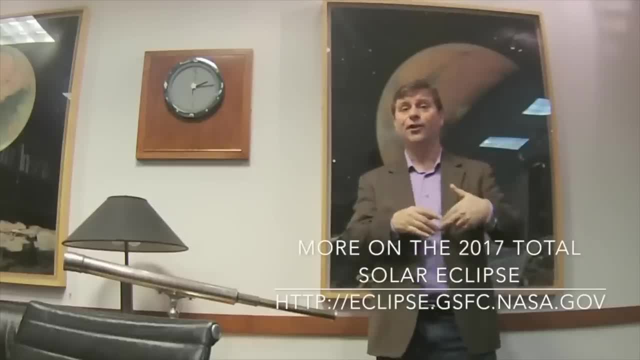 Alright, so all of these things occur only because of the geometry and relative inclination of the orbits. That's it. So the phases occur because of the position of the Moon with respect to the Earth and the distant, distant, distant Sun, and not because of the shadow. The shadow only plays a. 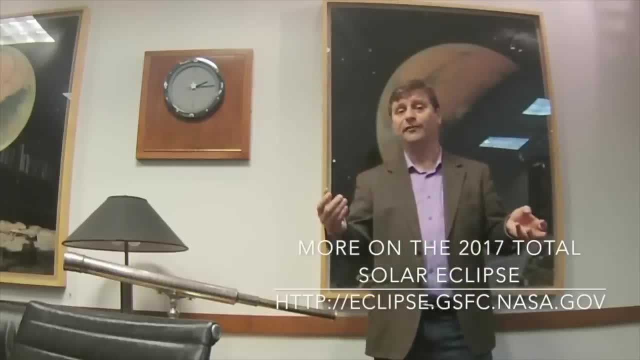 part in eclipses, and if it's the Earth, then it's the Sun. If it's the Earth's shadow on the Moon, we call that a lunar eclipse, and if it's the Moon's shadow on the Earth, we call that a solar eclipse. And there's two types of- oh, another kind of solar eclipse. 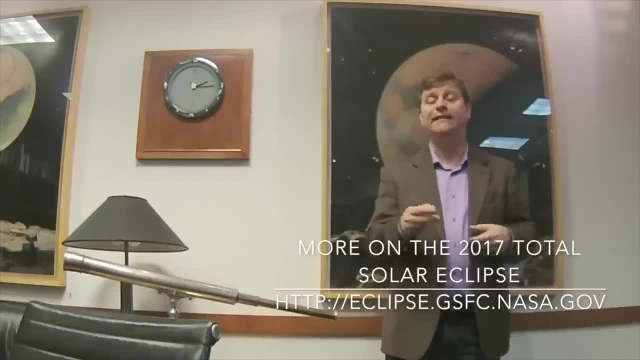 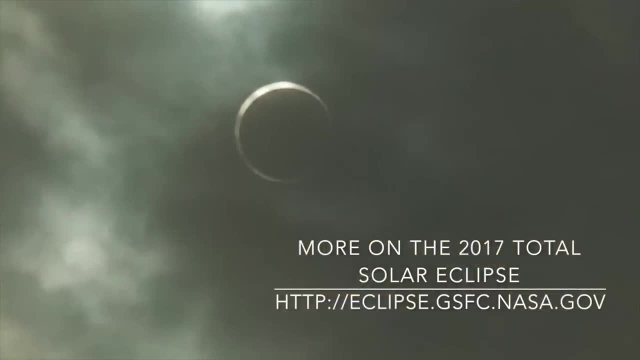 that occurs. there's another weird word for one. it's called an annular eclipse, and an annular eclipse is when the Moon is a little bit further away in its orbit than perfectly covering, so it doesn't completely cover the Sun and there's a little ring, or annulus. 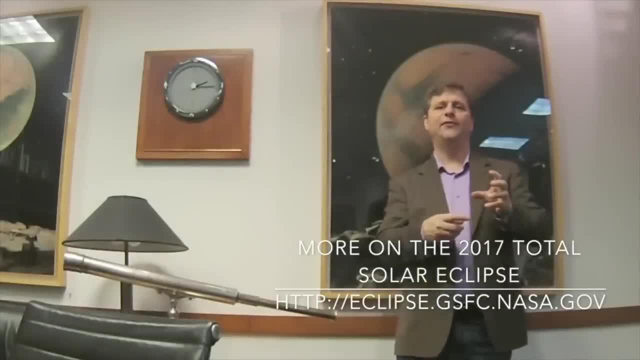 that is around the Sun, and so it's a partial solar eclipse and it's an annular eclipse, meaning an annulus where you ring around the Moon and so you see this wonderful ring and that's also pretty cool today. That's also wonderful to see. But I would suggest that, if you get a chance, 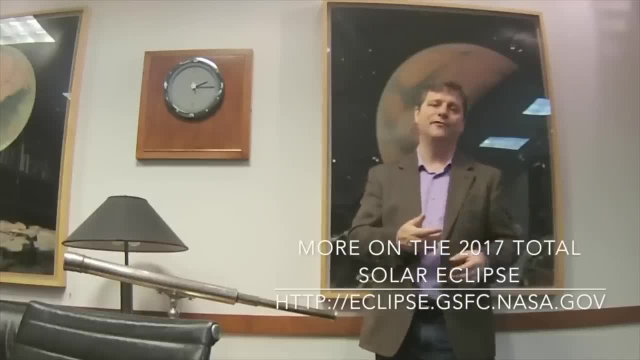 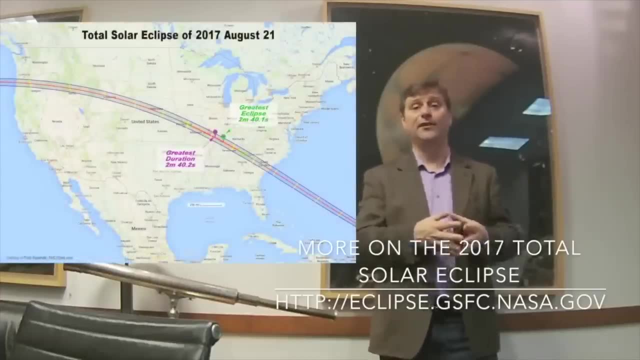 August 21st of 2017, and, if this video's still around, on April 4th of 2024,. go see that as much as you can. it's very important. These are exciting events in astronomical history and it's something you can tell your kids, grandkids, great-great-grandkids. 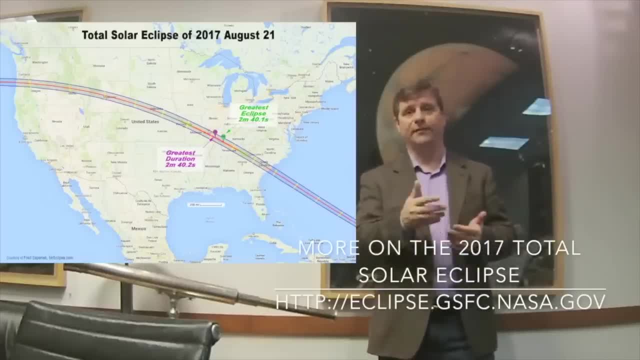 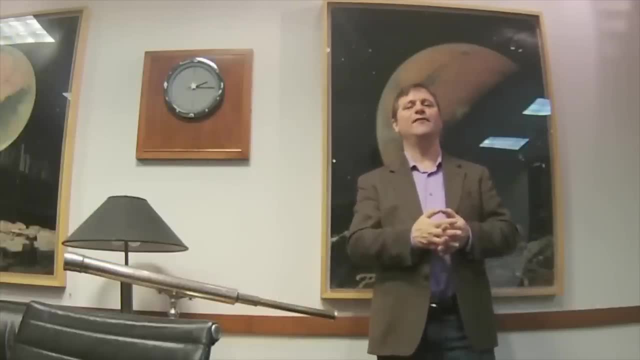 great-great-great-grandkids, and even write about and blog about or even just tweet or Instagram or what have you. Alright, so there's a bit about the motion of the Moon around the Sun and the light that reflects off of the Moon. 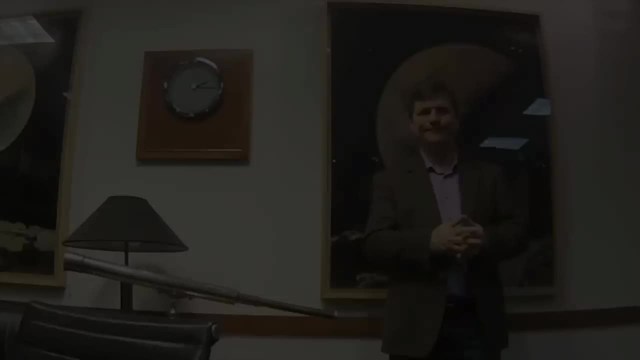 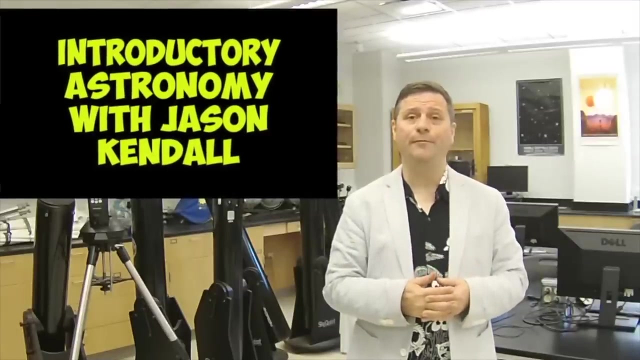 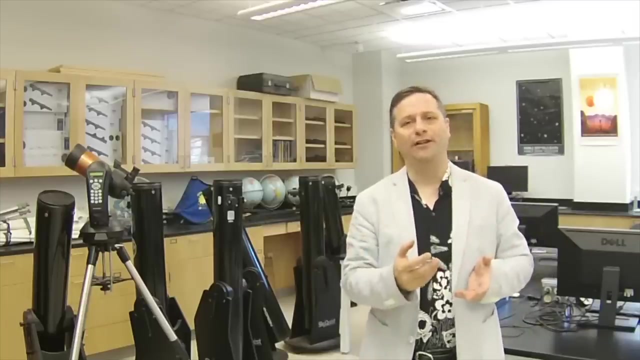 and its results. See you next time. Hello, this is Jason Kendall and welcome to my next lecture on introductory astronomy. Today we're going to be talking about distances and why they're so important and how we get them. Distances in astronomy are both extremely important and really hard. 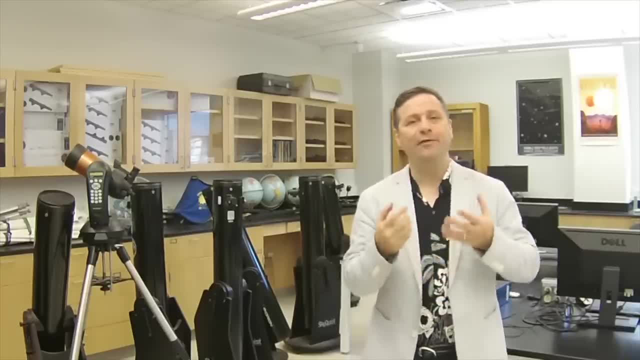 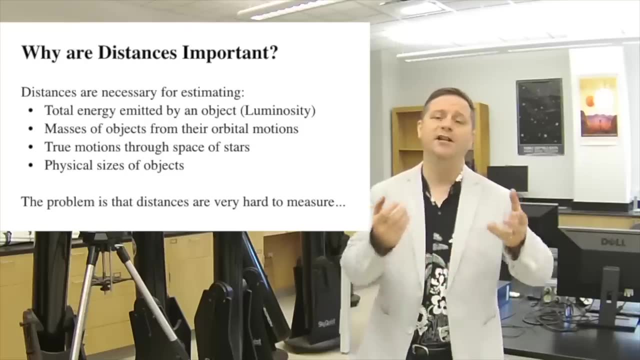 to get. So why are they important? Because if we can get the distances to stars, then we can learn more about them, such as their physical size or their luminosity, how bright they are. We can determine their masses indirectly, and then we can also determine 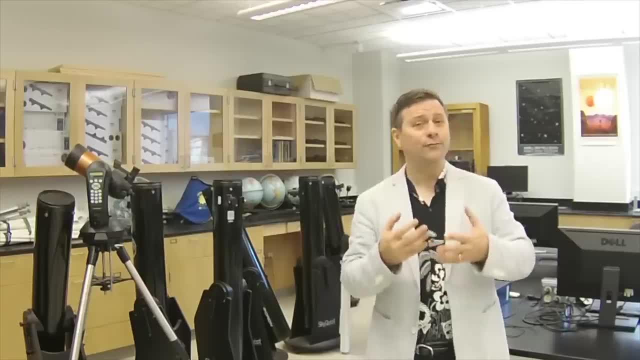 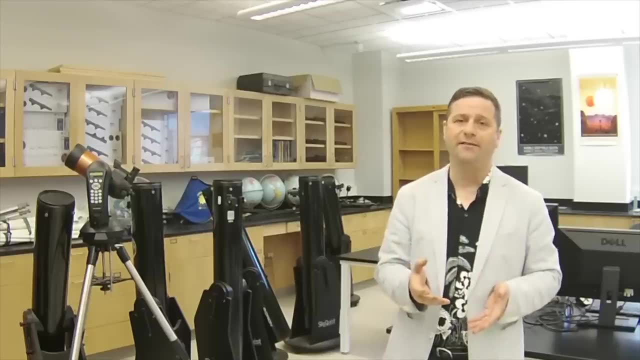 their true motion through space. So distances are really important, and if we don't actually get distances, we can't actually get many other physical parameters about stars out there. So how do we go about doing that? Because nobody's ever really been to a star. 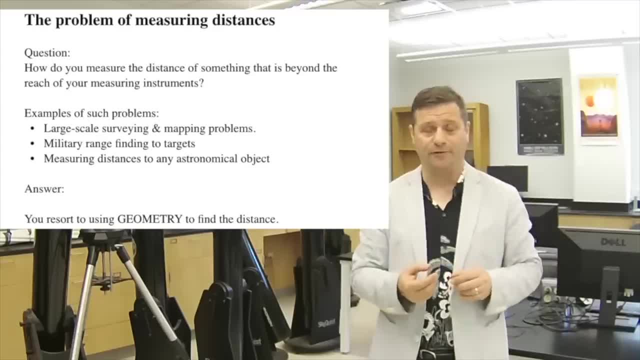 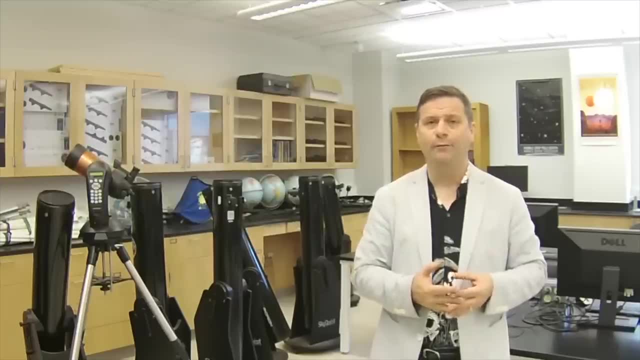 nobody's ever laid down a whole bunch of meter sticks or strung some string to another star, and even the Sun, which is extremely close, at 93 million miles closer than any other star. we haven't actually sent anybody to it because, well, they would get burned up, but it's also 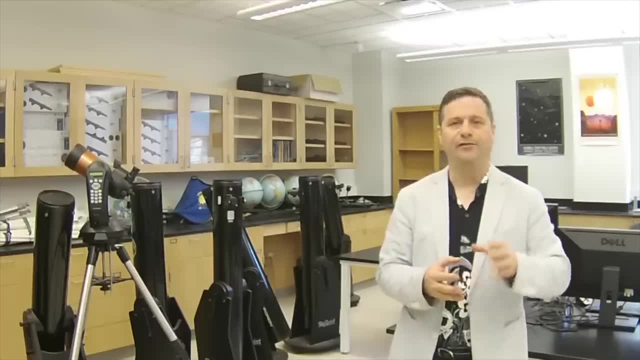 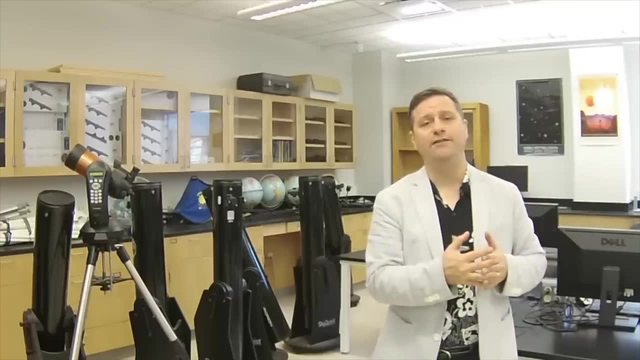 an extremely difficult project just to go into orbit around the Sun, close in for study In any event. so we've never actually been to the stars that are distant in the sky, that look like points of light in the sky at nighttime. So why not? Well, the 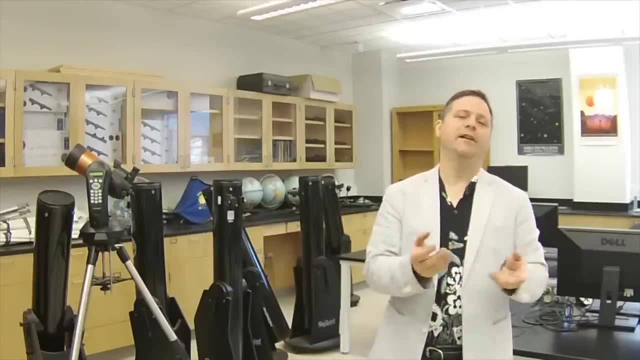 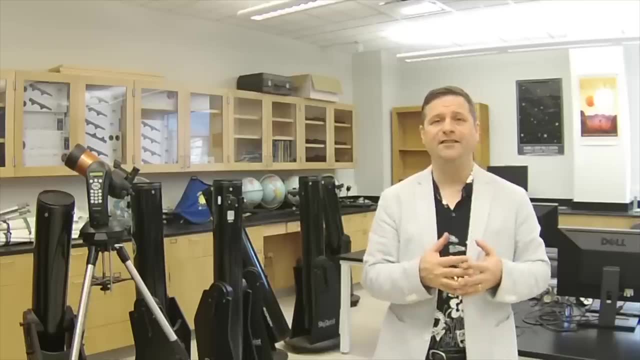 problem is that we can't actually get there by anything. we can't touch it. So since we can't touch it, we have to use geometry in order to get the distances to these stars. Well, let's actually take a first step and see how we use geometry to get. 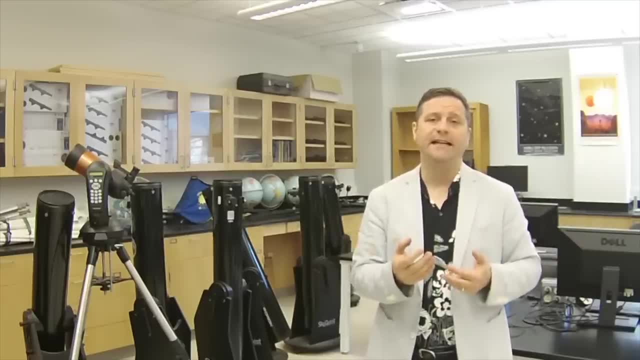 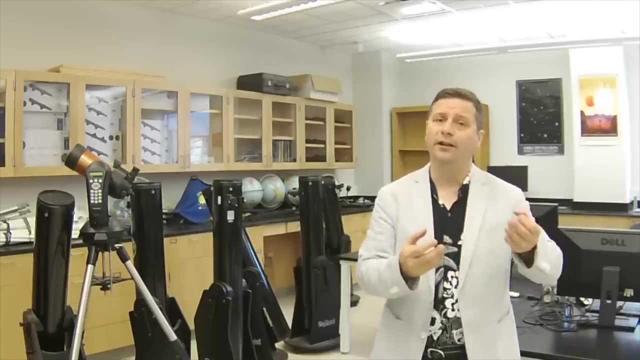 distances. One of the more simple ways we can think about it is that it's done pretty much all the time by surveyors. Surveyors use the process of trigonometry and they use triangulation in order to get distances to these far stars. 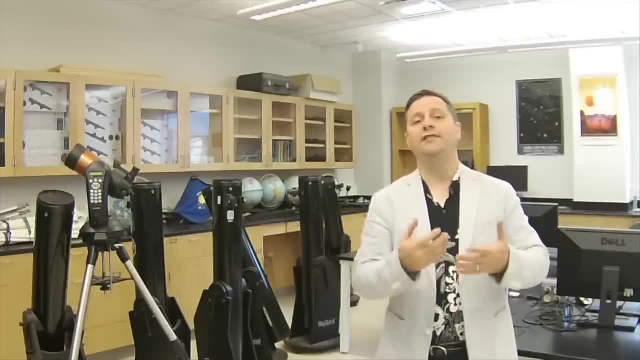 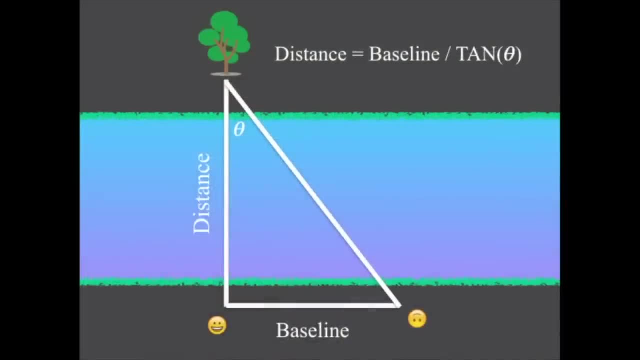 Well, how do they do it? Well, let's pretend that we're trying to measure the distance across a river and maybe we're on one side and there's some significant tree on the other side. so we look at that tree and we say, okay, well, how far is that tree across the river? Well, let's say we 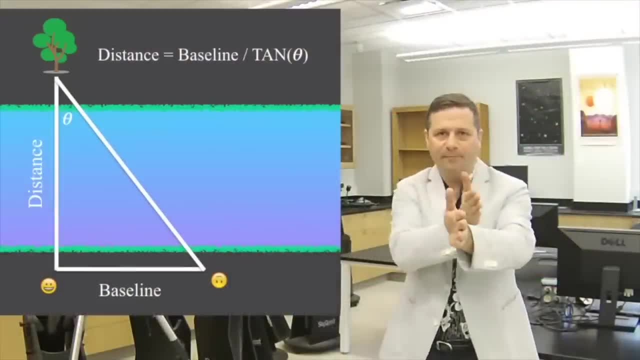 can then say we'll be on one side and let's say we find the place where it looks to be the closest across, So we'll call that our starting point, and so we'll look straight across the river so that it's 90 degrees to the shoreline, and so 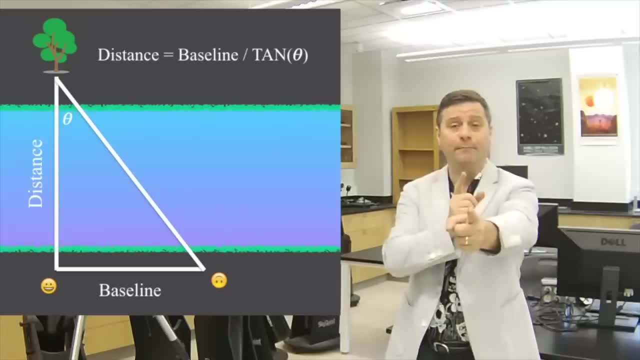 we'll start with that and we look straight across the river and that's our distance we want to measure. We want to measure the distance from that starting point to the tree across the river. Okay, so we plant a flag and we point a little arrow. 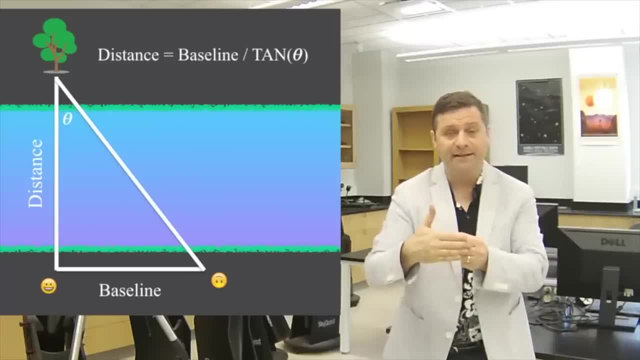 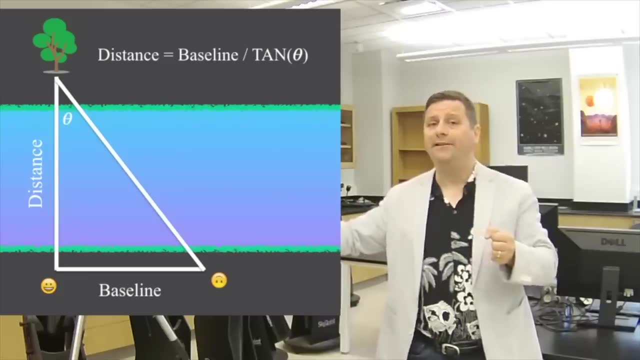 and we make a mark on the ground that says this way to the tree, and then we make a 90 degree angle like that, and then we walk, say 200 yards away, along that 90 degree angle and look across again to the river. 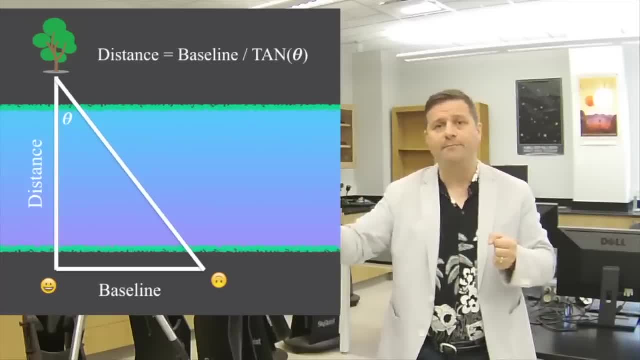 Now, here we're pretending that the river might be a couple, maybe a mile or so across. so the tree: you have to use a little telescope in order to see the tree, whatever. but the point is you've got to walk maybe 200 meters. 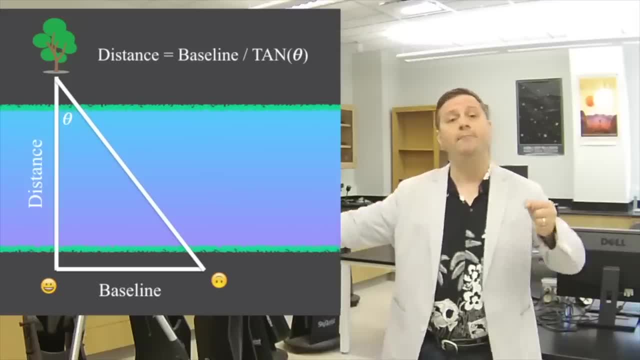 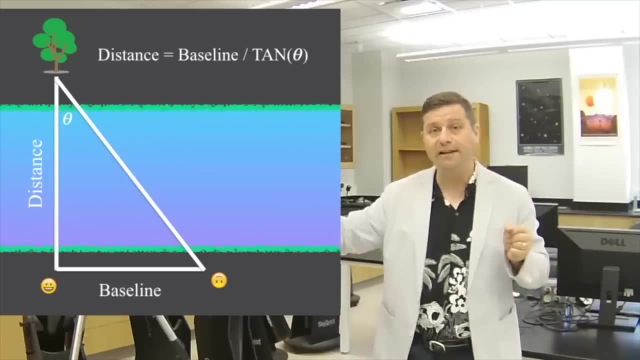 or 200 yards up the stream to create what we call a baseline. So when you get to the other end of the baseline you put down your little telescope again and sightline all the way to the tree again. you find it and you find. 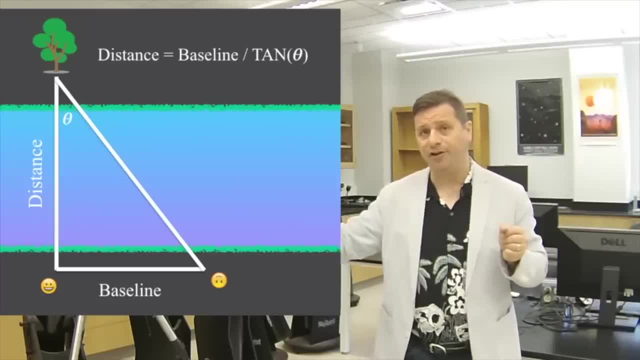 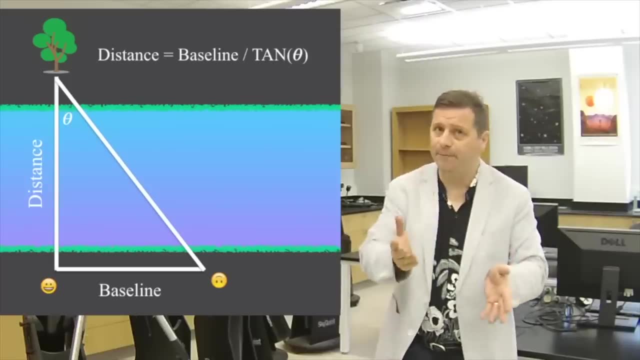 that the angle between the sightline at the second location and the baseline is not 90 degrees. It's less than that. So, in the very simplest way, we simplified it just for that, because it's never this simple in real life. but we're trying to make it really simple so the idea gets across. 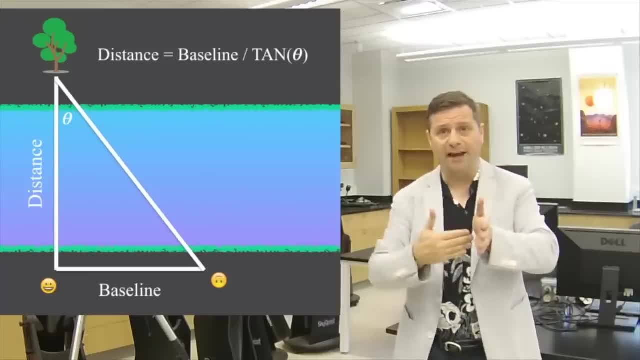 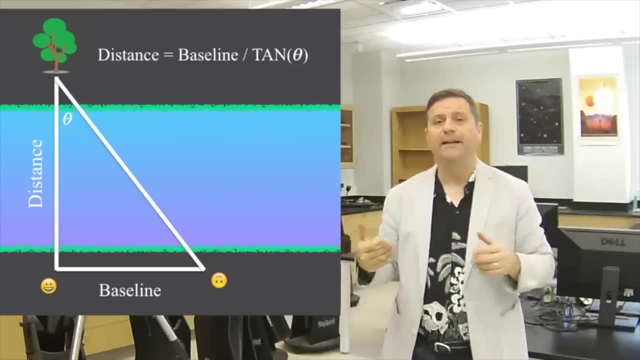 The idea is that you now have a right triangle where it's 90 degrees here, less than 90 degrees there, and some small angle between the two sightlines at the tree, So that the sum of all the angles inside a triangle is 180 degrees. so let's say this is 90,. 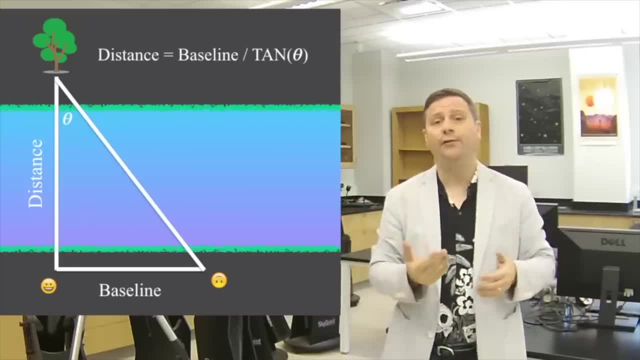 the other sightline, say maybe, is 85, and so the angle between the two sightlines at the tree is 5 degrees. So how do we get that distance? We use simple 9th grade geometry and trigonometry class stuff and we say the baseline divided. 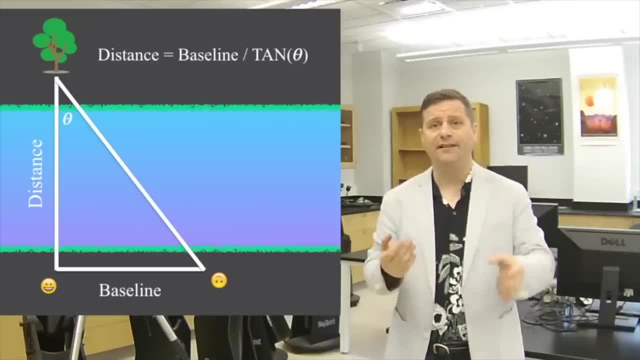 by the distance across the river is equal to the tangent of the little angle that subtends the two sightlines. That's just the opposite over the adjacent, in the old way of thinking about it, where the opposite is the baseline, which is opposite the little angle that subtends the two lines. 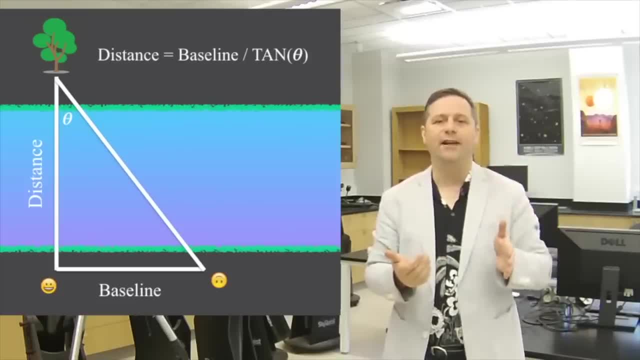 from the tree and the adjacent is the side of the triangle adjacent to the that we're trying to measure. We ignore the hypotenuse because the hypotenuse is not the adjacent angle. it's called the hypotenuse, Alright. 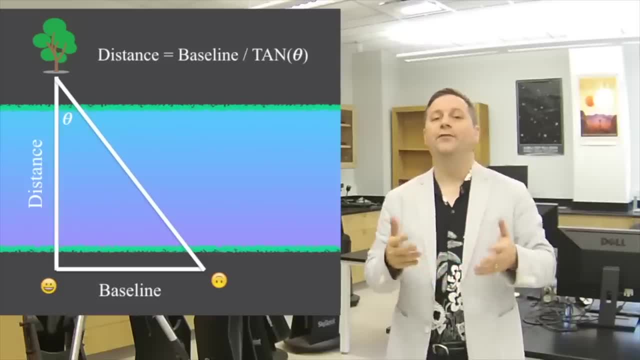 So the opposite over the adjacent equals the tangent of the angle. so therefore the distance across is simply the baseline divided by the tangent of that little angle, which might be 5 degrees. So that gets us our distances across a river. But that's the basic. 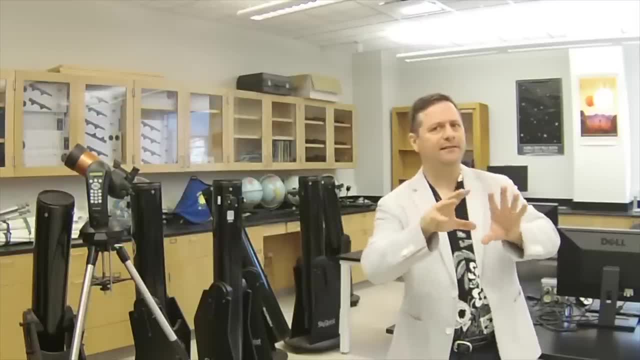 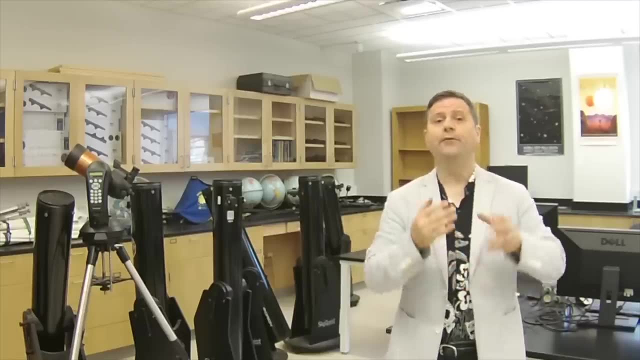 idea. but now let's pretend. when we looked at this thing we said okay, so maybe when we were across the way the tree was. the reason we picked that tree across the river was because it was standing in the middle of a field. 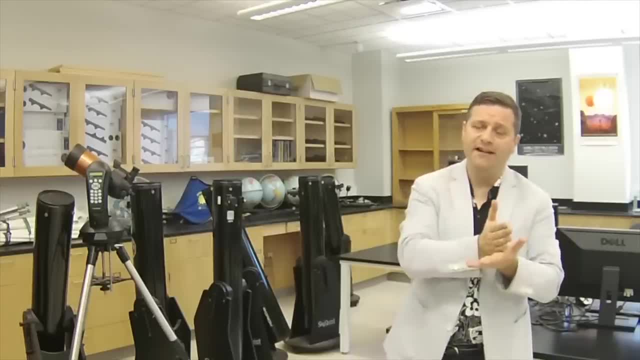 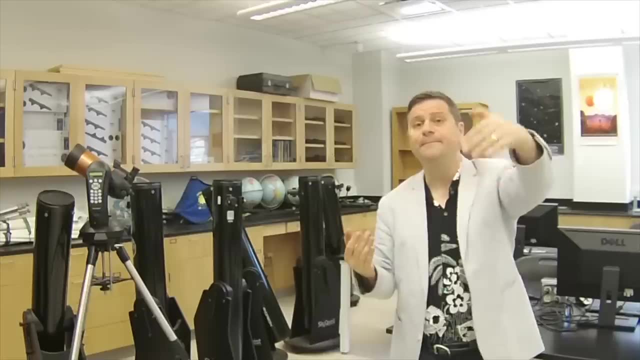 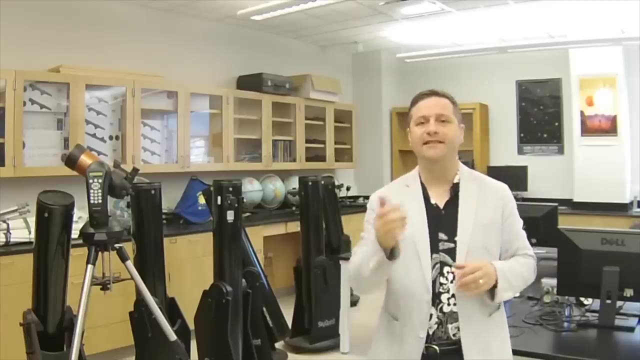 and there were a whole bunch of things behind it. So when you went from one place on the baseline to another, the tree, the things that looked like it, shifted with respect to the background stuff across the river, And that shift we call parallax. So what is parallax? A better way of thinking about parallax is: 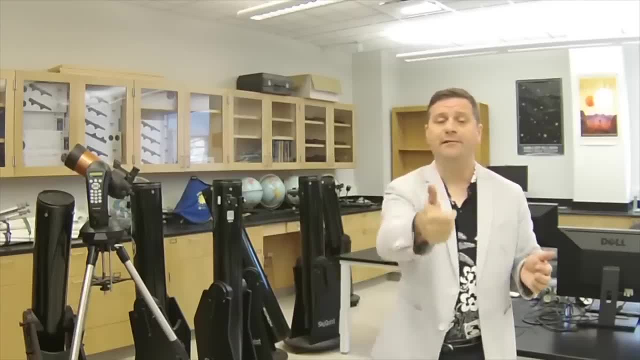 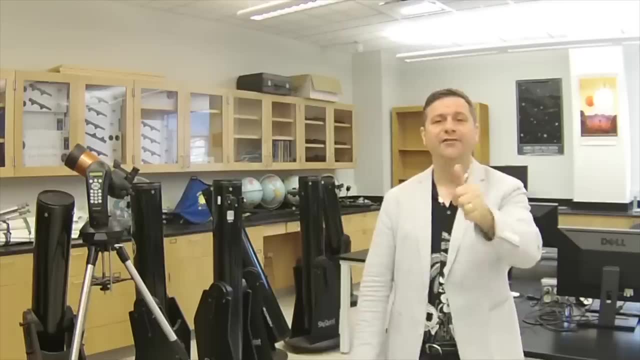 let's make a really easy thing that you can do right here at home. What you do is you take your thumb, Take your thumb at arm's length and you bring it close to your face and then you blink your eyes left and right, back and forth, and you see that your thumb apparently 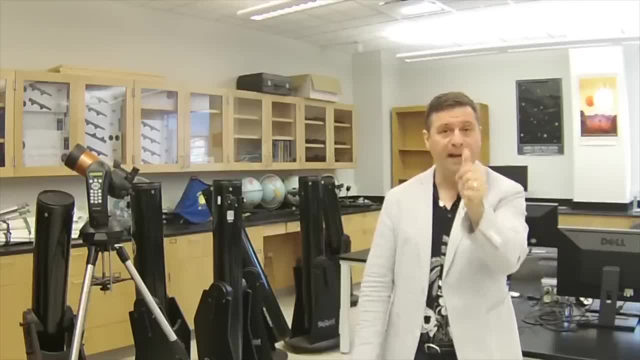 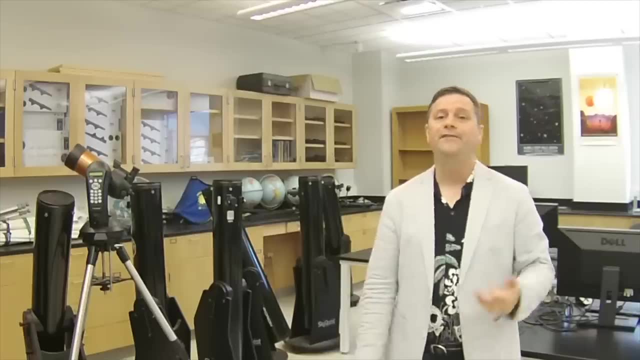 jumps left and right. Now, if it's close the jump is big, but if it's far, the jump is smaller. And if it's really far- let's say you stretch your arm out or look at somebody else's thumb- then the jump is really small. So parallax. 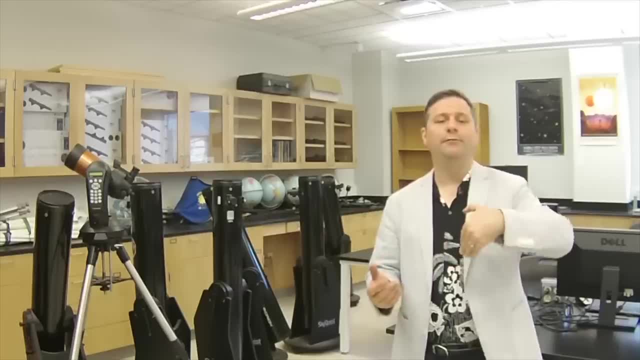 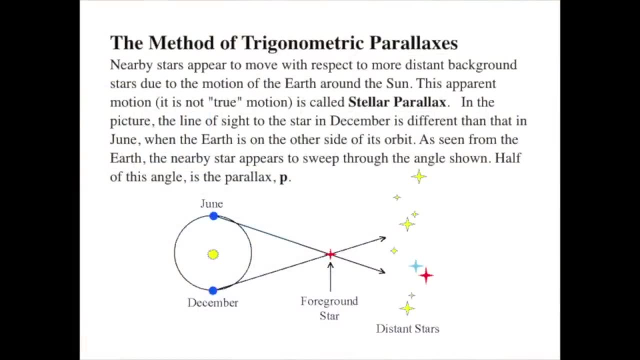 is the shift that you see with respect to background things when you change the angle, the place from which you're observing. So stellar parallax will then be well with the parallax that we see with respect to background stars. So maybe there's some close stars, some close foreground stars and some really far. 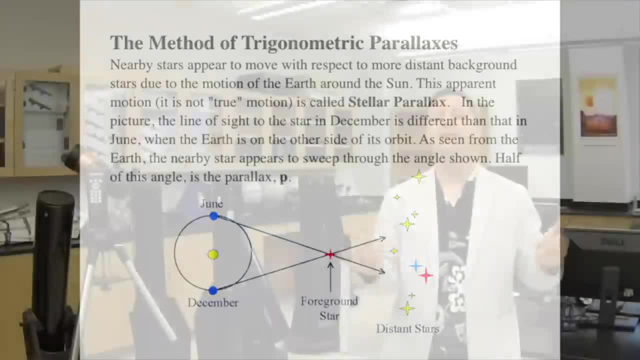 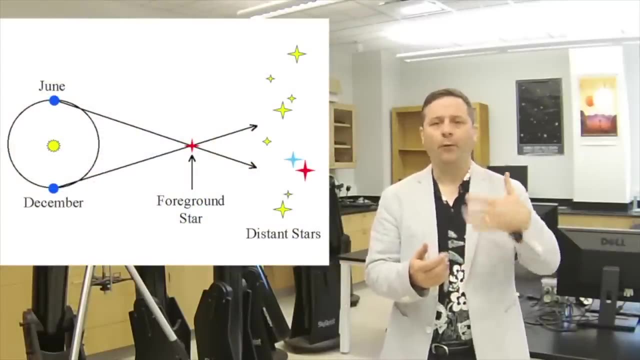 distant stars. And you know, stars are apparently distributed in space, so why not? And that's the case. That is the case. There are some nearby stars and some far stars, So what exactly is the parallax for stars? Alright, so if we have some nearby stars, 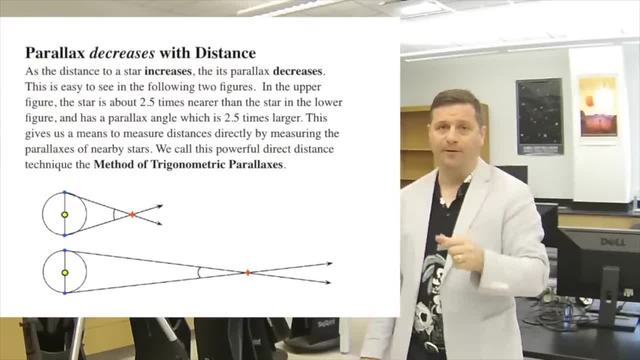 they will have a big parallactic shift and if they're far they'll have a smaller parallactic shift, And the farther they are, the greater the parallactic, the less the shift is, until it gets so far that it's imperceptible. 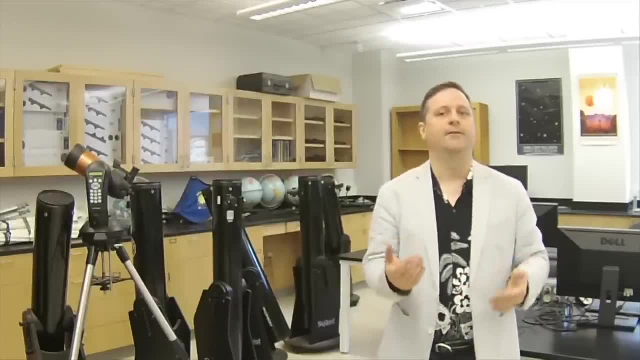 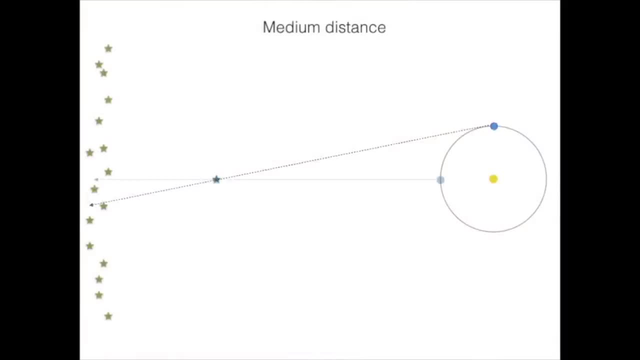 Or incredibly imperceptible. But what's our baseline? Okay, The baseline for looking at stellar parallax is the orbit of the Earth around the Sun. So as the Earth goes from, say, December around the Sun to June, we have two different vantage points And these vantage points are separated. 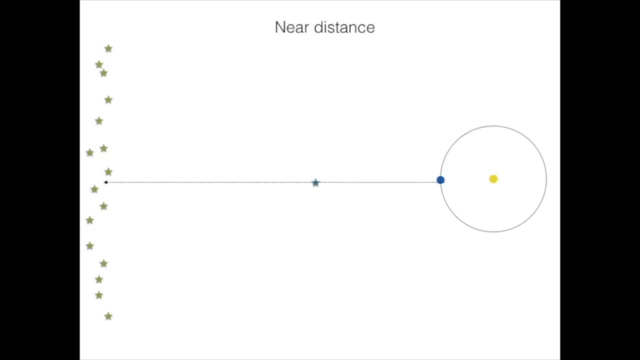 by a distance of 300,000, 300 million kilometers Or 180 million, So 93 million miles, 180 million miles. the radius of the Earth's orbit is 93 million miles, or about 150 million kilometers, So the diameter of Earth's orbit is about. 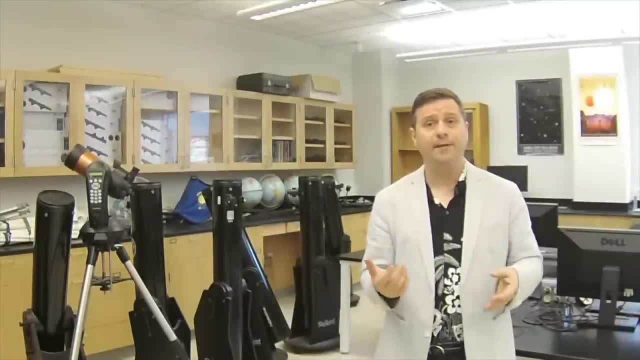 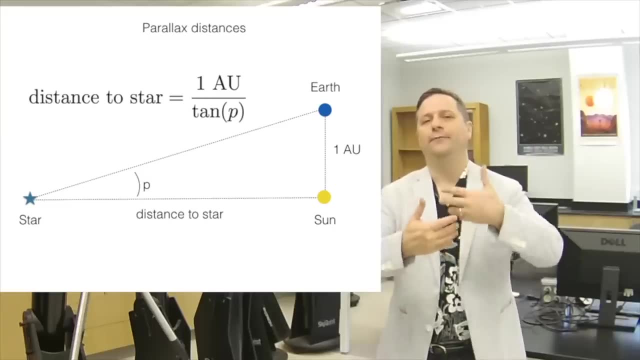 300 million kilometers, Which is a really big baseline, But it's just barely enough for us to get the distances to the stars. Okay, So how do we get that? So what are we talking about? Okay, So, this little angle. we're going to make a new definition, The angle that we're going 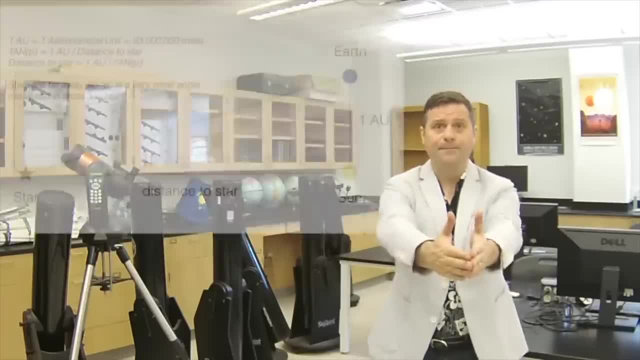 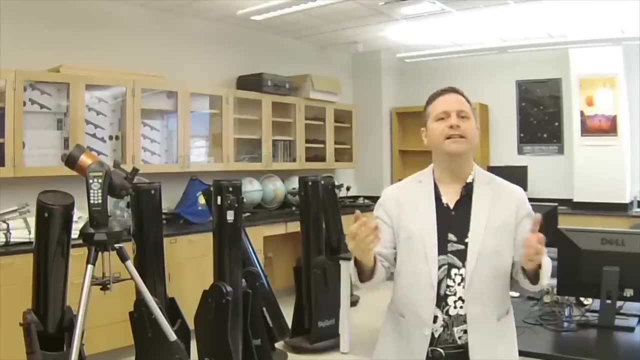 to call the parallactic shift isn't the full angle, It's half the angle. So we're going to make this angle with respect to the center of the solar system, which is the Sun, Kind of weird, but that's how we're going to define parallax Half of the shift. 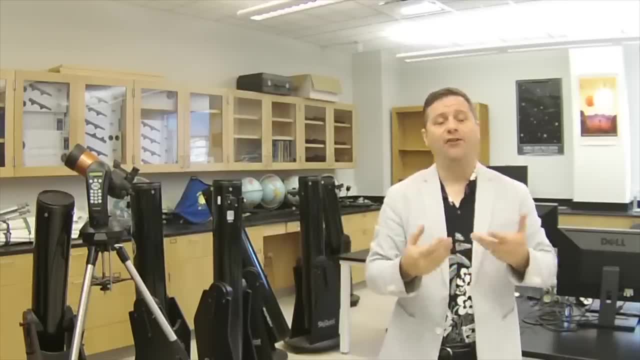 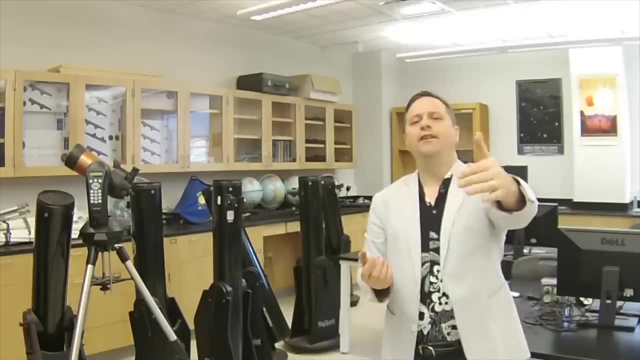 that we see from, say, December to June. Okay, So parallax is our fundamental measurement. So how do we do it? Okay, So, when we measure these things, what is their size? The size of a typical parallax is very, very small. 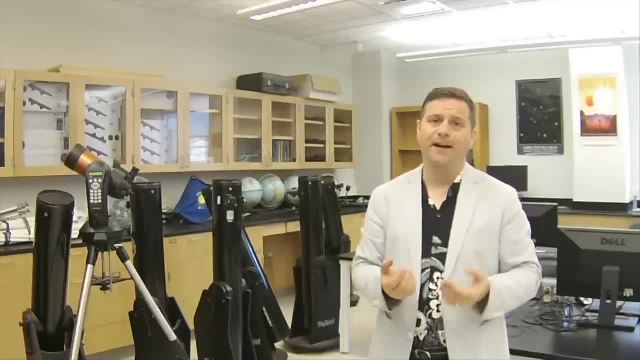 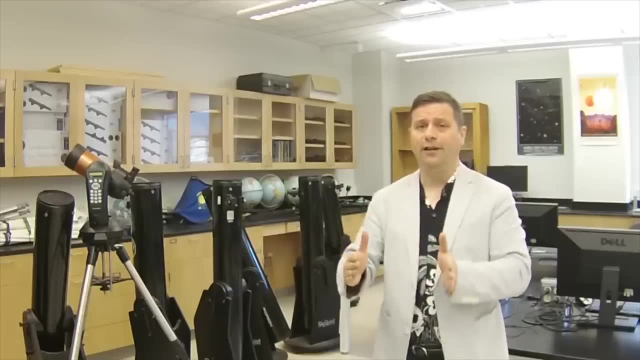 for the stars, The size is on the order of an arc second. That's a really small measurement. So with the baseline of one astronomical unit which is 93 million miles the length, the triangle is extremely narrow And it goes out very, very far. It goes out to one arc second. 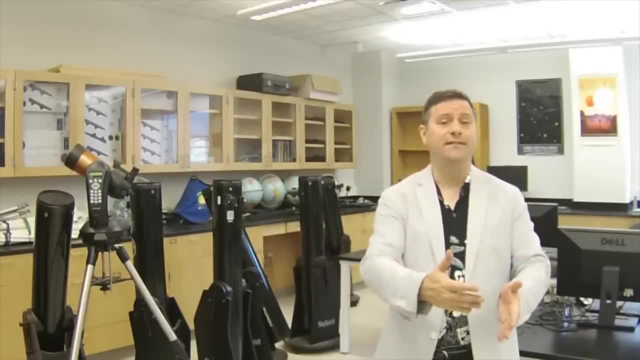 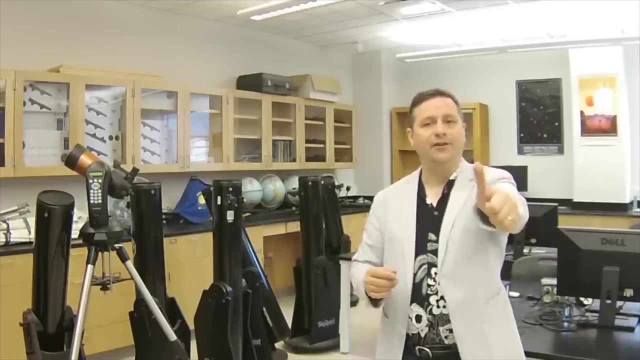 Alright. So instead of with our tree example, it might have been five degrees. So what's an arc second? Alright, So an arc second is the following: Let's take your thumb and take it at arm's length again. We'll do that whole trick. 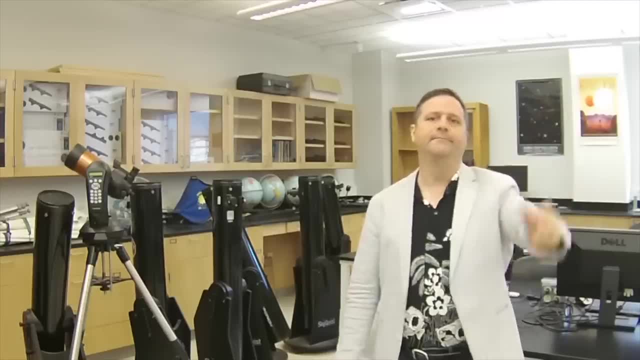 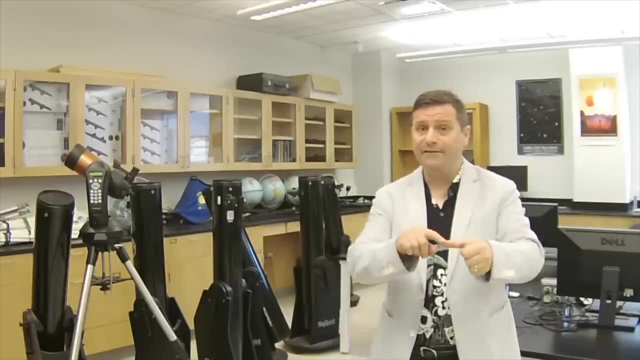 again A lot of tricks like this that keep up with thumbs and hands. This is backyard astronomy. Okay, So your thumb held at arm's length is about a degree across. Now if you make 60 even marks across it, those would each be one arc minute, So every degree. 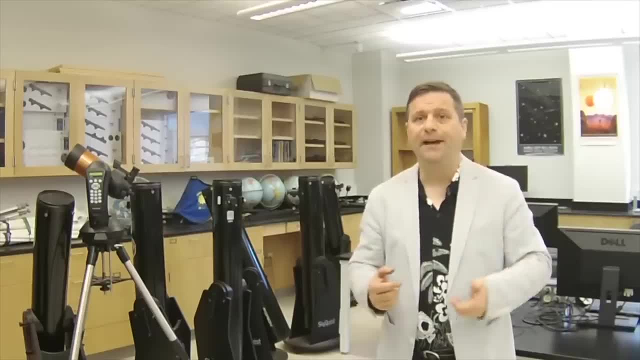 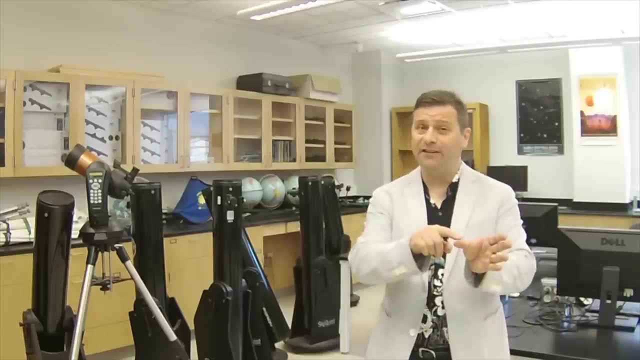 can be broken up into 60 arc minutes. And guess what? Every arc minute can be broken up into 60 arc seconds. So imagine that you took 60 marks across your thumb- little tiny marks like on a ruler, and then, in between each of, 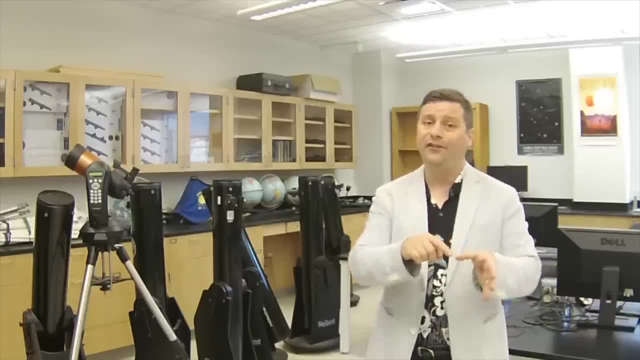 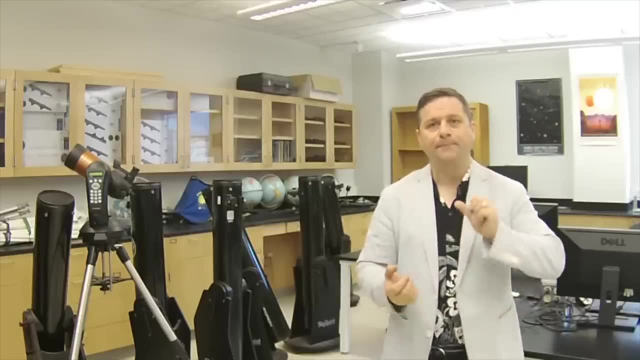 those marks, you put 60 more marks, So there would be 3,600 little marks across the back of your thumb. That's a lot of little marks and I'm sure it would be a mess. but hey, it's all for science. Okay. So what's an? 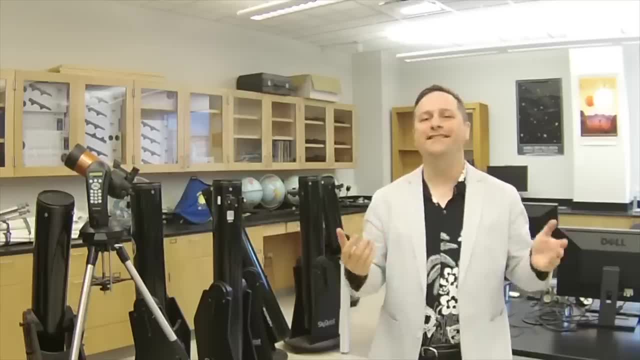 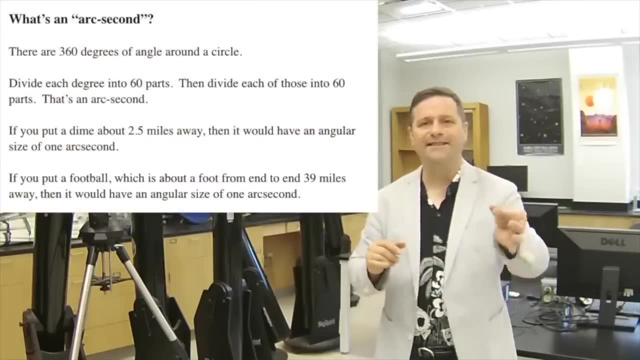 angular shift of one arc second. Or how big is something that is one arc second? Well, take a dime and place it about two and a half miles away. That's the size of one arc second. Or take a football, you know. 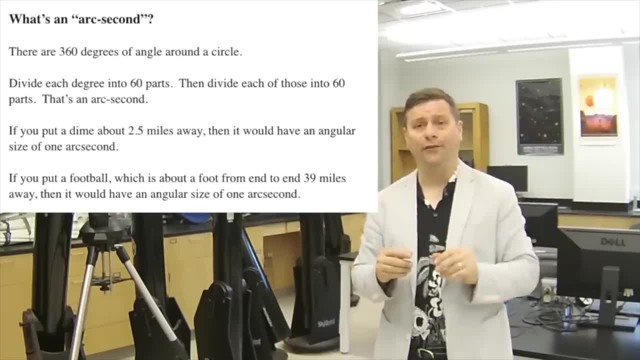 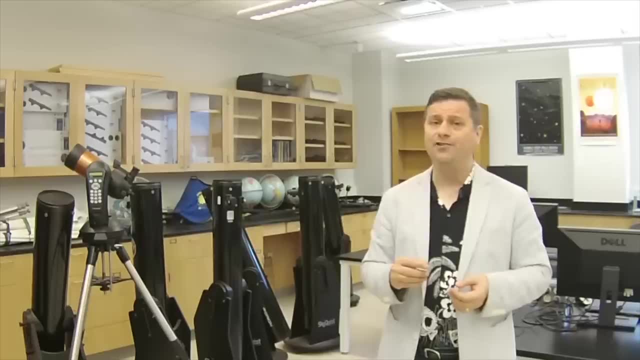 NFL football and you place it 39 miles away. That's about one arc second. An arc second is a really small angular measurement. The typical things when you look at the moon say: when you look at the moon, the moon's about half the size of your thumb. 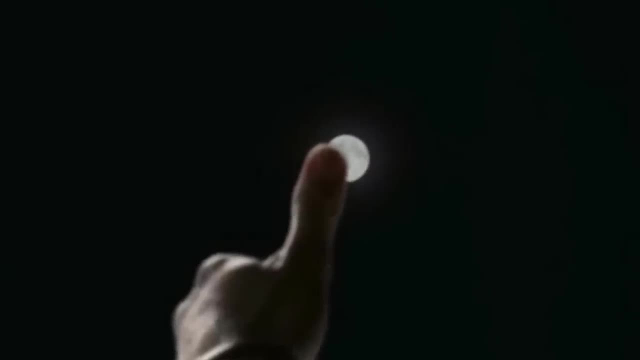 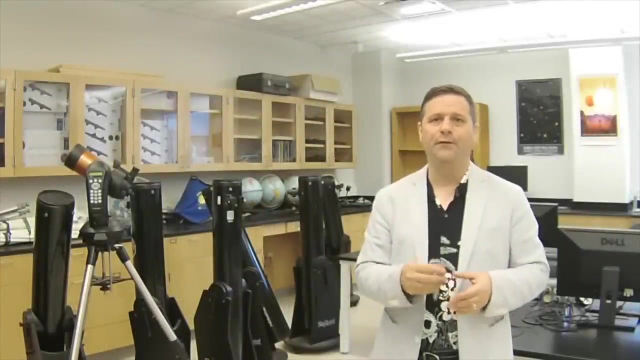 the standard size of things that you can see on the moon without the aid of a telescope are about five to ten arc minutes, So you're looking at things that are incredibly small angles, so arc seconds are really, really tiny. Alright, So what kind of parallaxes do we see? 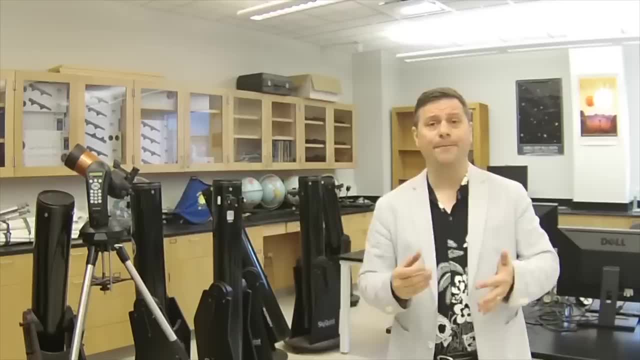 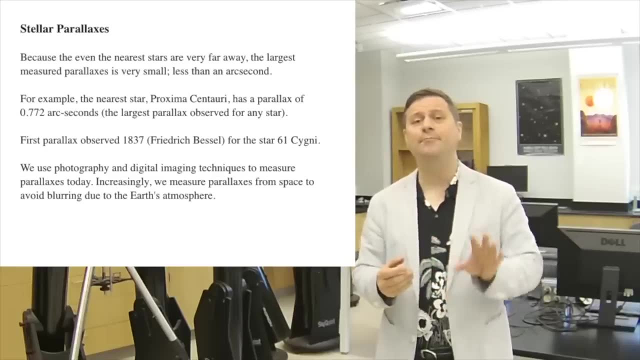 for stars. In fact, no star that we see in the sky has a parallactic shift that is greater than an arc second. Every star has a parallactic shift less than an arc second, And the biggest parallactic shift is for. 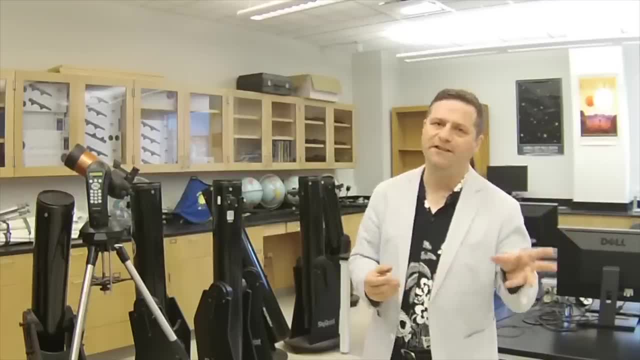 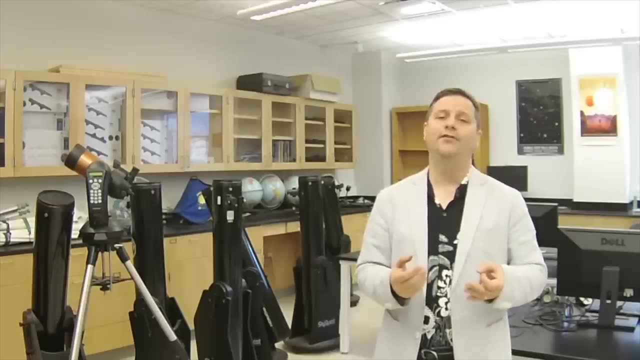 Proxima Centauri, which is about three quarters of an arc second- .77 arc seconds to be specific, And that makes it have a distance of approximately 1.3 parsecs. We'll get to that in a second, But really, let's actually kind of go back and see how tough this. 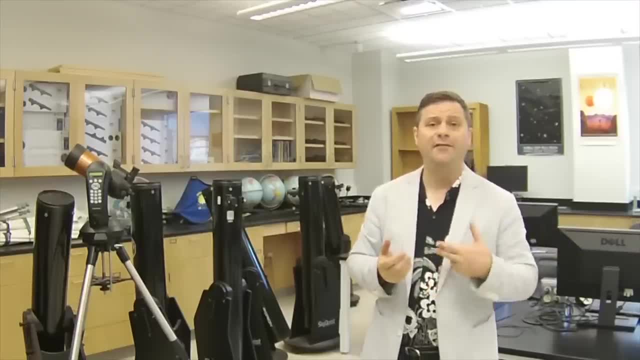 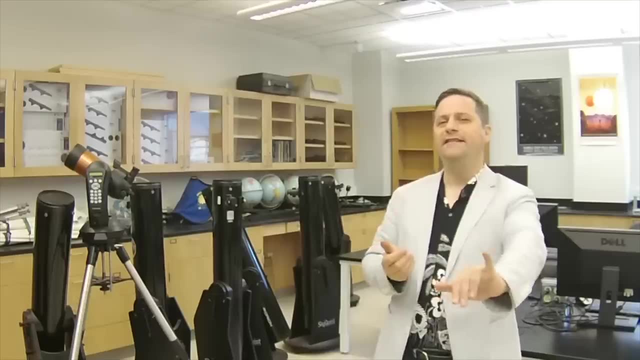 thing is, In fact, its parallaxes are so difficult to measure that the first one was only measured in 1837, 61 Cygni, which is a nearby star. Alright, So how far are these things when we say, let's see what we mean by the distances derived from parallaxes. 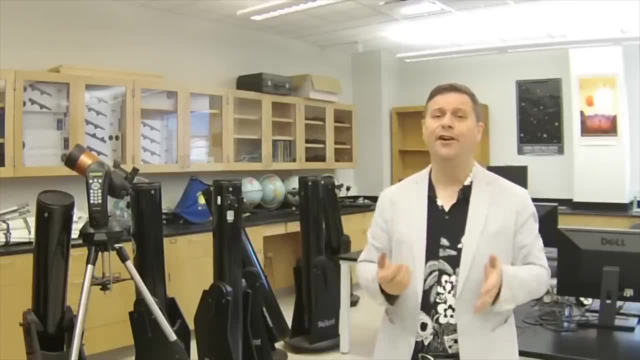 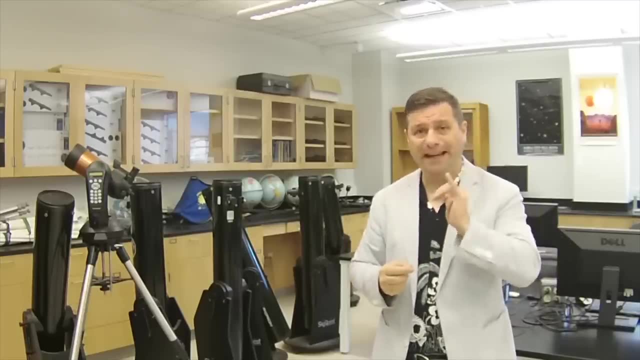 If we look at Alpha Centauri and say how far it is based on that triangulation method, if the distance between the Sun and the Earth was the width of your pinky, then the distance to Alpha Centauri is about 1.7 miles. 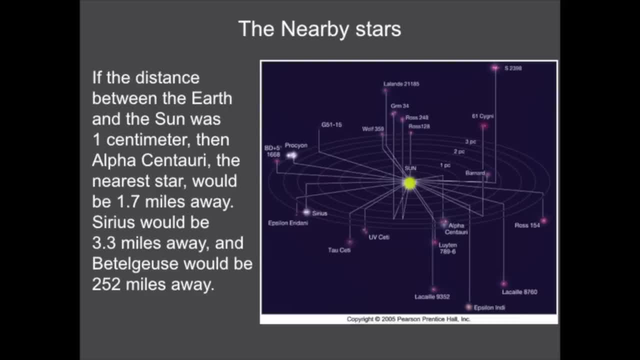 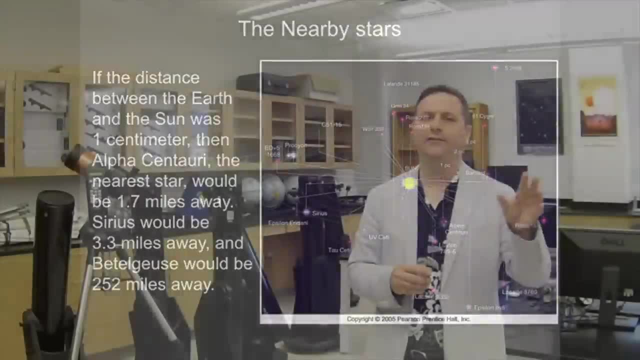 And the distance to the brightest star in the sky, Sirius, is about three and a third miles, And Betelgeuse, which is that star in Orion that everybody says three times just for fun, Betelgeuse is 250 miles away. So 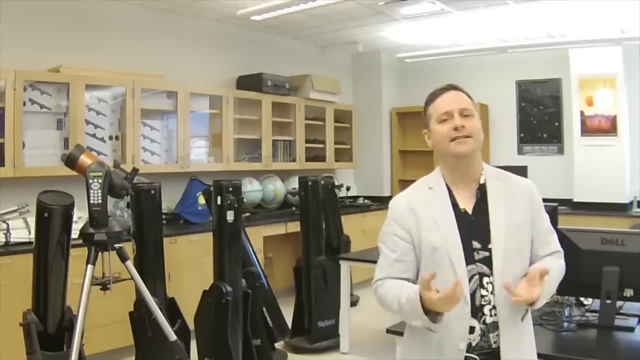 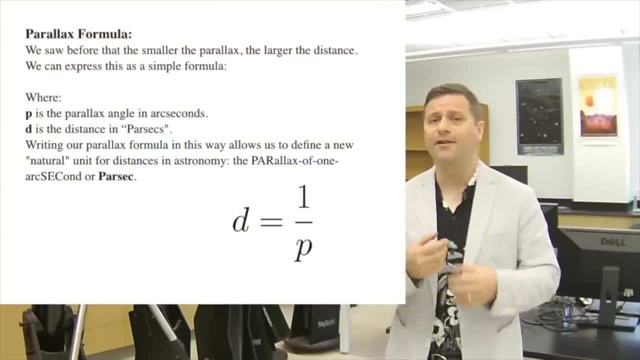 where did that distance come from? Well, we derive a concept called the parsec. If a star has a parallax of one arc second, then we define its distance to be one parsec. That's what it means. Parallax of one arc second, a parsec, That's what parsec stands for. 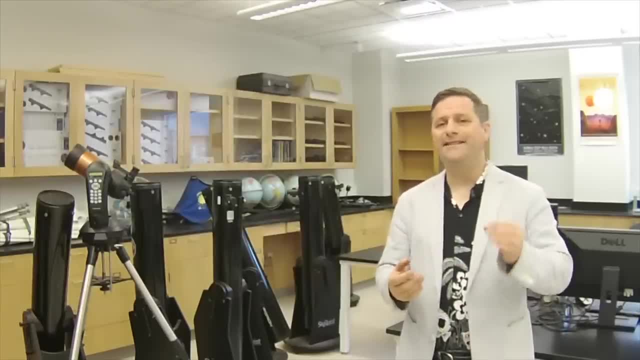 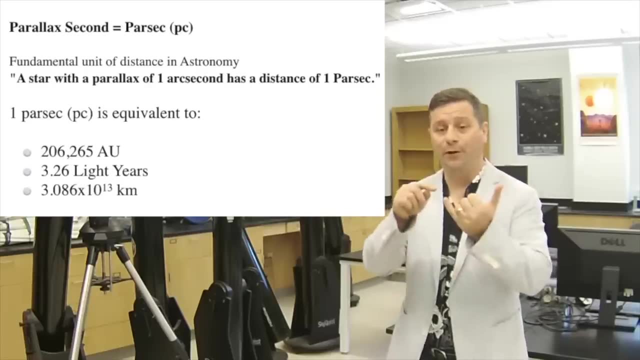 So what's a parsec? A parsec is the same as 206,265 astronomical units. So one astro- pretend- one astronomical unit is the width of your pinky. That's 93 million miles. now, Now take 206,000 of those. 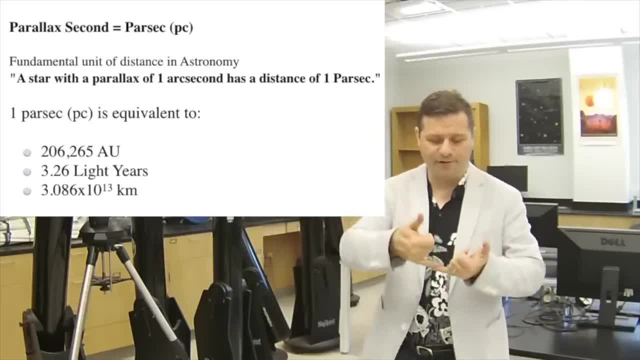 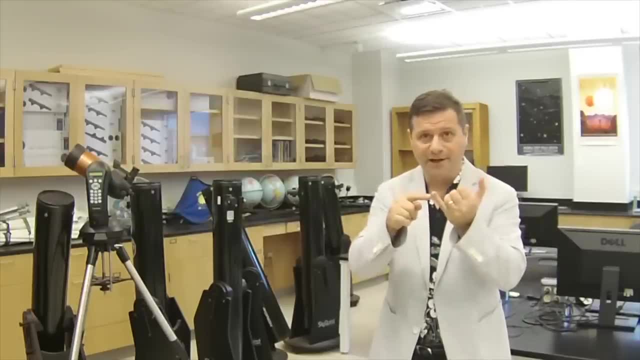 That's a long ways out. So make 206,000 times your pinky going left and right and that'll get you to the next star, Assuming that the star is 206,000 miles away. The Sun is here and the Earth is there Now on this size scale. 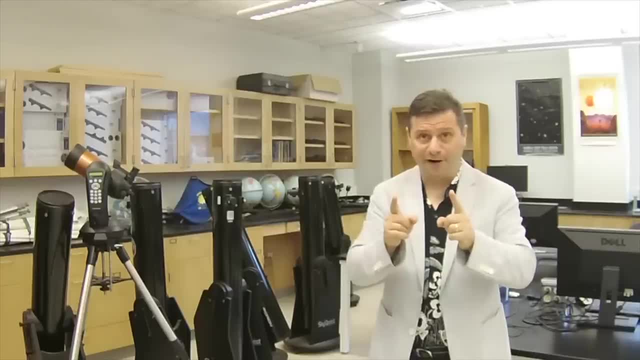 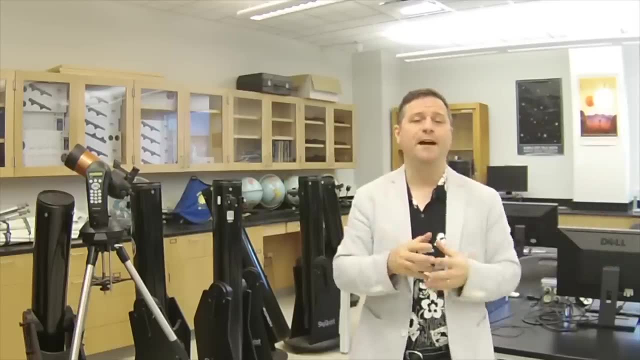 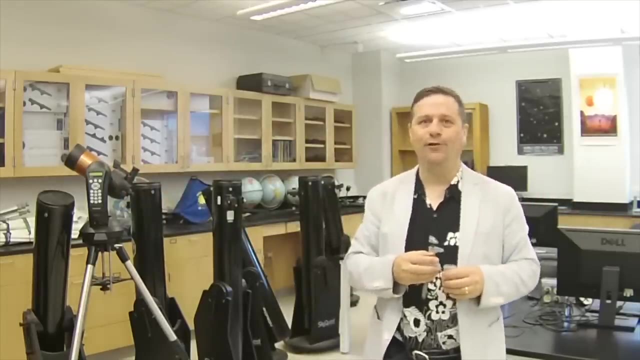 Jupiter's about that far from the Sun, Saturn's about that far from the Sun and Neptune's about this far from the Sun, and the Voyager is about this far from the Sun. So getting to the next star is a long, long, long ways. So how far? 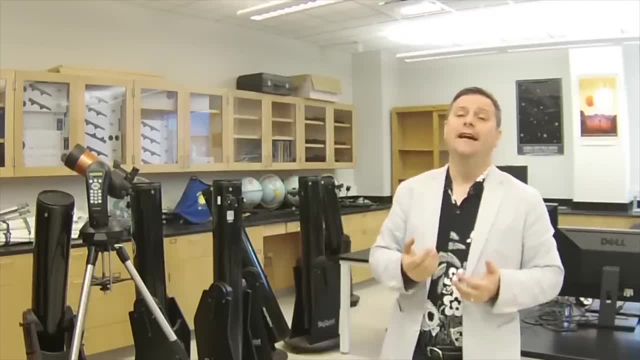 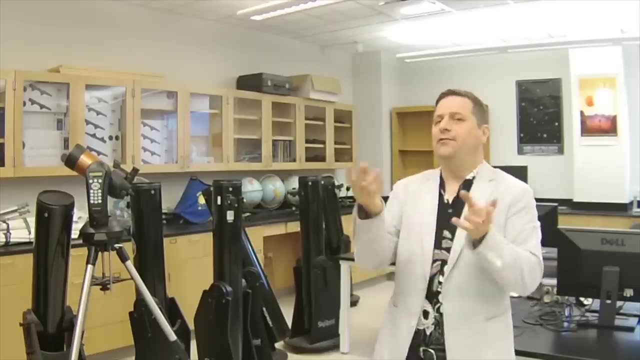 is 206,265 astronomical units. Well, it's about 30 trillion kilometers, or about 18 trillion miles, Or let's use another wing that you're probably familiar with, It's about three and a quarter light years, But what's a light year? A light year is the distance light travels in a year. Light has a distinct speed: 186,000 miles a second. So we can think how far does light go in one year, And that works out to be about 30 trillion miles, right? 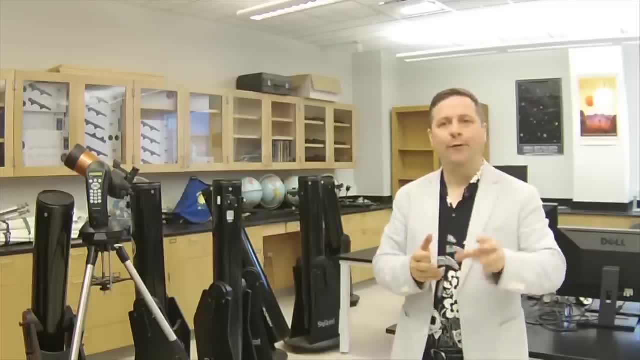 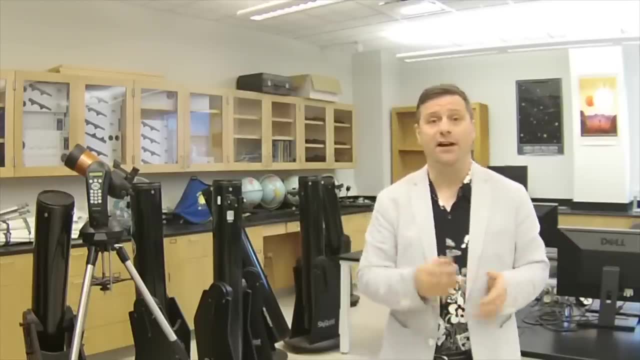 So well, it's about 6 trillion miles, Anyway. so a light year, though, is a weird unit of distance, because we're assuming that we can talk to the little photon that traveled all that light packet. The light packet doesn't carry a ticket with it saying. this is when I left. 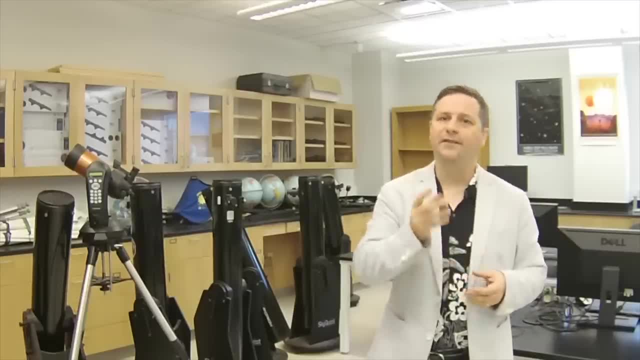 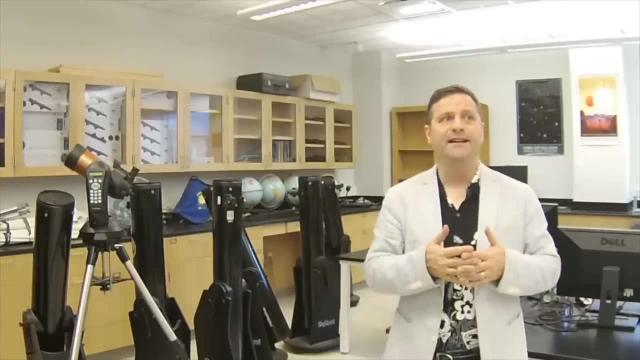 my place, my station. Now it doesn't have a clock on it, It doesn't have a ticket, It doesn't have any way of saying: this is when I started. So a light year is a really bad unit of distance because there's no way to say: 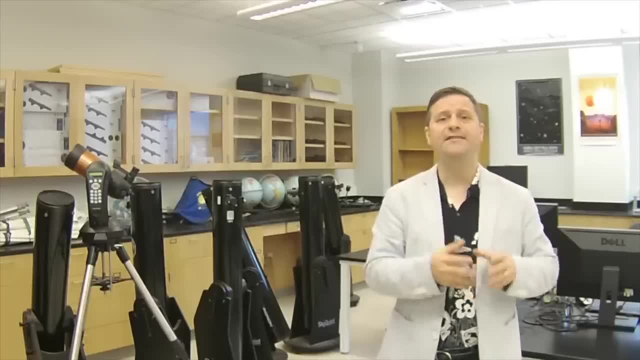 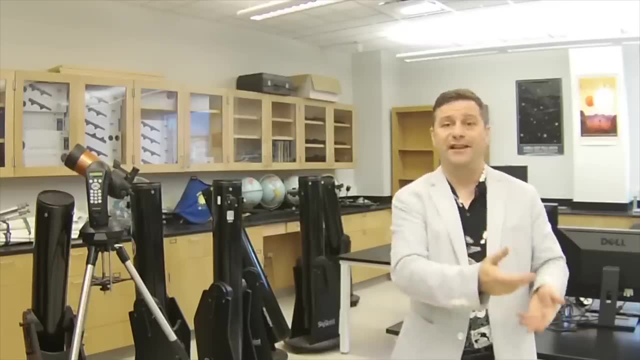 when the light started. However, a parsec is a fantastic unit of distance because it's based on geometry, so it's a real unit. So people use light years all the time because it sounds kind of cool, but light years are a unit of distance, not of time, And they're a really bad. 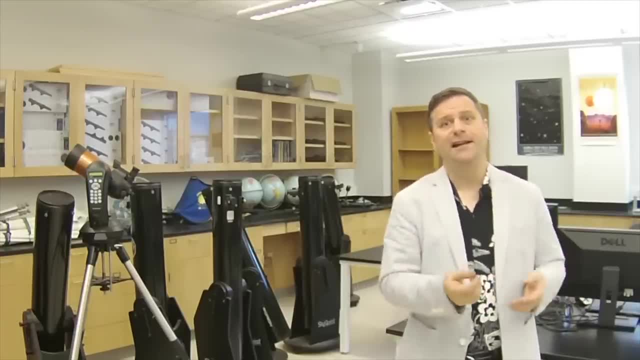 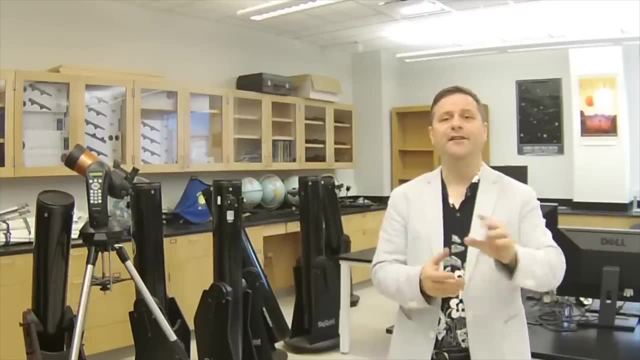 unit, because you know what's a light year? It's like okay, fine, And in fact we'll find that that actually has some very strange meanings when we talk about relativity. Anyway, so the parsec is the fundamental unit of distance in 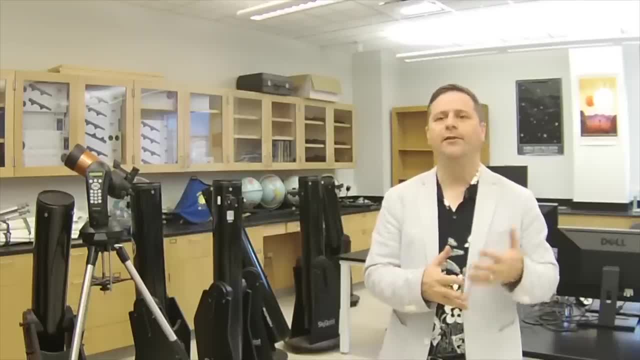 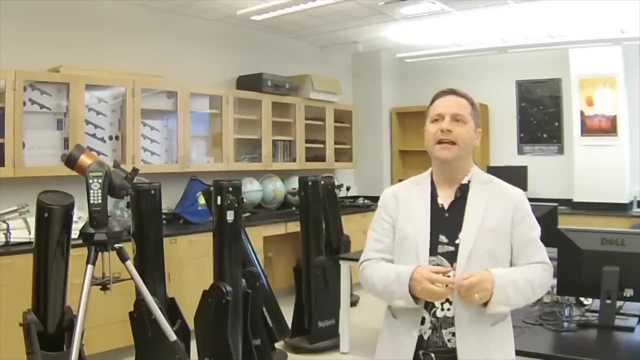 astronomy, And it's the basis for which things are a great distance. Alright, so how are we going to do these measurements of parallax? Well, parallax- the best you can do on the ground- is about a hundredth of an arc. second, 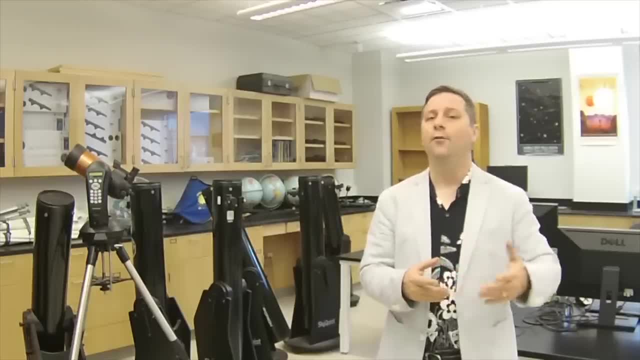 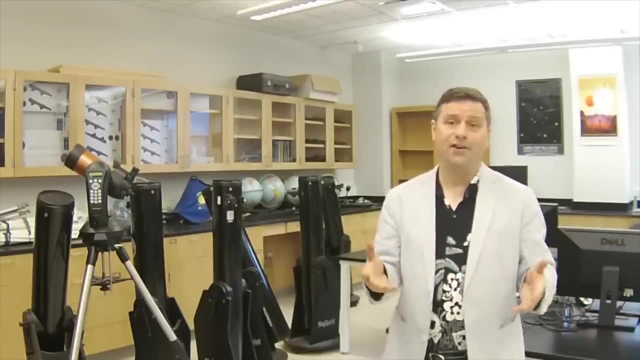 So that's pretty far. That gets you out to about a hundred parsecs or 300 light years. So on the ground you can see a parsec that goes out to about 300 light years. There's not a lot of stars within 300 light years. 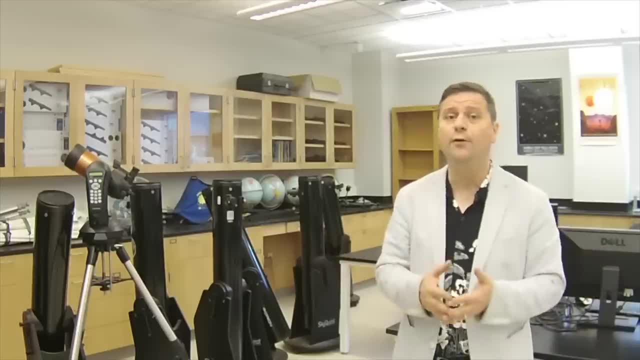 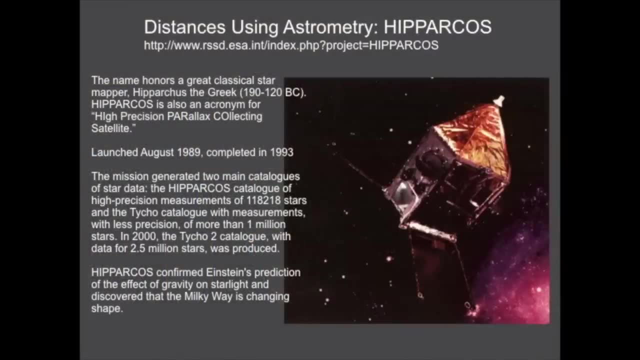 In fact there's very few stars, It might be less than a few hundred. within that time, In the early 1990s, 1989 to 1993, the European Space Agency flew the Hipparchus mission and they got stellar parallaxes, really good parallaxes for. 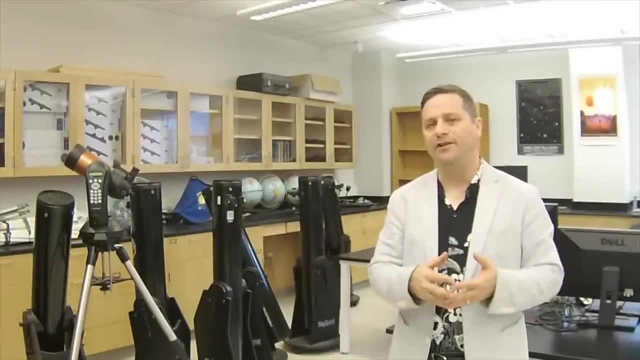 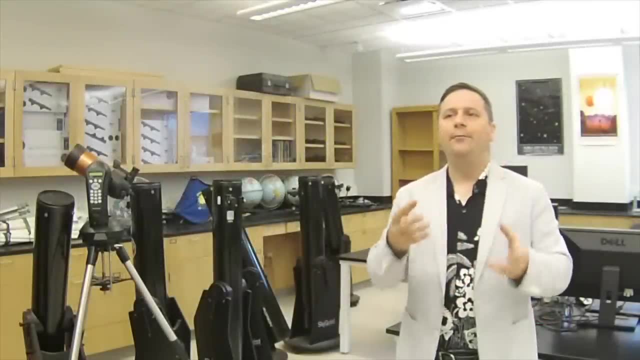 about 100,000 stars or so, down to about a hundredth of an arc second, and two and a half million stars, about ten times further but lower precision. So that was our main catalog of stellar parallaxes for a long time, until the Gaia mission. 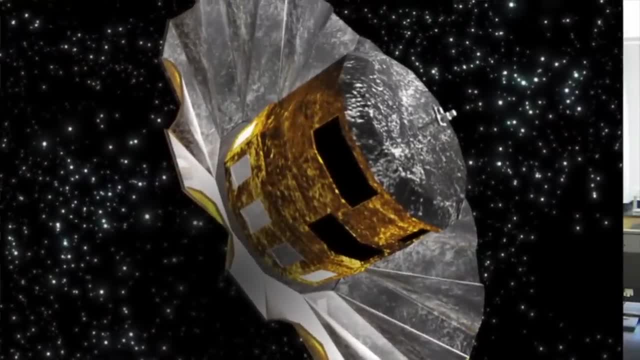 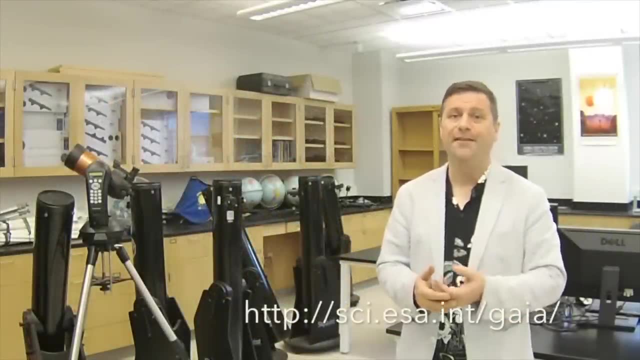 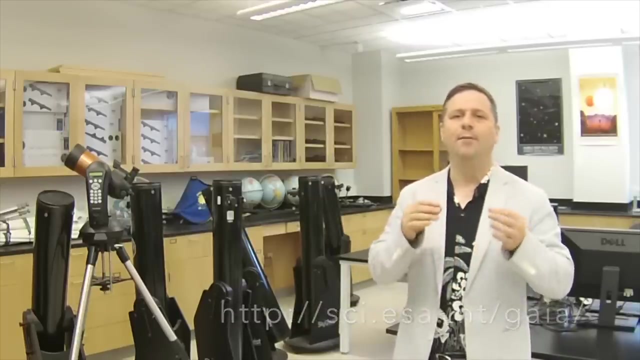 very recently gave their data set out and they have a data set of about a billion stars and they go out to about ten micro arc seconds. That's really far. One part in ten to the fifth of an arc second- Really far things and that gets us almost across the galaxy. 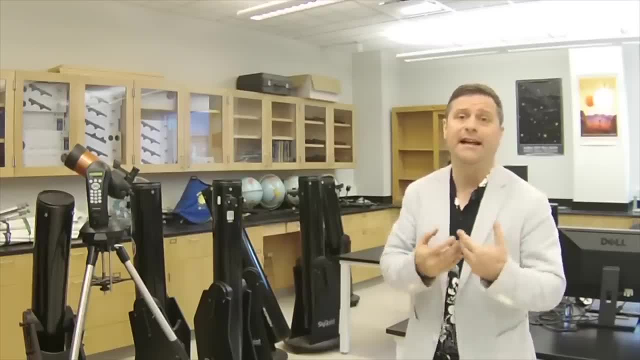 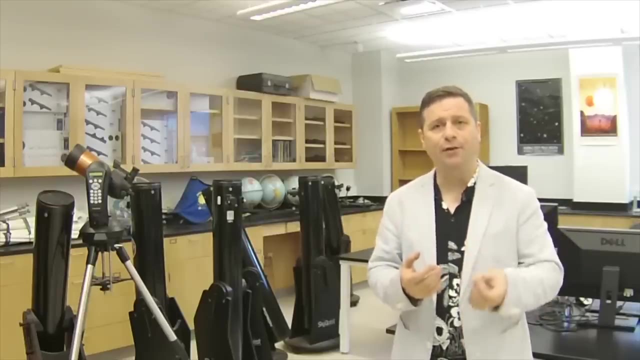 We get about half of the Milky Way can have its parallax done by Gaia, which is an amazing thing, and that data set will be used for a long period of time. One of the key pieces of the parallax distance is we have to know the distance to the Sun. 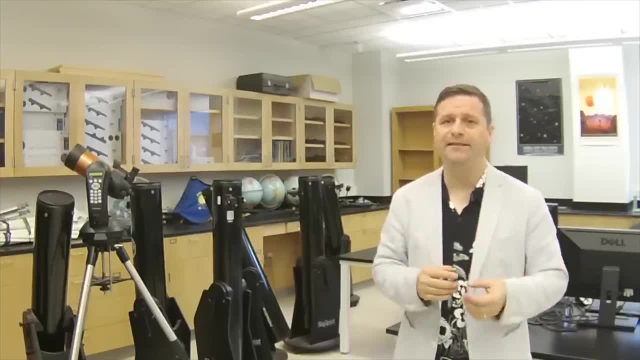 Because the parallactic angle, the parallactic distance, is so incredibly dependent upon the distance to the Sun. how do we get that? Because without the distance to the Sun, we'll never get the distance to the stars. So the distance to the Sun. 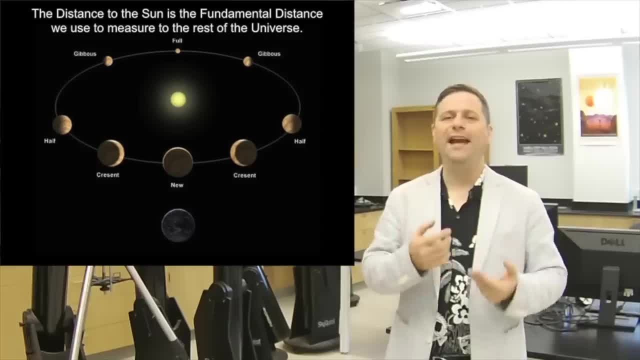 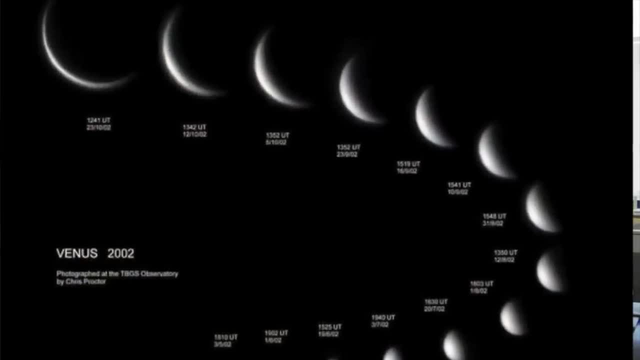 is calculated in a very tricky way. If we look at the planet Venus and we see how it orbits the Sun, we'll notice that at times in a telescope, Venus displays a quarter phase, just like we talked about with the Moon. 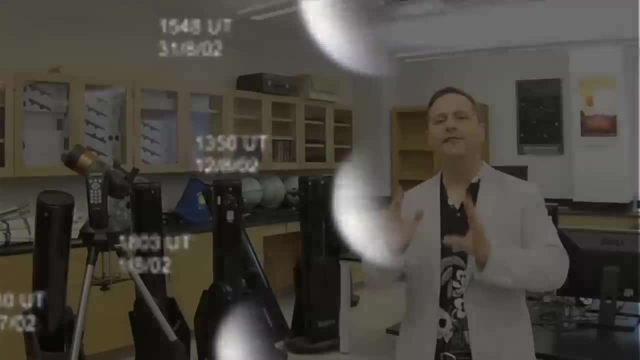 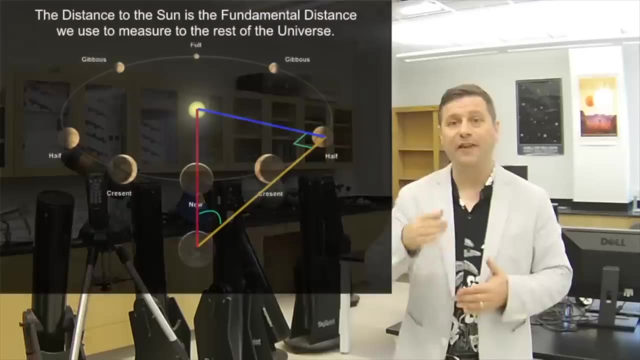 The Moon has quarter phases which look like half illuminated. When Venus is in quarter phase, it's exactly. we're seeing only one quarter of it. So that means that the angle that if we look at Venus, then Venus makes a 90 degree. 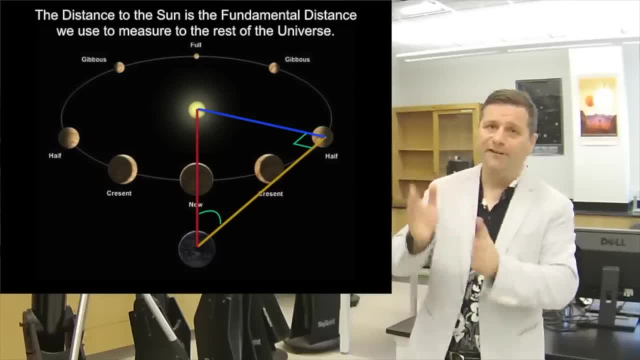 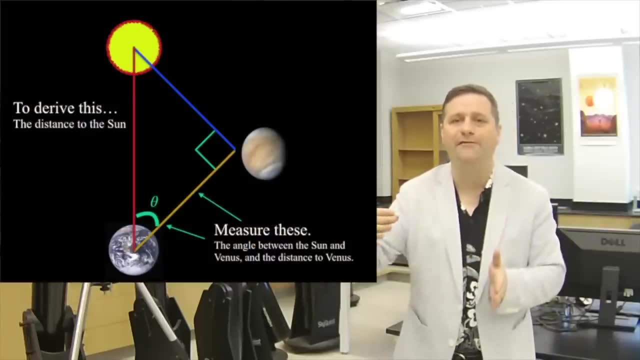 angle with respect to the Sun, And so when we look at Venus, it's roughly a little bit more than 45 degrees away from the Sun in the sky, and then it'll be half illuminated, which means it's at quarter phase, and so, therefore, we have a right triangle and all we 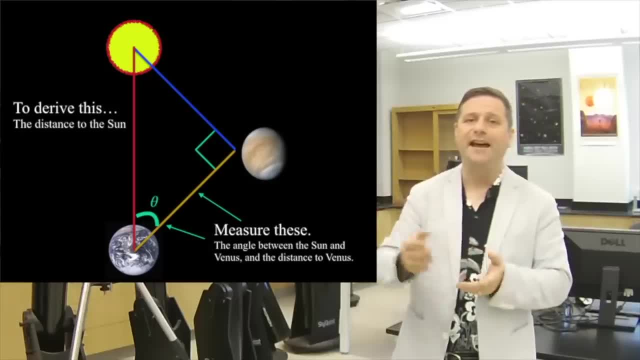 have to do is measure the distance between us and Venus. at that time We've got a right triangle and that gives us the distance to the Sun by simple geometry and trigonometry again. So we can triangulate our way to the Sun, not by actually measuring it out there, but by bouncing radar. 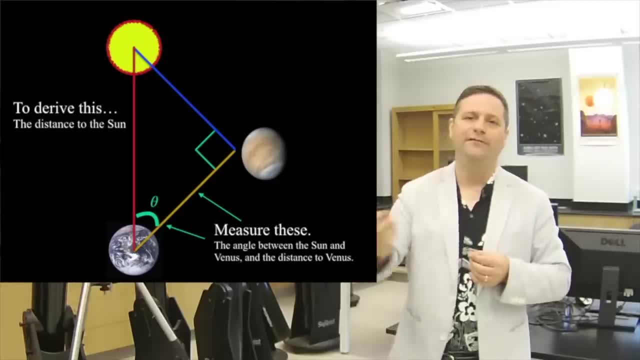 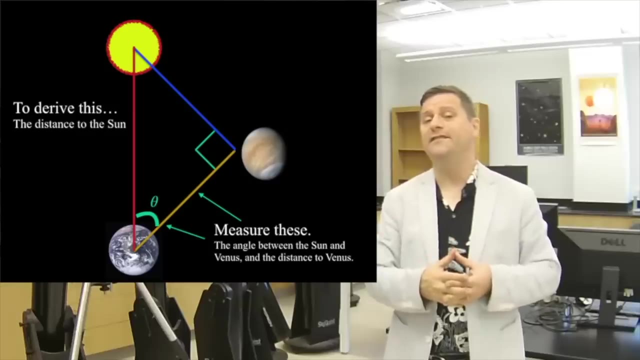 beams off of Venus, radar waves off of Venus, see how long it takes to get from there and back, and then measure the angular separation between the Sun and Venus when it's at quadrature or when it's at quarter phase. and what do we get? We get the distance to the Sun. 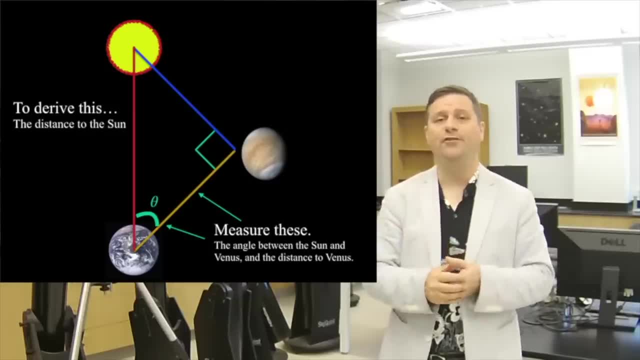 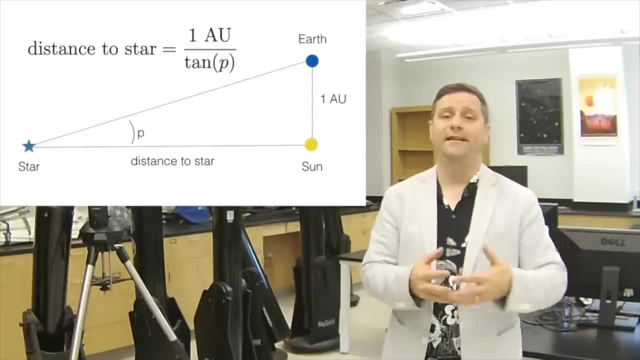 by trigonometry. Once we get the distance to the Sun by trigonometry, then we get the distances to the stars, And this is the basis by which we start to get distances deep into the cosmos. And it all starts with parallax, which is derived: 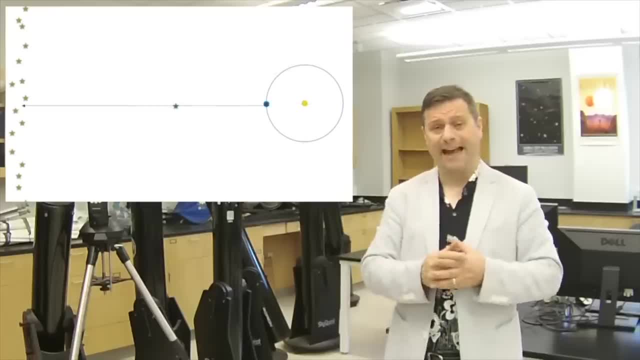 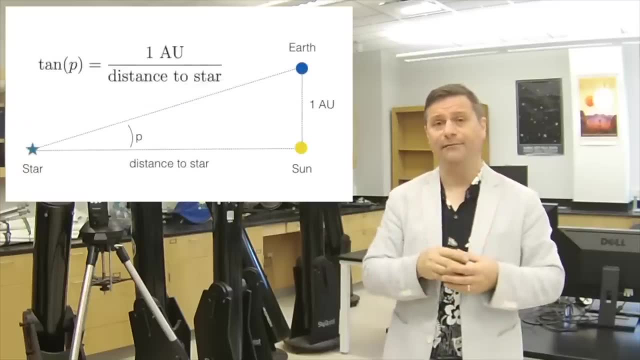 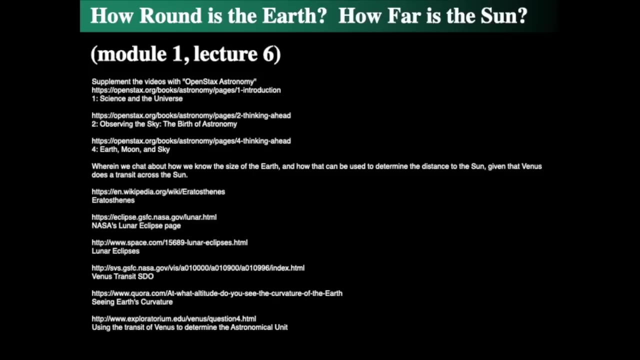 as a result of the Earth going around the Sun, and we see an angular shift of the stars in the sky as the Earth goes around the Sun over the course of a year. Alright, we'll see you next time. Hello, this is Jason Kendall and welcome to my next intro astronomy lecture. 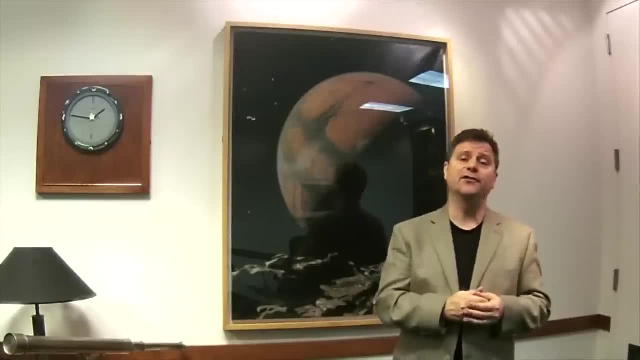 Well, last time we talked about parallax and determining the distances to the stars and there was one really important caveat, and that caveat was: first we need the distance between the Earth and the Sun, And that's a really hard thing. I kind of glommed over. 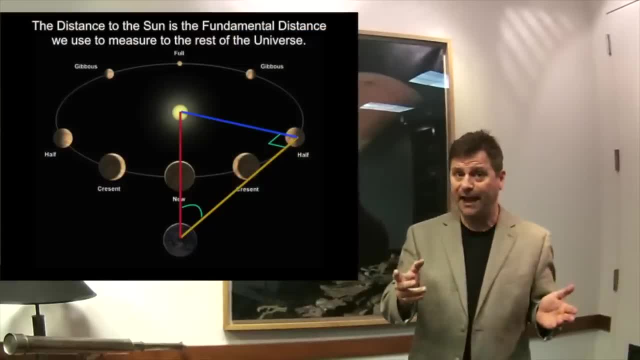 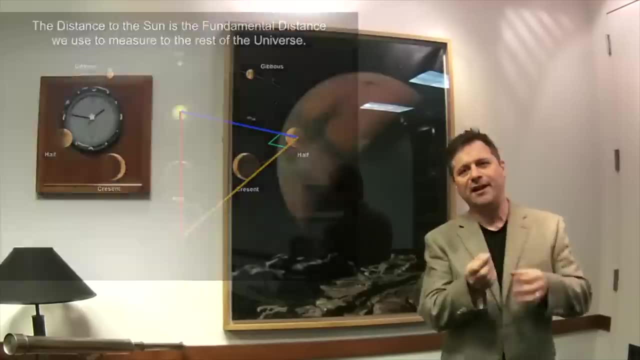 it by saying that we look at the distance between the Earth and the Sun today by doing radar reflection off of Venus and using geometry in order to get that distance. But that's kind of a cop-out because we've known it for longer than that and in fact people have made good guesses. 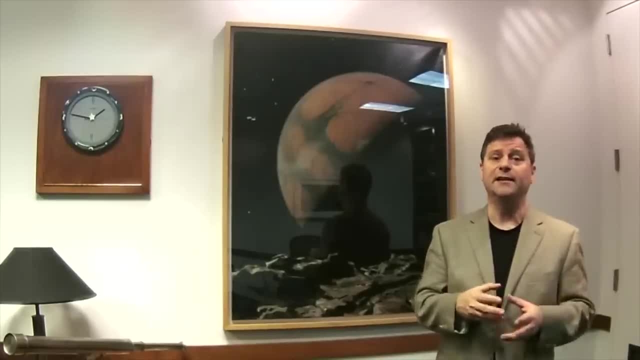 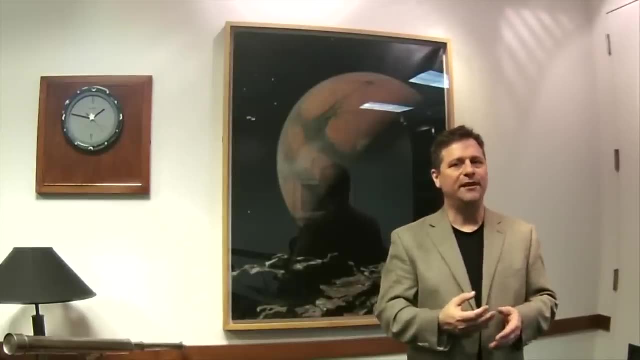 as to the exact distance between the Earth and the Sun for a long time, But let's see exactly how we can get there. One of the more important things that we have to think about, then, is to say: well, if we want to get the distance between the Earth and the Sun, perhaps we need to know how big 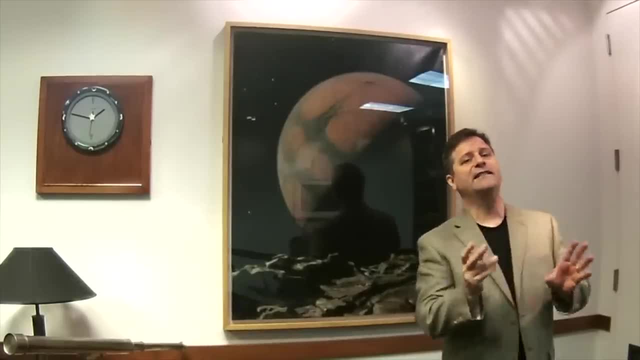 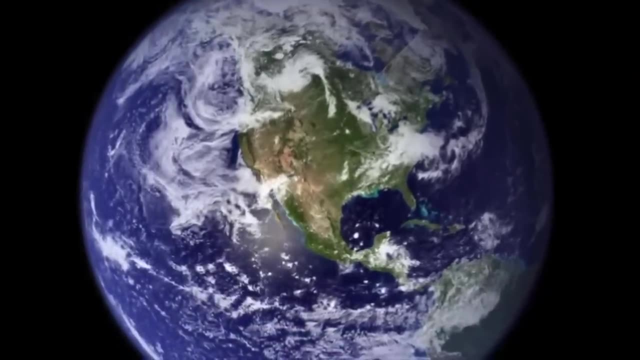 the Earth is itself first. So let's actually take a diversion and go back and say, well, how do we know how big the Earth is? And in fact we're going to actually find something fascinating along the way. So again, we're going to be talking about distances and how we get to parallax. 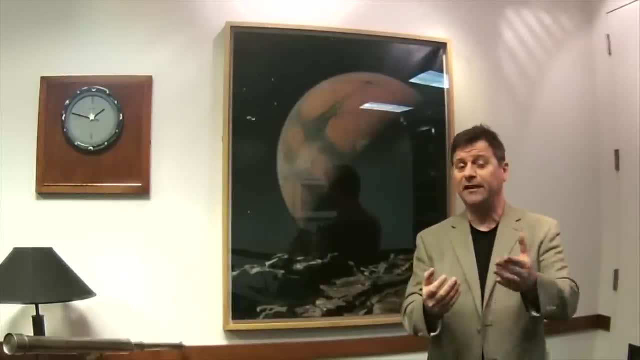 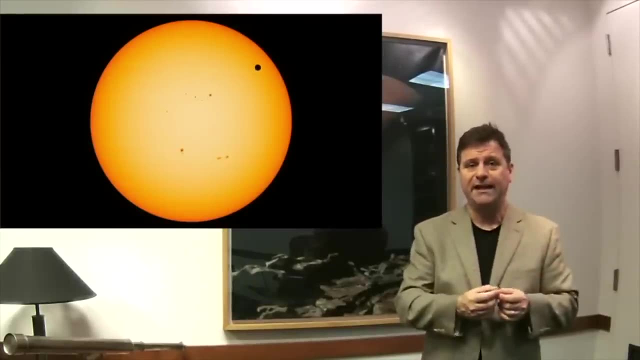 how we're going to actually then use the diameter of the Earth to get the distance to the Sun using the parallax of Venus during a transit, during a transit across the Sun. But that's for later. We have to build up a whole bunch of stuff in order to get there, So let's get the size. 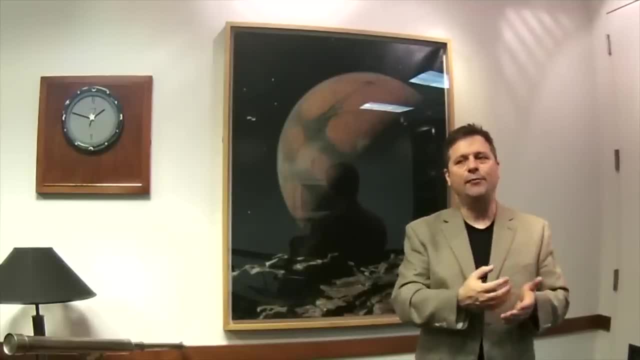 of the Earth. Alright, so let's think about how we can actually do that. The Earth is extremely large and if you take a plane flight and you go across country, it's very difficult to even see the curvature of the Earth. You have to get hundreds of miles above the Earth. 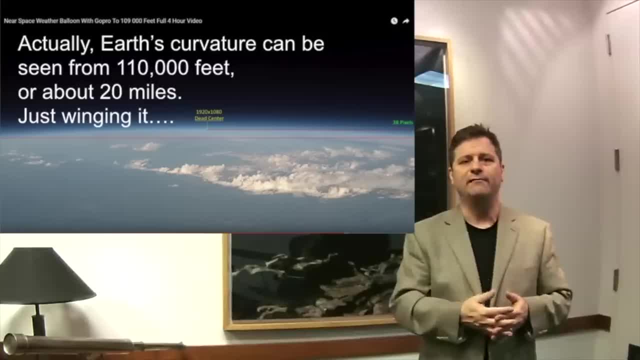 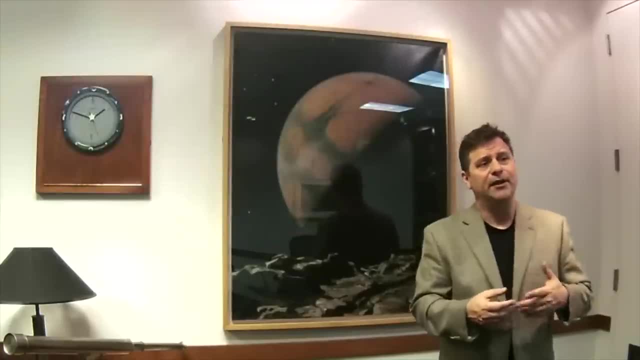 in order to begin to see curvature. Now, you can actually start to see it around 40 or so miles, but the point is that you have to be very high up in order to see the curvature of the Earth, Alright, so how do we actually? 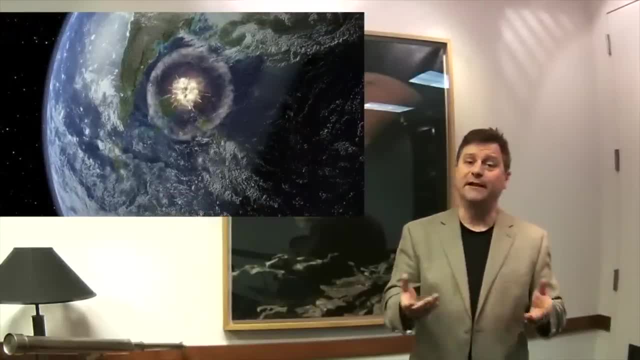 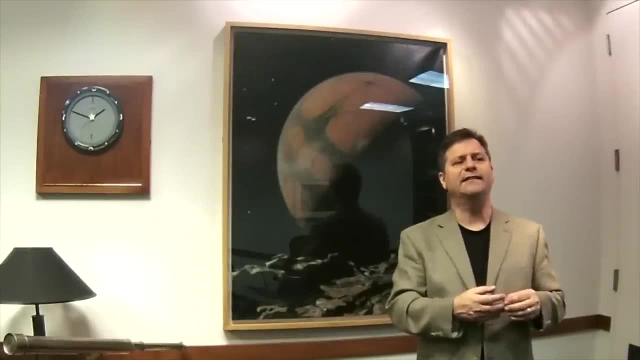 know that the Earth is curved. Let's pretend we never built a space program like the dinosaurs and that's why they're not around. But let's see. if we look at how far around the Earth is, we can look at lunar eclipses, which we talked about previously. 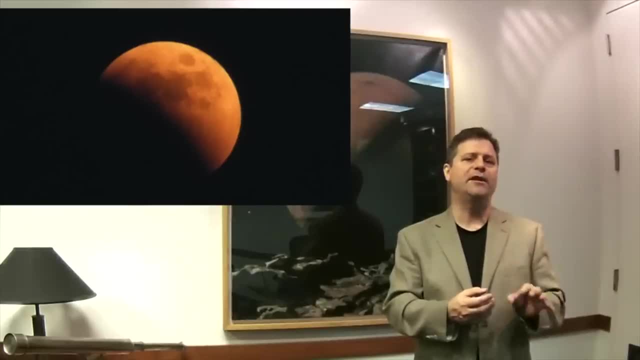 And we noted that the lunar eclipses only happen at full Moon. And as the Moon goes into the shadow of the Earth, as the Moon goes into the shadow of the Earth, we find that the shadow is not straight, it's curved. So people have known for thousands. 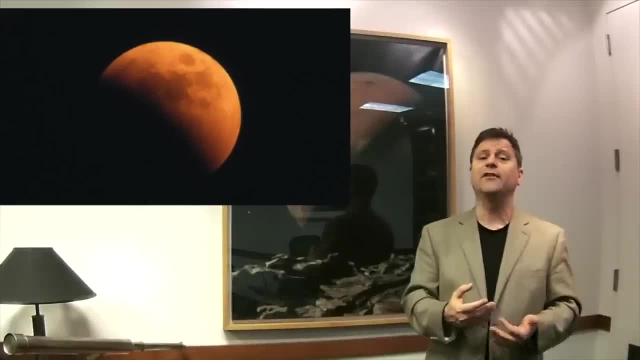 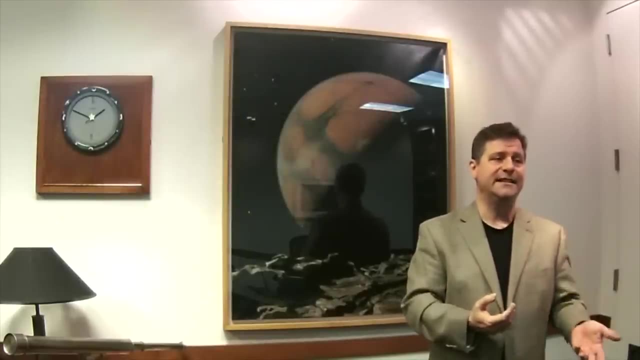 of years that the Earth is actually round because of the shadow of the lunar eclipses on the Moon. Alright, so how can we actually translate that into understanding distances? Well, let's actually see how big the Earth is, and if we then say, well, 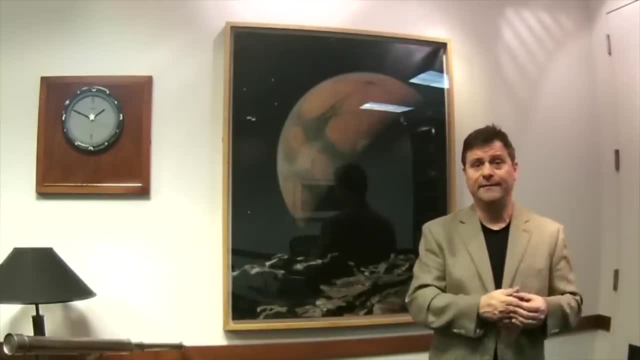 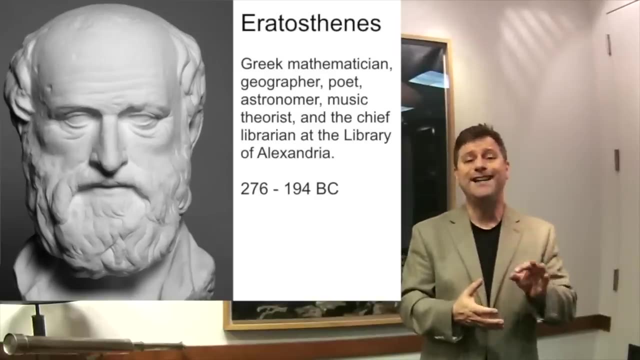 there was a wonderful- we can use actually shadows to do that- Actual shadows cast by the Sun. So about 200 BC, a Greek philosopher by the name of Eratosthenes- Eratosthenes, it's a very interesting name- who lived. 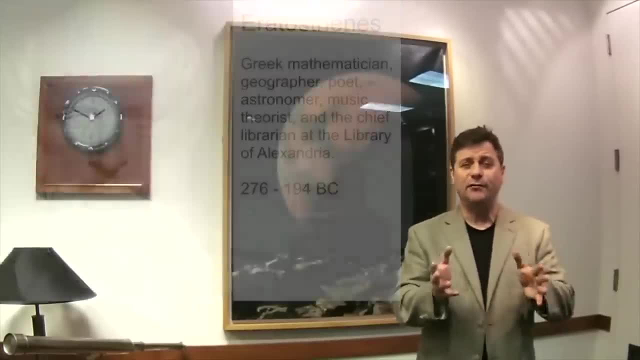 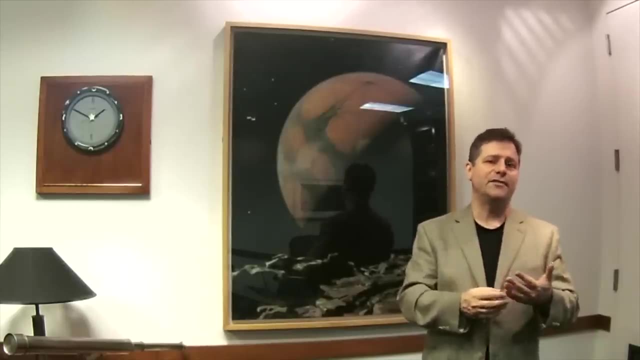 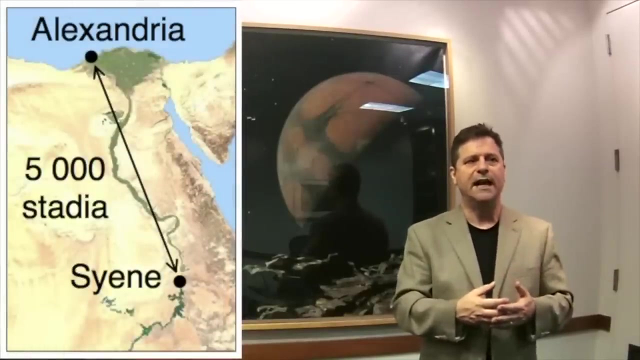 in Alexandria, Egypt, at the time, about 200 BC. as a Greek philosopher, he determined and learned that right around the first days of summer there were places, specifically in Syene, which is like now- it's now current day- Anwar. 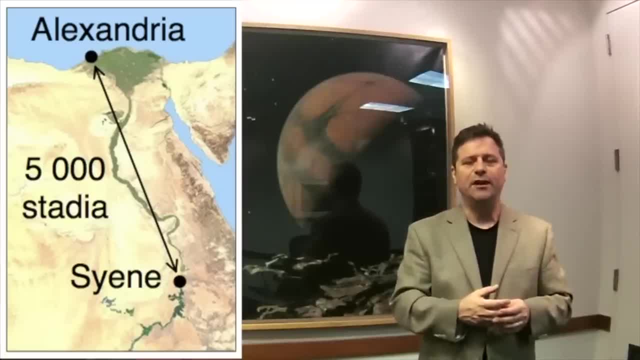 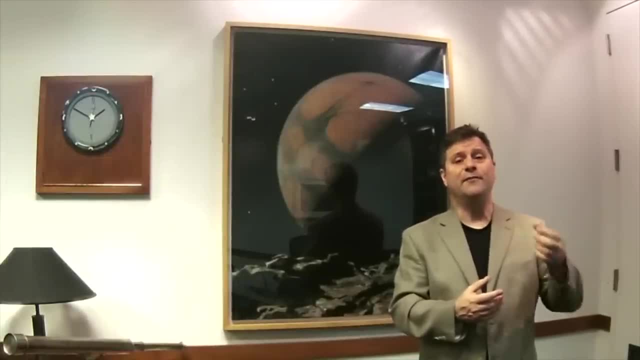 in Aswan- I'm sorry Aswan, in Egypt, But in Syene of the time it was seen at the first days of summer that the light from the Sun would go all the way down to the bottom of a deep well and not. 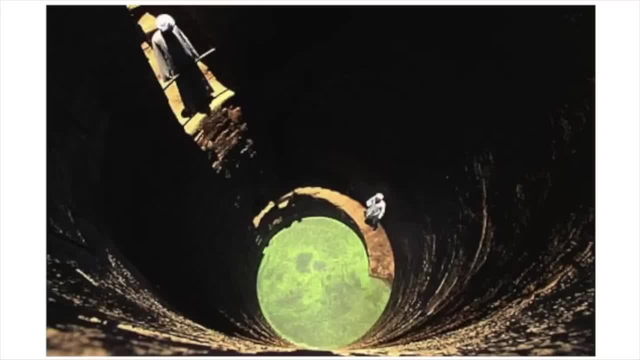 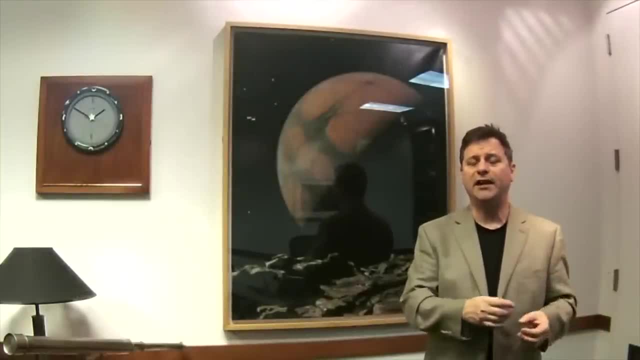 cast a shadow on either side. In fact it would totally illuminate the bottom of the well, assuming the well is completely straight down. It also tall poles would cast no shadow and they would actually have zero shadow around them on this first day of summer at noon. Well, he also learned. 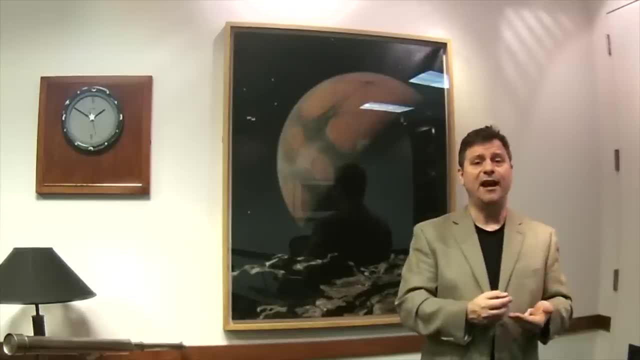 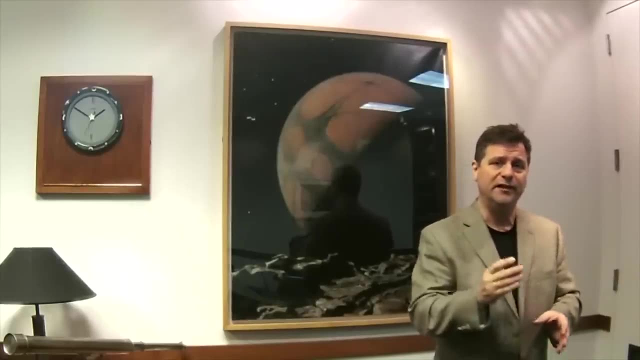 that in Alexandria, at exactly the same time, shadows were cast that wells down to the bottom- they're very deep- did have. the Sun did not penetrate all the way down to the bottom, but only made a circle on the side of the well. 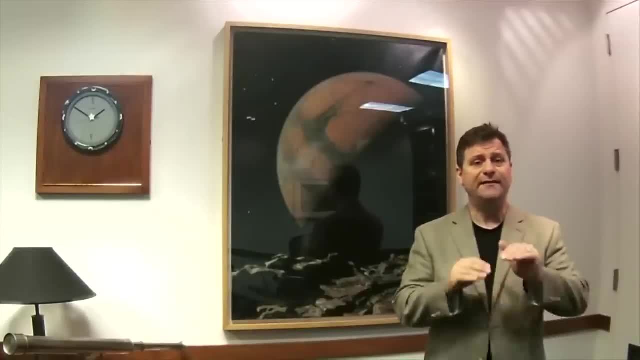 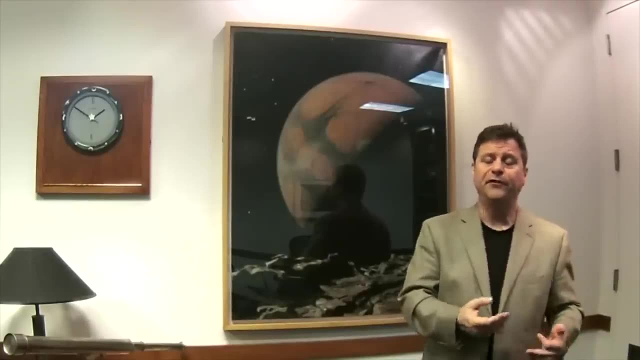 So there was something different, And the only way that that could be at the exact same time on the exact same day is that the Earth is not flat, but rather it's curved. So what Eratosthenes decided to do is he decided to measure the distance between Syene. 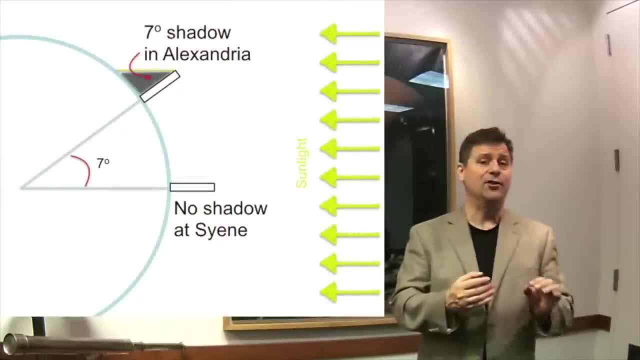 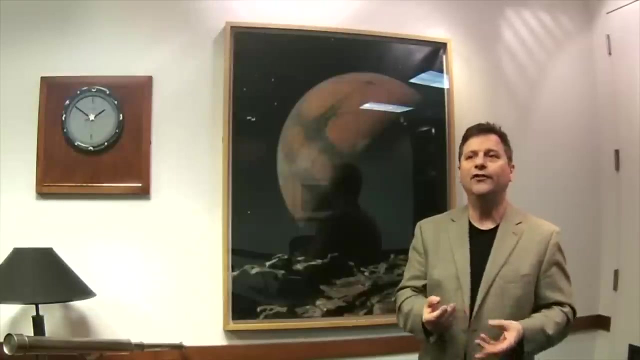 and Alexandria and measure the angle of the shadow in Alexandria when it had no shadow in Syene, And he found that the angle of the shadow at that time was about 7 degrees And he also found that the distance between Alexandria and Syene was. he used a particular 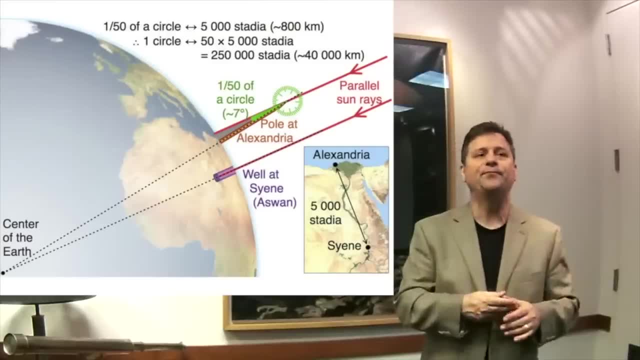 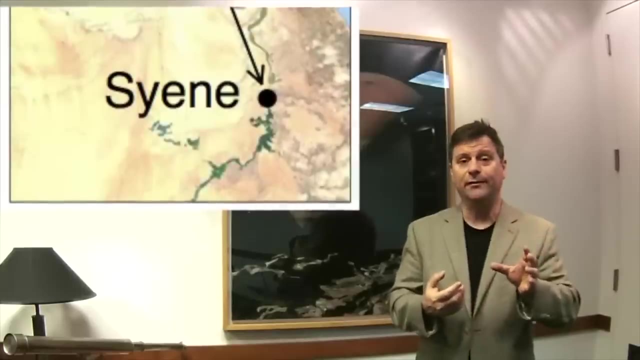 measuring unit called a stadia, and a stadia is about .6 kilometers, so it's a little bit less than a kilometer. So what we find is that if the distance between Alexandria and Syene could be measured- and of course back in 200 BC, there's only one. 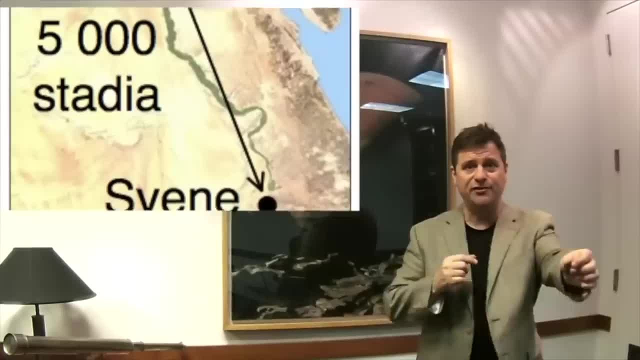 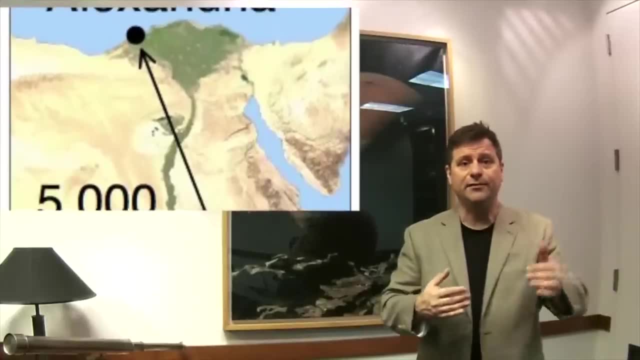 way to do it. You had to get somebody to walk it and that's how a stadia was measured. So somebody literally put down some poor schmuck, put down thousands upon thousands of these meter sticks and figured out the exact distance between Syene and Alexandria. 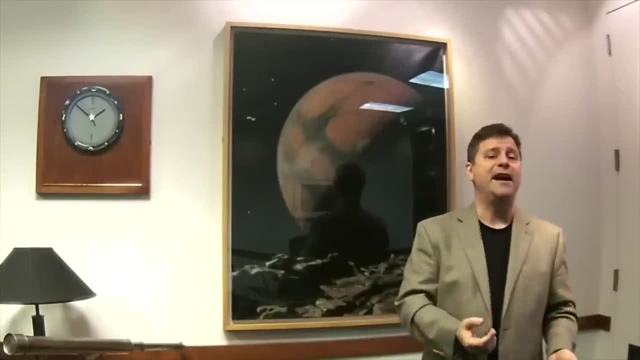 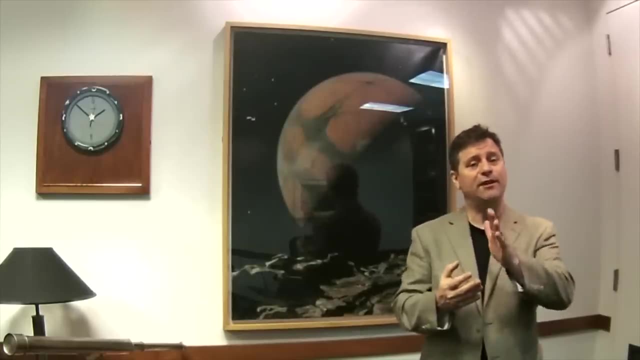 To a pretty good and fair approximation. So it was found to be about 5,000 stadia distant and they're almost directly north-south from each other and the angle separation in one location had zero and the other location had 7 degrees, so we can. 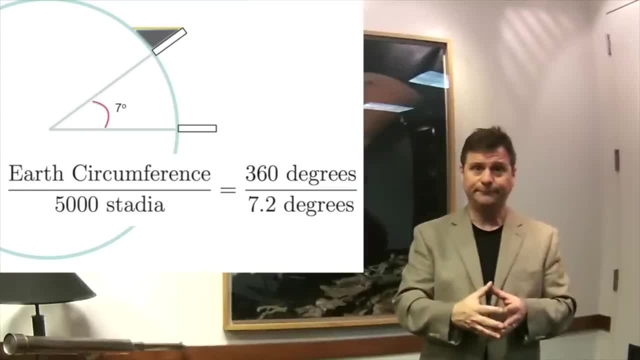 use very simple geometry in order to determine the actual size and the circumference of the Earth. Well, we know that the circle has 360 degrees and if the shadow cast is only 7 degrees, meaning a tall pillar had some length of some shadow. so how you get this angle would be to look at the angle in the shadow and 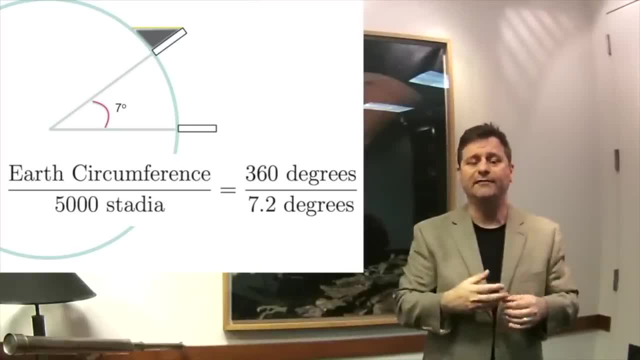 determine it from that. You can use a plumb line, and so forth. There's a lot of different ways to measure angles of shadows, and they weren't alien to people of his time. So, but 7 degrees divided by 360 degrees, well, that's the same thing as saying the length. 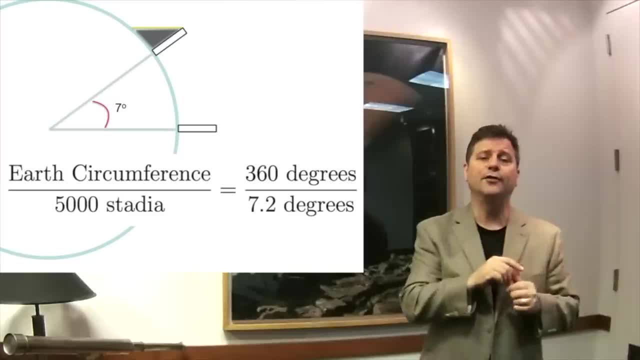 of an arc on the surface of the Earth compared to the entire circumference of the Earth. So the length of the arc was 5,000 stadia and the circumference of the Earth is what we're trying to discover. So if we have, 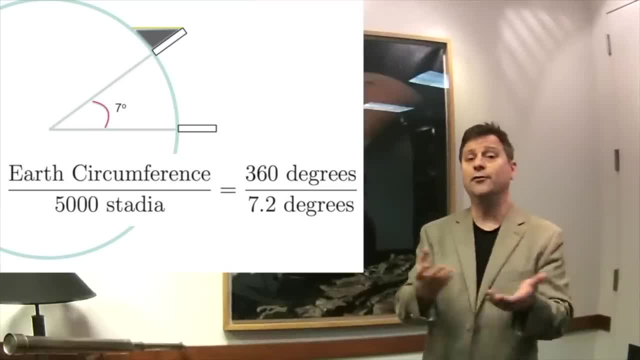 7.2 divided by 360, and that's equal to 5,000 divided by your number, then that works out to be about 250,000 stadia, Or more specifically, 7 degrees is about 1 50th of 360.. 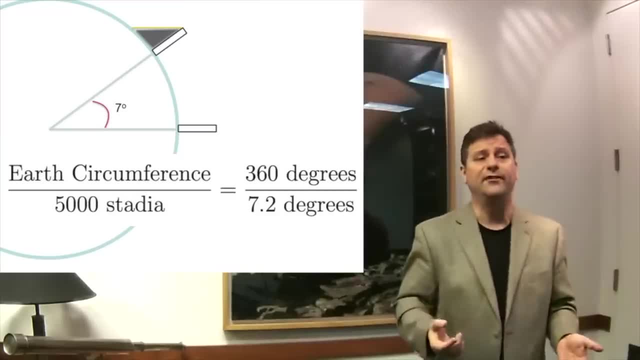 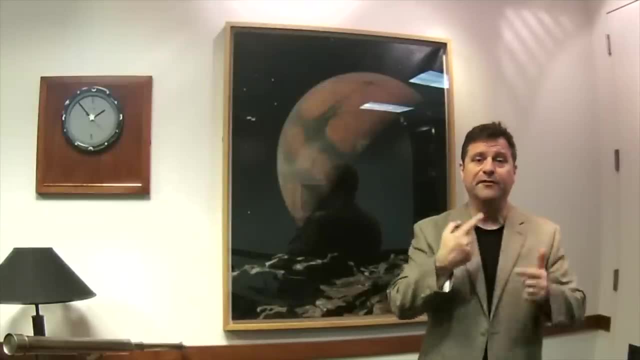 So 5,000 stadia times 5, 50 is about 2,500 stadia. Now, since it's a circle, we assume the Earth is round, so it can be spherical. so a circumference would be 2 pi divided by. 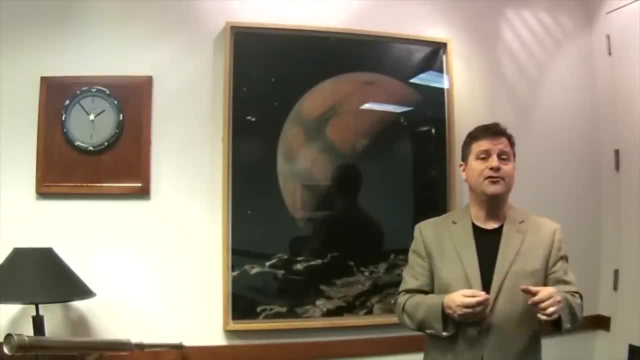 that and that gives us, according to his measurements, about 6,366 kilometers as a radius of the Earth. Now, that's a really good measurement, because it's within 1% of the modern value of about 6,378 kilometers. 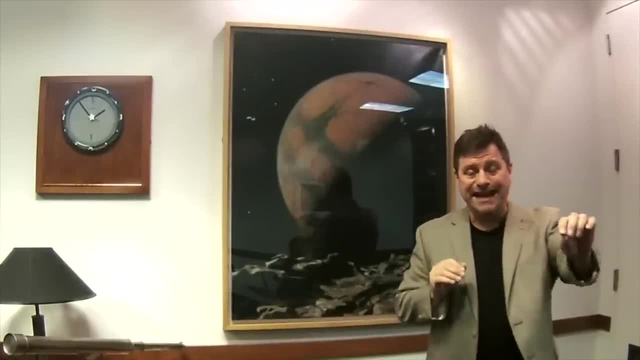 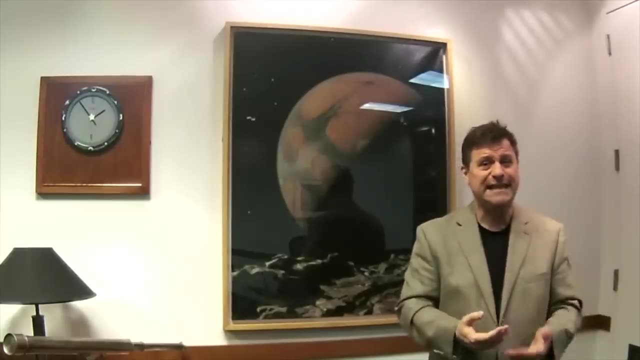 So look at this way, Just having some guy pace off the stuff and doing a very accurate measurement across the land between two cities in 200 degrees BC, well over 2,000 years ago, was able to actually determine the radius of the Earth's size to within 1%. 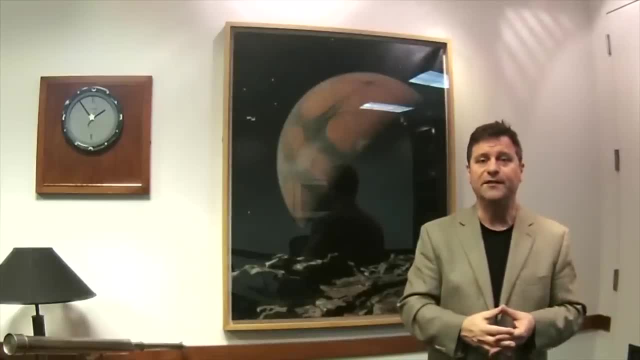 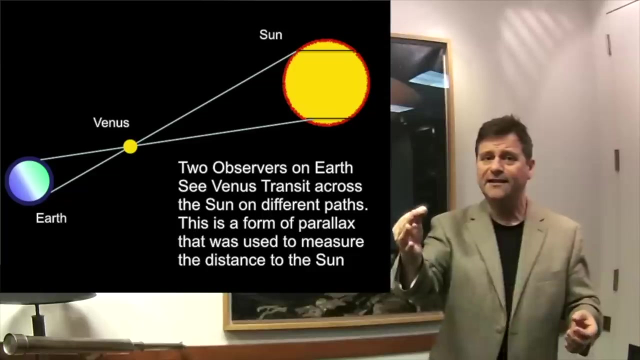 of the modern value made with extremely accurate measurement systems. Well, we use, then, this diameter of the Earth as a baseline, and the baseline can then be used during transits of Venus. When Venus goes between the Earth and the Sun, very rarely does it cross the 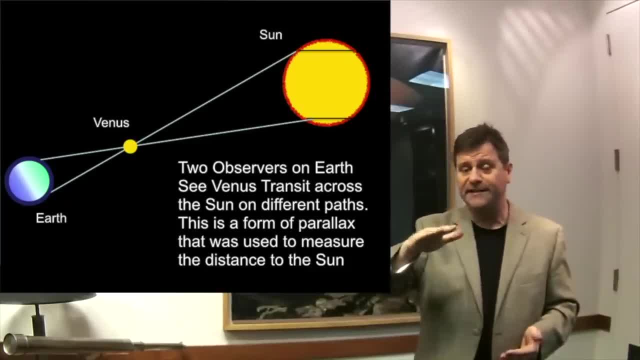 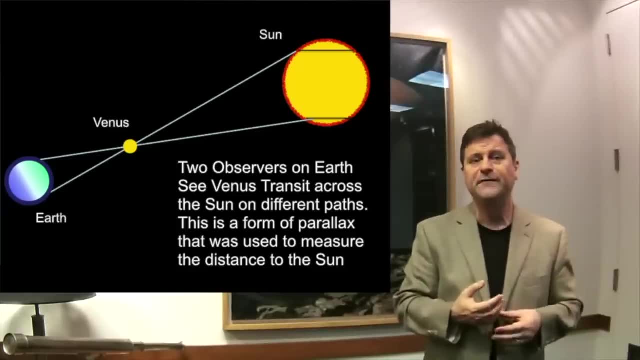 Sun's face as it does so because Venus's orbit is tilted slightly with respect to the Sun, with respect to Earth's orbit around the Sun. So Venus transits are rare, But when they happen, you can use two people situated across the diameter. 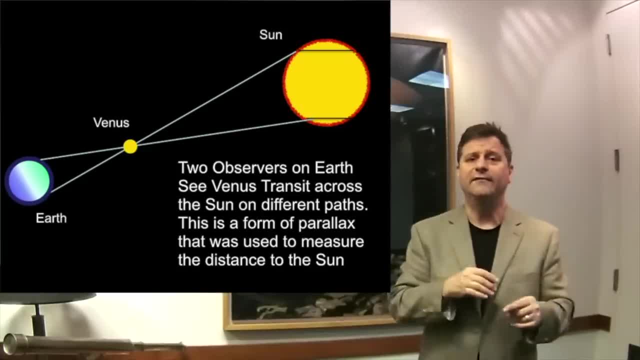 of the Earth, say at the North and South Pole or across very far apart, to check the timings of the transits across Venus, and that can give you a parallax of Venus with respect to the Sun, And that parallax gives you distance. So this is a really interesting thing. 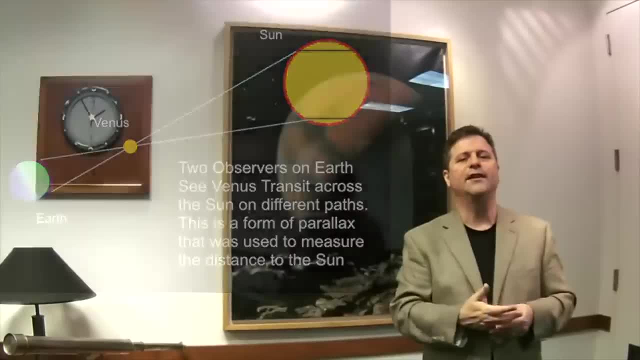 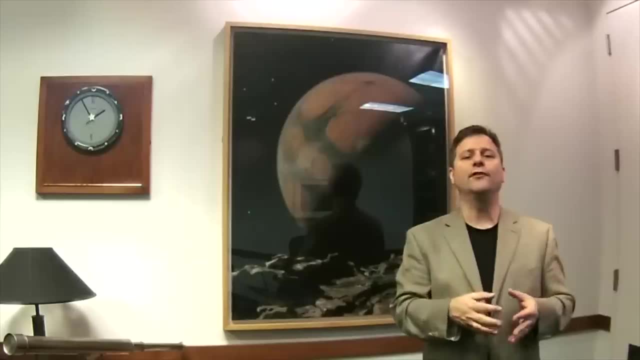 but actually, how do we get that? How do we know that that works? Well, that's going to rely on the development of calculus. It's also going to rely on the development of Newton's laws of gravity, Kepler's laws of motion and utilizing Galileo's. 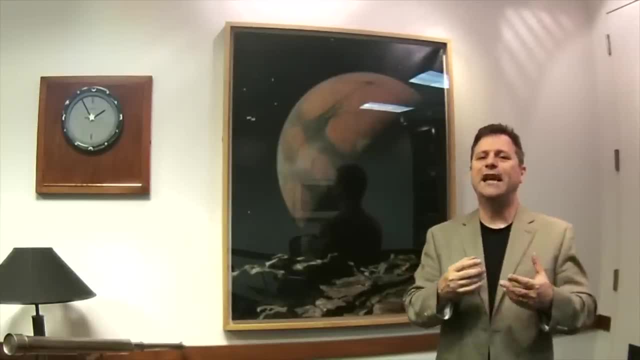 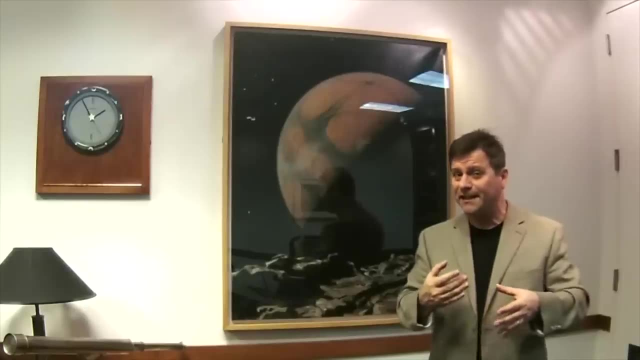 relativity concept, More specifically, the idea that we do actually orbit the Sun, that actually the Earth does go around the Sun and it doesn't feel like that. So to think that the Earth is actually round, even though it looks to all of us to be flat, and then to think: 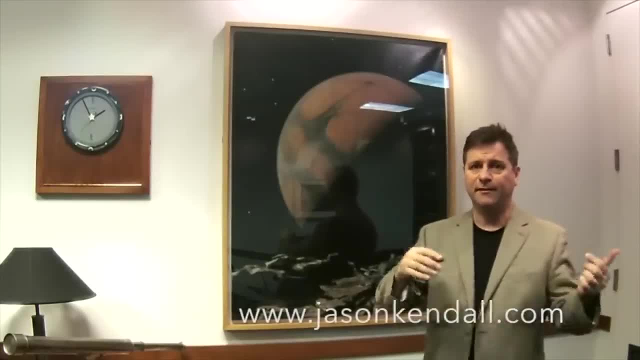 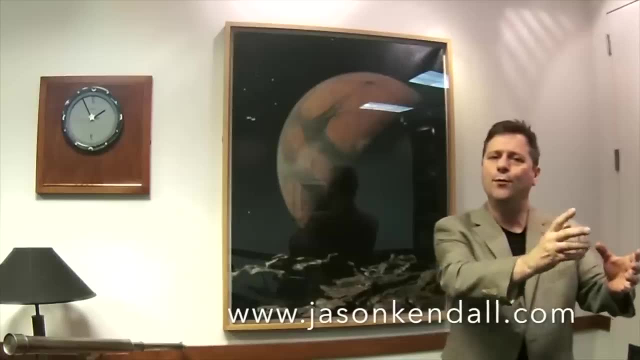 that if the Earth is stationary, then as the Moon and the Sun go around, we have these relative sizes. but then to actually make the step to say how does the Earth move? And that is a big story that we'll come to very soon, See you. 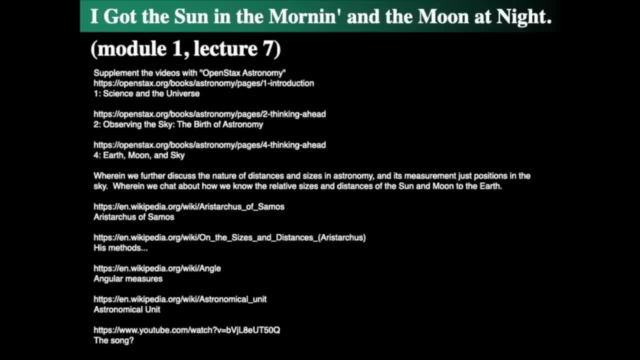 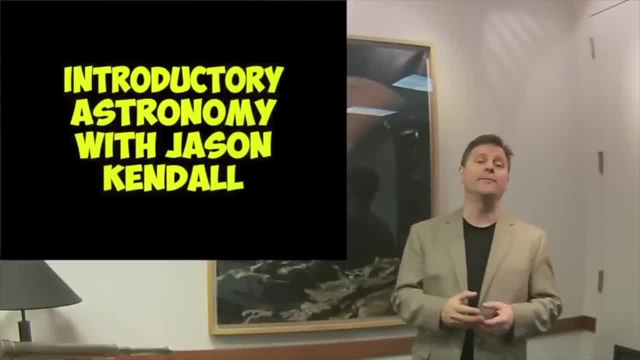 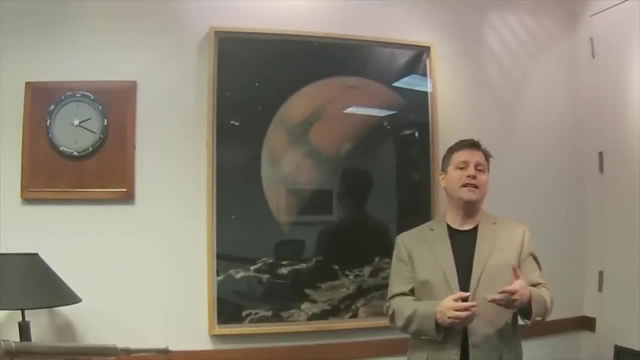 next time. Hello everyone, My name is Jason Kendall and welcome to another one of my introductory astronomy lectures. Well, today we're continuing the concept of distances and sizes. Last time we looked at the nature of the size of the Earth, pacing it out. 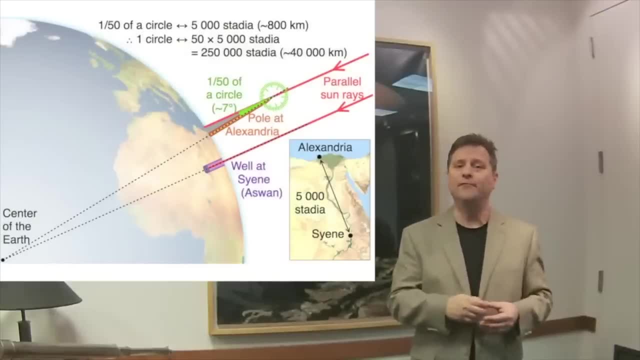 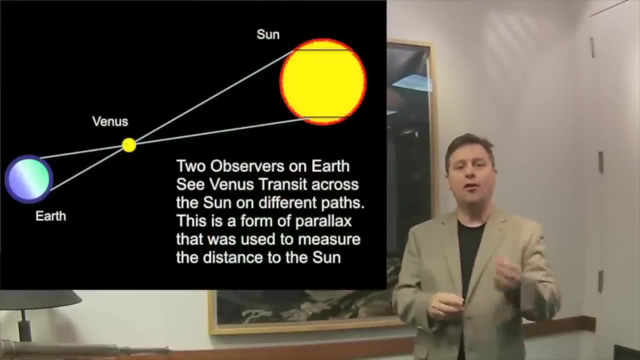 using stadia and shadows and various places on the equator, But if I want to actually then say, fine, that's how big the Earth is. but we can also use simple geometry to make extraordinarily good guesses as to the relative 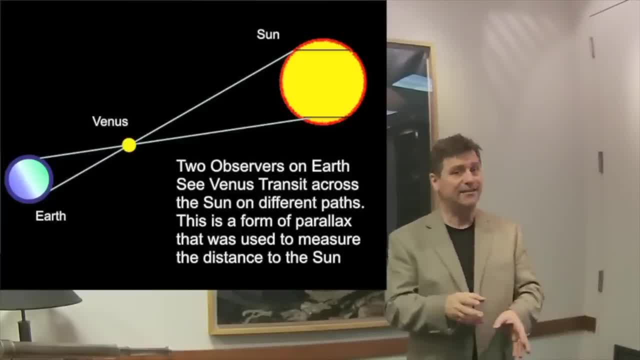 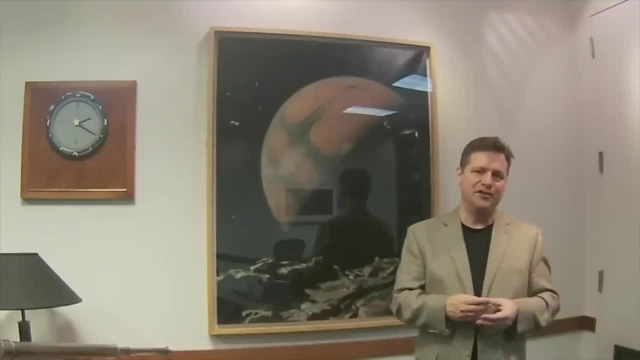 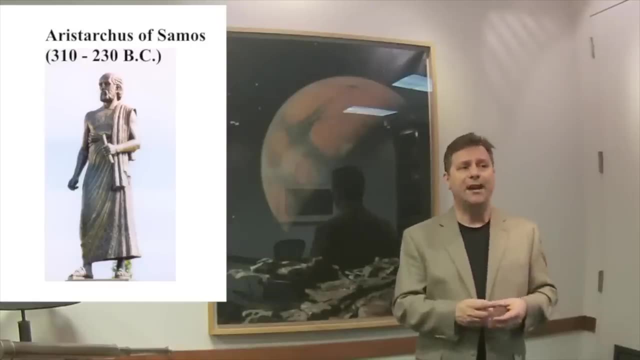 distances between the Earth and the Sun. Not the exact distances, but getting very, very, very close. In fact, this method would work if it were easier to do. Alright, so let's describe yet another ancient Greek philosopher, this one, Aristarchus of Samos. Aristarchus lived from about 310. 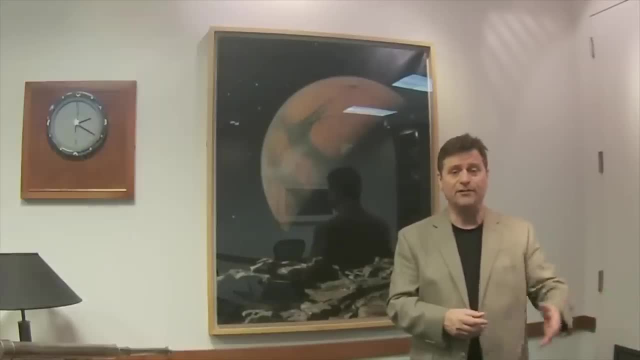 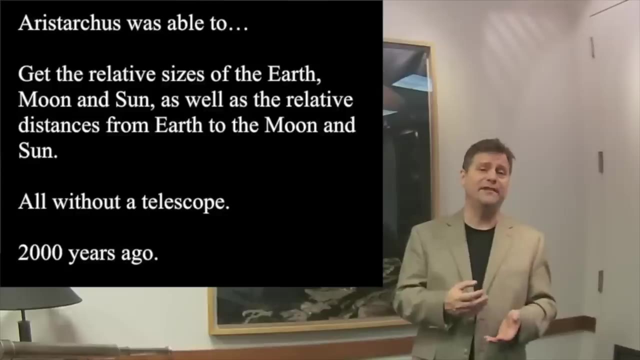 BC to about 230 BC, so this is over 2200 years ago- And what he found was that he was able to deduce the distances, the relative distances, and in fact get a good estimate for the exact distance to the Sun and the exact distance. 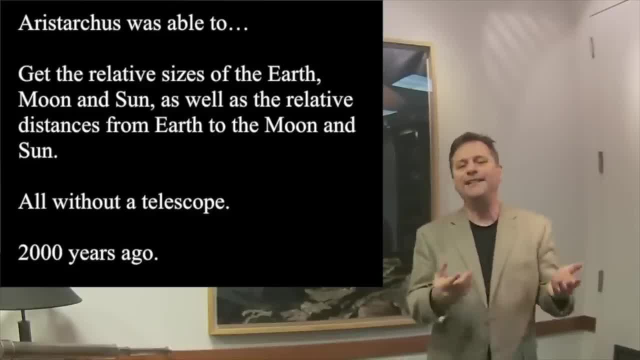 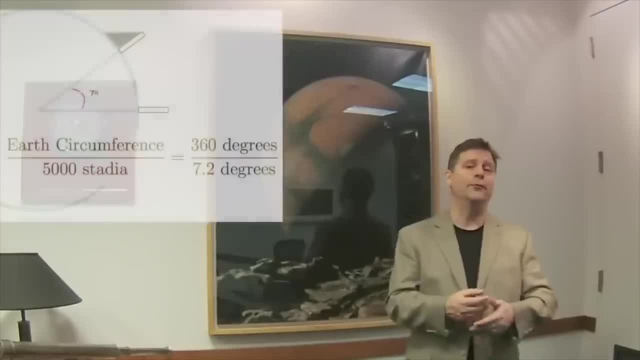 to the Moon and their relative sizes as well. So how did he do this? He did this all by eye and by hand. Remember, his contemporary actually knew the size of the Earth, so we can actually use that and plug that in later in order to get the actual sizes of the Sun. 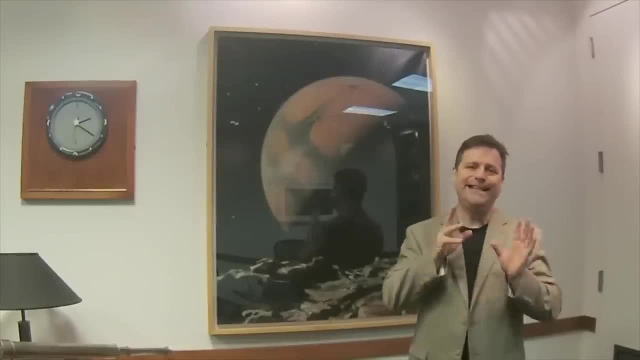 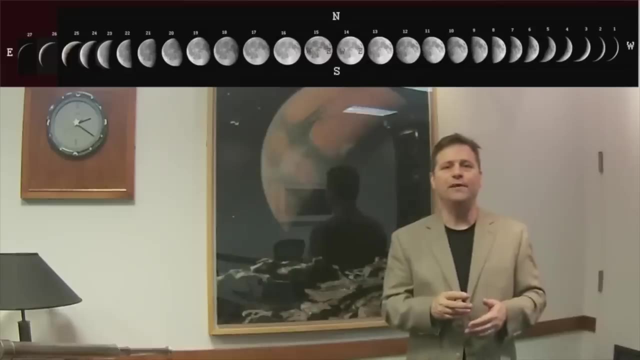 and the Moon, according to Aristarchus. So how did he do it? So let's go back and remember our phases of the Moon. So we look at all of the phases of the Moon that we see going around, and one of the phases is, of course, first quarter. So 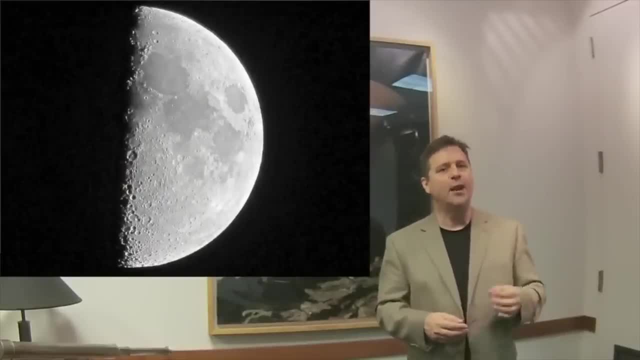 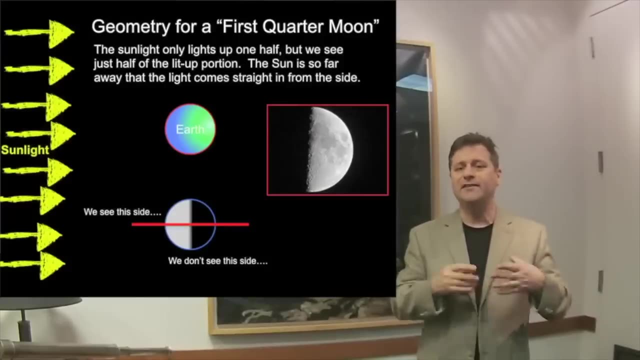 when the Moon is at first quarter phase. we know that the geometry in space. if we look down from above, we see that the Moon is in one part of a triangle between the Moon, the Earth and the Sun. But the Moon in that 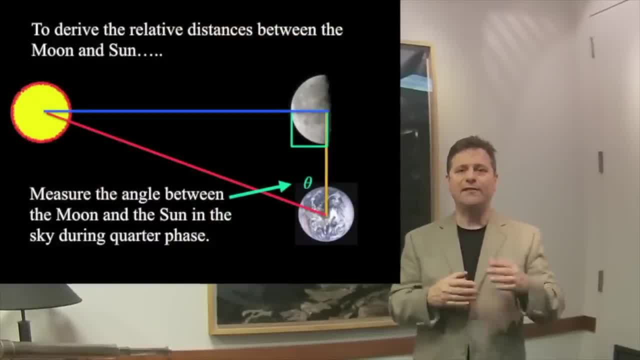 triangle is at the 90 degree point. So we have a 90 degree triangle with the Moon at the 90 degree point, and that's when it's a quarter phase. Remember it's half illuminated, That means it's quarter phase. 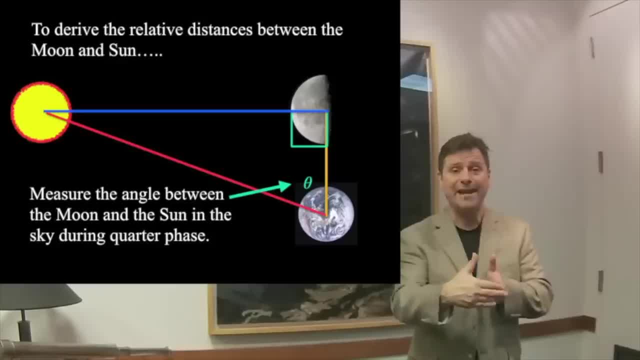 That means it's 90 percent. that means we have a 90 degree angle between the terminator, meaning the day and night boundary, and the edge of the Moon that we can see. So that is a quarter phase, or 90 degrees. 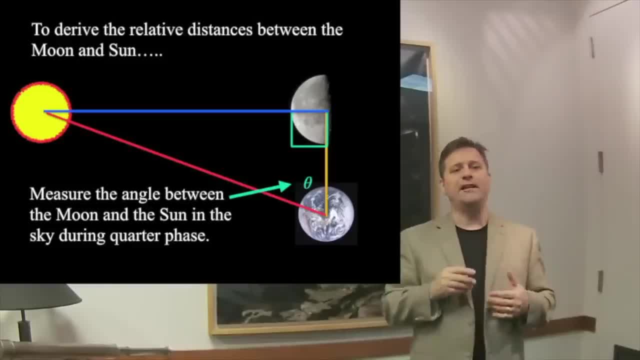 around a circle. So we got our 90 degree area. So when Aristarchus then looked and went, hey, that's a 90 degree angle, which means that all I need to do is get some sort of rough distance, or in fact, actually I can get their relative distances pretty easily. 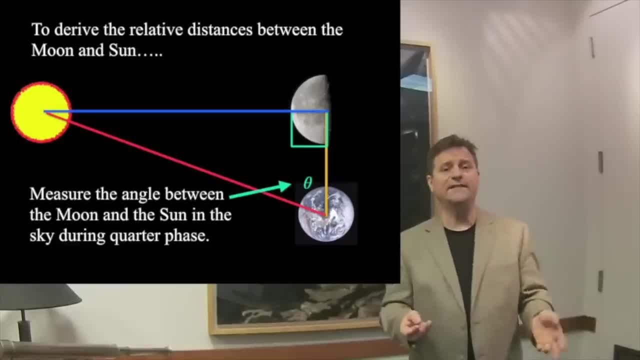 Because, using simple geometry, we can get their relative distances because of the size of a triangle, and all we have to do is measure angles. And so what he did is he endeavored like crazy to measure the angle in the sky between the Moon. 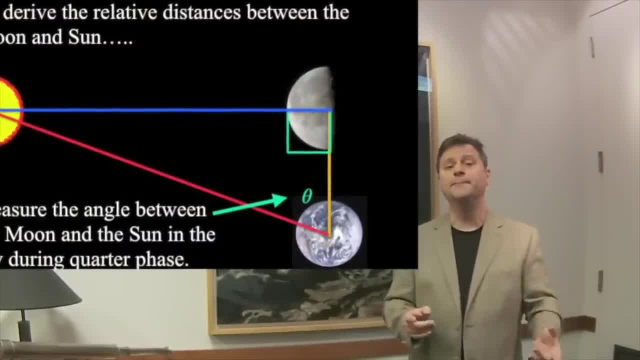 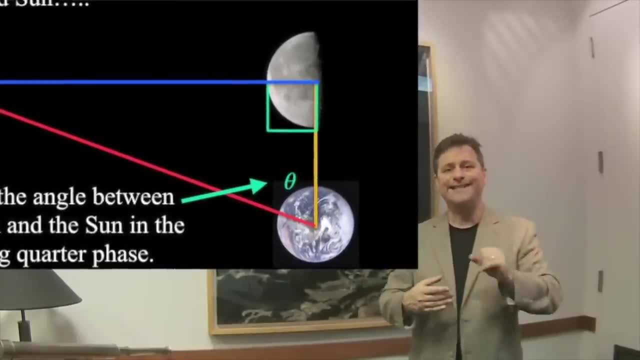 and the Sun. Remember, the 90 degree angle of the triangle is where the Moon is, but then the angle that we, when we look at the Moon and we look at the Sun, that is less than 90 degrees, and so we can use trigonometry or specifically, 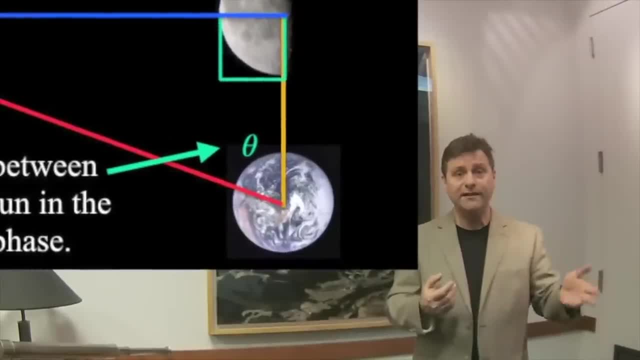 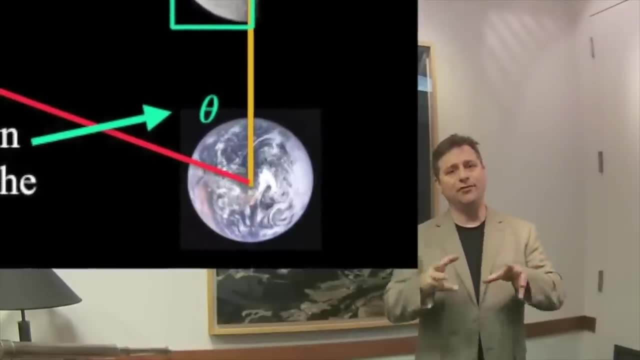 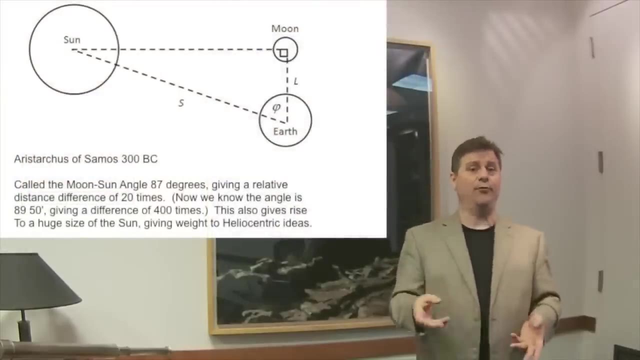 the cosine of the angle to get the relative distances between the Earth and the Sun. So what he measured in the sky was he measured, roughly speaking, about 87 degrees. That's a pretty good measurement. It's not 90 degrees, it's about. 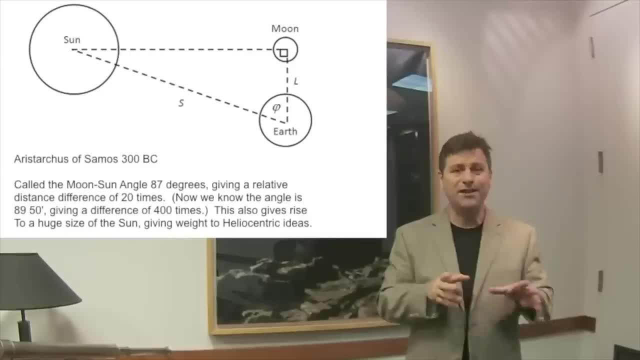 87 degrees, So he was able to roughly get about 1 degree. Remember that your thumb held at arm's length is about a degree. So he used a similar method or something more accurate than that, but he got about 87 degrees between the Moon and the Sun in the sky. 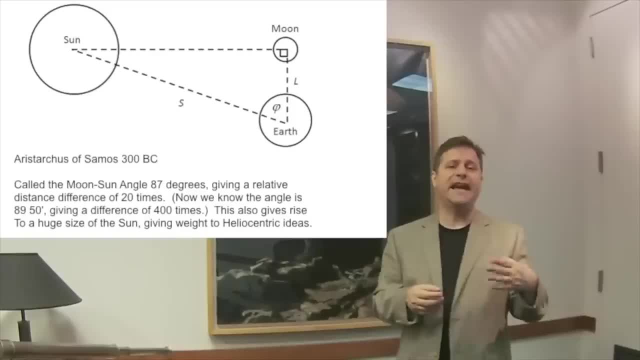 Well, at quadrature or when the Moon is at first quarter, the real angle is about 89 degrees in 51 minutes. so it's a little bit closer to 90 than Aristarchus actually measured, But let's go with his measurement If the angle of 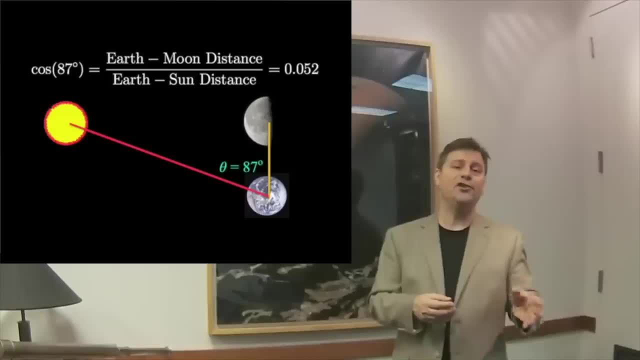 measurement is 87 degrees, then the ratio of the Earth-Moon distance compared to the Earth-Sun distance is about 1 to 20.. Specifically, the Sun's distance is about 19 times that of the Earth-Moon's distance. So, Aristarchus. 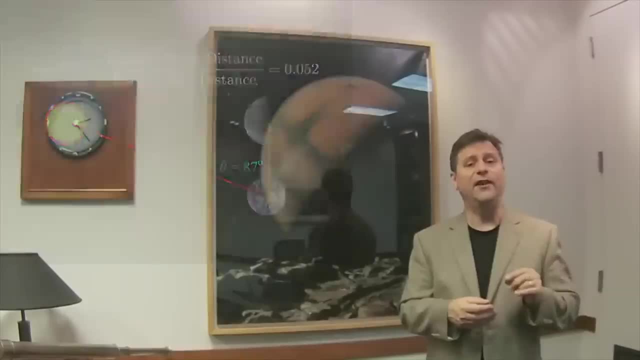 found out something very important. He found out that the Sun is much, much, much further than the Moon. Now he could also turn this around and say: wait a second. if we look in the sky and we look at the Earth and the Moon and the Sun, well, they look to be the 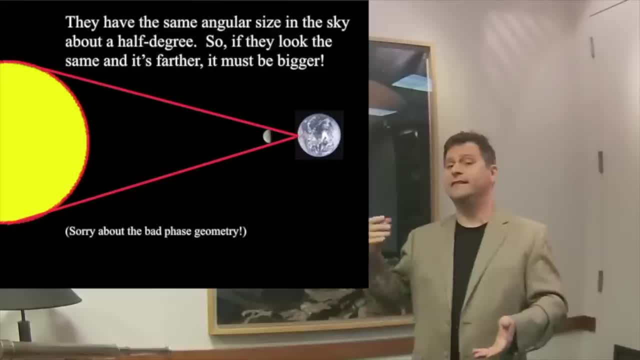 same size in the sky. So therefore, if the Sun is 19 times further than the Moon, it has to be 19 times bigger. So that's the nature of angular things that subtend angles across the sky. So he knew that the Earth, that the Sun was really. 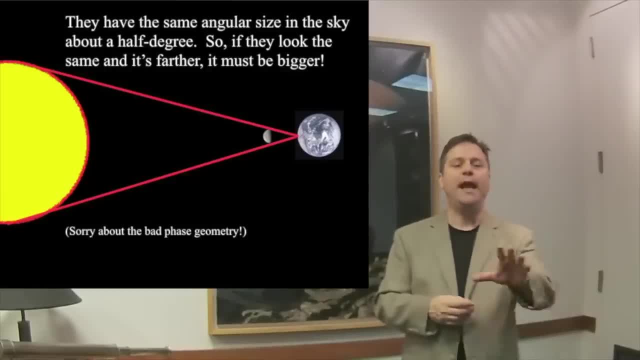 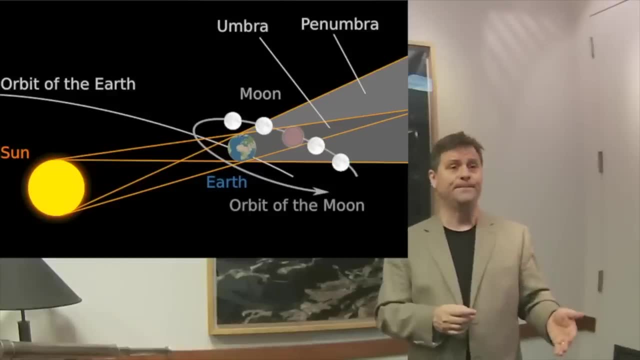 big. He said, well, wait a second, how big is the Moon? And we thought, hey, let's go back and look at those lunar eclipses again. And if we look at the lunar eclipse, he actually timed how long it traveled through the shadow, and specifically, 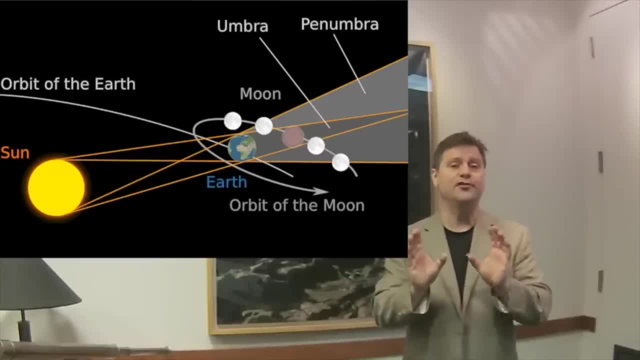 from the first contact of the umbra of the Earth's shadow, the darkest portion, the first contact, until it went completely into the shadow- and then timed the duration of the eclipse And Aristarchus determined it was roughly about twice. So he 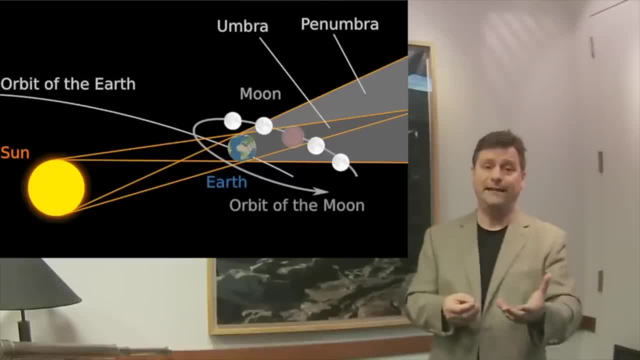 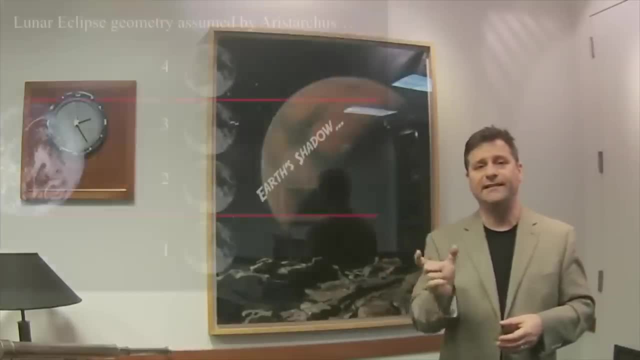 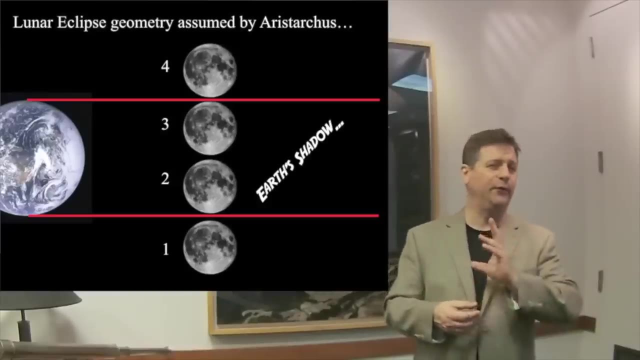 thought that, because the length of totality of the lunar eclipse was about twice that of the time it takes to go from first contact to second contact, then he determined that, roughly, that the Sun, that the Moon, is about half the size of the Earth. Well, this assumes something. It assumes that the shadow of the Earth is. 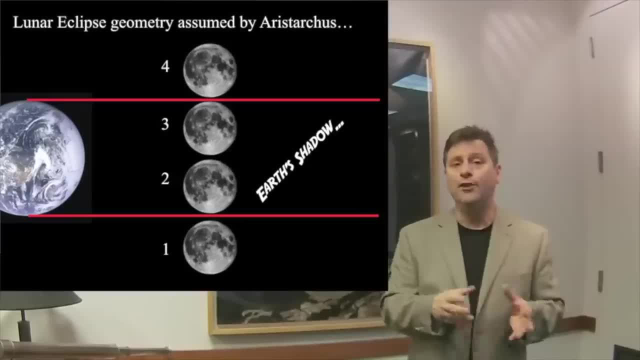 linear and goes out for a very long way and doesn't taper. We know it tapers. So the Moon's shadow tapers because the Sun is big, and so there's a place far behind the Earth where it does not cast a shadow. 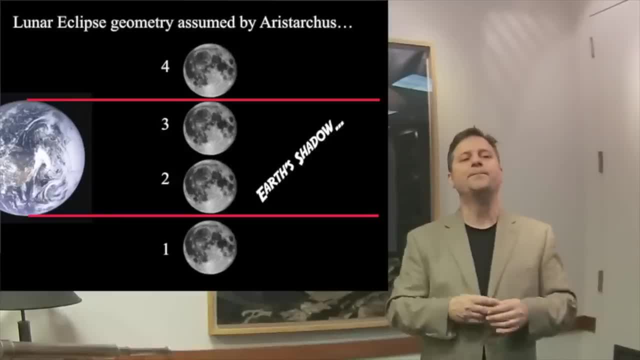 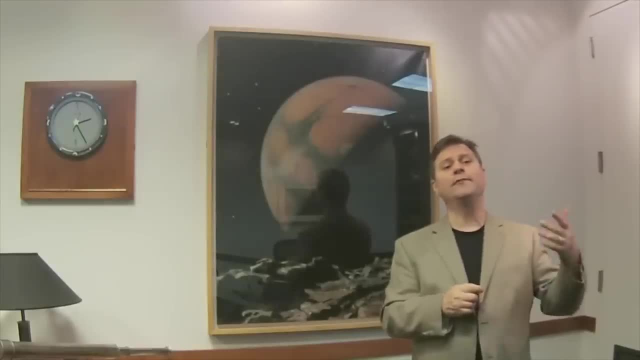 Anyway, but that wasn't what Aristarchus thought. Aristarchus said: well, wait a second. The Moon is about half the size of the Earth. That's interesting. And if he determined that it was about half the size of the Earth? 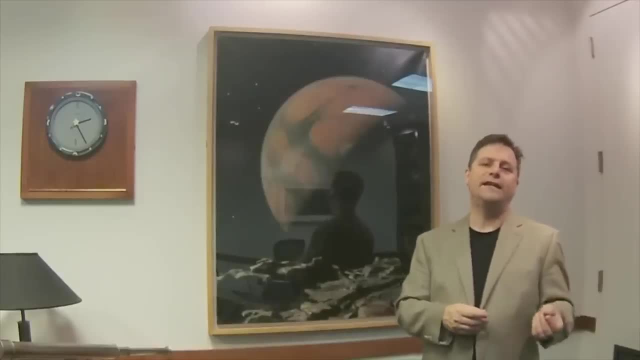 then he could turn that around and determine that about twice times 19, he determined that the Sun was at least about 40 times the size of the Earth. That's a really interesting discovery. So he found something really fascinating with that and that helped him. 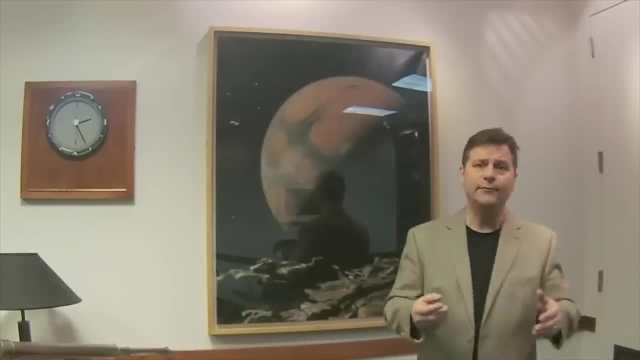 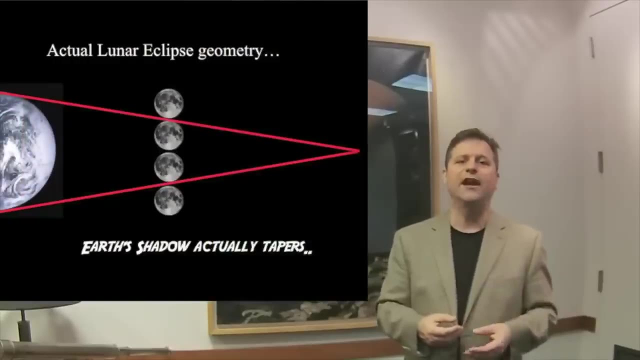 But he only did this with totally biased eyeball, with very rudimentary measurements, and actually determined some very important parameters. But today we know that the Earth's actual size is about four times that of the Moon. So when the Moon is in the shadow, it's actually 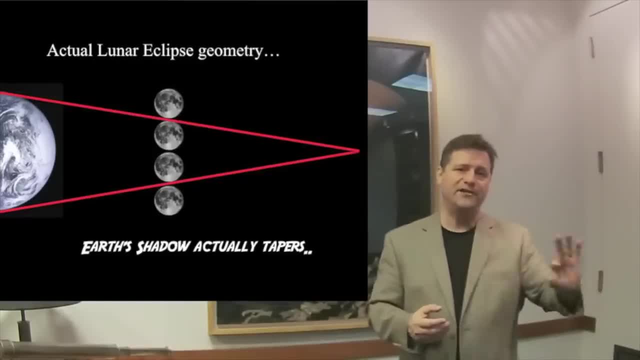 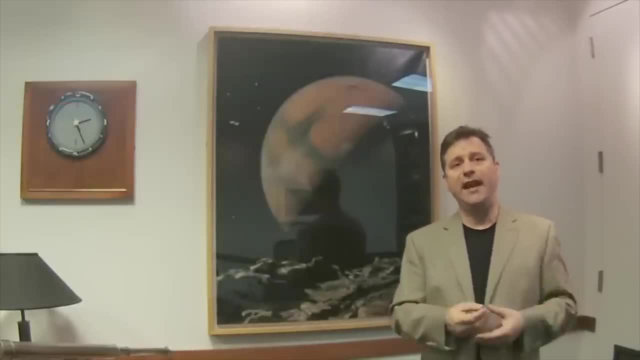 a smaller object and the shadow of the Earth actually tapers to a point, so that's why it can travel so quickly through it. So what Aristarchus did is he used angles between the Moon and the Sun and he determined they were the same angular size. so he 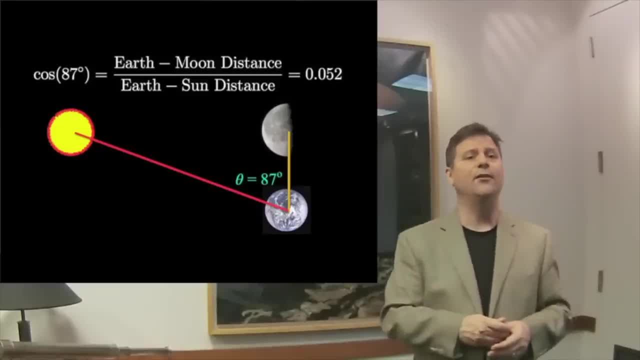 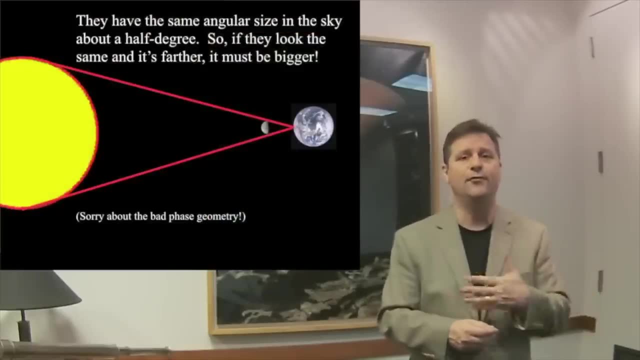 determined that the Sun was much further than the Moon. He also determined the size of the Sun based upon the size that he thought the Moon was, based on how long it took to go through a lunar eclipse, And you could even use Eratosthenes' description of the size of the. 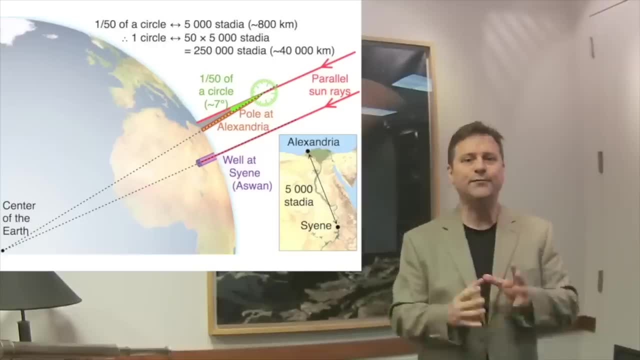 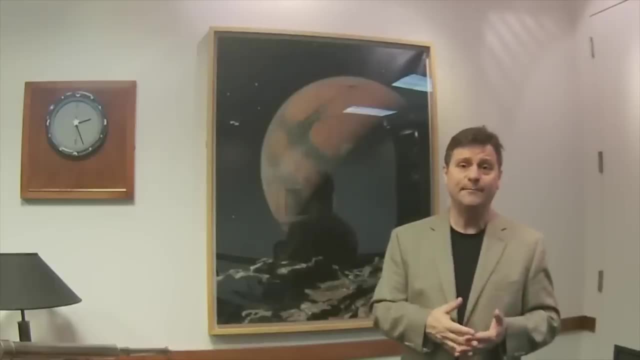 Earth in order to get the relative sizes of all of them. So that's really interesting. Well before 200 BC it was understood, at least to a pretty good guesstimation. Now Aristarchus' measurements were off by pretty considerably, but that's okay. 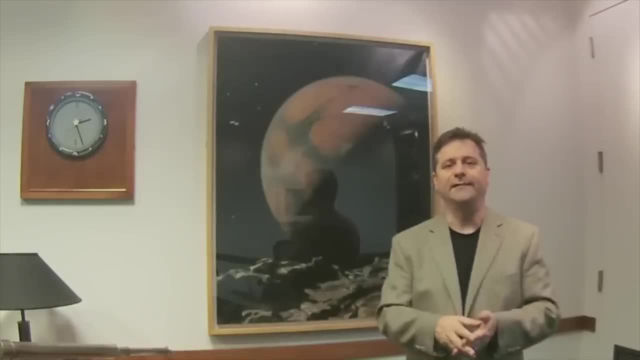 We have to give him props for trying, because who else does this kind of thing? And basically the true Earth-Sun distance is about 400 times that as the Earth-Moon, So he's off by a factor of say- oh, I don't know- 20, but 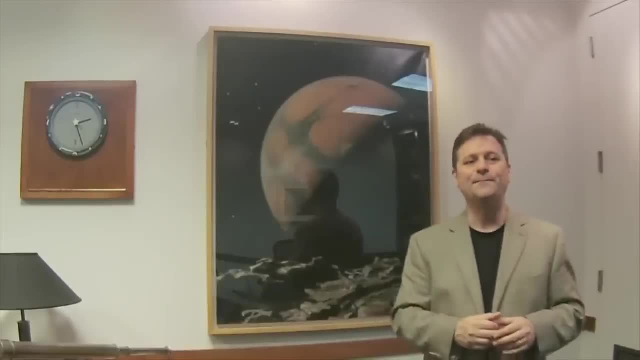 that's okay. Let's let him live with that. He did great, But what we did learn is that the Moon is closer to the Earth than the Sun. We also learned that the Sun is much, much, much larger than the Earth, and it's much larger than the Moon. 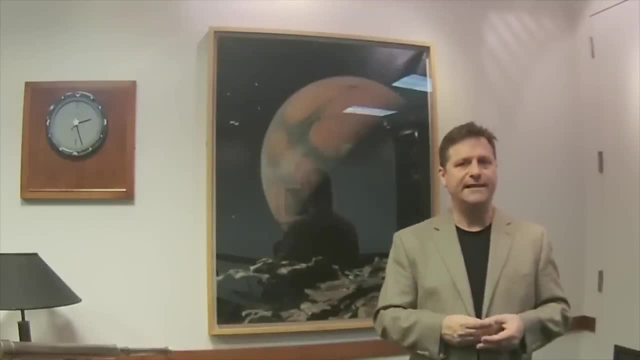 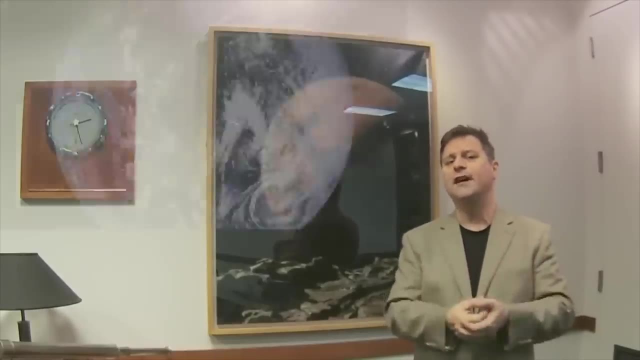 So this brings up some very interesting questions and points, And one of them that came about later, or at least in the contemporary moment, is the great debate about whether or not the Earth should be at the center of the cosmos, And we're going to discuss that shortly. 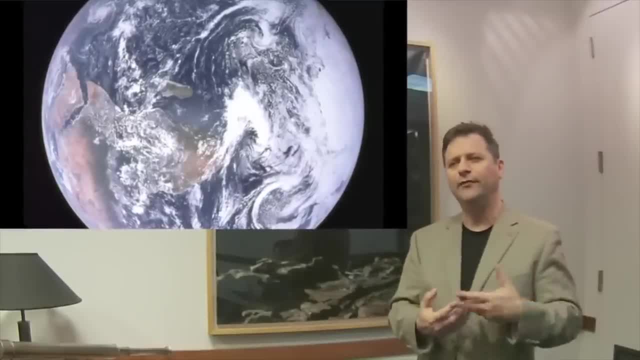 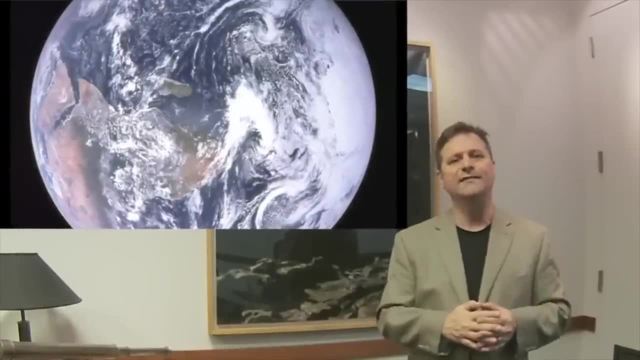 But we can look at this and say, well, the Sun is really a lot bigger than the Earth, so shouldn't it be at the center of everything? And that makes kind of sense, I guess. but that doesn't actually prove anything. It says: 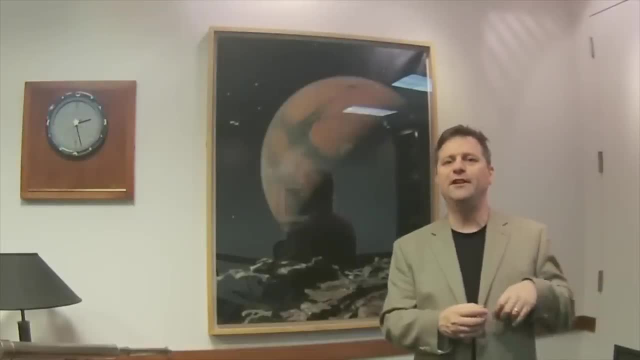 it should be, but that doesn't necessarily mean it is be, And the should and is are very, very different objects. So let's actually discuss that next time when we start to go down the rabbit hole of how big, how we know. 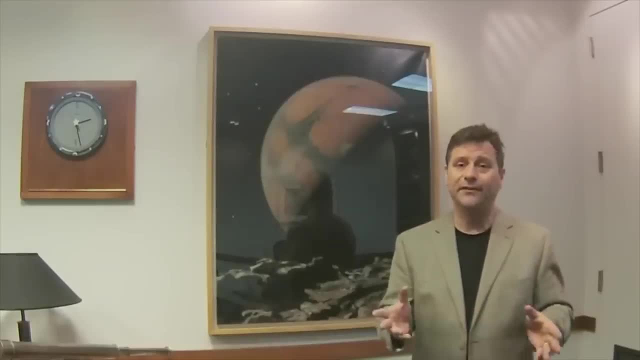 that the Earth actually moves in the sky, Because I know that you don't feel it Occasionally. people say, well, did the Earth move? And that's an interesting question If you happen to live in an earthquake zone. yes, it moves occasionally, But we can also think that 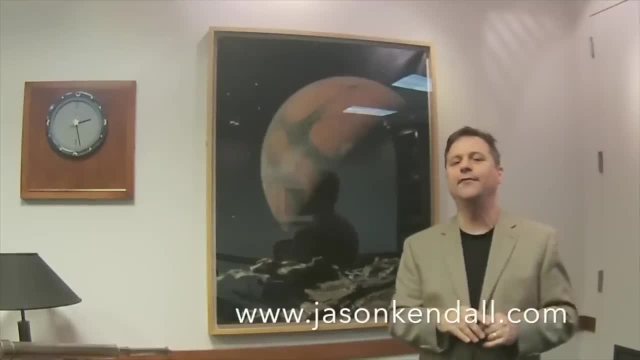 how do we know that the Earth is actually moving around the Sun? And that was one of the great questions of all astronomy. In fact, that led to the development of the calculus and it led to the development of modern day science, just by asking these simple questions. 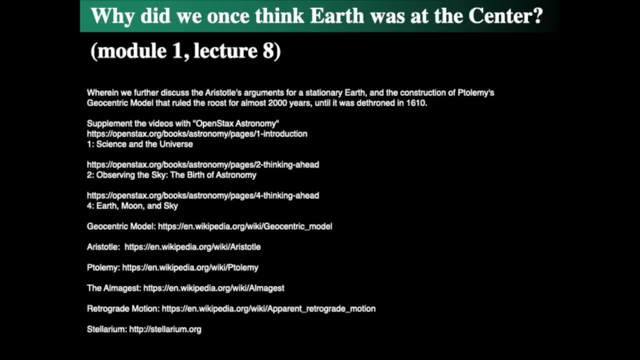 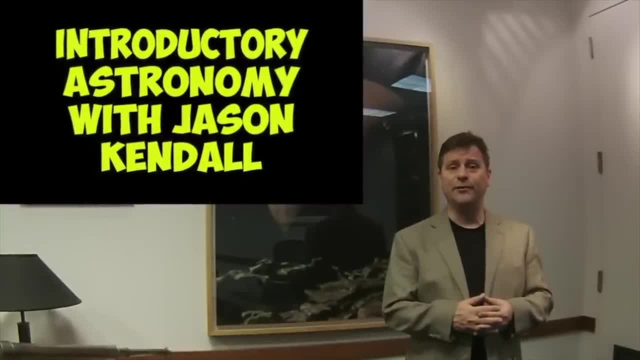 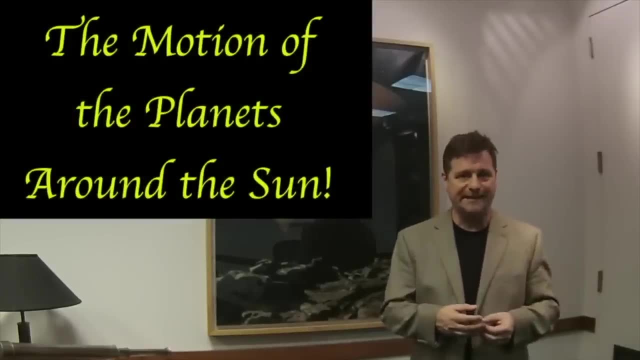 Okay, so we'll see you next time. Hello, this is Jason Kendall, and welcome to the next of my introductory astronomy lectures. Today we're going to be talking about the motions of the planets around the Sun. Around the Sun- Wait a second. We haven't known that forever, In fact. 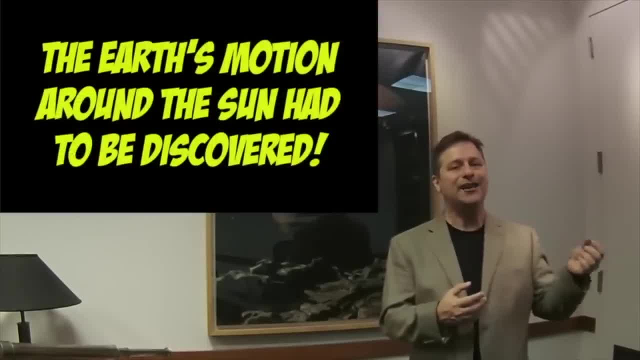 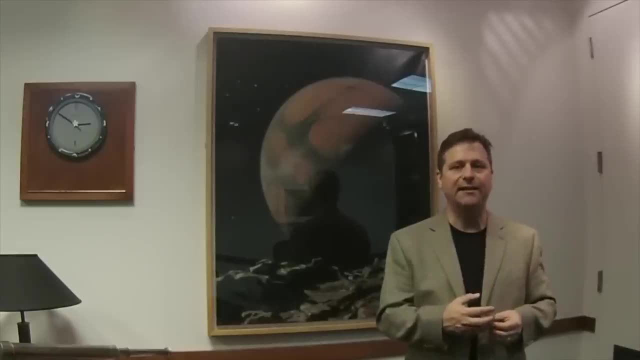 the object of looking and discovering that the Earth actually goes around the Sun is one of the central ideas to all of physics and, frankly, modern thought. The discovery of the Earth's motion around the Sun and the development of thought that led us to that are probably some of the most important things. 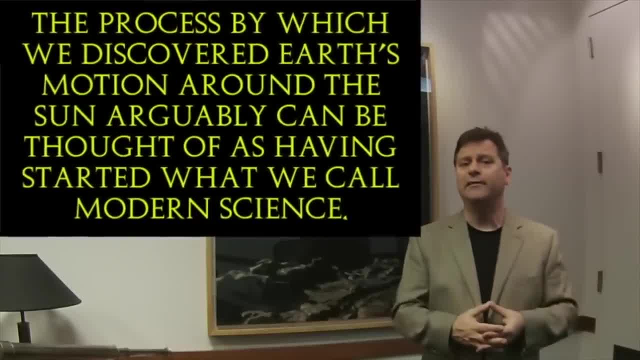 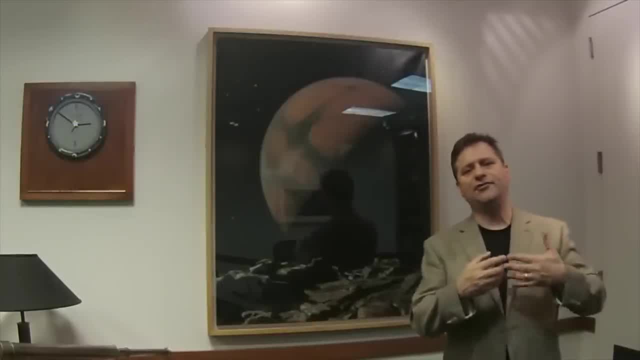 in what we call Western thinking And in fact, it traces the beginnings of what we call science. Alright, so what are these motions? Alright, well, first, let's actually start off with some basic things. Well, when we look up at the night sky and we look, 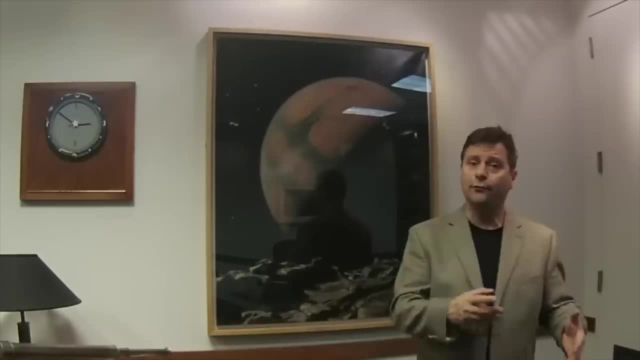 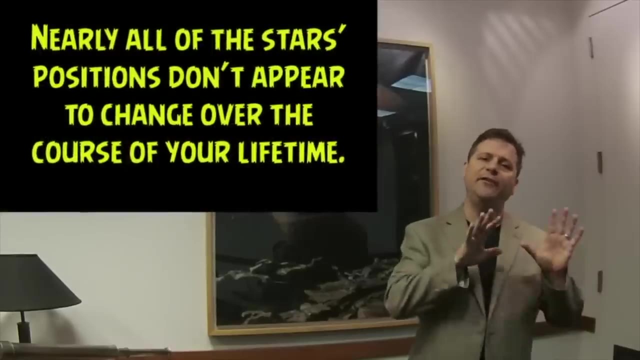 year after year after year, we see that the stars rise in the east and set in the west, and they go at a certain angle, depending on your latitude, but they always do that and they always seem to be staying fixed with respect to each other in the sky. And those are the stars. But then we 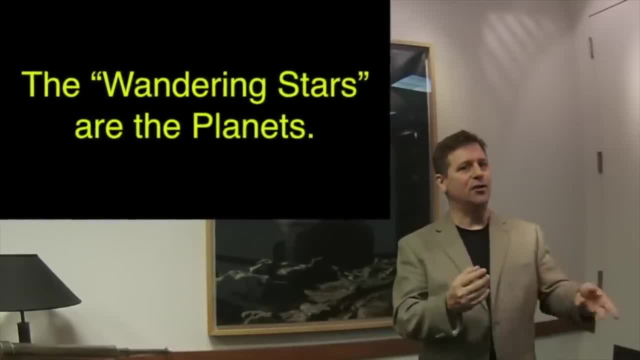 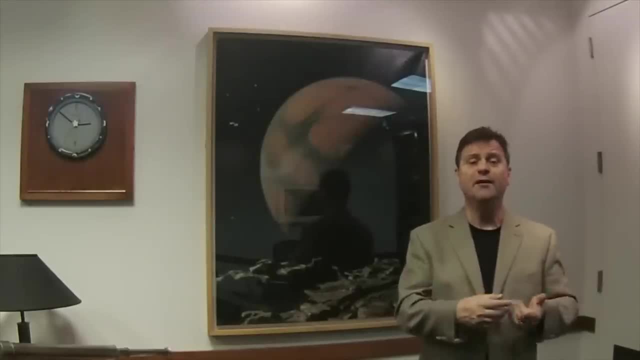 find that there are wandering stars, some stars that don't stay fixed with respect to the others, And, in the classical terms of the wandering stars, we have the Sun, of course, Moon. wow, it's up there. we have the Sun, the Moon, we have Mars, Mercury. 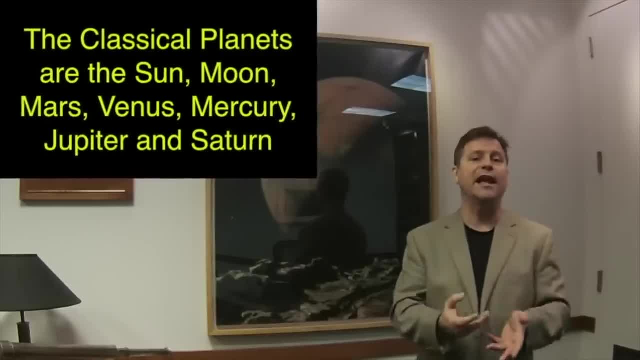 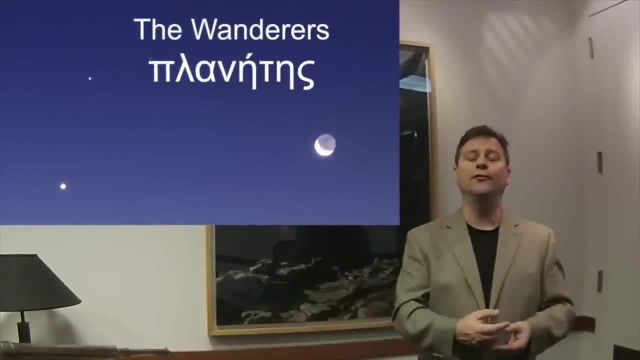 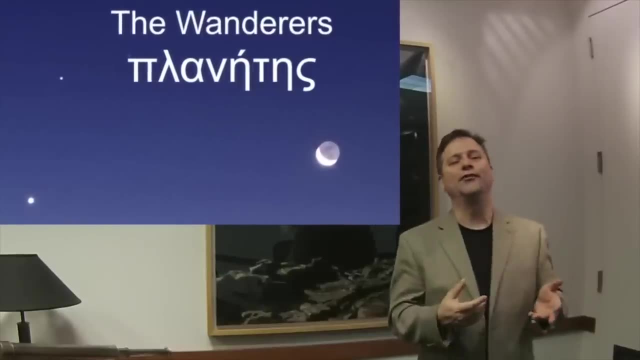 Venus, Jupiter and Saturn. So those are the classical planetas, the planets. And planet in Greek indicates wanderers, which means wandering stars. so the word planet, the oldest meaning for that word, is wanderers, wandering stars. So what are the wandering stars? The wandering stars also. 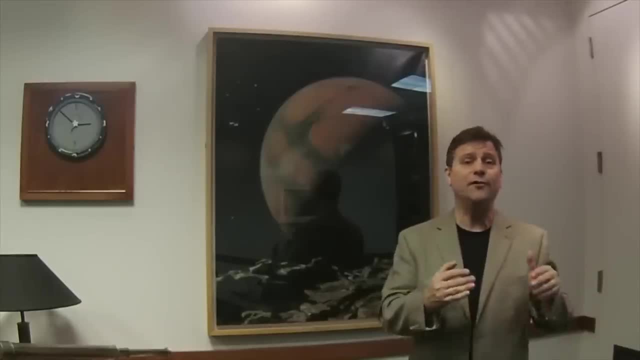 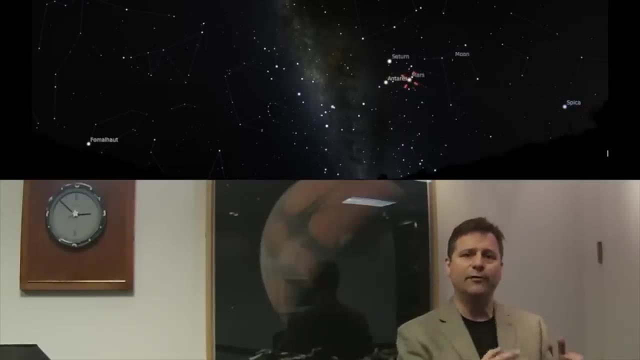 appear to rise in the east and set in the west. just like all the other stars, however, they steadily drift eastward every day, So over a very short period of time, over many days. if you watch them day after day after day, you will see. 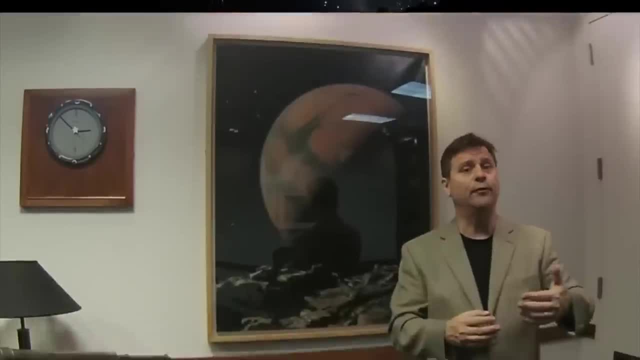 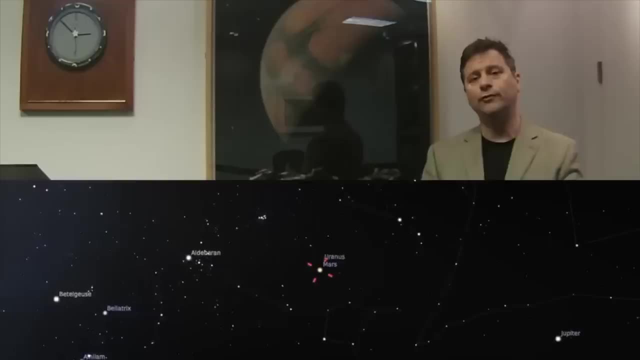 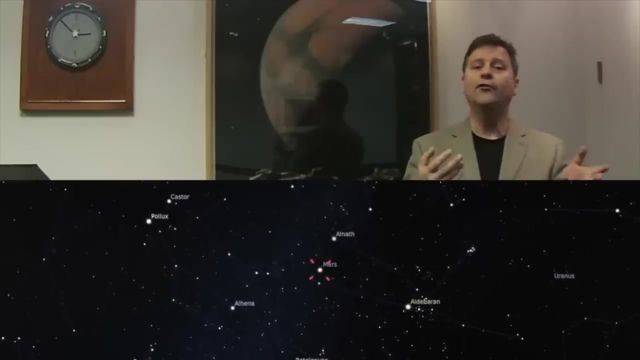 them slowly drifting eastward And occasionally they will drift westward on what we would call retrograde motion. So retrograde motion is the drifting slowly to the east of the planet and occasionally it does a backward loop that we would call retrograde motion, And Mars shows this quite explicitly. 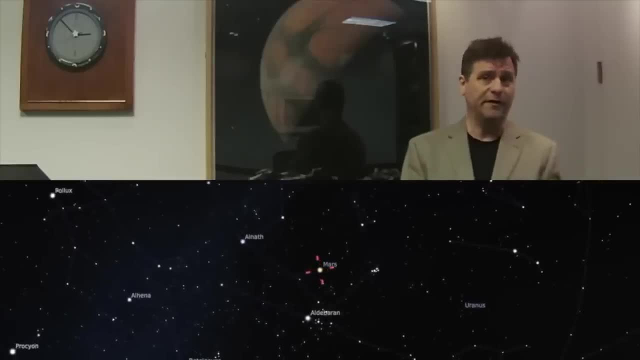 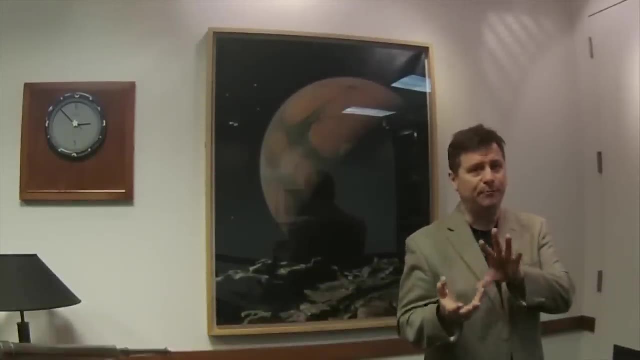 Mars' retrograde motion was one of the great, important things to study in terms of the motion of the planets around the Sun. Alright, we also know, or at least appear to know, that the planets reflect light. They don't have their own. 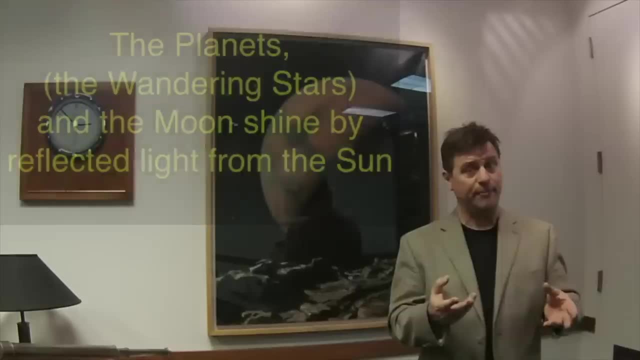 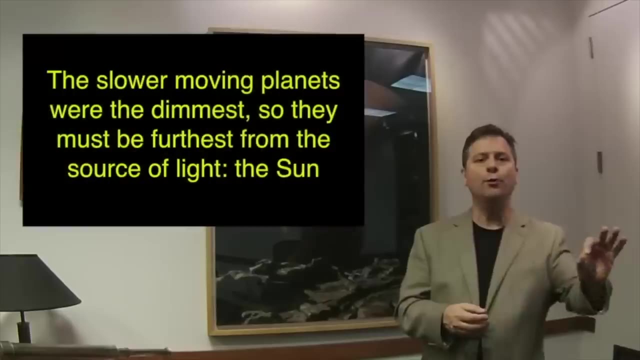 light of their own. Now that is an interesting statement in and of itself, and it's hard to really determine that from the sky. but the ancients thought and noticed that the slower moving planets were also the dimmest. So they reasoned that hey, if they're the dimmest, they must. 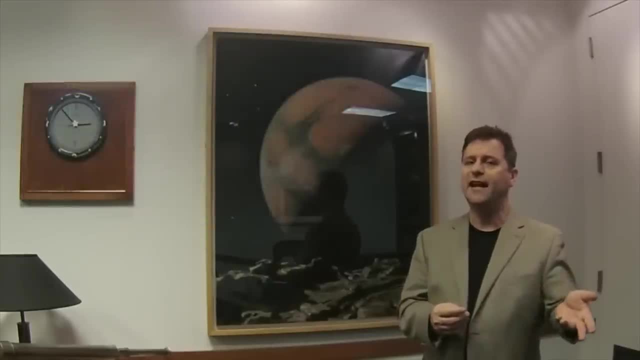 be the furthest, And if they're reflecting light from the bright Sun, which they knew was happening with the Moon, if the Moon was reflecting light, then the other planets may be reflecting light too, And they're very close with respect to the stars. so therefore, 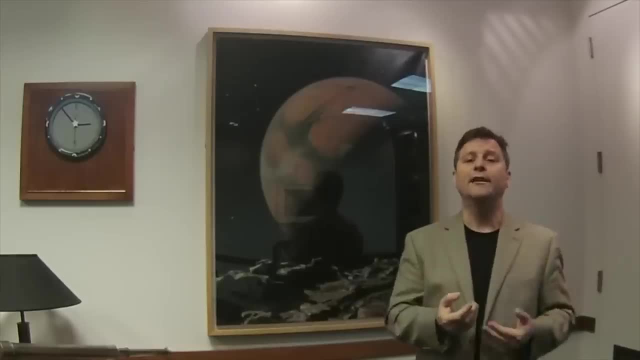 if they're farther from the Sun or farther from the Earth, then therefore they would be dimmer. So that's an old argument that the ancients knew about as well. So this led to the direct trying to understand the influence of these things and what they 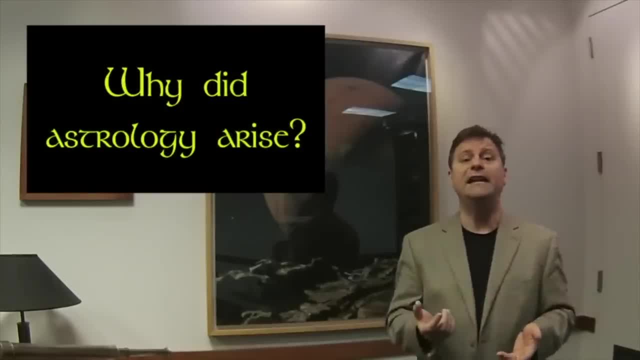 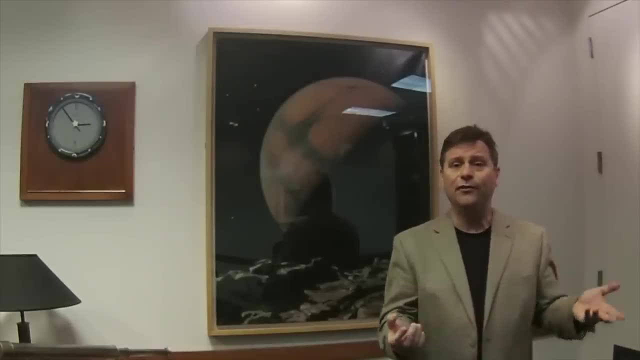 meant Because there was a difference between the motions of the planets and the stars and the things on the Earth. Because the ancients knew, and everybody's known, that the stars have always risen in the East and set in the West, And they always have done this. So 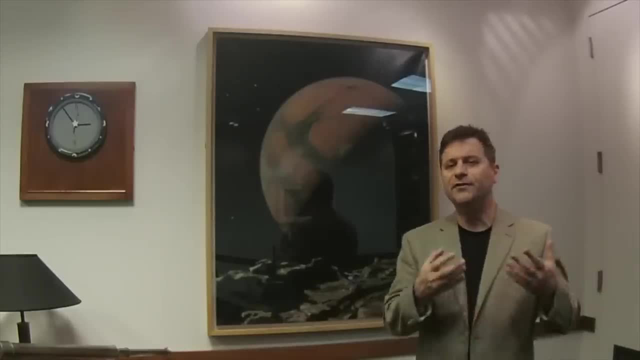 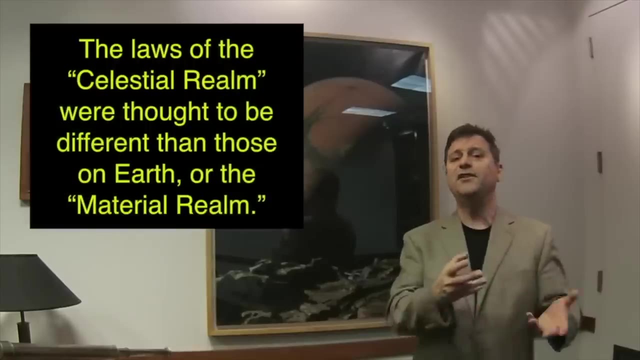 planets' motions are extremely regular, So there's a difference between what happens in the celestial sphere and what happens in the material world. The material world we'll call the Earth, And so to ancient philosophers and scientists of the day, we wouldn't really call it science, trademark science, but science or what we would. 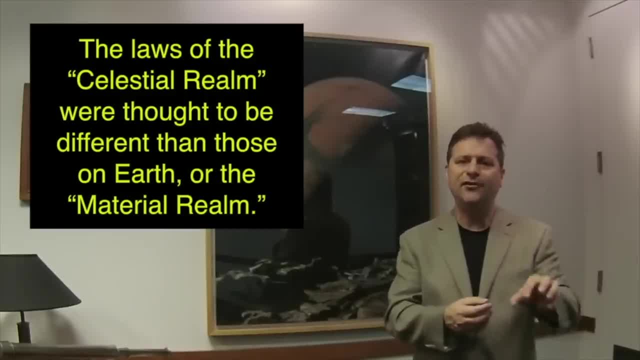 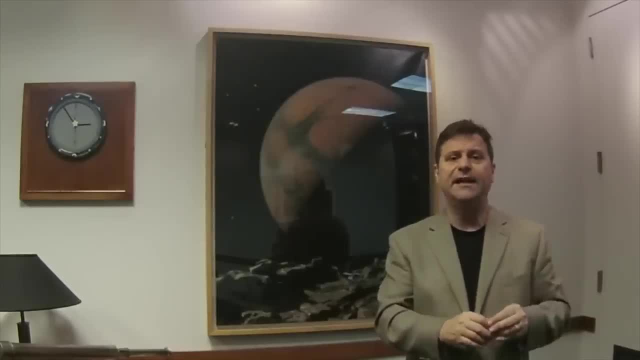 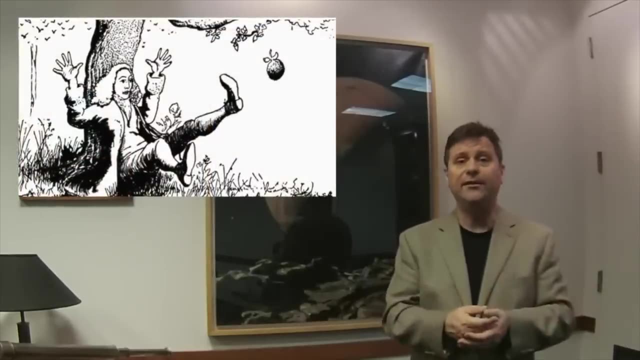 call the beginnings of science. They had the idea that you actually had to. the operating principles for the Earth were different than that for the stars. In fact, they didn't seem to behave the same at all. So, for example, you take an object like an apple and you 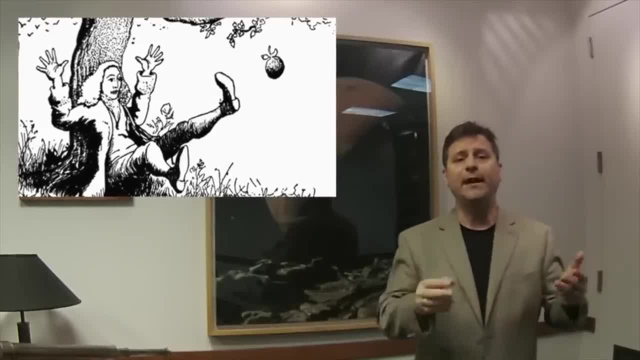 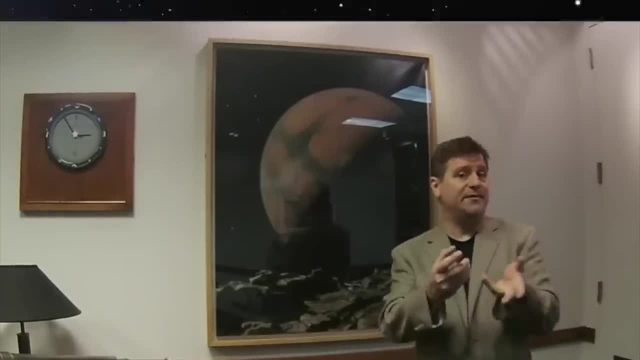 go up a tree and if you take an apple and drop it out of a tree, guess what happens? It falls towards the Earth And it's free. so it falls. Well, look at Mars in the sky. Mars must be free of the. 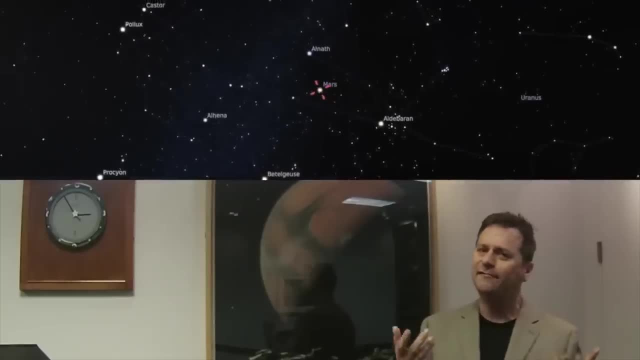 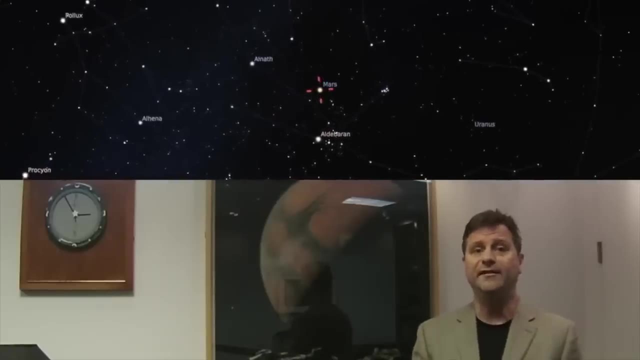 stars? And if it's free of the stars, why doesn't it fall to the Earth? That's a really interesting question. Same with Saturn, Same with Jupiter, Same with the Moon. Why doesn't the Moon simply fall to the Earth? 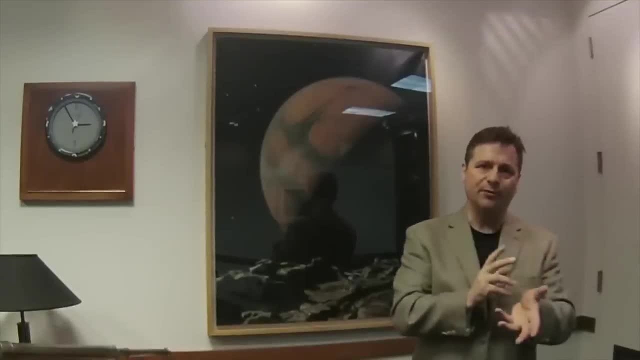 It stays up there for whatever reason. So, whatever principles act on the Earth, appear to be acting different, have a different set of principles that work with respect to the planets and stars, And so, therefore, people who studied the stars weren't deemed these wonderful notion of what we call the astronomer. 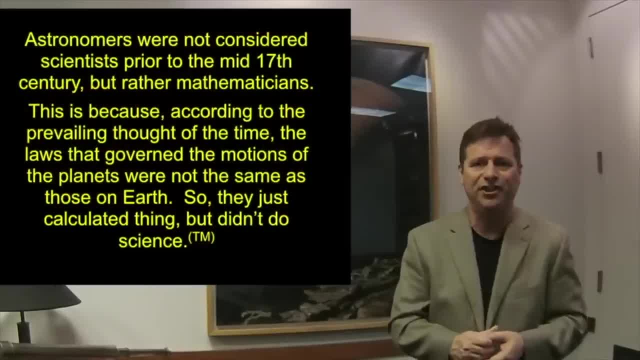 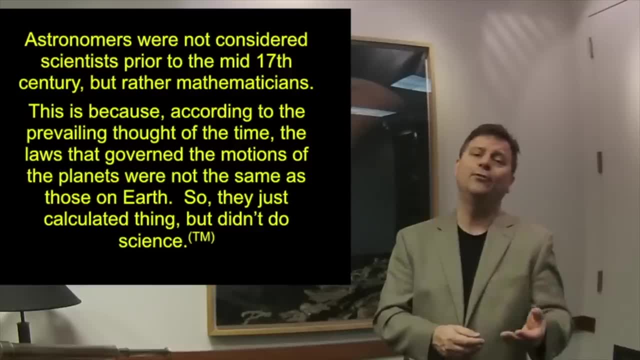 They weren't even called scientists. They weren't even called physicists. They were called mathematicians. They were mathematicians who calculated things, who calculated the length of the day and the length of the year, And the principal reason for studying the stars was calendars, So you knew when to plant things and when to do things. 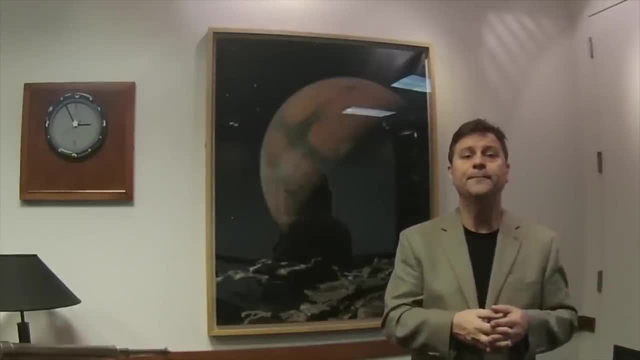 when important annual events would occur and when important monthly events would occur, And so you would also. then, if you were making calendars, you would notice that there were important events that happened at certain times. So, therefore, if those important events coincided with the apparent positions of the things in the sky, 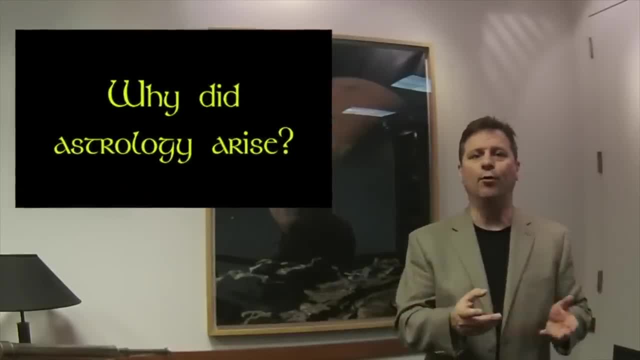 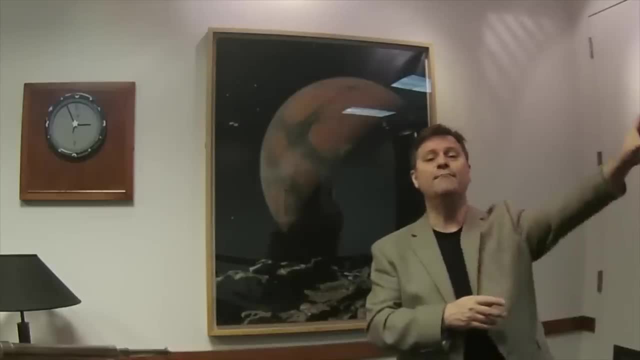 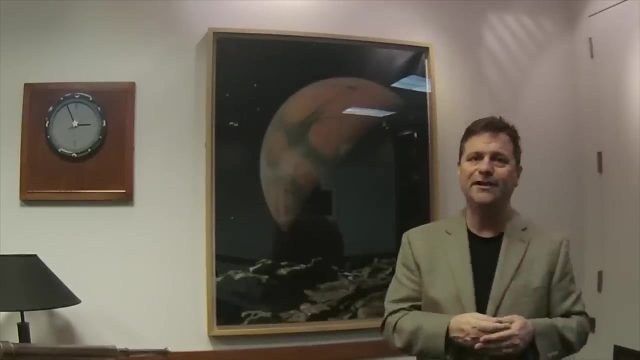 then they might be related, And thus was born astrology. Astrology is the apparent or supposed link between the motions of the planets and the stars and what happens down here on Earth. Well, just gotta go to show you that astrology is simply a construct. It is a way that people have looked up in the sky and 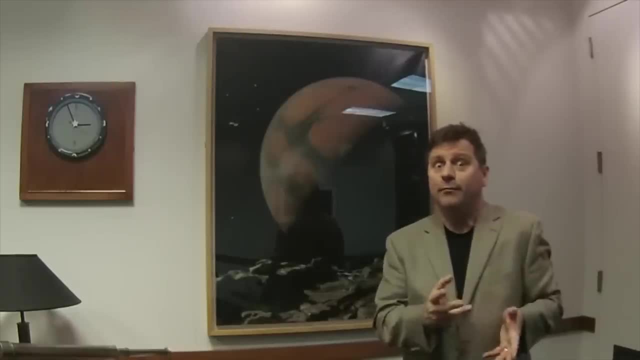 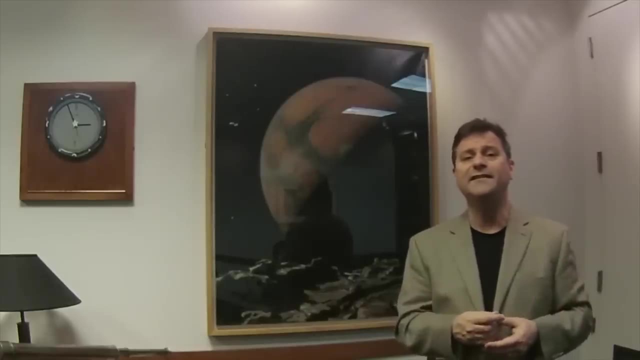 looked up there and said, wow, that's happening now. That must be related In the same way that when you look up in the sky on a cloudy day, on a summer, wonderful day, looking up, you see faces and dogs and cats and 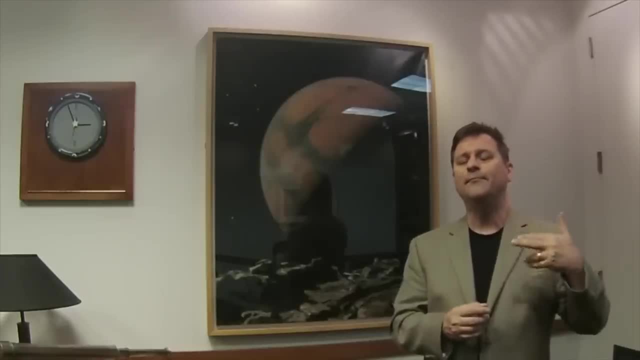 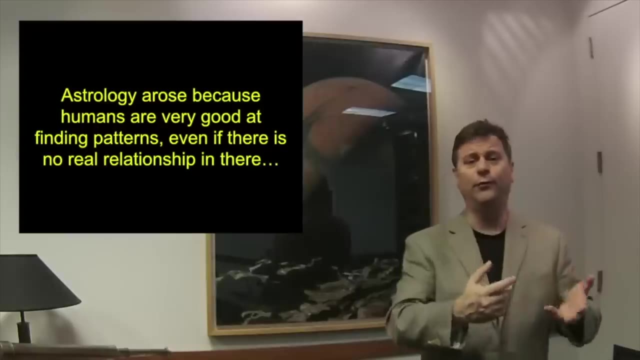 kittens and shapes in the clouds. You always see faces in the clouds, but you never see clouds in faces. That's because we're really good- Humans- are extremely good- at finding patterns in things. So we found this pattern that seems to be there, but it isn't, So astrology is just simply a trick. 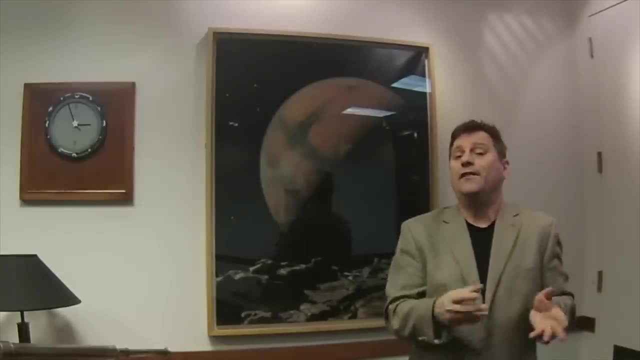 It's a way of saying when things are happening, And so, oh yes, you were born when Mars was ascended. Well, you can't argue with that. but there is no meaning to that, There is no influence to that. So today we now know that if two astrologers 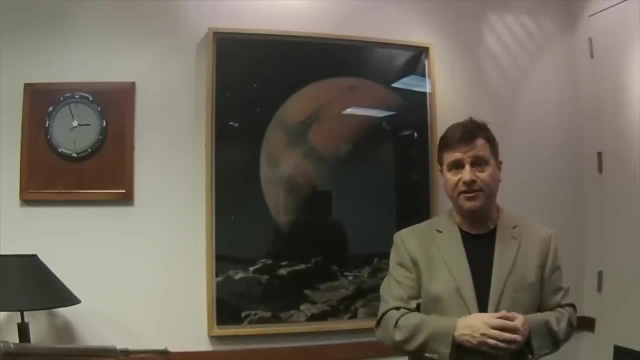 you ask five astrologers your opinion, you're going to get seventeen opinions. So they don't agree with each other. They have no way of agreeing with each other. But that's where astrology was born. Astrology was born by the extensive study of the behavior and movement. 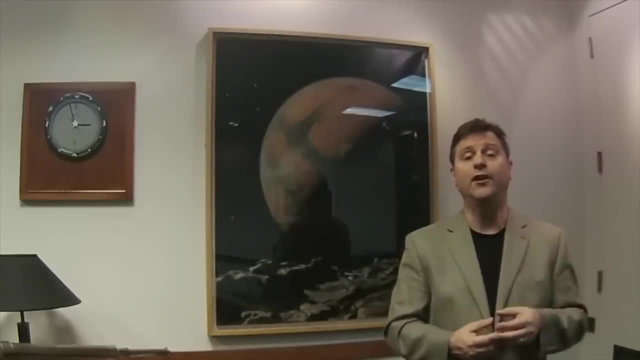 of the planets and the motions of these wandering stars. So let's give it some credit where credit is due, because it kept people looking at the sky and it was very important to determine calendars. So if we look at the sky and we try to determine what's up there and how it moves, we naturally want 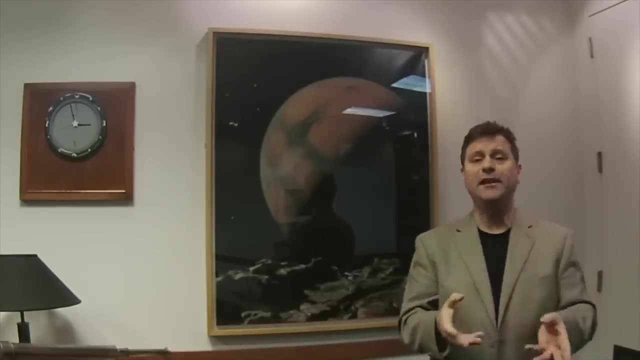 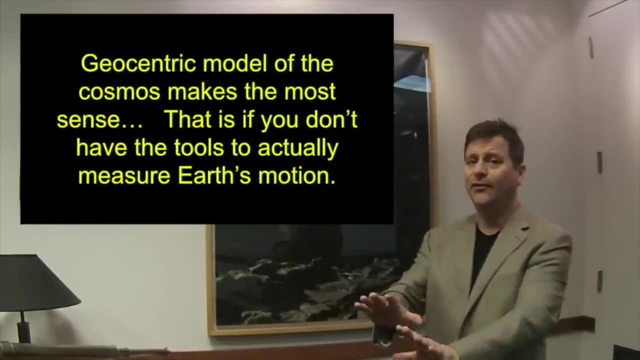 to come up with some sort of explanation for it, And that explanation that seems to be the most rational is the geocentric model, Not rational by what it really is, but rational by our experience. And rational by experience means we simply don't feel the Earth. 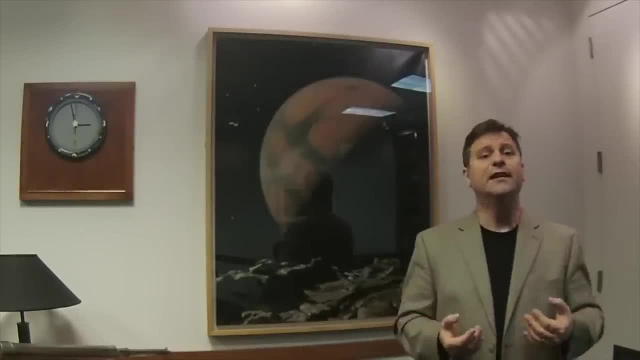 moving underneath us, And there's other arguments as well, that the ancients used to actually justify geocentrism and actually beat down geocentrism in its nascent beginnings. But let's actually look at that for just a second, because this is a very interesting set of arguments. 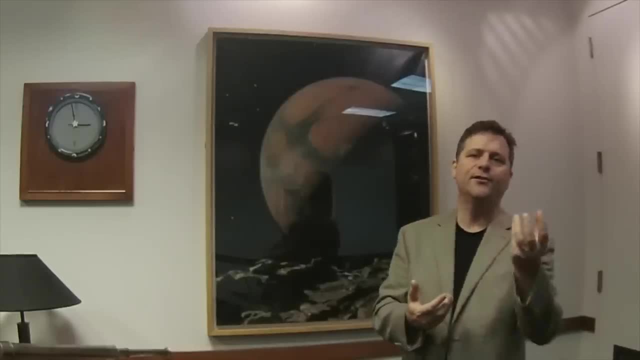 Alright, so in a geocentric model, meaning the Earth is at the center of the cosmos, this philosophy held that the Earth was at the center. Well, why did Aristotle, who was around from about 380 BC to about 320 BC, why did he come up with that? 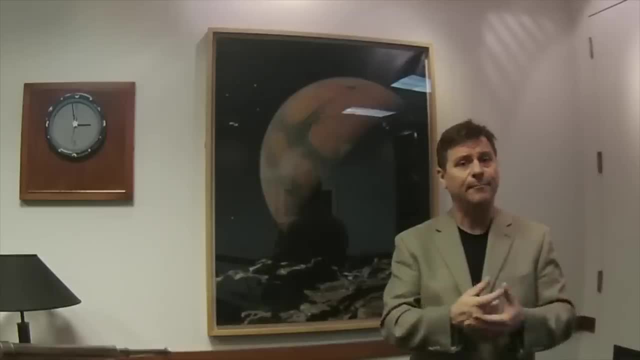 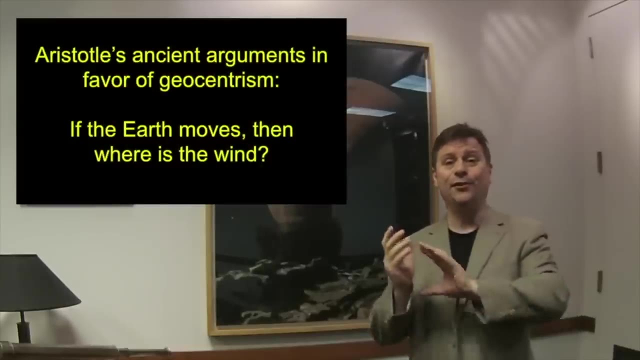 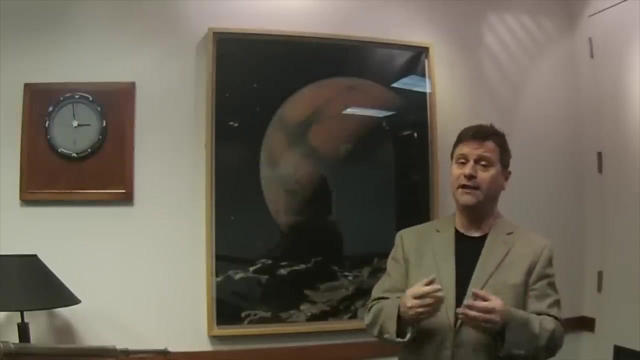 the Earth must be still, That it must not be moving Well. he used a number of arguments, And his first argument was: where's the wind? The wind, if the Earth was moving well, where's the catastrophic winds of us moving through the cosmos? Alright, that's a good argument. Where's the wind? 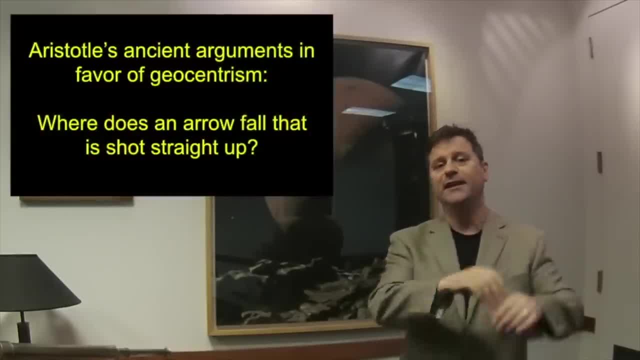 Second, let's say you take an arrow and they had archers back then. you take an arrow and shoot it straight up. Where does the arrow fall? The arrow falls straight back down at your feet. If the Earth were moving, then the Earth should move out from underneath the arrow and fall to the ground. 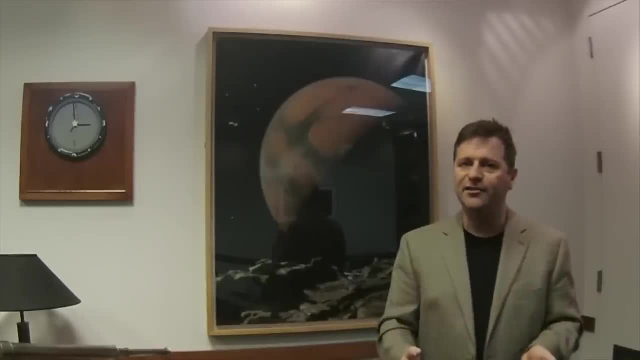 Hmm, that's an interesting thought. Why doesn't it do that? It doesn't do that because the Earth's not moving, or so Aristotle thought. Third, we can turn it around the other way: Build a tall building, go to the top of a tall cliff, and if you drop a rock? 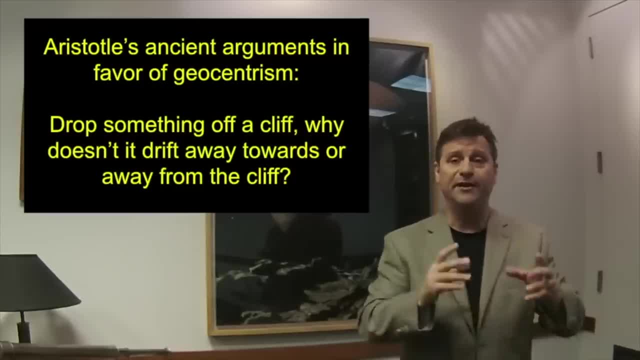 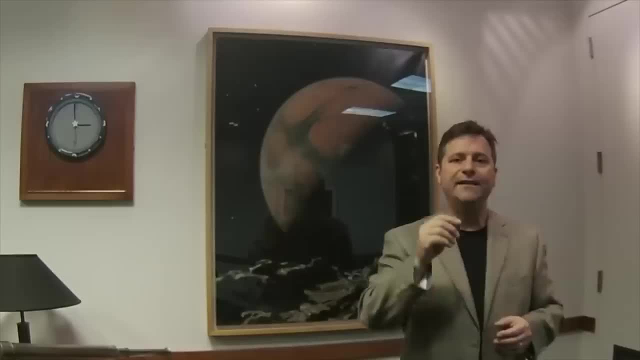 if the Earth was moving, or rotating for that matter, because everybody at the time knew it was round, didn't know how big it was until a hundred years later, in Aristotle's world. the Earth should then move away from it, And the rock would not plummet all the way to the ground. 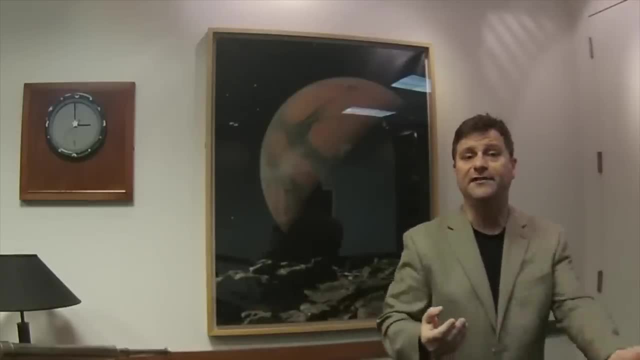 at the base of the cliff, but will drift either towards the cliff, if the cliff is to the east, or away from the cliff, if away from the cliff is to the east, if the Earth is rotating, Alright now, that's a very interesting set of arguments based on 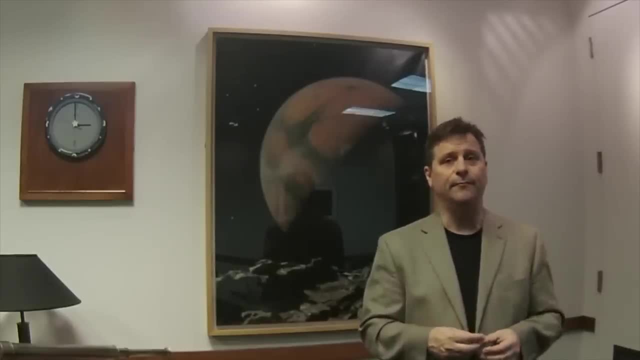 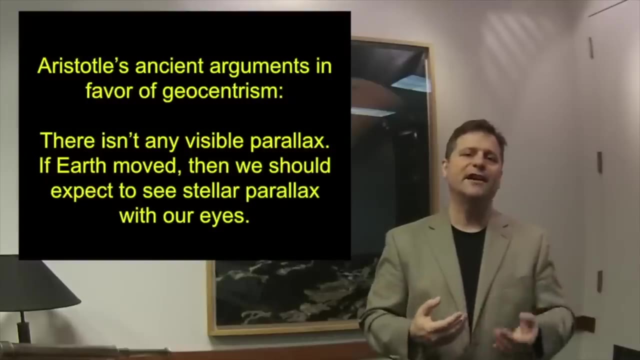 Coriolis. The next argument against geocentrism, or for geocentrism, which is interesting in itself, is parallax. Aristotle reasoned that if you don't see parallax in the sky, then therefore the Earth cannot be moving, And this is, as we've described before, an extremely difficult 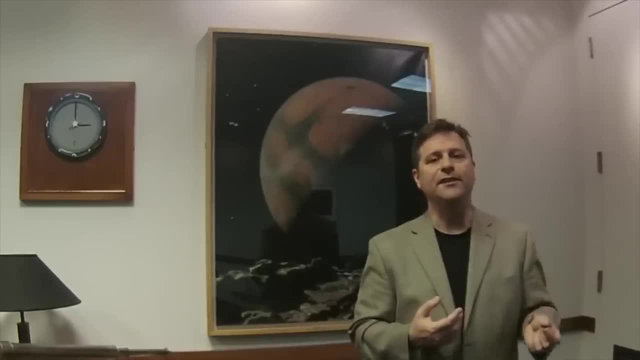 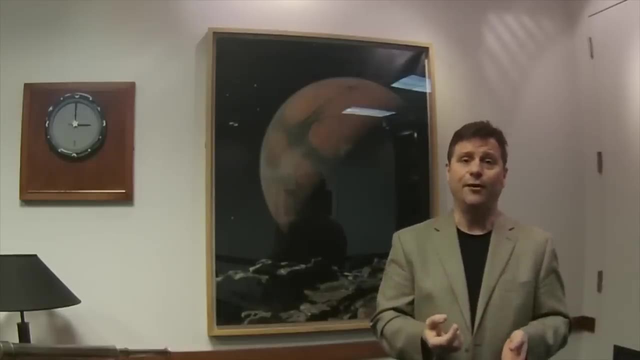 measurement to make and wasn't even accomplished until the 1830s, well over 2,000 years after Aristotle's death. So we can forgive him for not seeing it because the stars are extremely far away. Alright, the next thing that he had, those are some funny little arguments. one argument said that 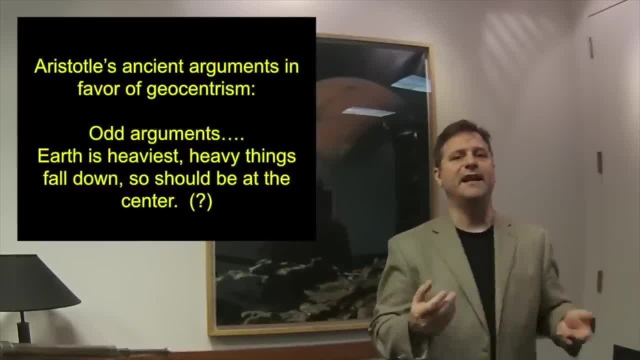 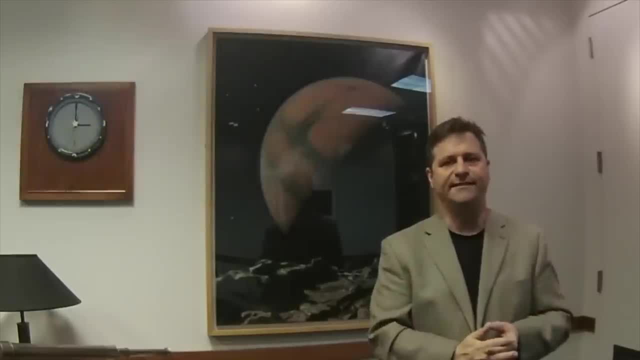 the Earth was the heaviest, and so if it's the heaviest, it must go to the lowest point, and the lowest point must be at the center of everything, because that's where the heaviest thing should lie is- at the center. It's kind of a 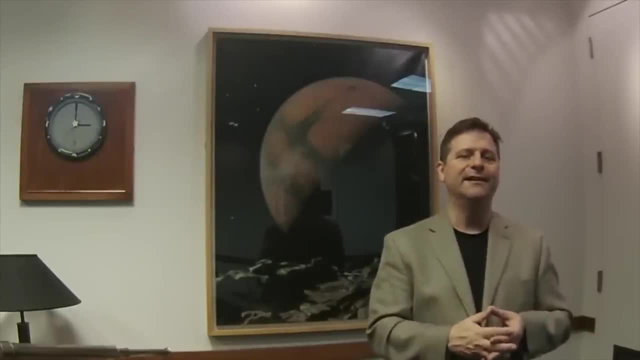 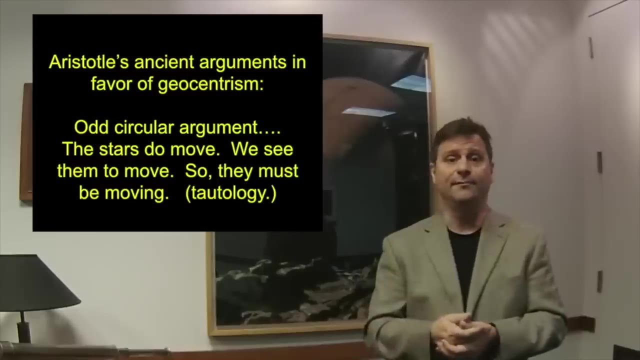 woo-woo argument, but we can live with it. And then he also said: now here's an interesting thing: the stars move. Well, we see the stars moving, we don't see the Earth moving. so therefore, the stars are moving, we're not moving, So we can look at. 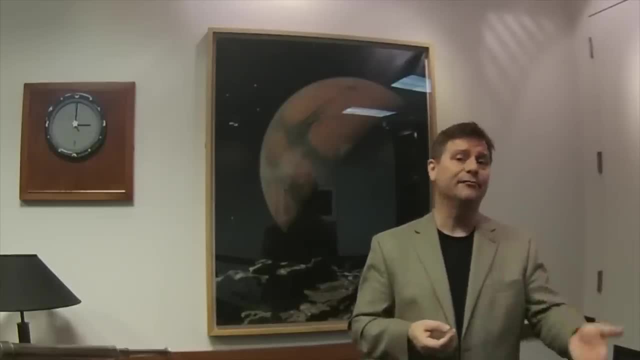 Aristotle and think there's a smart guy who came up with a lot of reasons in 360 or 340 BC as to why the Earth doesn't move Now, remember, technology that we have today did not exist for him, So his ideas carried a huge amount of weight and tended. 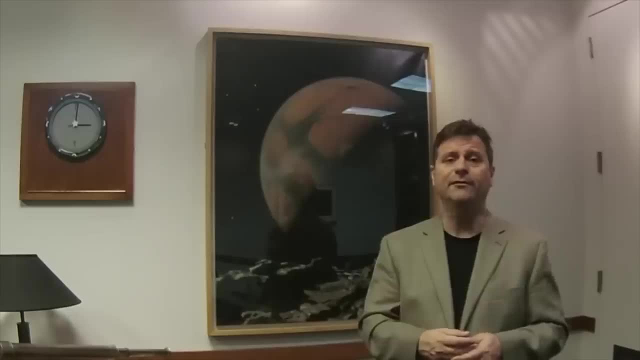 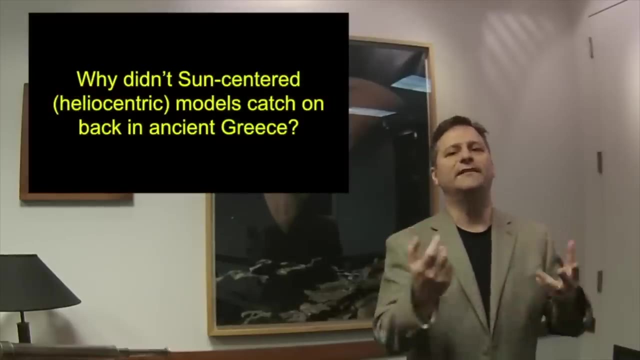 to actually tended to hold progress back for a very long period of time. Alright, so then let's actually look at some other things. Why didn't people say that the Sun was at the center? Didn't we just learn from the last lecture that the Sun is 20 times bigger? 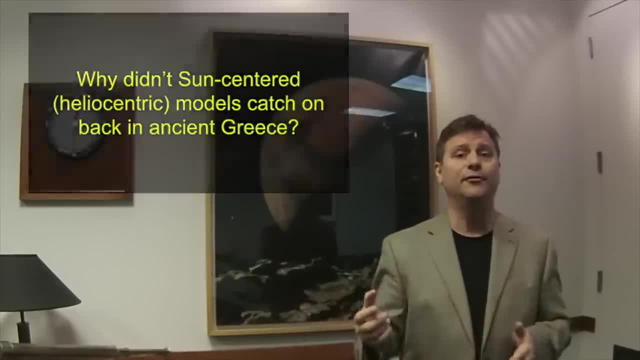 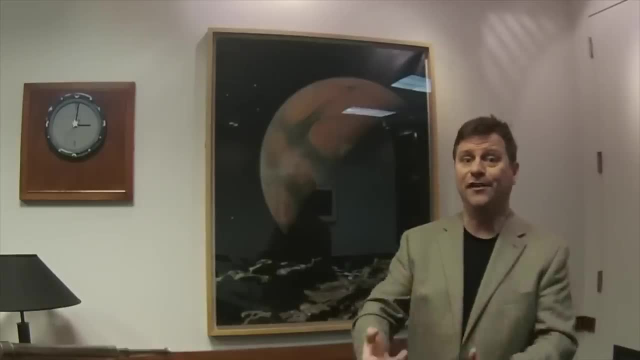 than the Moon. Well, it's 20 times bigger than the Moon and the Moon is half the size of the Earth. so it means it's actually. it's a huge, huge object. The Sun's really big. If the Sun's really big, shouldn't it be at the center? 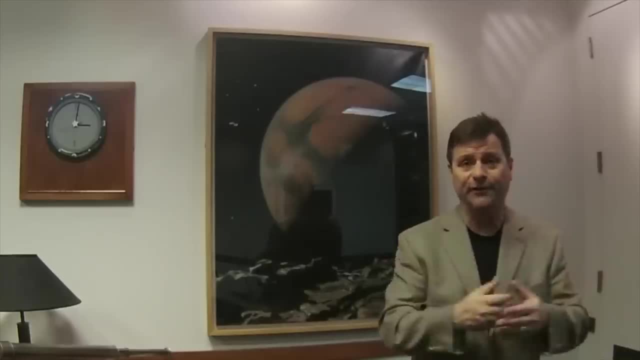 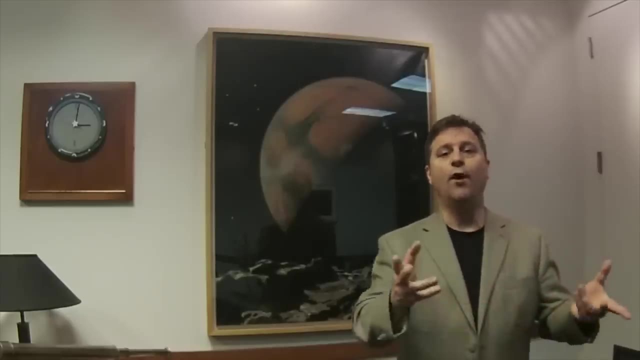 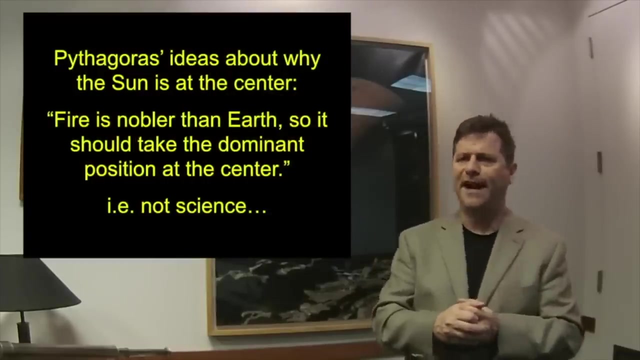 And people supported it, such as Pythagoras of Pythagorean theorem. Yes, he posited that the Sun should be at the center. Well, why did he say that? It's because fire is nobler than Earth, So therefore, fire should be at the center. 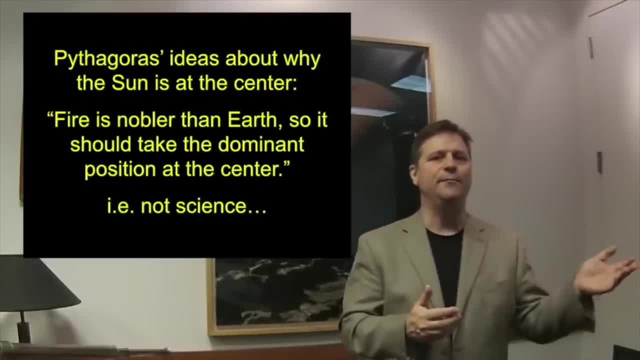 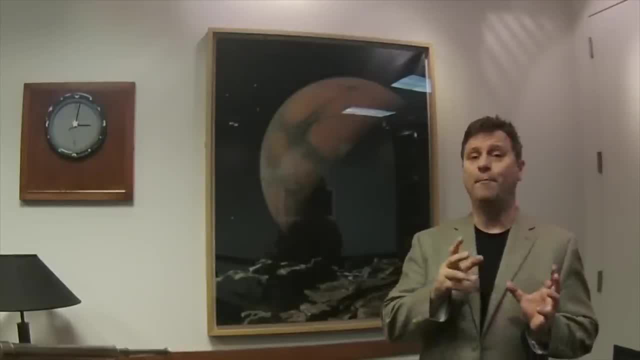 Well, it's not very scientific. so Pythagoras was known to be a little bit of a mystical woo-woo and if we look up at the Pythagorean solids, they were actually kept secret because they thought that these things were powerful, mystical. 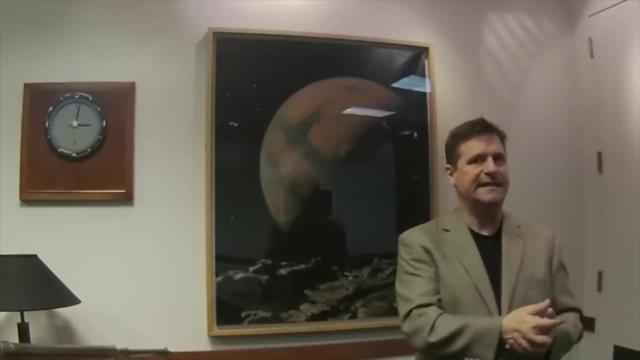 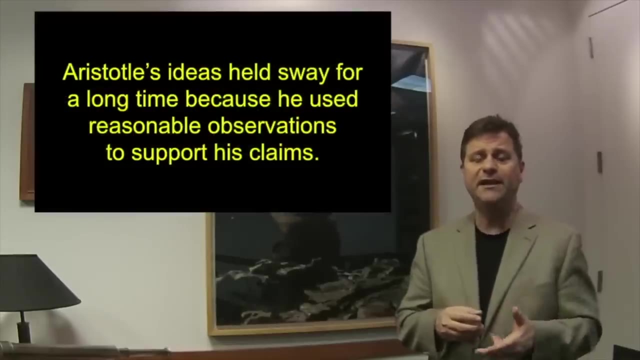 forces. So Pythagoras wasn't so much a scientist as a mystic and a mathematician. So Aristotle's ideas held deep sway because he actually tried to reason through the nature of the cosmos. That he got it wrong we can excuse. 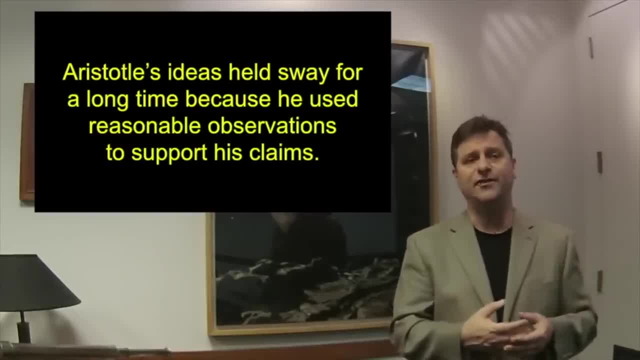 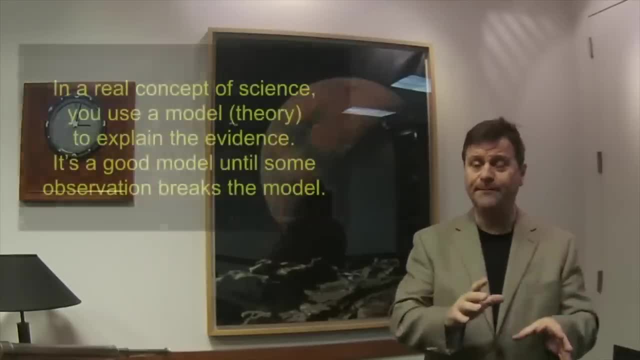 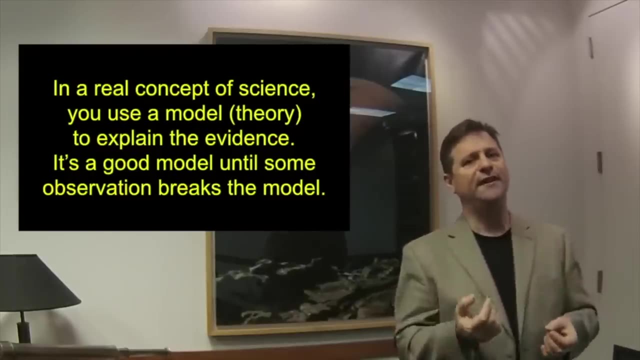 because of technology and because we have modern technology that assists us in understanding things a little bit better. But his models worked, and models that work stay put in science until there's something that breaks the model, And that's the important thing that occurred later. But let's actually find 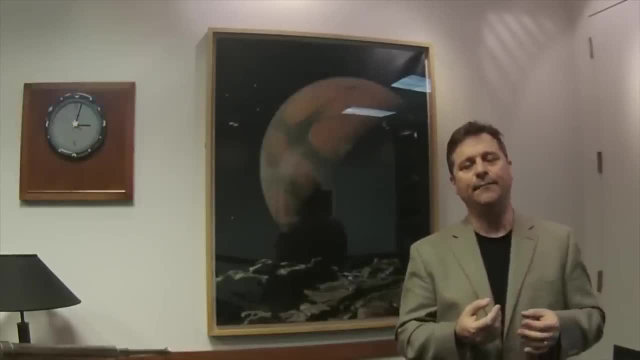 how we can build a model. In 140 AD, about 500 years, almost 500 years after, 400 years after Aristotle, the Greek philosopher, mathematician, Claudius Ptolemaeus wrote his Almagest and the Almagest. 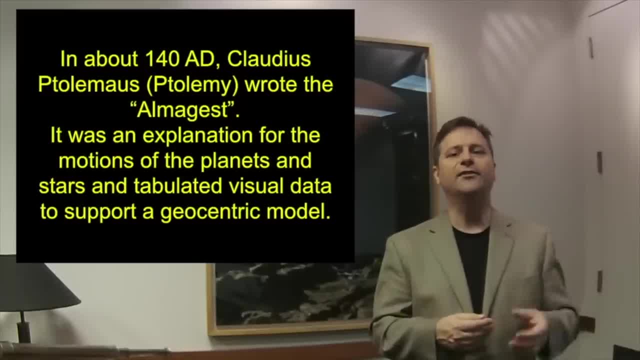 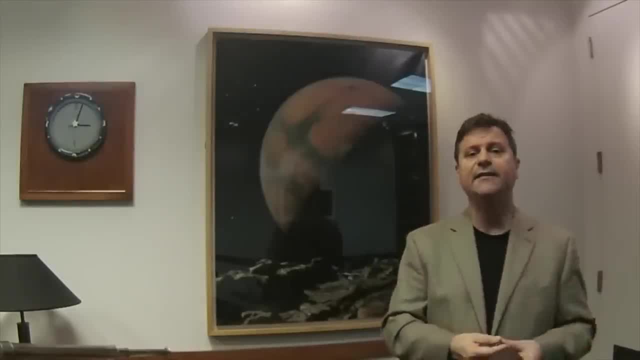 was an enormous, enormous undertaking where he plotted the charts of the heavens and tried to determine how things actually moved, And so he created a model of the cosmos, the geocentric model, that held sway for almost a thousand years, Actually 1500 years, All the way up through Galileo's time and beyond. 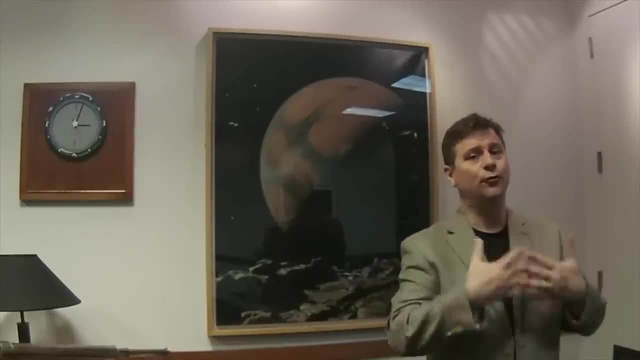 That the earth was at the center. So this is an incredibly important thing. So let's see. what did he do? Okay, so first Ptolemy posited, along with Aristotle, that the earth was at the center. Alrighty, so then he wanted to see how things moved. 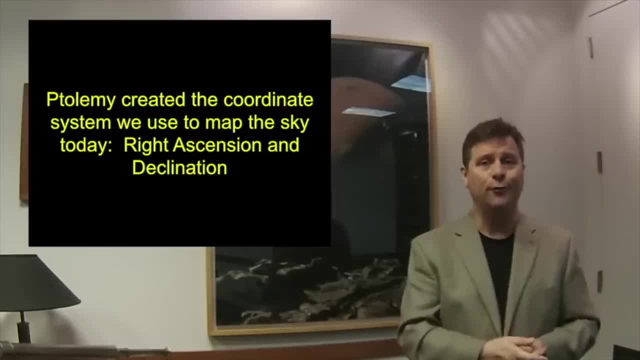 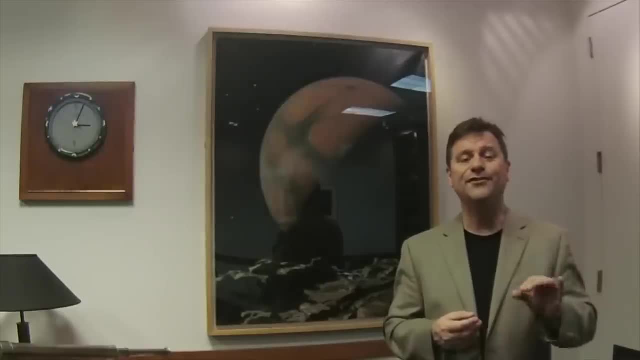 So he created a coordinate system, the equatorial coordinate system, which is the right ascension and declination, and he used the right ascension and declination of the stars and planets to determine the positions. Yep, that's where that coordinate system comes from. It comes from 140 AD. 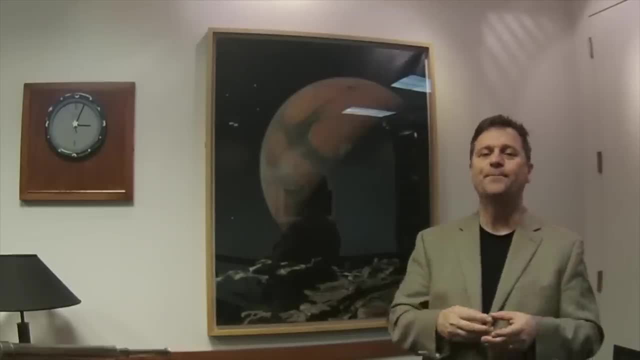 That's an old, old, old coordinate system, Anyway. so what did he do? He posited that around, that around the earth is at the center and in order to see both the prograde motion and the retrograde motion of the planets. here's what he posited. 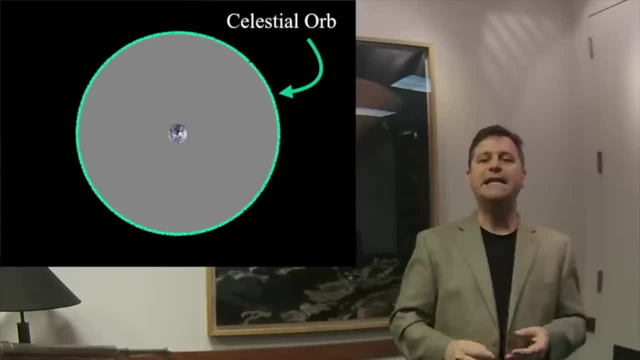 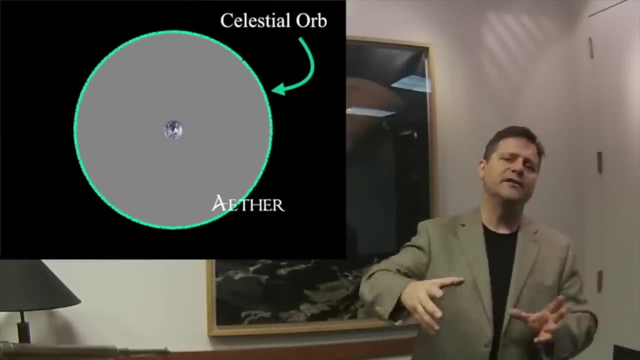 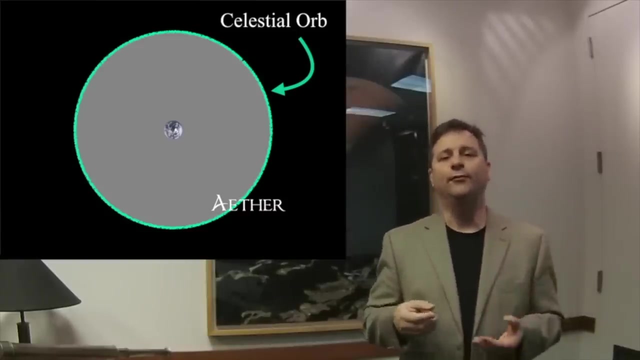 must occur. Every planet must be embedded in some orb and the orb must be made of some ether. And this ether is in a circle that surrounds the earth. and embedded in that orb of ether, the planet rides on a circular orbit called a deferent. The deferent is: 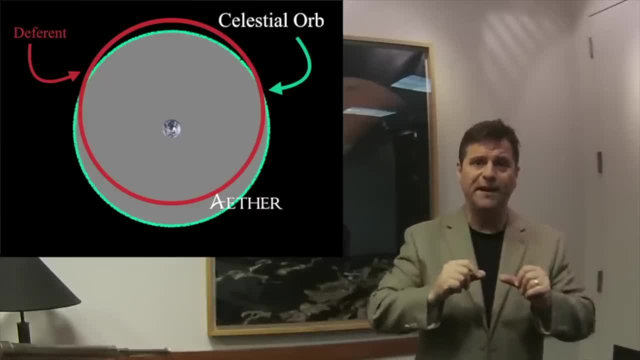 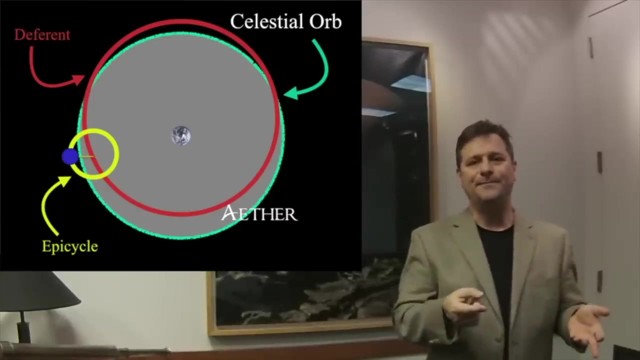 actually the orbit that it rides upon, and it's a perfect circle. Now, the planet itself doesn't actually ride on the deferent inside of the ethereal orb, but what it does is it rides on an epicycle on top that's centered on the deferent. So you've got this epicycle, that's on. 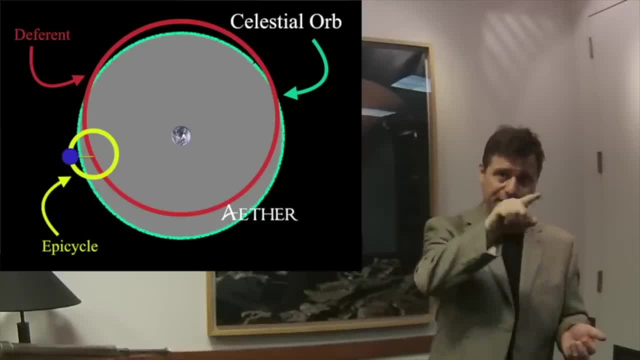 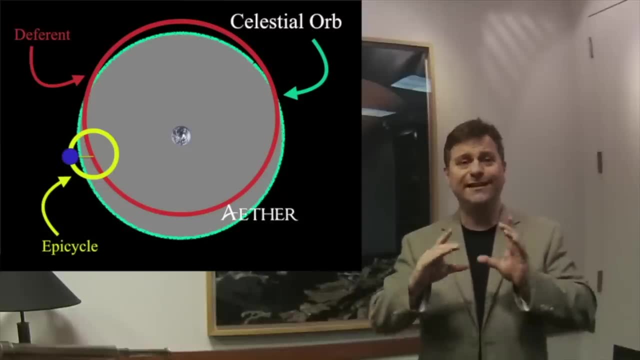 the deferent. so as the planet goes around the earth, it does these little loop-de-loops all the way around. So we've got these little loop-de-loops. In addition to that, the earth is not exactly at the center, but offset, And so the offset is offset by a little. 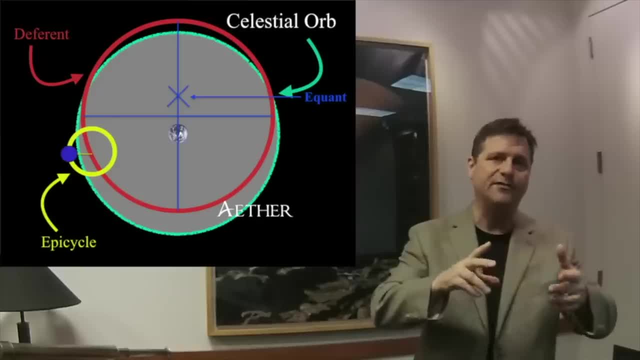 bit of distance and each of the planets has a different offset from center of the earth. So the earth isn't truly at the center, according to Ptolemy. Well, it's actually: the center of it is actually between the earth. 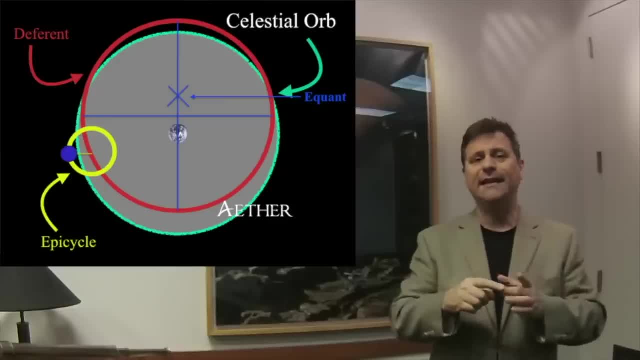 and a place called an equant, And an equant is a place that's equidistant from the center. So he posited a little of the earth here. equant is there. there's the center of the deferent. it rides around this deferent like this, and then it rides on epicycles around. 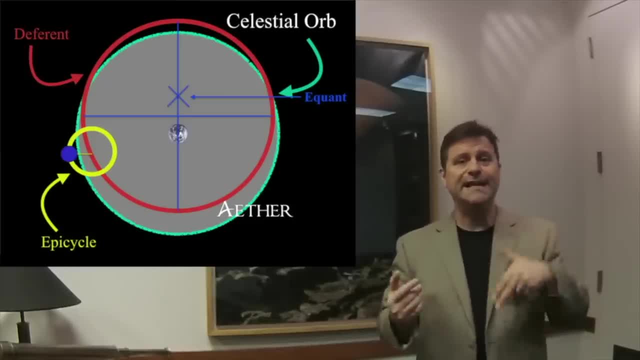 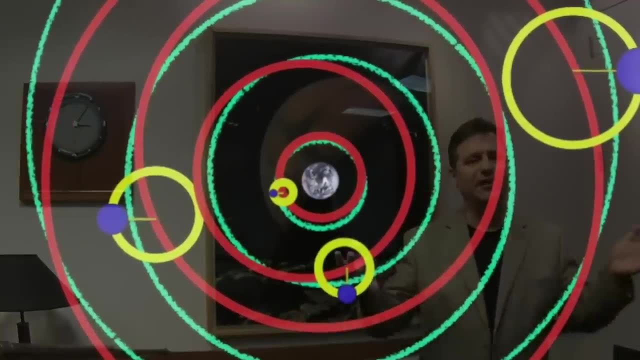 the deferent. It's a fairly complicated system and every single planet had its own set of epicycles, deferents and equants. Every single one of them did, And the earth was offset from the equants, from each one of them. In fact, in order to 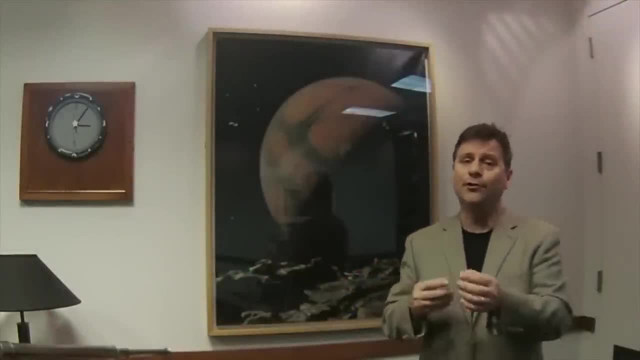 see the patterns of Mercury and Venus. Mercury and Venus had to have their deferents ride in between the sun and earth, So it was an even odd thing, because Venus was between the earth and the sun in order to always stay in the position of the sky that it was seen in, Alright. so this is a very 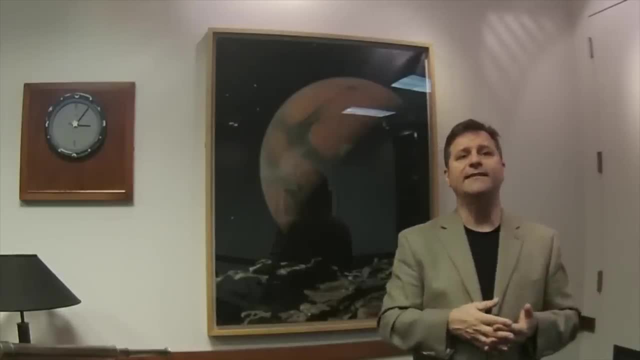 complicated system. We would look at this and say it's very complicated, extremely complicated, and the reason why almost nobody back then was a public speaker about astronomy- because it took years and years of work to really understand what the Almagest actually says and how to actually